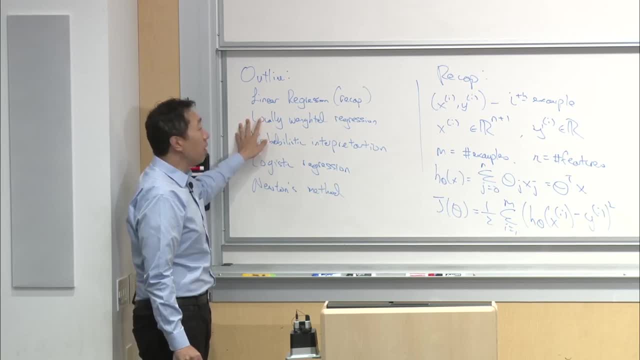 um, talk about locally weighted regression, which is a a way to modify linear regression to make it fit very non-linear functions. so you aren't just doing straight lines And then, uh, we'll talk about probabilistic interpretation of linear regression. 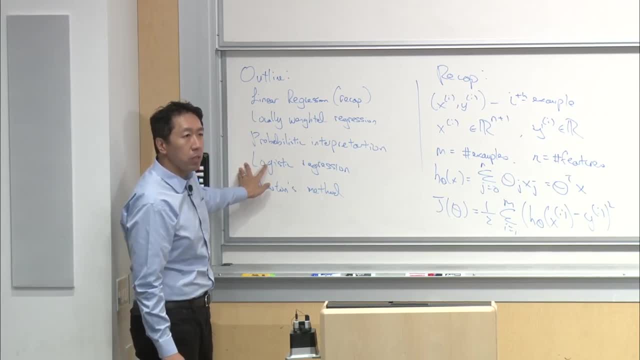 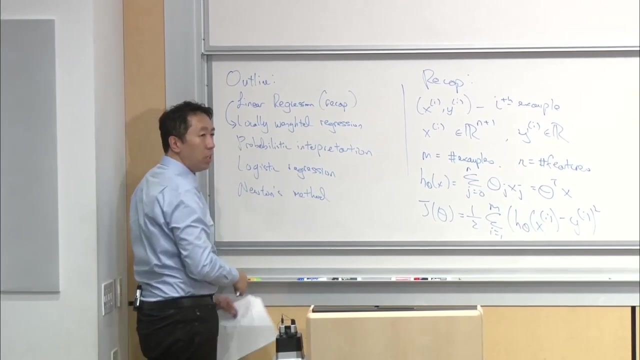 and that will lead us into the first classification algorithm you see in this class, called logistic regression, And we'll talk about an algorithm called Newton's method. uh, for logistic regression. And so the dependency of ideas in this class is that um locally weighted regression will depend on what you've learned in linear regression. 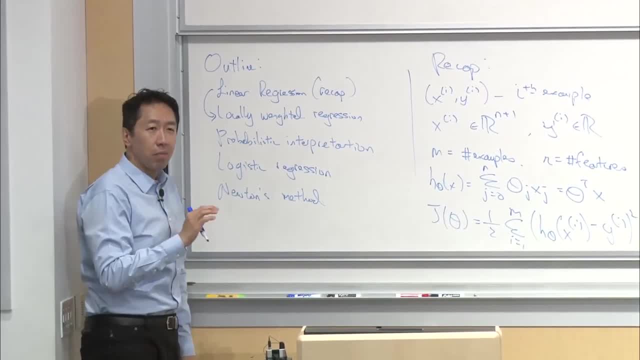 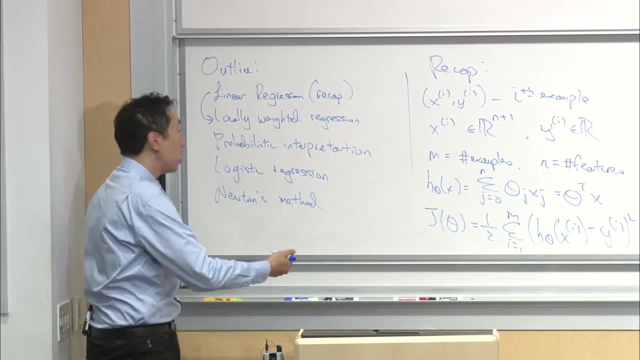 And then, um, we're actually gonna just cover the key ideas of locally weighted regression and let you play some of the ideas yourself in the um problem set, one which we release later this week- And then, um, I guess, give a probabilistic interpretation of linear regression. 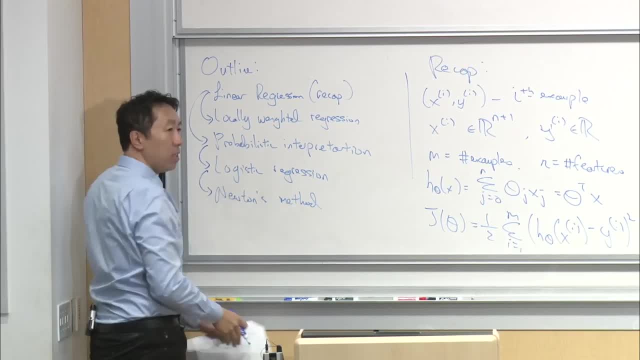 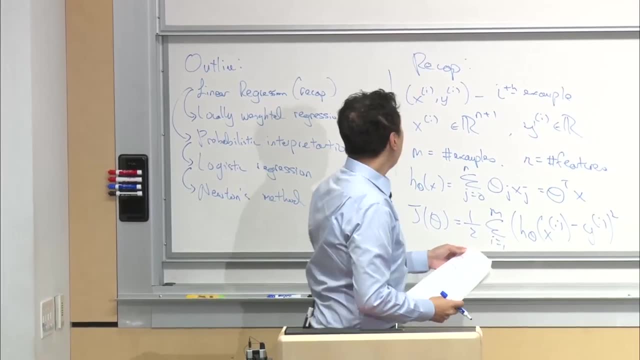 logistic regression will depend on that um and Newton's method is for logistic regression. okay, To recap the notation you saw on Wednesday, we use this notation x, i, comma, i, y, i, y, i to denote a single training example where 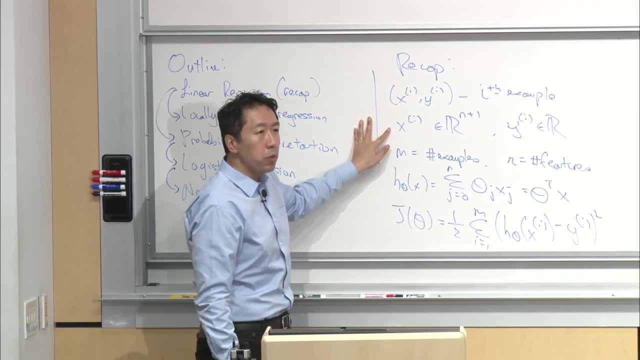 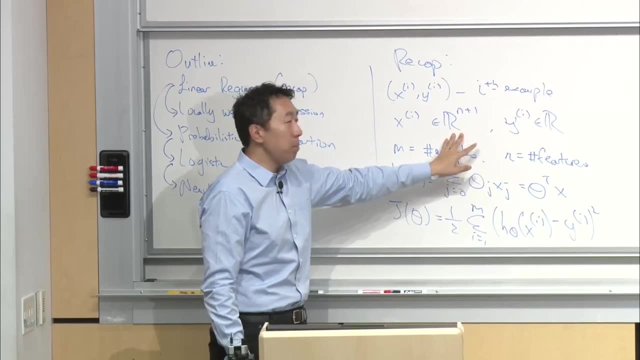 uh, x i was n plus 1-dimensional. So if you had two features- the size of a house and the number of bedrooms- then x i would be 2 plus 1, would be 3-dimensional, because we had introduced a new. 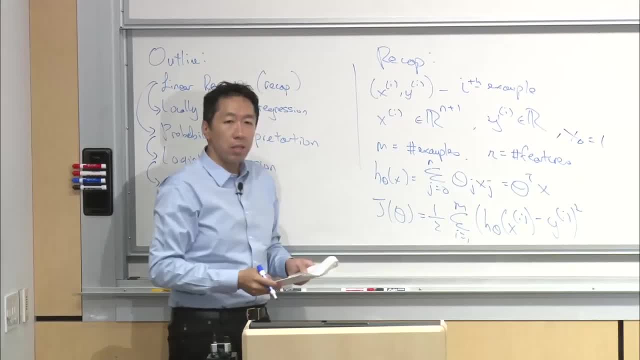 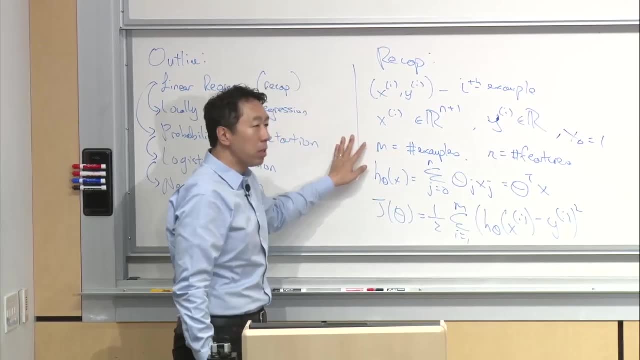 uh, sort of fake feature, x, 0,, which was always set to the value of 1.. Uh, and then y, i, in the case of regression, is always a real number. n was the number of training examples. n was the number of features. 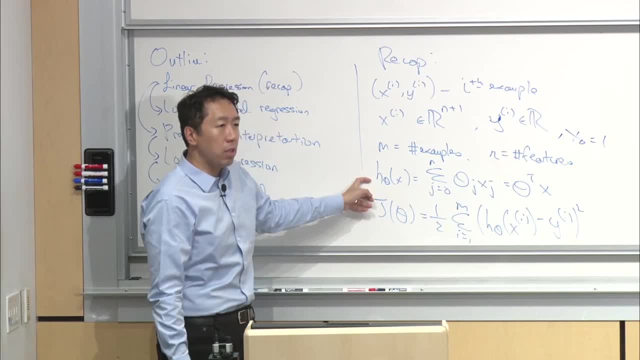 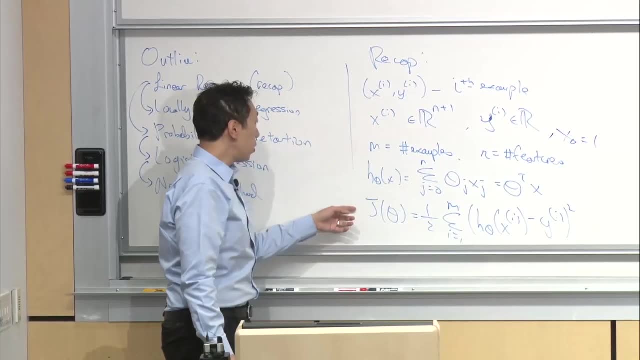 And uh, this was the hypothesis, right, It's a linear function of the features x, um, including this feature x 0, which is always set to 1.. And uh, j was the cost function you would minimize. 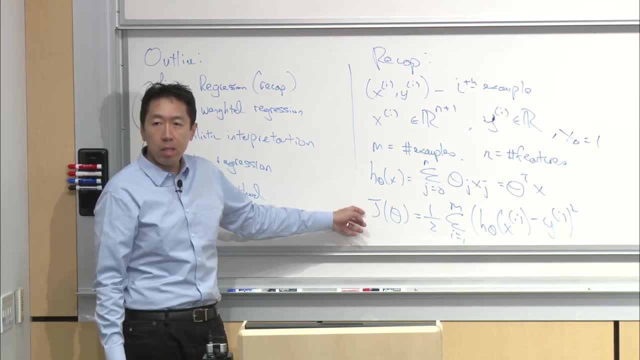 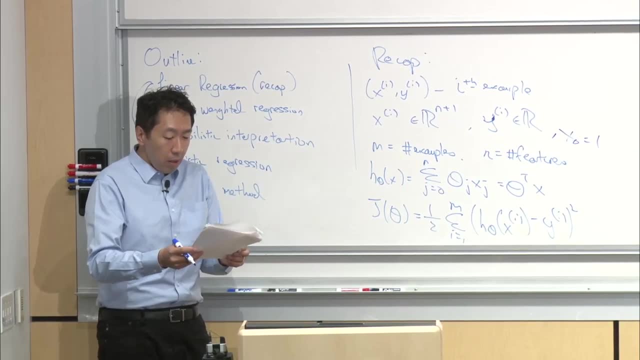 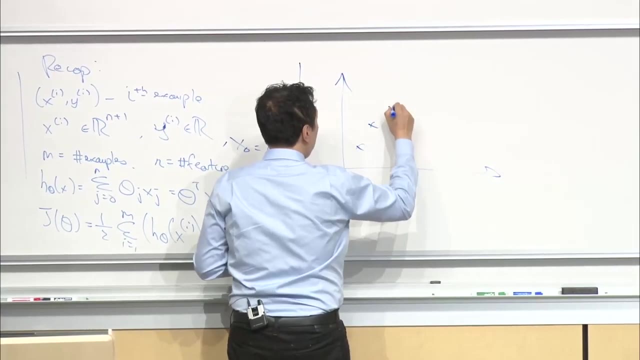 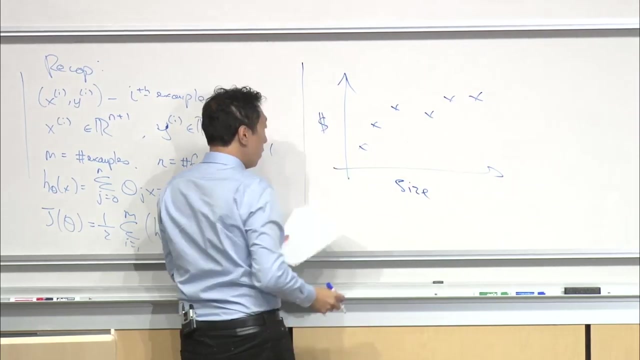 You minimize this as function of j to find the parameters theta for your straight line fit to the data. okay, So that's what you saw last Wednesday. Um, now, if you have, if you have a dataset that looks like that, where this is the size of a house and this is the price of a house, 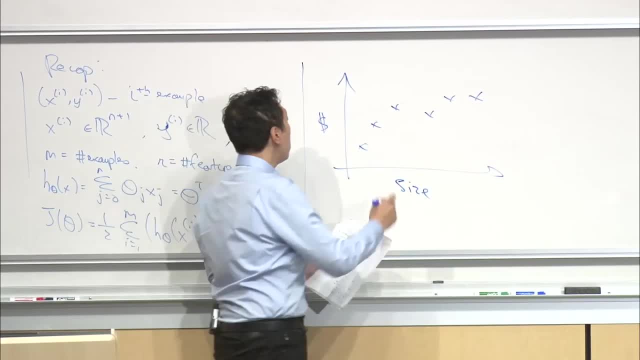 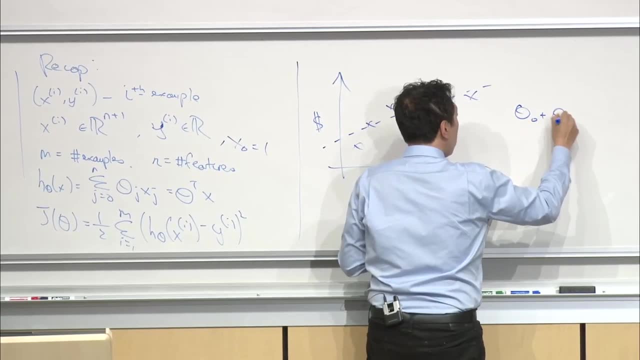 what you saw on Wednesday, last Wednesday, was an algorithm to fit a straight line right to this data. So the hypothesis was of the form: theta 0 plus theta 1, x or x, or theta 1 x- 1, right. 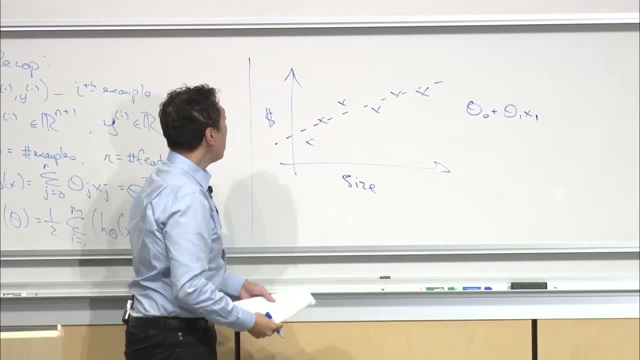 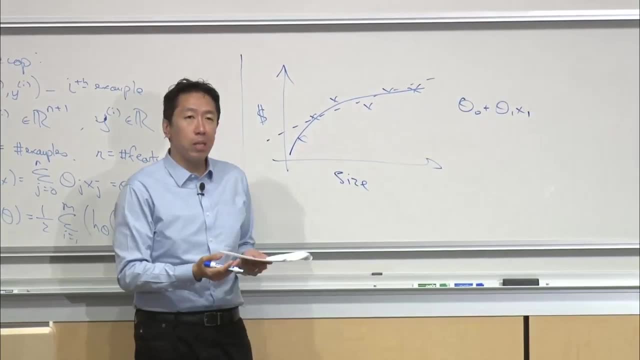 Same thing, Um, but with this dataset maybe it actually looks. you know, maybe the data looks a little bit like that, And so one question that you have to address when uh fitting models to the data is: what are the features you want? 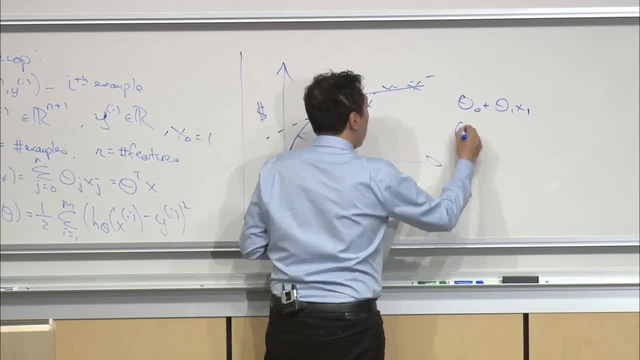 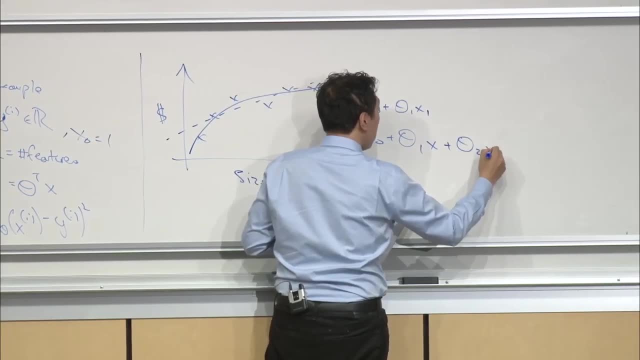 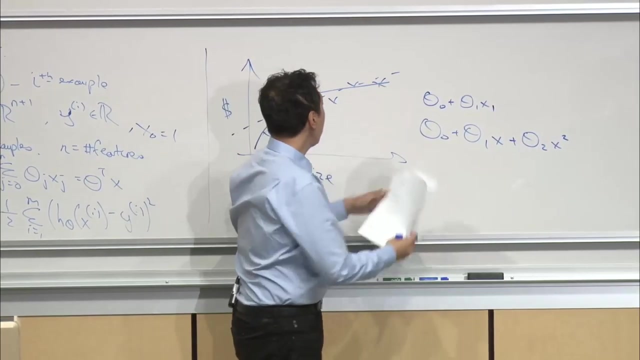 Do you want to fit a straight line to this problem? Or do you want to fit a hypothesis of the form um theta 1 x plus theta 2 x squared, since this may be a quadratic function right Now? the problem with quadratic function is that a quadratic function eventually starts. 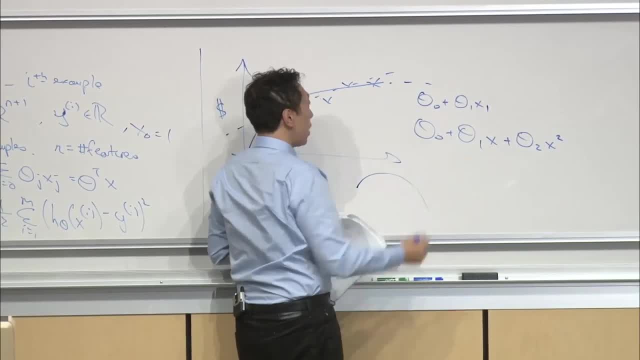 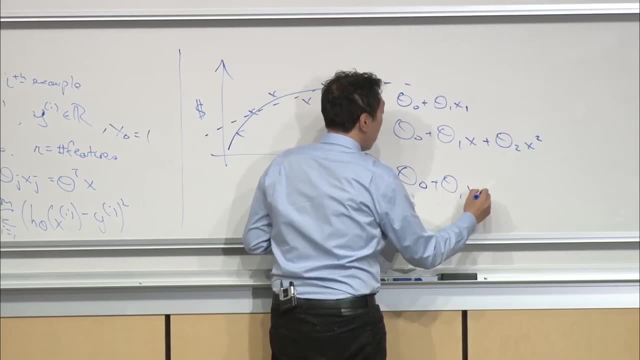 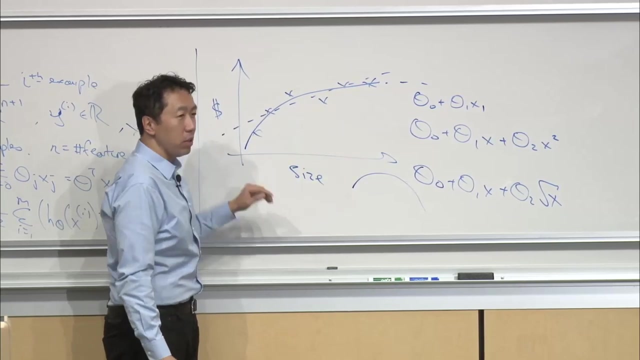 you know, curving back down. Well, that would be a quadratic function that starts curving back down. so maybe you don't want to fit a quadratic function, Uh, instead, maybe you want, um, to fit something like that If- if housing prices sort of curve down a little bit. 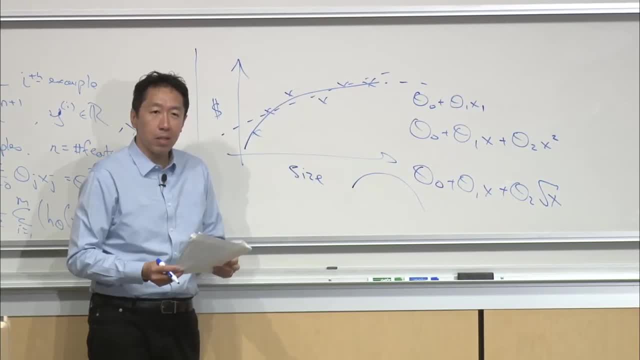 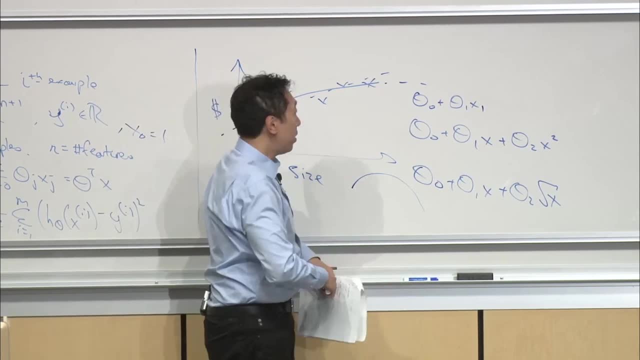 but you don't want it to eventually curve back down the way a quadratic function would right. Um, so, oh, and- and if you want to do this, the way you would implement this is you define the first feature. x1 equals x. 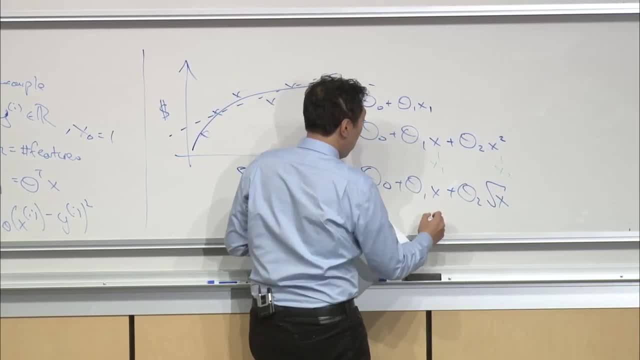 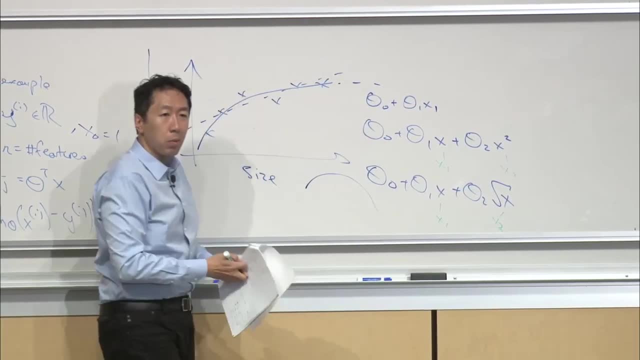 and the second feature, x2 equals x squared, or you define x1 to be equal to x and x2 equals square root of x right, And by defining a new feature, x2, which can be the square root of x or square root of x. 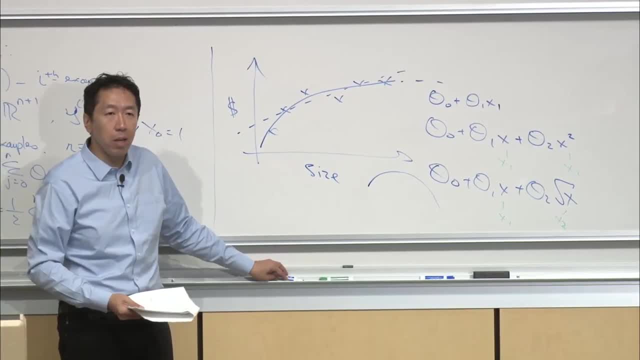 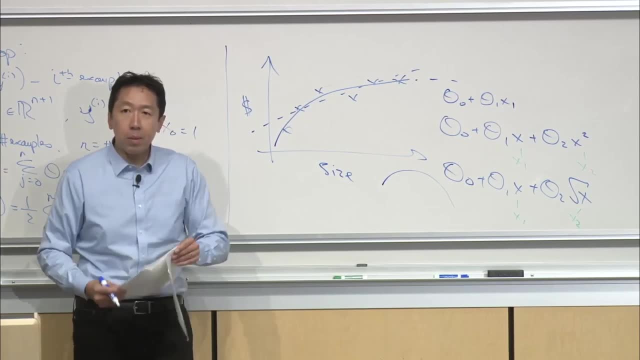 then the machinery that you saw from Wednesday of linear regression applies to fit these types of um, these types of functions, to the data. So later this quarter you'll hear about feature selection and algorithms, which is a type of algorithm for automatically deciding. 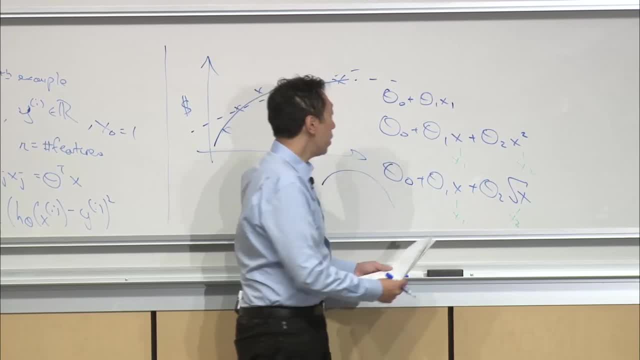 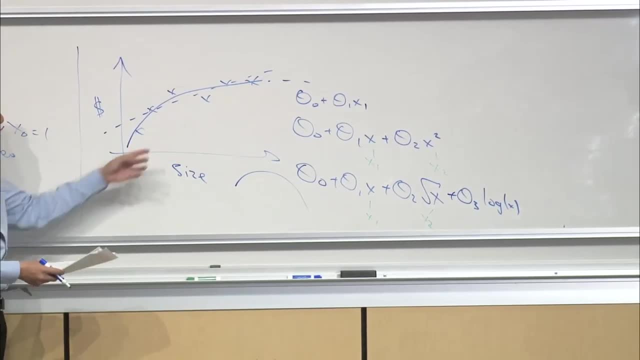 do you want x squared as a feature, or square root of x as a feature? or maybe you want um longer of x as a feature? right, But what set of features? um does the best job fitting the data that you have. if it's not fit well, by a perfectly straight line. 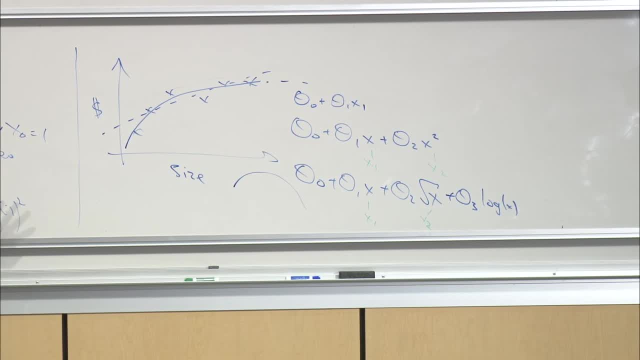 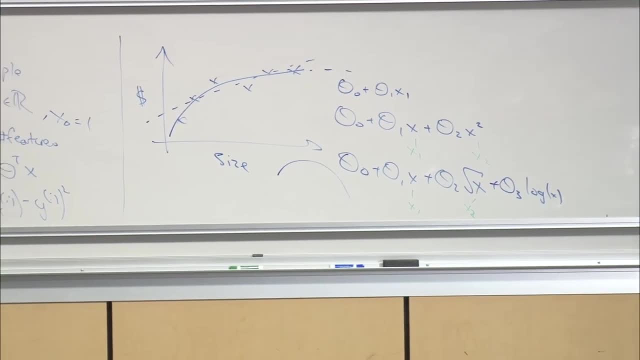 Um, what I'd like to do today is- so- so you hear about feature selection later this quarter. What I want to share with you today is a different way of accessing this out- this problem of what if the data isn't just fit well by a straight line. 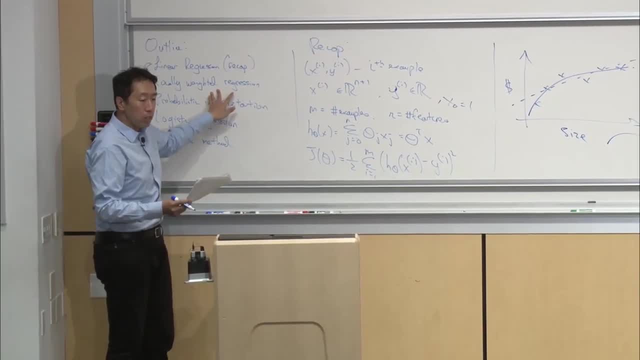 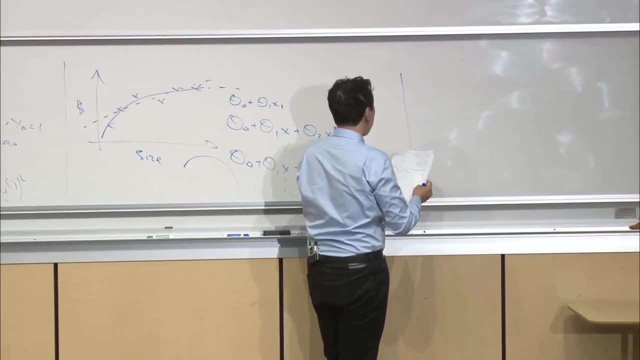 And, in particular, I want to share with you an idea called uh- locally weighted regression, or locally weighted linear regression. So let me use a slightly different um example to illustrate this um, which is uh, which is that you know. 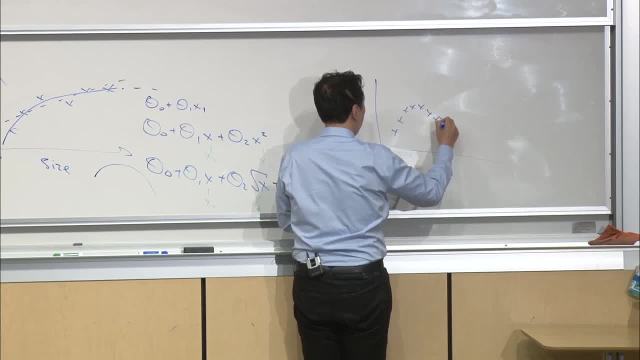 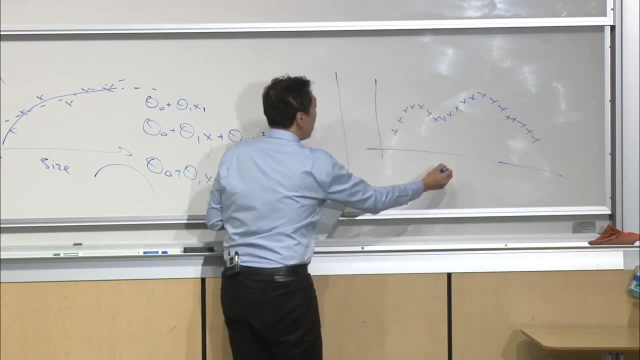 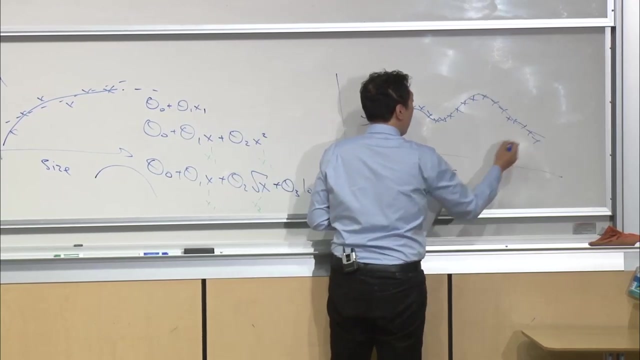 if you have a dataset that looks like that, right, So it's pretty clear What the shape of this data is. um, but how do you fit a curve that, you know, kind of looks like that, right, And it's- it's actually quite difficult to find features. 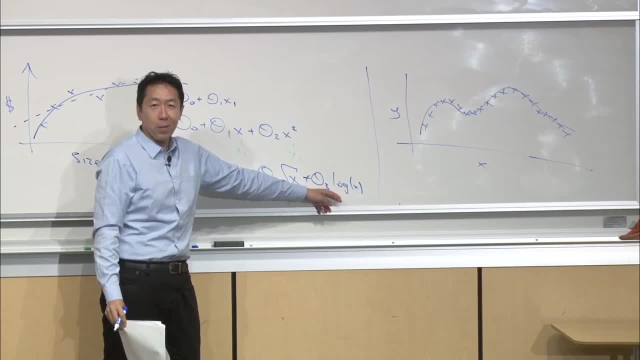 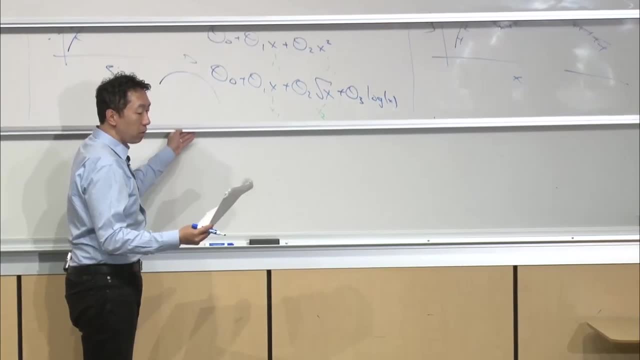 Is it square root of x? log of x, x, cubed like third root of x, x to the power of 2 thirds. But what is the set of features that lets you do this? So we'll sidestep all those problems with an algorithm called. 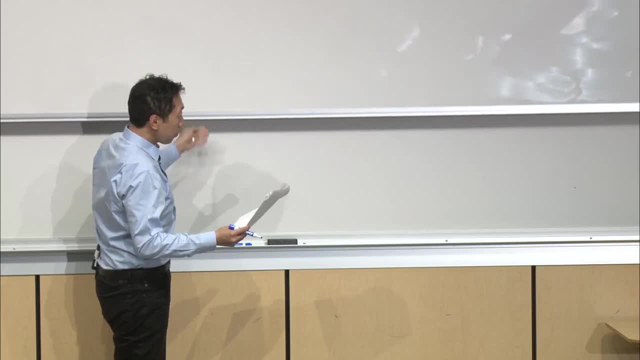 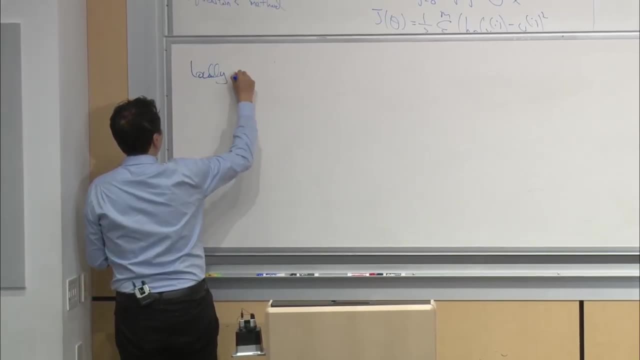 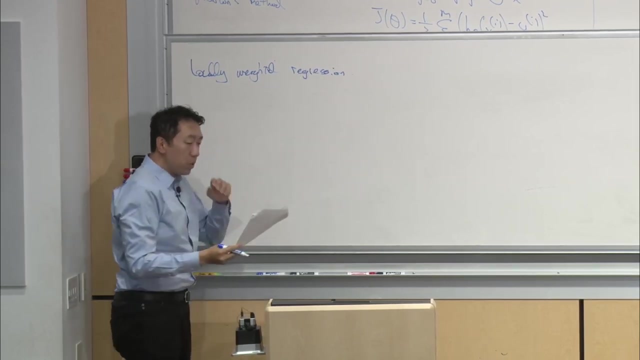 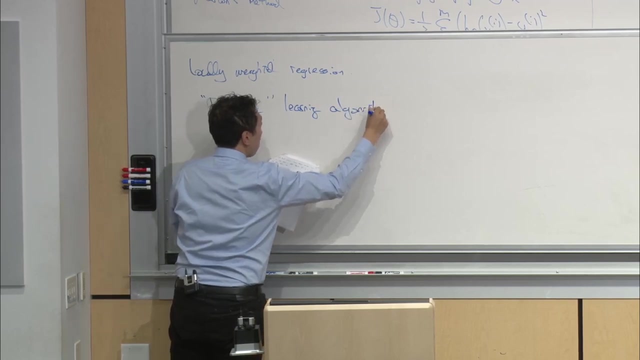 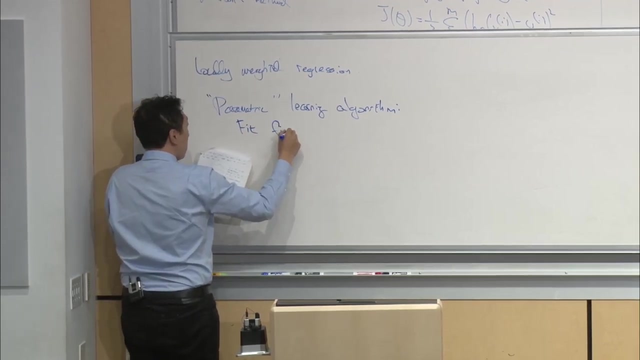 uh, locally weighted regression, Um. and to introduce a bit more machine learning terminology: um. in machine learning we sometimes distinguish between parametric learning algorithms and non-parametric learning algorithms. But in a parametric learning algorithm there's a? uh you fit some fixed set of parameters. 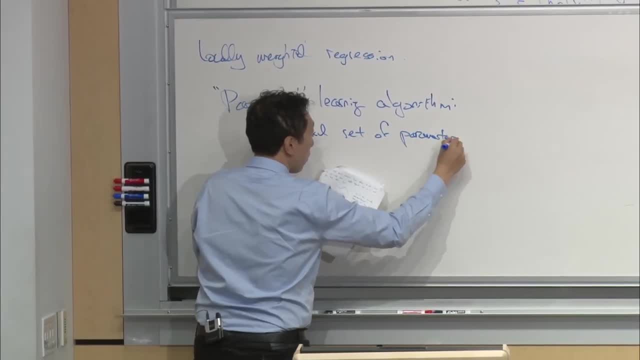 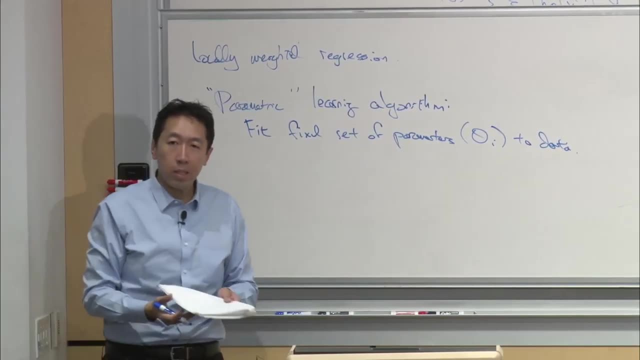 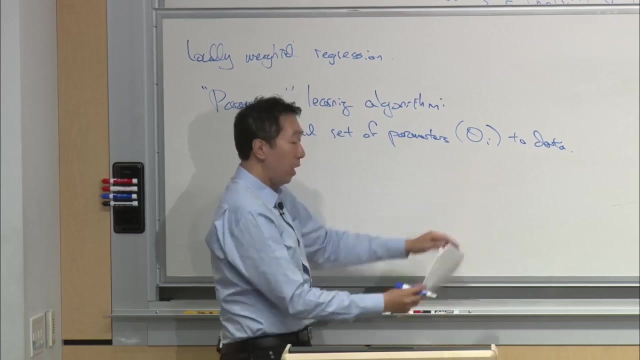 Uh, such as theta i to theta, And so linear regression, as you saw last Wednesday, is a parametric learning algorithm Because there's a fixed set of parameters, the theta i, so you fit to theta and then you're done right. 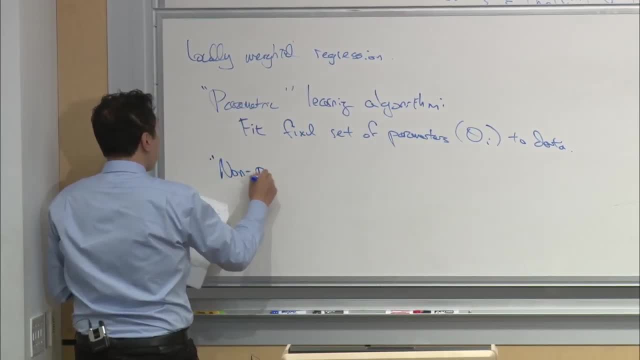 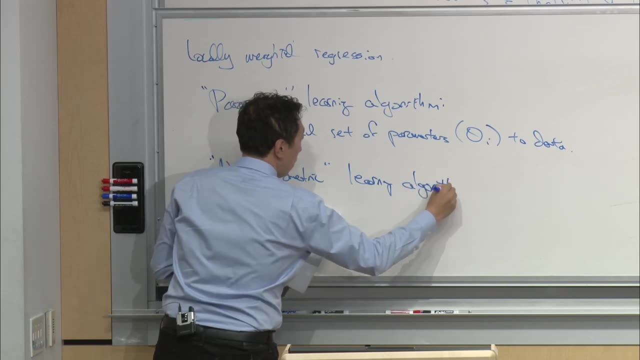 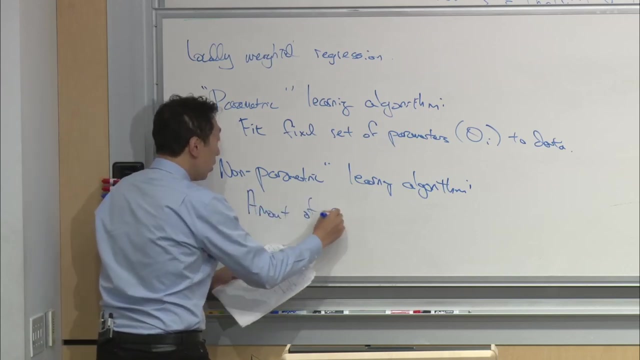 Locally weighted regression will be our first exposure to a non-parametric learning algorithm, to a non-parametric learning algorithm, to a non-parametric learning algorithm, um, and what that means is that the amount of um data slash parameters. 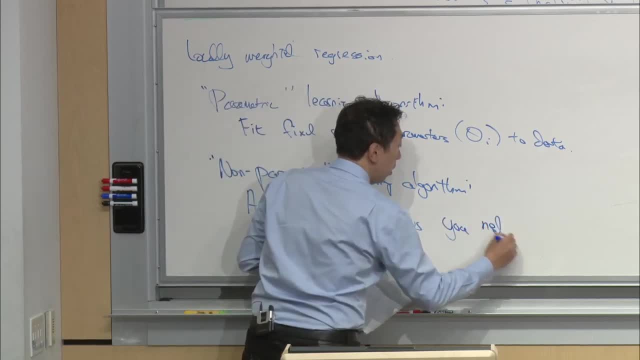 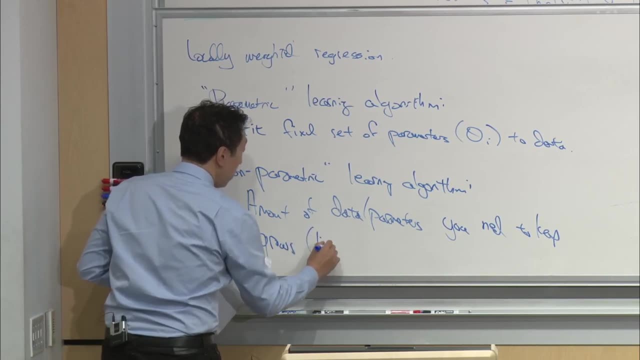 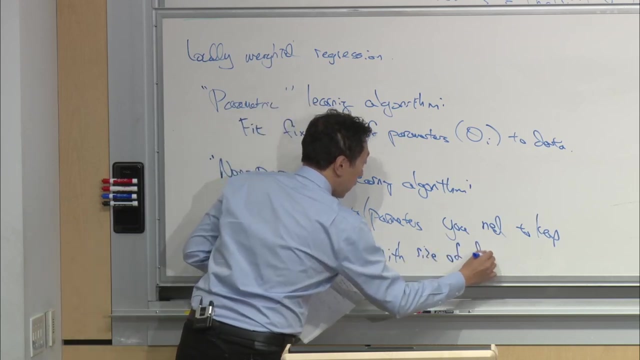 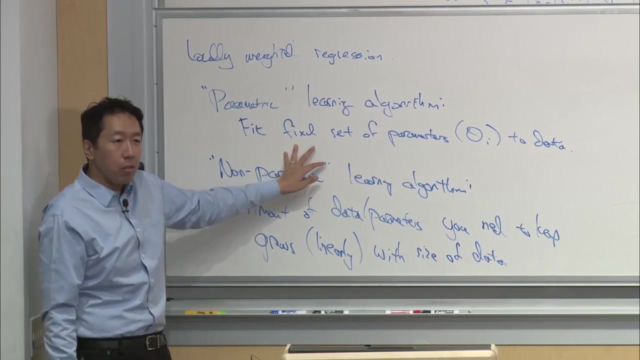 uh, you need to keep grows and in this case it grows linearly with the size of the data, with size of the training set. okay, So with a parametric learning algorithm, no matter how big your training, uh, your training set is. 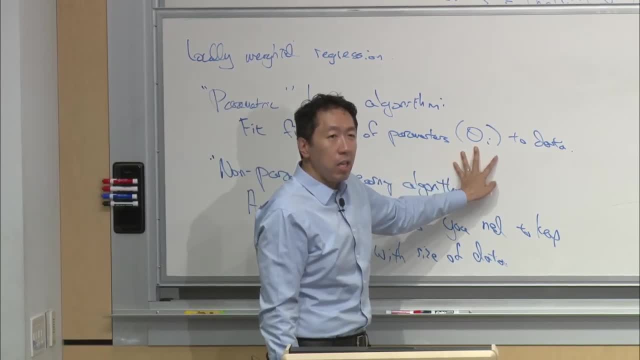 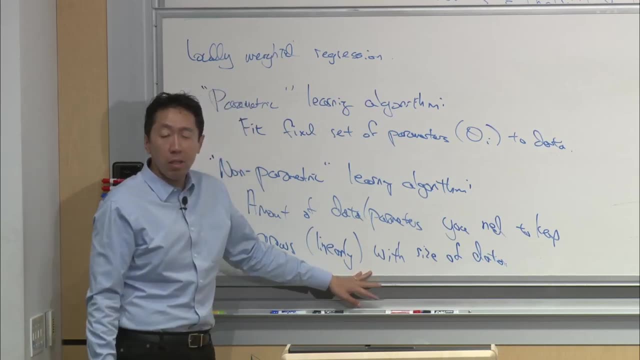 you fit the parameters theta i, then you could erase the training set from your computer memory and make predictions just using the parameters theta i In a non-parametric learning algorithm which we'll see in a second. the amount of stuff you need to keep around in computer memory. 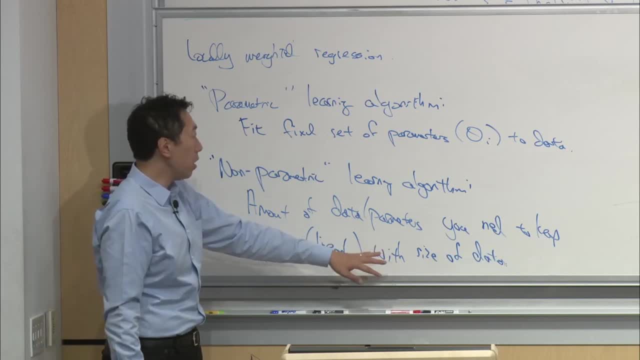 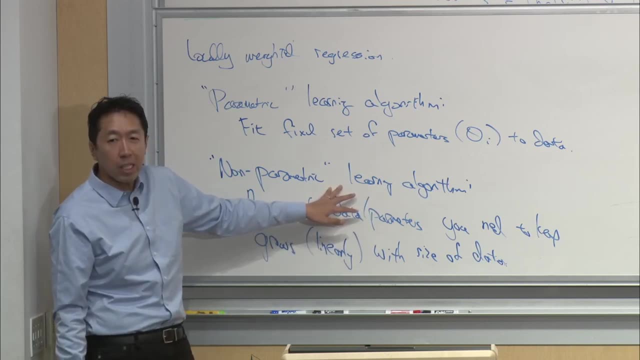 or the amount of stuff you need to store around grows linearly as a function of the training set size. Uh, and so this type of algorithm is, you know it may- may- may not be great if you're a, if you have a really, really massive data set. 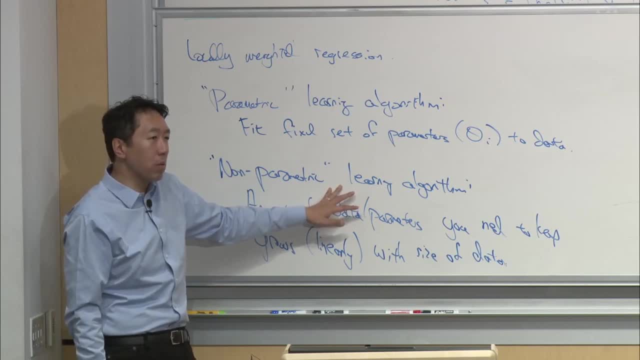 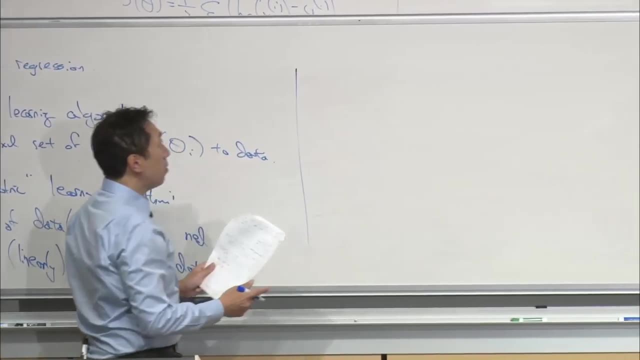 because you need to keep all of the data around, you know, in computer memory or on disk, just to make predictions. okay, So, but we'll see an example of this And, uh, one of the effects of this is that 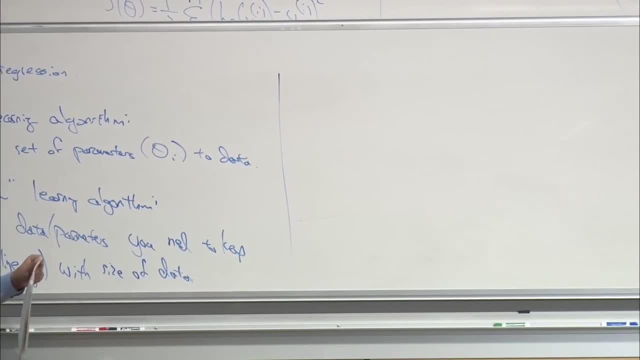 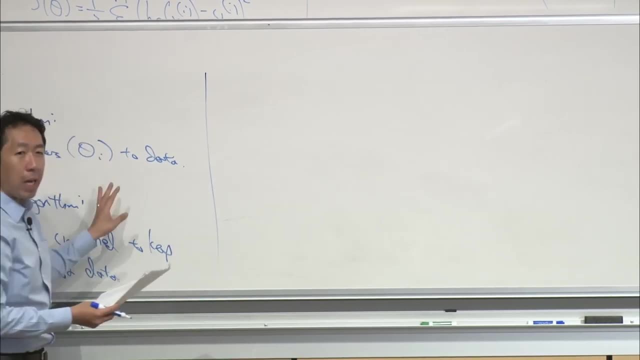 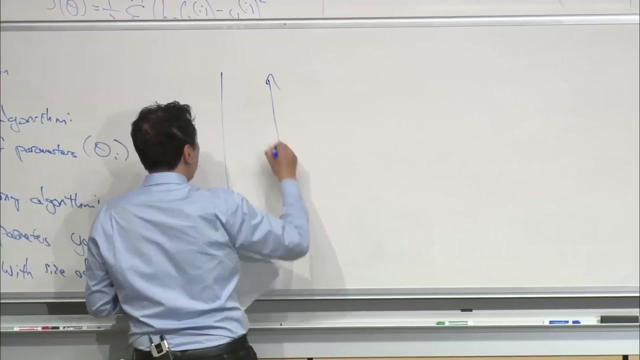 will that- it'll- it'll be able to fit that data that I drew up there. uh, quite well, without you needing to fiddle manually with features. Um and again, you get to practice implementing locally weighted regression at homework. So I'm gonna go over the high level ideas relatively quickly and then let you. 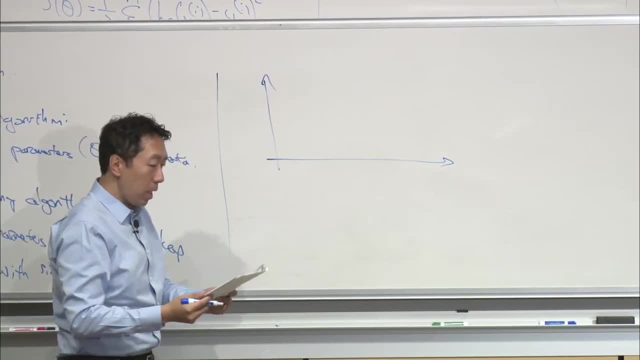 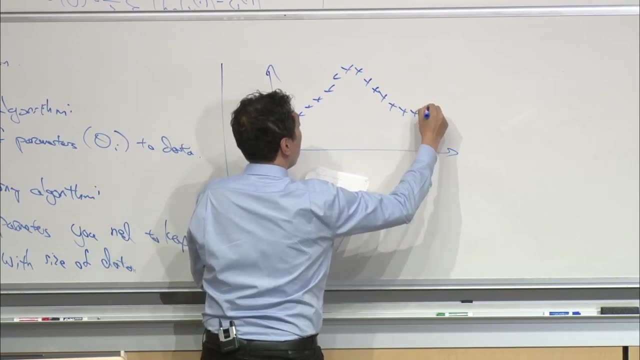 uh, uh, gain practice, uh, in the problem set. All right, So let me redraw that data set. Let me do something like this. Well, all right, So- so-. so say, you have a data set like this: 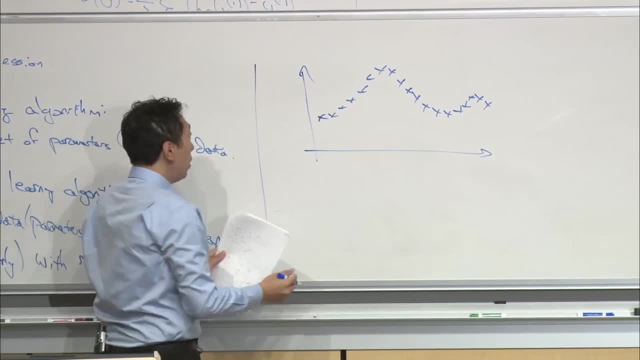 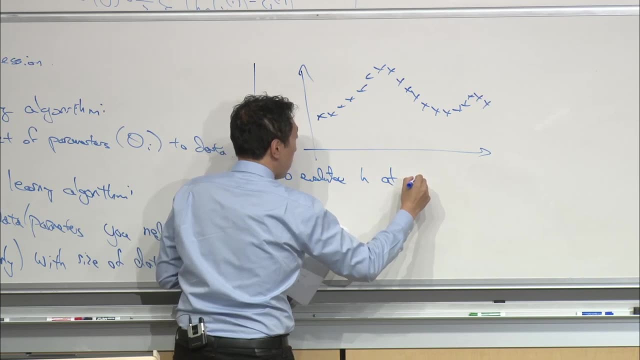 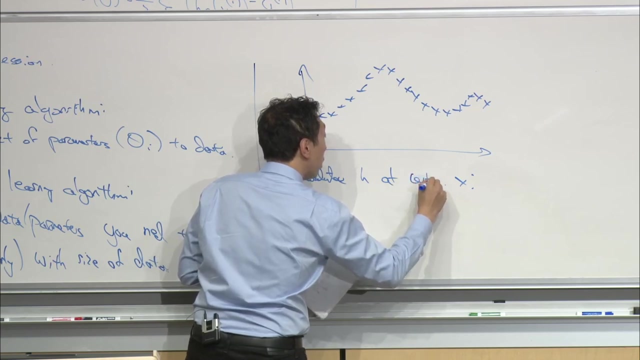 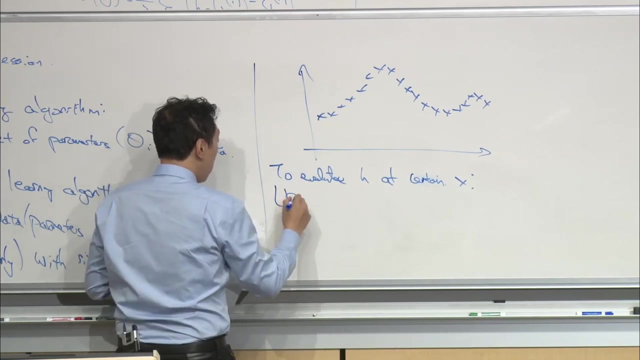 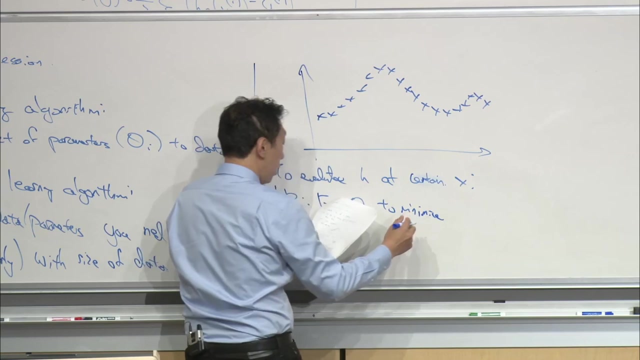 Um, now for linear regression. if you want to evaluate h at a certain value of the input, right, So to make a prediction at a certain value of x, what you- for linear regression, what you do is you fit Theta, you know. 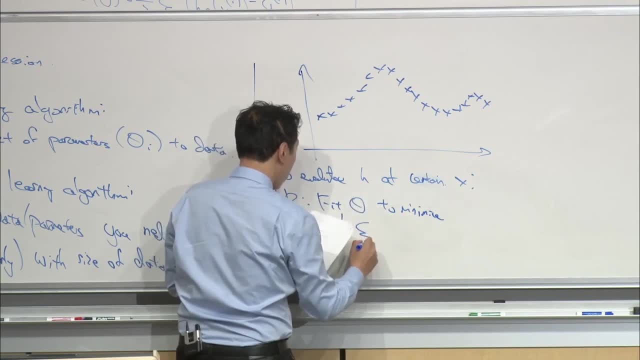 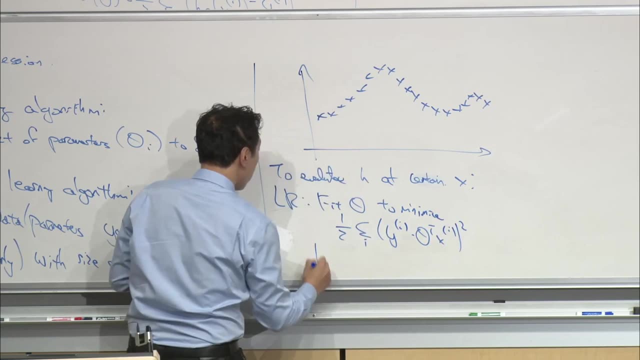 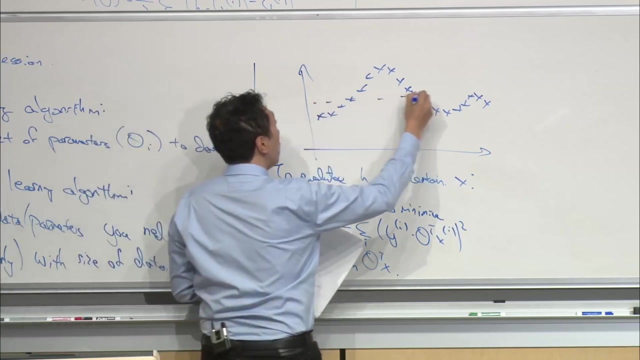 to minimize this cost function, Um, and then you're a term, So I'm gonna fix this, I'm gonna fix this, I'm gonna fix this, um, I'm gonna fix this. return Theta transpose X, right, So you fill the straight line and then you know. 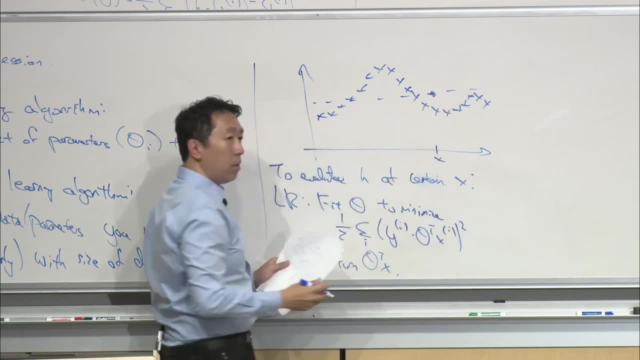 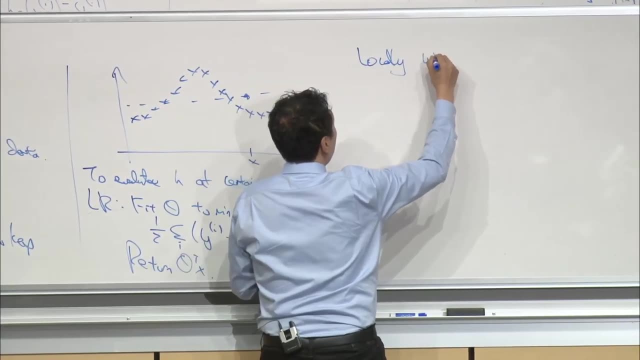 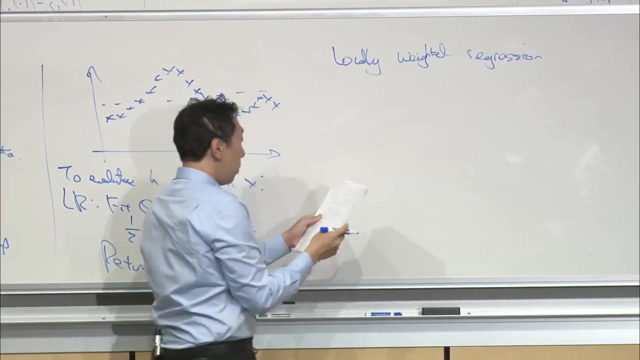 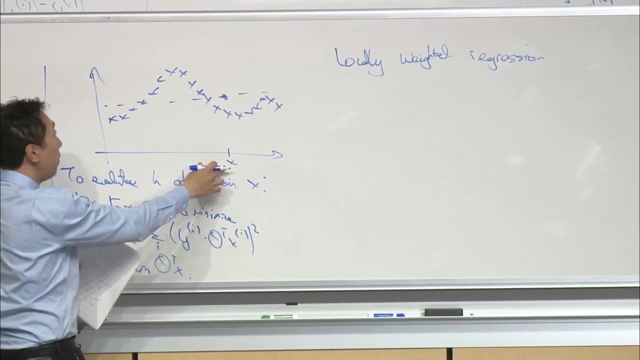 if you want to make a prediction at this value X, you then return Theta, transpose X For locally weighted regression. um, you do something slightly different, which is, if this is the value of X and you want to make a prediction around that value of X, 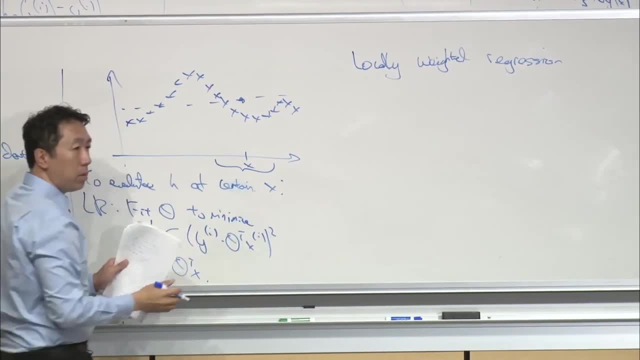 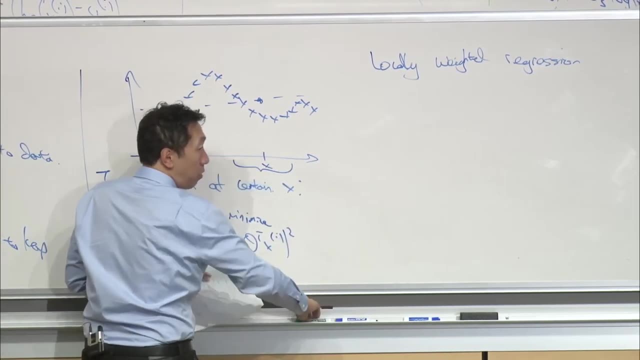 what you do is you look, in a lo- local neighborhood, at the training examples close to that point X where you want to make a prediction, And then, um, I'll describe this informally for now, but we'll- we'll formalize this in math in a second. 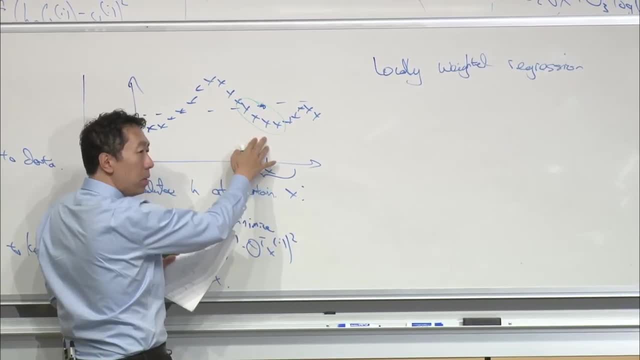 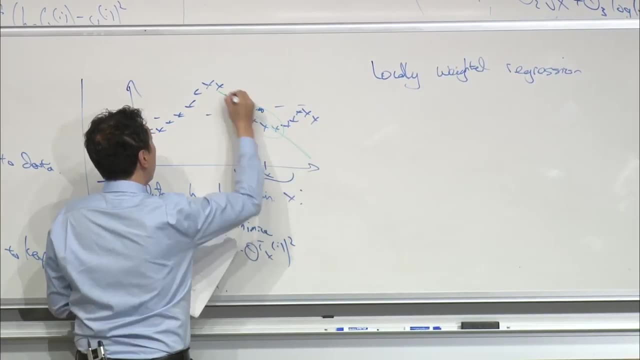 Um, but focusing mainly on these examples and you know, looking a little bit at further out examples, but really focusing mainly on these examples. you're trying to fill a straight line like that, Focusing on the- training examples that are close to where you want to make a prediction. 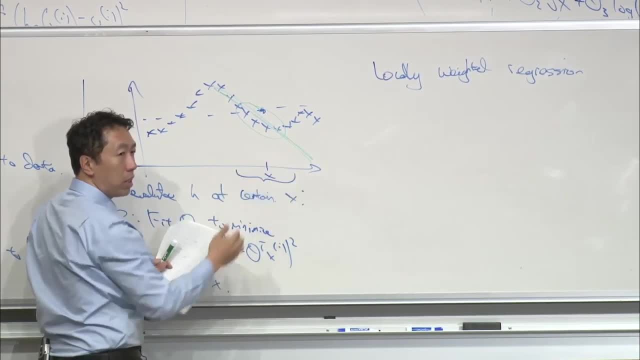 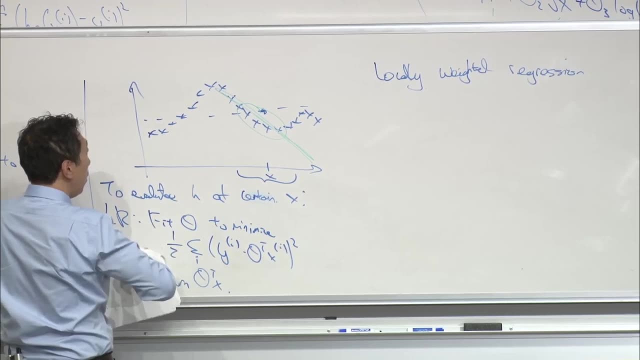 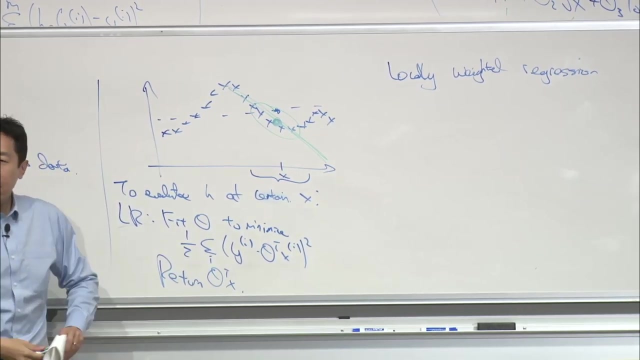 And by close I mean the values are similar. uh, on the X-axis, The X values are similar. And then to actually make a prediction, you will uh use this green line that you just fit to make a prediction at that value of X. okay. 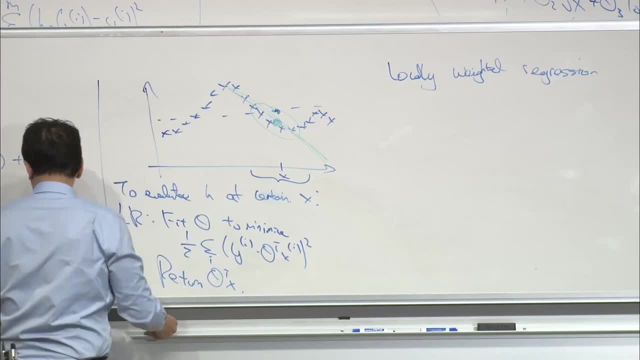 Now, if you want to make a prediction at a different point, um, let's say that you know the user now says, hey, make a prediction for this point. Then what you're gonna do is you're gonna make a prediction for this point. 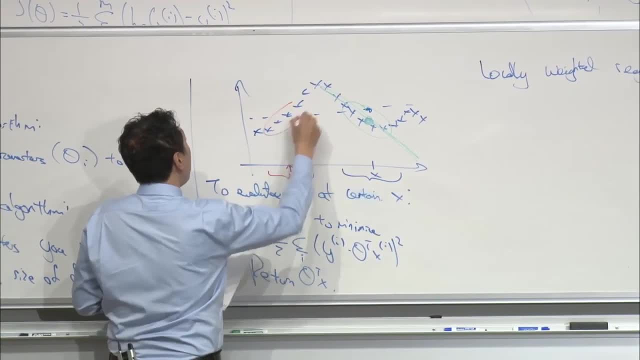 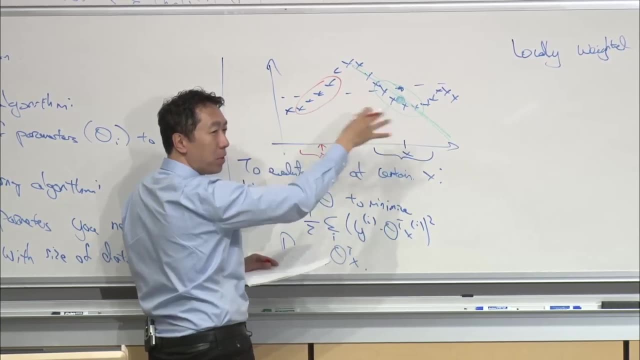 What you would do is you're gonna focus on this local area. kind of look at those points, Um, and when I say focus, say you know, put most of the weight on these points. but you kind of take a glance at the points further away. 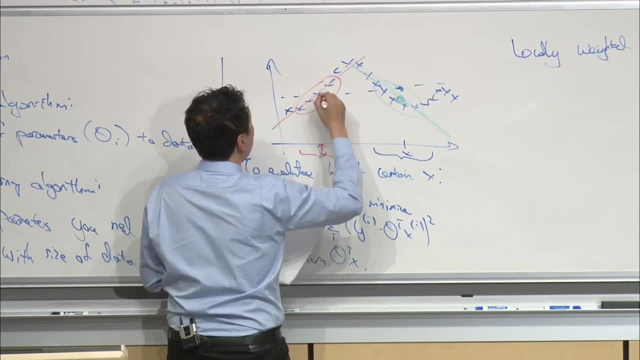 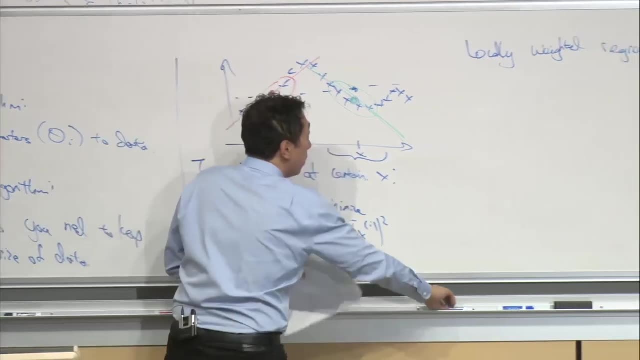 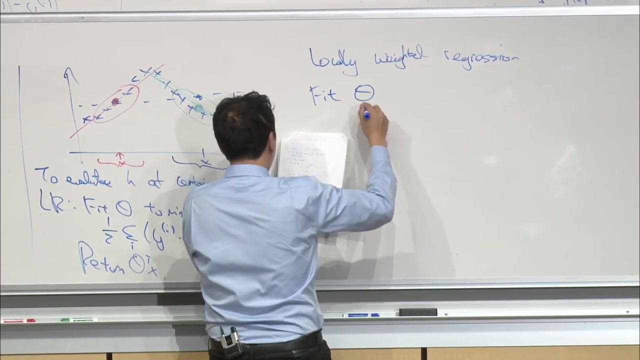 but most of the attention is on these- Fill the straight line to that, and then you use that straight line to make a prediction. okay, Um, and so to formalize this in locally weighted regression: um, you will fit Theta. 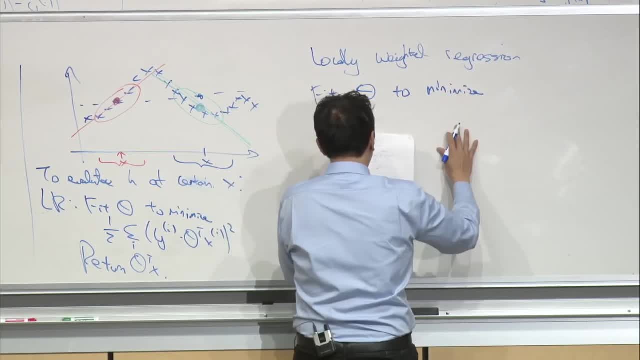 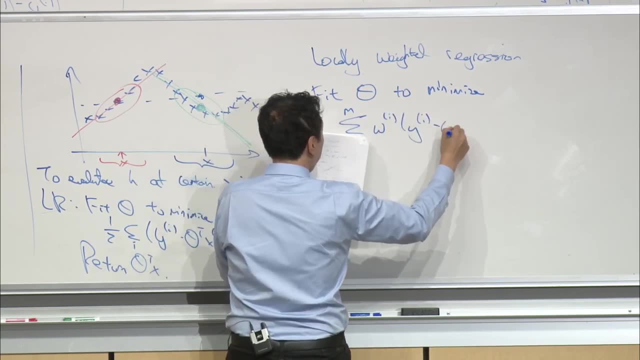 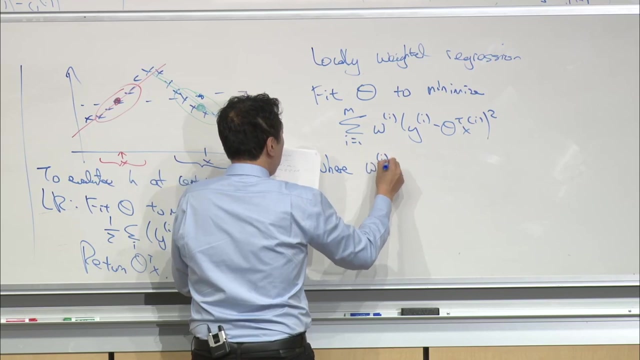 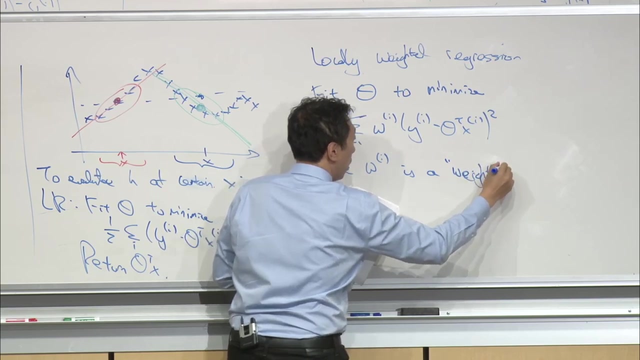 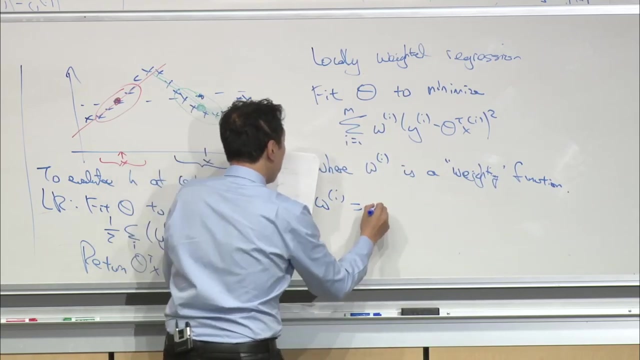 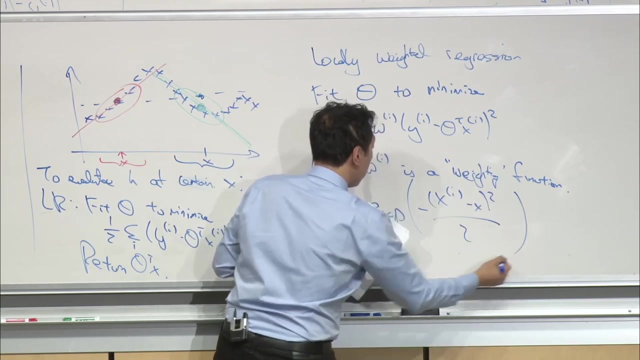 um to minimize a modified cost function Where wi is a weight function, Um, and so a good- well, default choice, a common choice of w. i will be this right: Um. I'm gonna add something to this equation a little bit later. 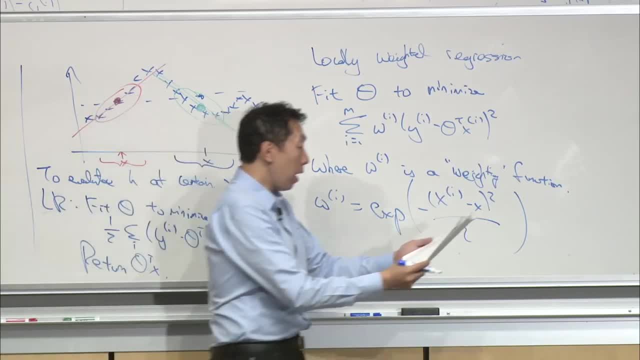 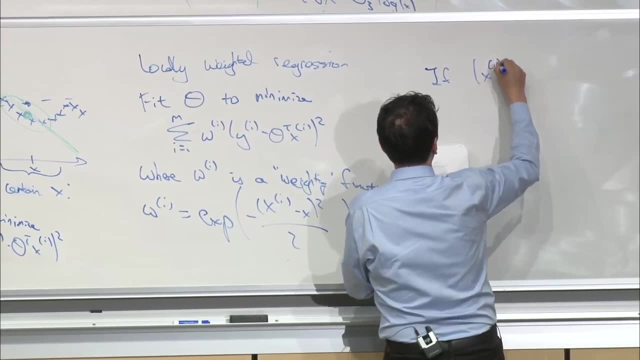 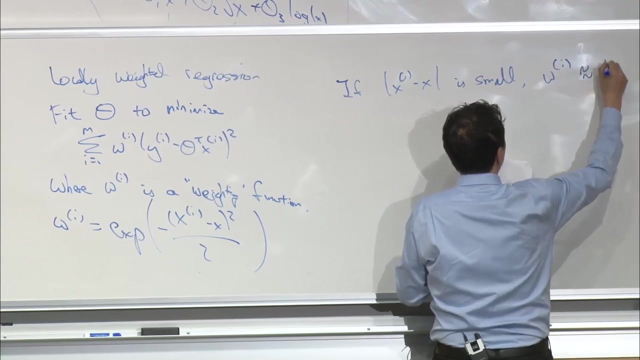 But, uh, w, i is a weighting function where, notice that this- this formula has um defining property, right, If x, i minus x is small, then the weight will be close to 1.. Because, uh, if x, i and x. 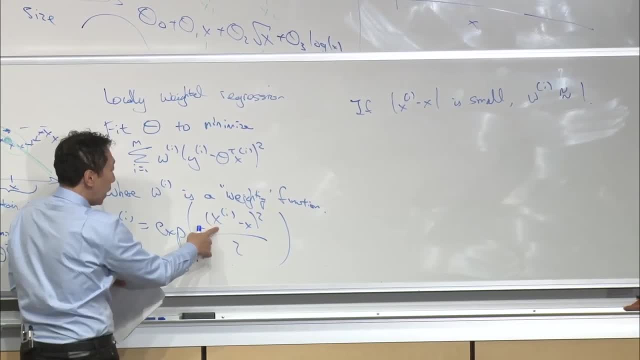 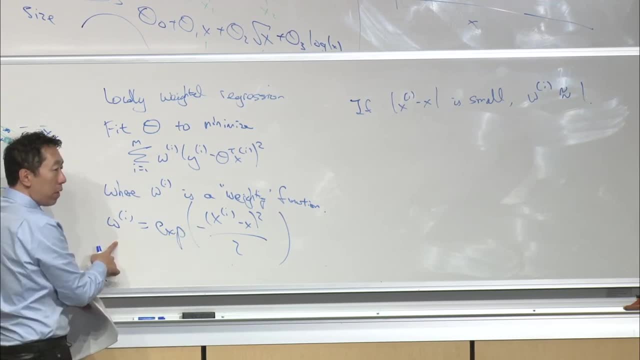 so x is the location where you want to make a prediction and x- i is the input- x for your i-th training example. So w? i is a weighting function. um, there's a value between 0 and 1 that tells you how much should you pay. 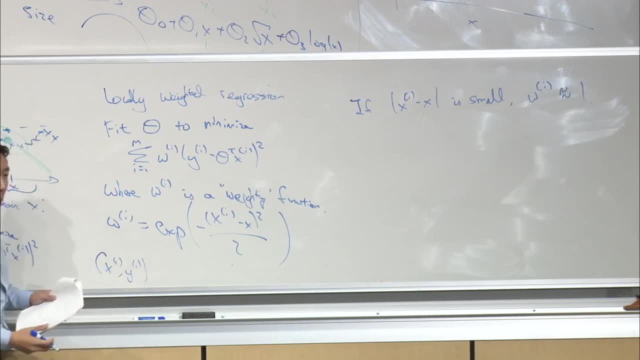 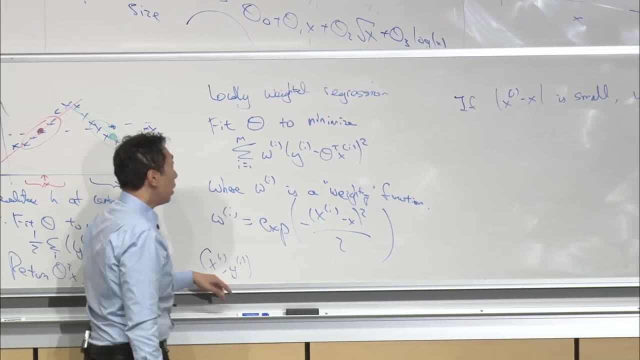 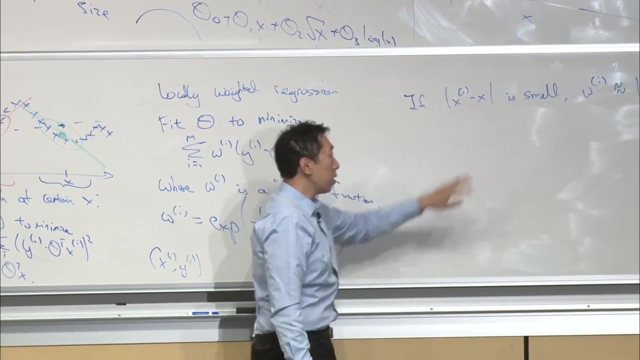 attention to the values of x, i comma, y, i when fitting, say, this green line or that red line. And so if x i minus x is small. so if that's your training example, that is close to where you want to make the prediction for x. 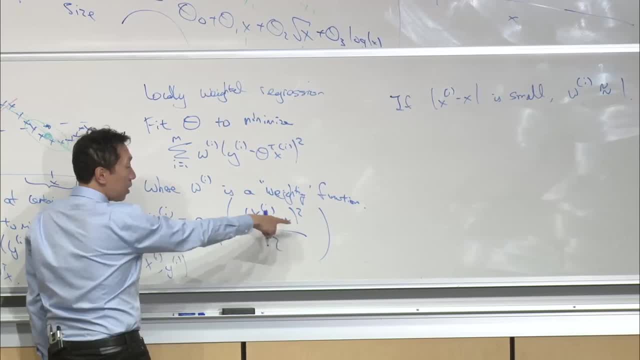 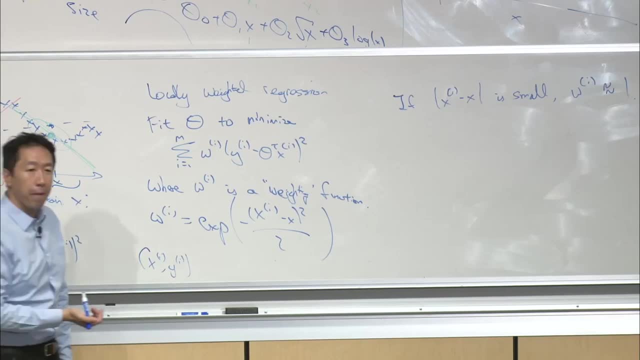 then this is about e to the 0, right, E to the negative 0, if the- if the numerator here is small and e to the 0 is close to 1, right Um. and conversely, if x, i minus x is large. 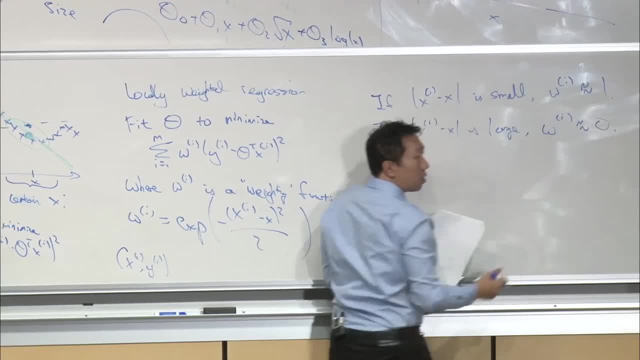 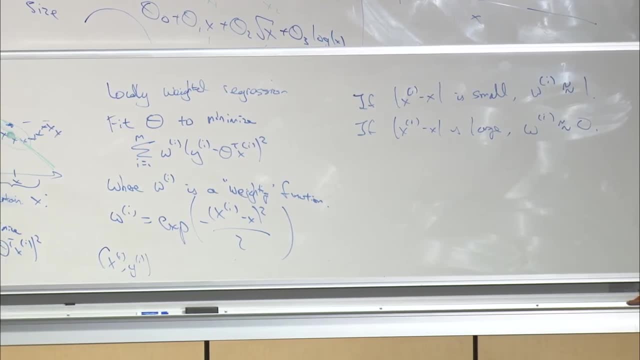 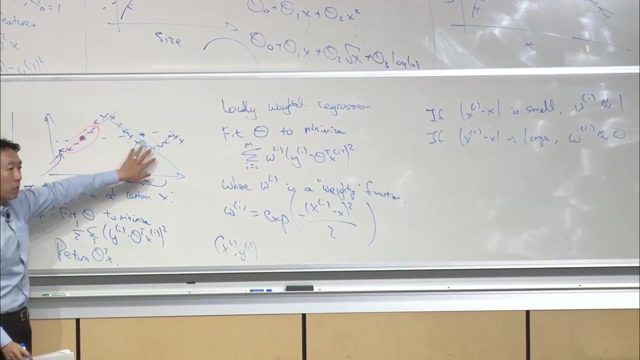 then w i is a weighting function. w i is close to 0. And so if x i is very far away, so let's say you're fitting this green line and this is your example x ording, then it's saying: give this example all the way out there. if you're fitting the green line, right. 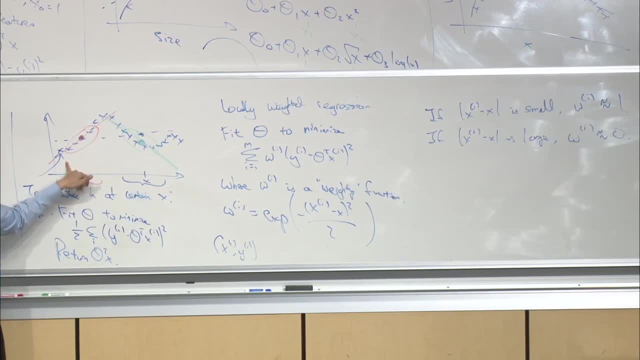 If you're looking at this first x saying that example should have a weight very close to 0, okay, Um. and so if you um, all you're doing is you are writing in that x, i swimming. you're writing in the y, i. 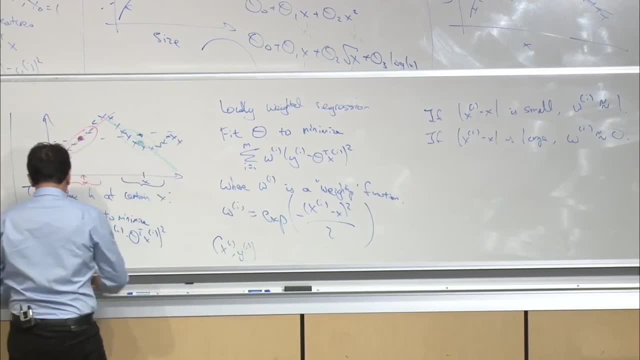 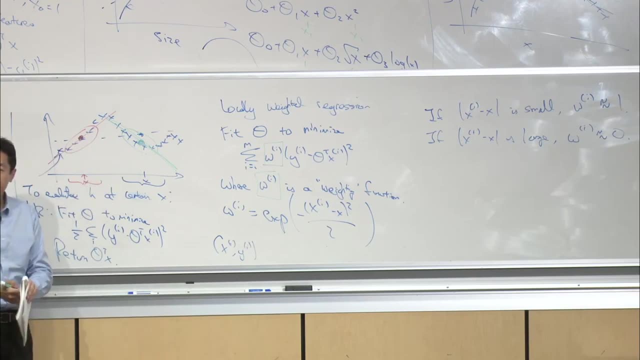 So when you're saying if the x i find close to 0,, Look at the cost function. The main modification to the cost function we've made is that we've added this weighting term right, And so what locally weighted regression does is the same. 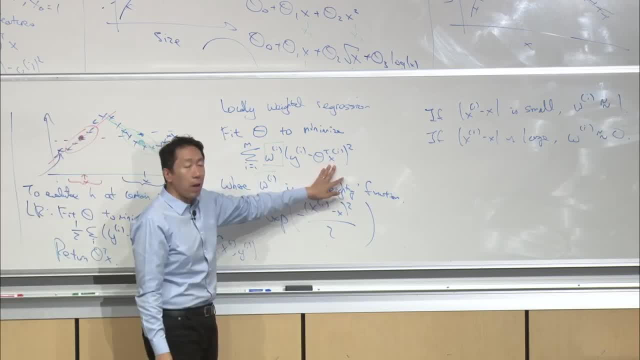 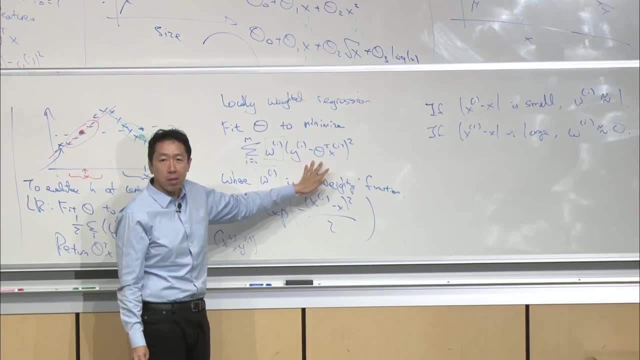 If an example x i is far from where you want to make a prediction, multiply that error term by 0 or by a constant very close to 0. Um, whereas if it's close to where you want to make a prediction, multiply that error term by 1.. 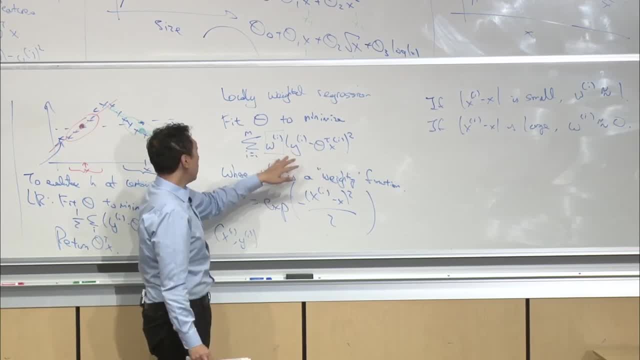 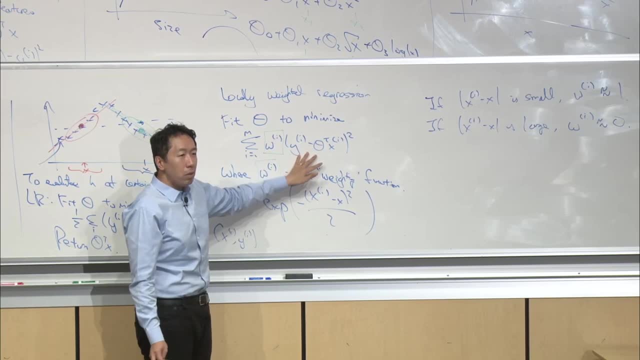 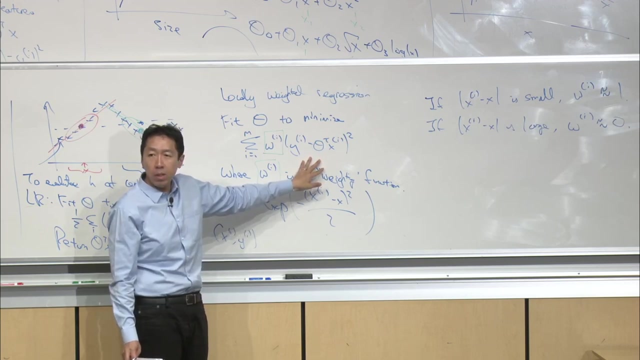 And so the net effect of this is that this is summing if, if you know, the terms multiplied by 0 disappear right. So the net effect of this is that this sums over essentially only the terms: uh, for the squared error, for the examples that are close to the value. 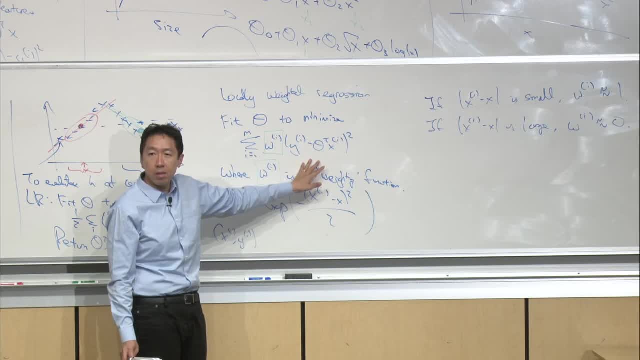 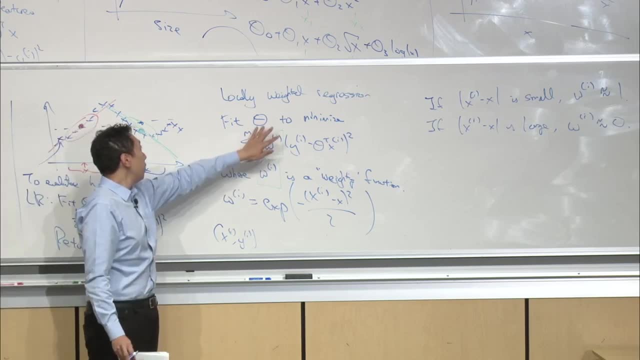 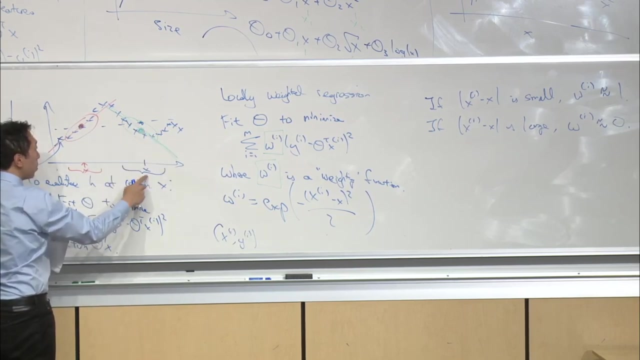 close to the value of x, where you want to make a prediction. okay, Um, and that's why, when you fit Theta to minimize this, you end up paying attention only to the points, only to the examples close to where you want to make a prediction and fitting a line. 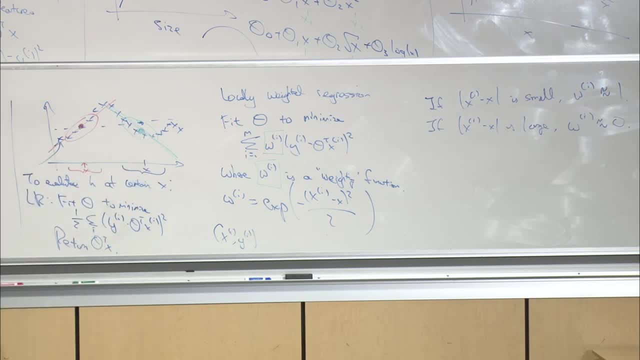 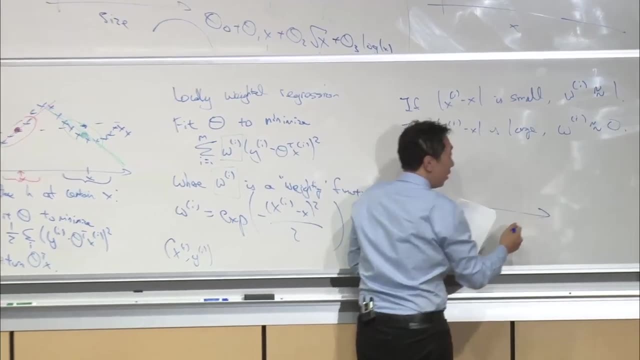 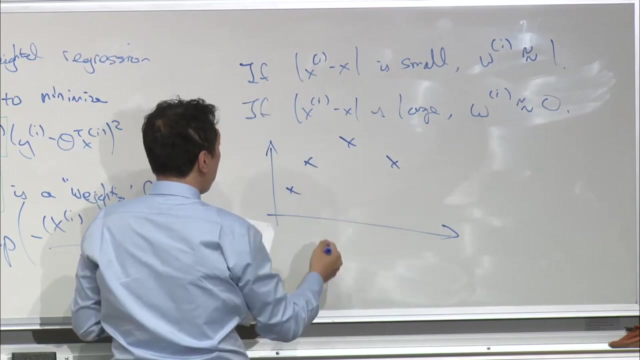 like a green line over there, okay, Um so let me draw a couple more pictures to to to illustrate this. Um so, if let me draw a slightly smaller dataset just to make this easier to illustrate. So that's your training set. 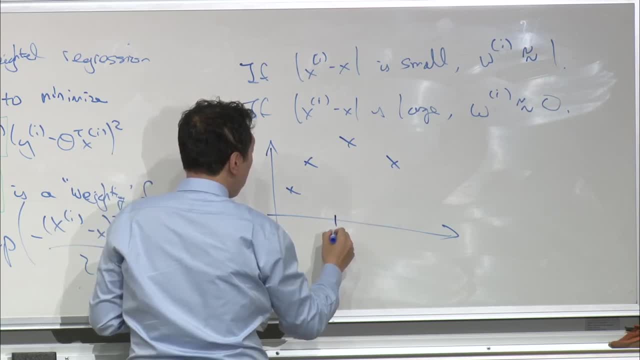 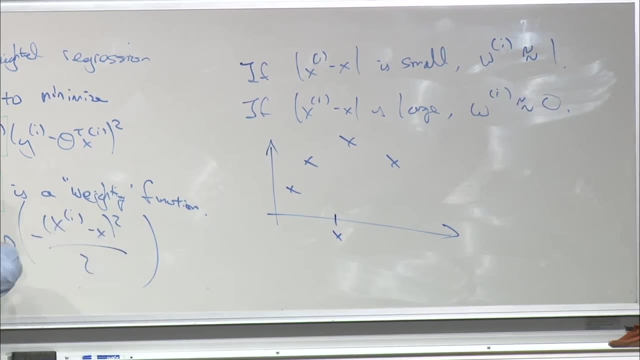 So that's, you know, examples x1, x2, x3, x4.. And if you want to make a prediction here, right at that point x, then, um, this curve here looks the the. the shape of this curve is actually like this right. 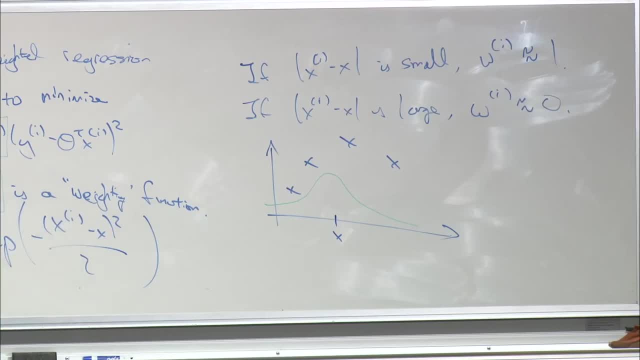 Um and it. this is the shape of a Gaussian bell curve, but this has nothing to do with a Gaussian density, right? So this thing does not integrate to 1.. So so this is just. sometimes you'll ask well, 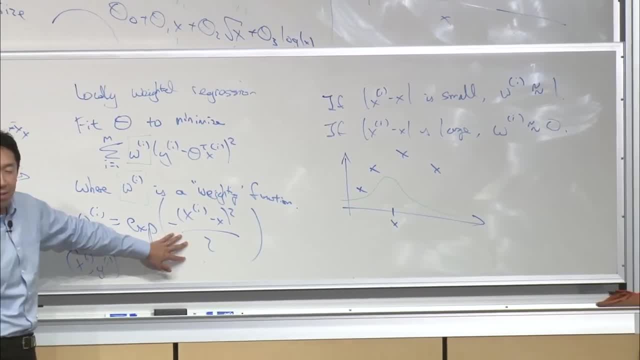 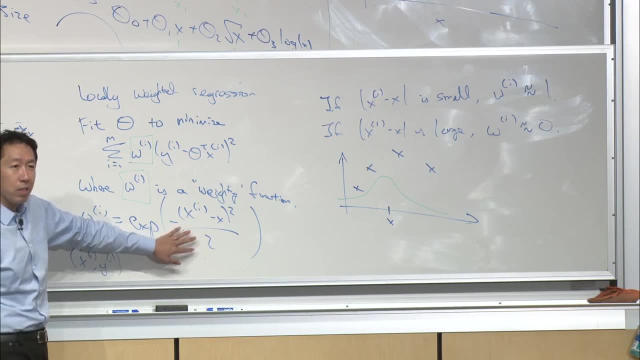 is this: is this using Gaussian density? The answer is no. Uh, this is just a function. This is just a function. that um is shaped a lot like a Gaussian, but you know, Gaussian density is probability density functions have to integrate to 1, and this is not. 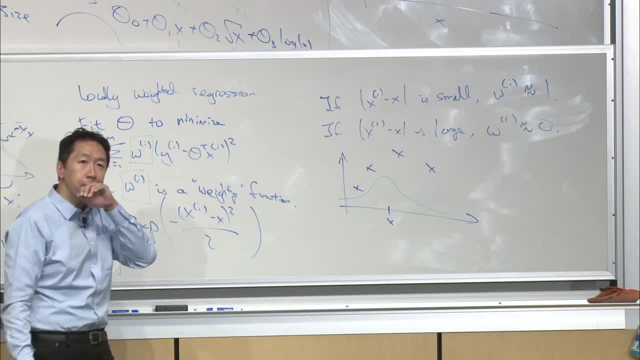 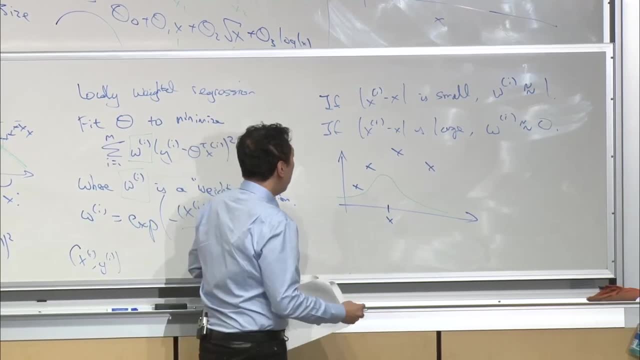 So there's nothing to do with a Gaussian probability density Question. Uh, how do you choose the weight of the- Oh, so how do you choose the weight? Let me get back to that. Yeah, Um, and so, for this example, 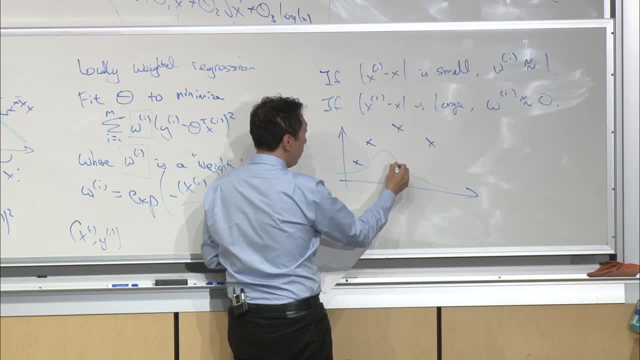 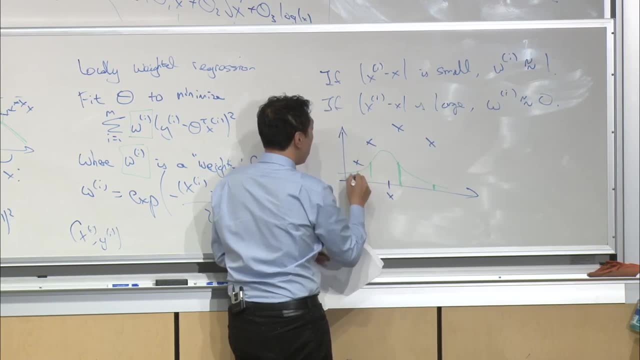 this height here says: give this example a weight equal to the height to that thing. Give this example a weight equal to that thing, Weight equal to the height of this height, of this height of that right. Which is why, if you actually 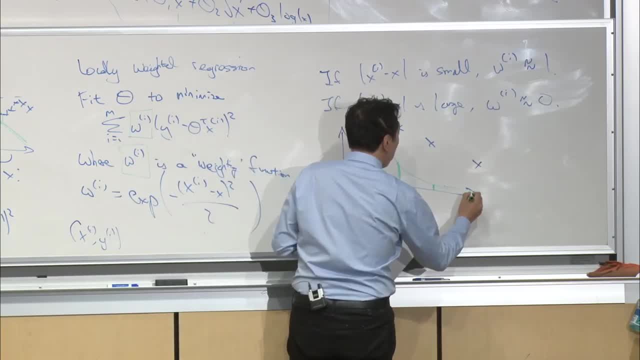 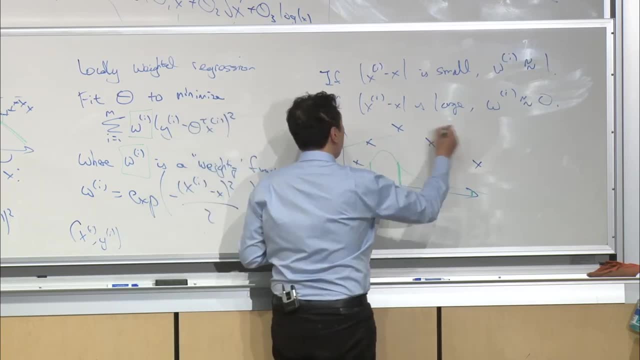 if you have an example that's way out there, you know it's given a weight that's essentially 0, which is why it's weighting only the nearby examples when trying to fit a straight line right. uh for the for making predictions close to this. 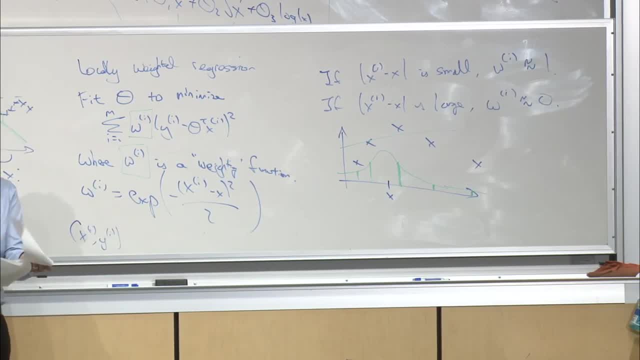 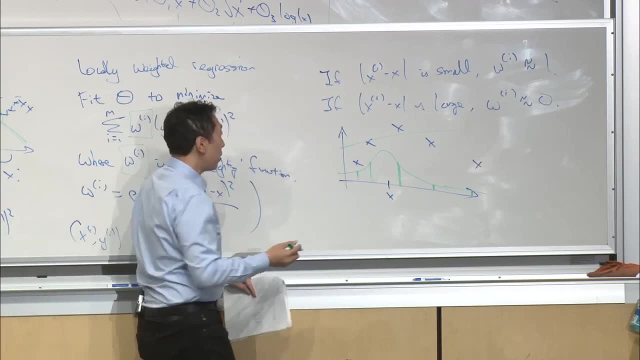 Okay, Um now. so one last thing that I want to mention, which is um the the the question just now, which is: how do you choose the width of this Gaussian density, right? How fast is it? How thin should it be? 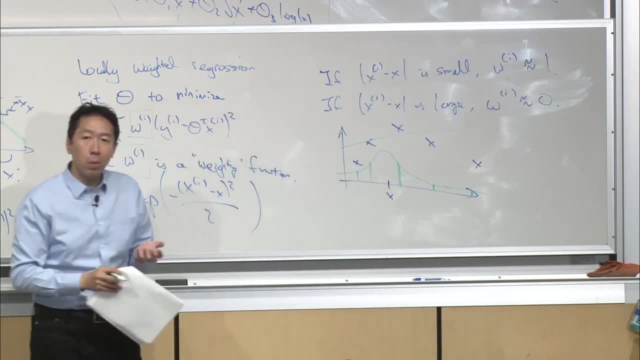 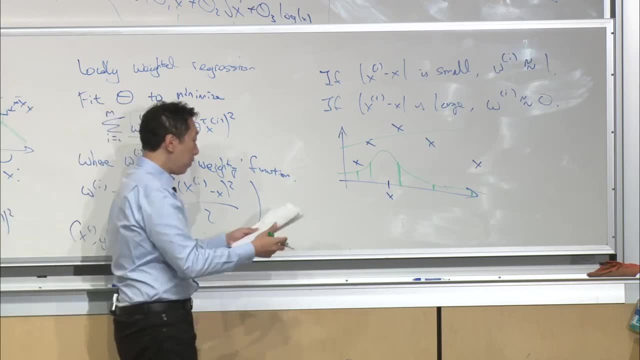 Um, and this decides how big a neighborhood- should you look in order to decide what's the neighborhood of points you should use to fit this? you know, local straight line, And so, um, for a Gaussian function like this, uh, this, I'm gonna call this the. 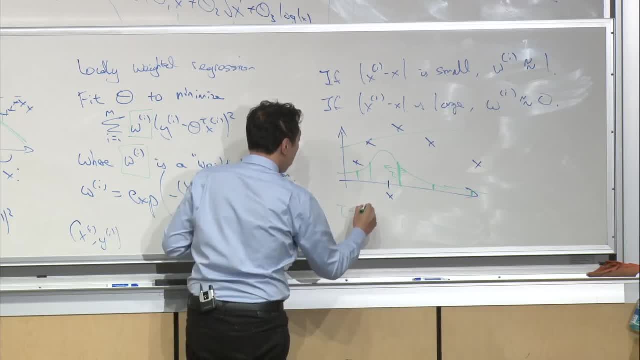 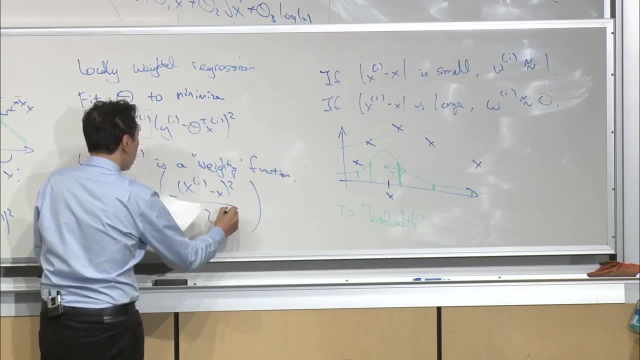 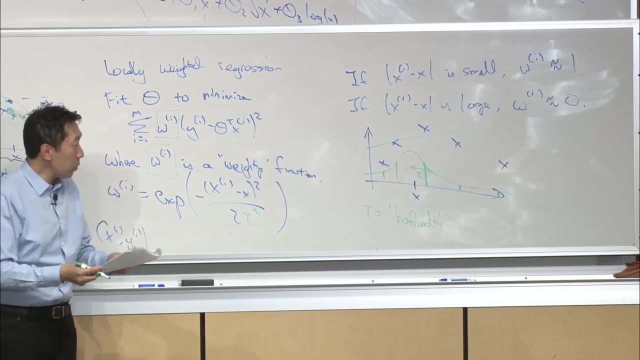 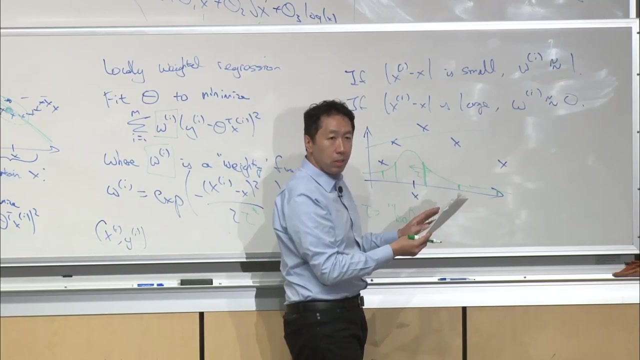 um bandwidth parameter, tau Right- And this is a parameter or hyperparameter of the algorithm- And uh, depending on the choice of tau um uh, you can choose a fatter or thinner bell-shaped curve, which causes you to look in a bigger or a narrower window. in order to decide. 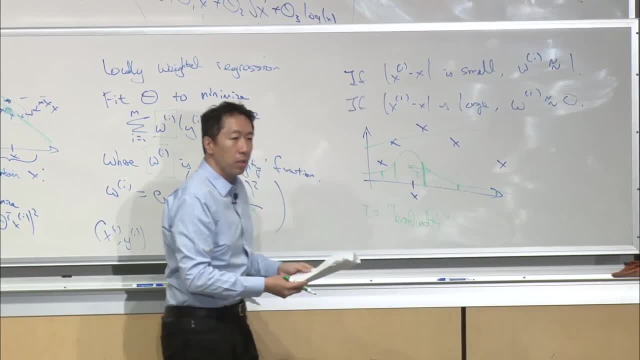 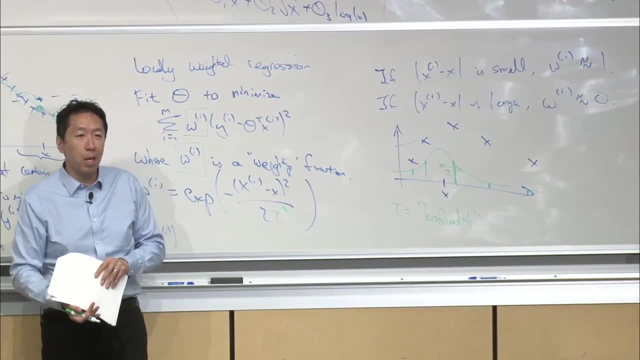 um, you know how many nearby examples you use in order to fit the straight line. Okay, And it turns out that um, and I wanna leave, I wanna leave you to discover this yourself in the problem um set, Um, if. 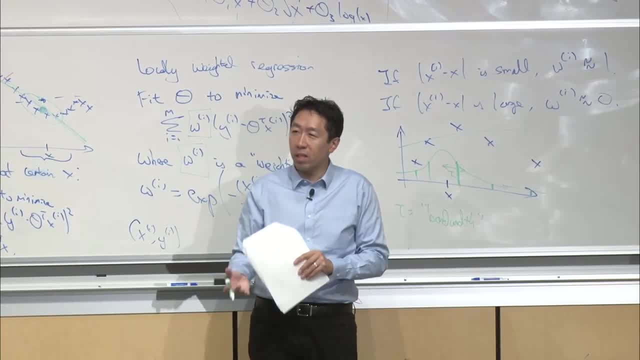 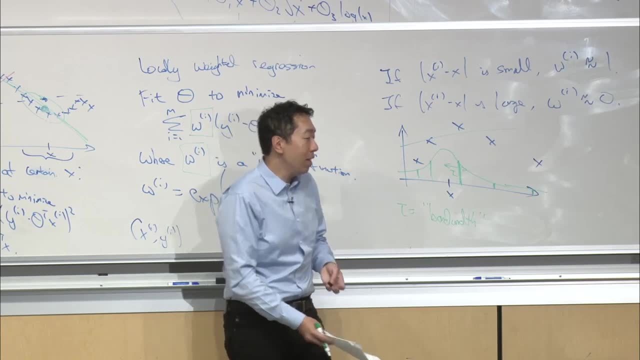 if you've taken a little bit of machine learning elsewhere and heard of the terms: oh, test is on, Okay, good, We're still on. Good, It turns out that, um, the choice of the bandwidth tau has an effect on. 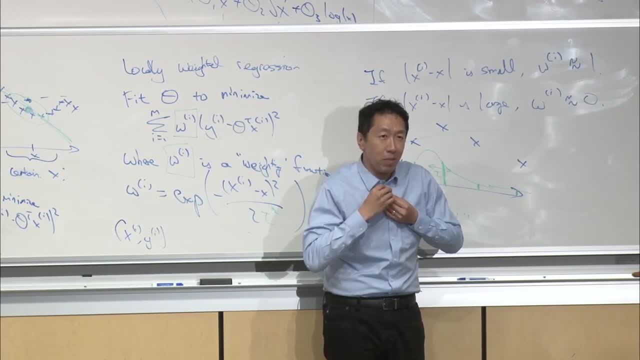 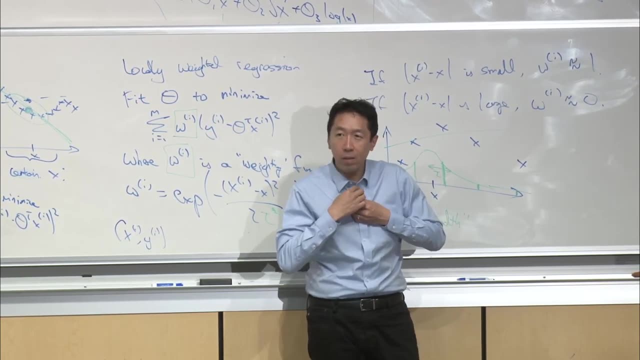 uh, overfitting and underfitting. If you don't know what those terms mean, don't worry about it. We'll define them later this quarter. But uh, what you get to do in the problem set is, uh, play with tau yourself and see why. 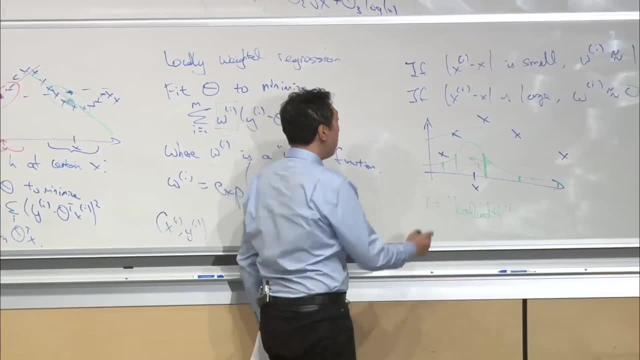 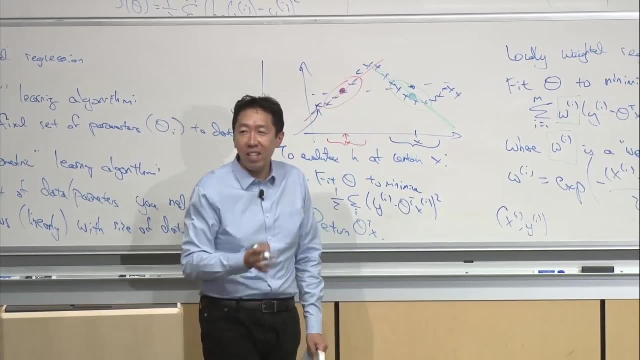 um, uh. if tau is too broad, you end up fitting- um, you end up over-smoothing the data. and if tau is too thin, you end up fitting a very jagged fit to the data. And if any of these things don't make sense yet, 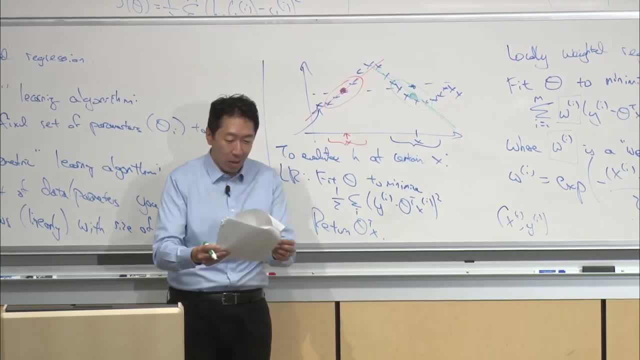 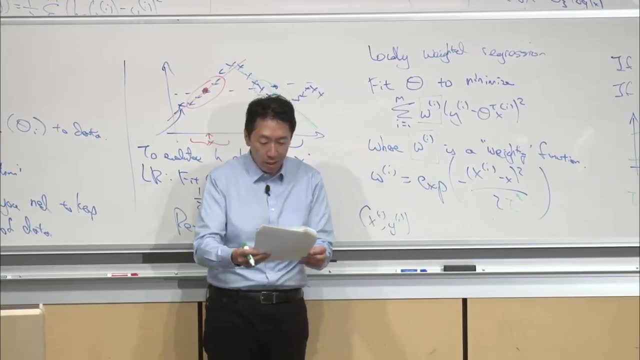 don't worry about it, they'll make sense after you play with it in the in the problem set. Okay, Um so yeah, since since you, you play with the varying tau in the problem set and see for yourself the net impact of that. 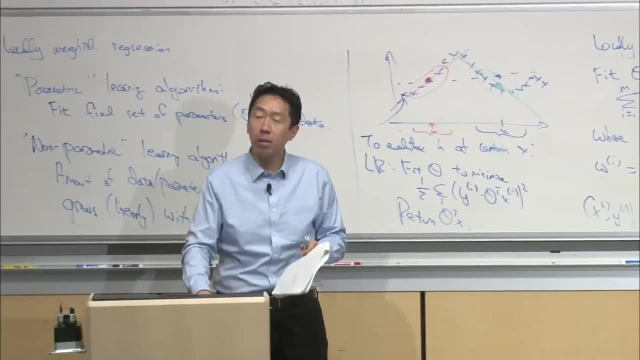 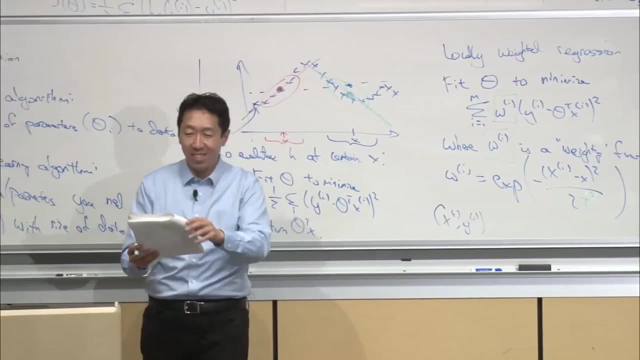 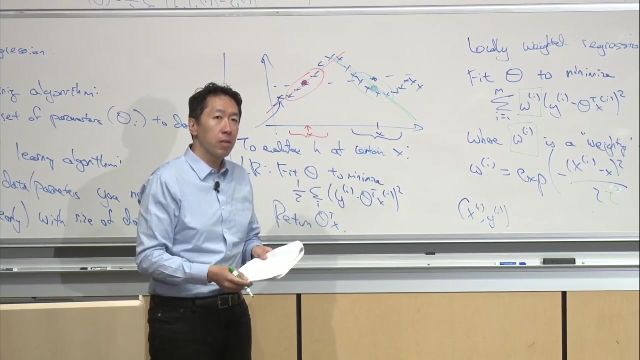 Okay. Question: Is tau equal to power error or is that just uh the one? Thank you, Uh, this is tau squared, Yeah, Yeah, Um. so what happens if you need to infer um the value of H at a point outside the scope of the data set? 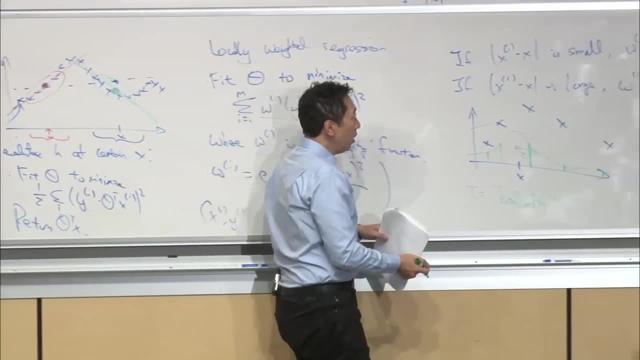 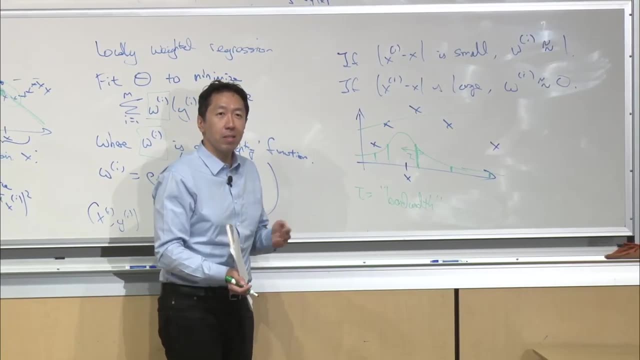 Uh, what happens if you need to infer the value of uh H outside the scope of the data set? It turns out that you could still use this algorithm. It's just that, uh um, it's results may not be very good. 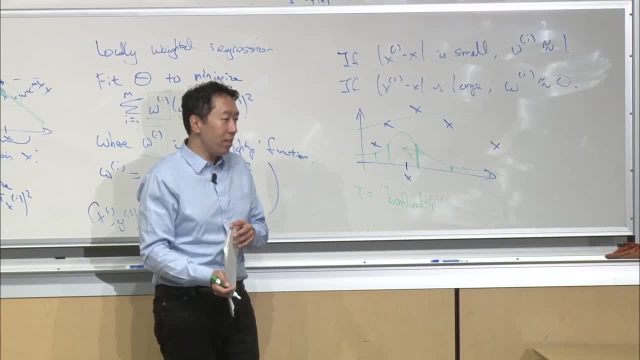 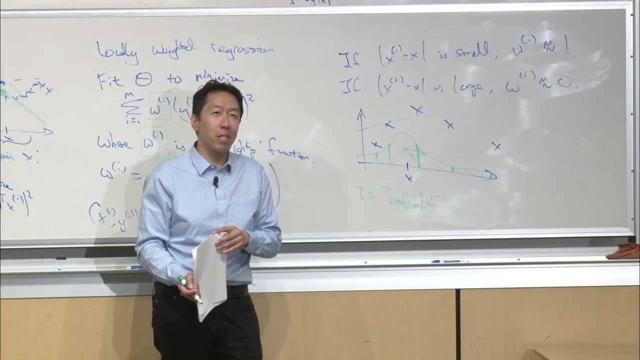 Yeah, It, it, it, it depends, I guess It um. locally weighted linear regression is usually not great at extrapolation, but then most- many learning algorithms are not great at extrapolation, So all- all the formulas still work. 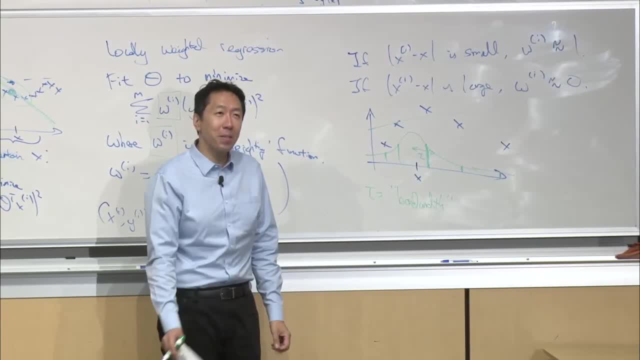 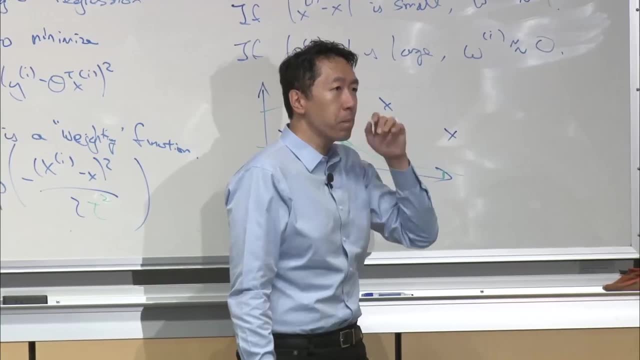 they still implement this. But, um, yeah, you can also try- you can also try it in your problem set and see what happens. All right, one last question: Is it possible to have like a variable tau and they monitor some parts of your data and have lots of uh-? 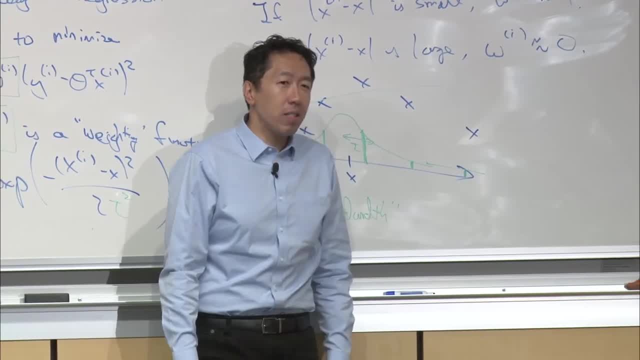 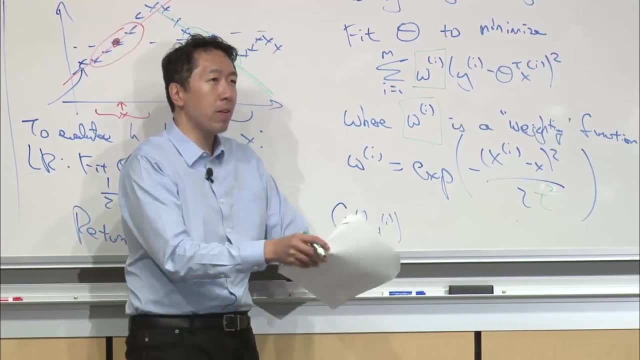 Oh yeah, Yes, Is it possible that a variable tau uh uh? yes, it is uh, and there are quite complicated ways to choose tau, based on how many points there are in the local region and so on. Yes, There's a huge literature on different formulas. 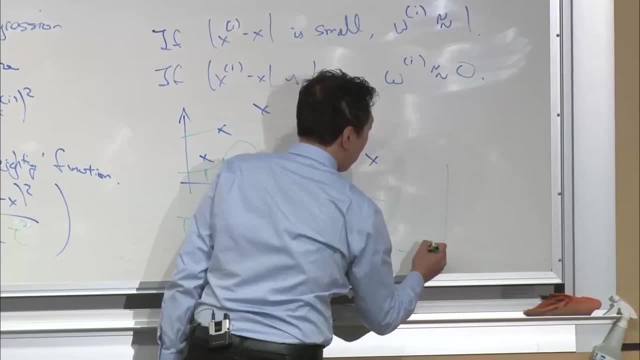 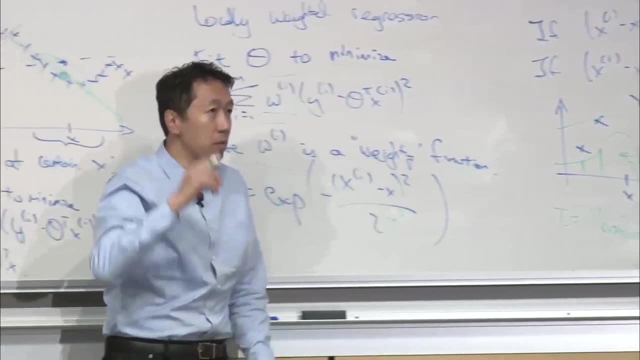 Actually, for example, instead of this Gaussian bump thing, uh, there's. uh, sometimes people use that triangle shape function, So it actually goes to 0, upsides and small a. So there are- there are- many versions of this algorithm. 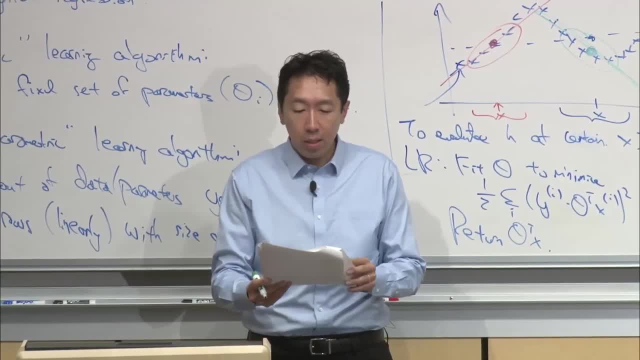 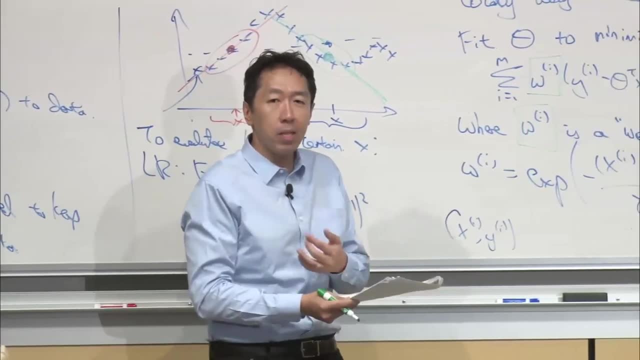 Um, so I tend to use, uh uh, locally weighted linear regression when, uh, you have a relatively low-dimensional dataset, So when the number of features is not too big, right? So when n is quite small, like 2 or 3 or something. 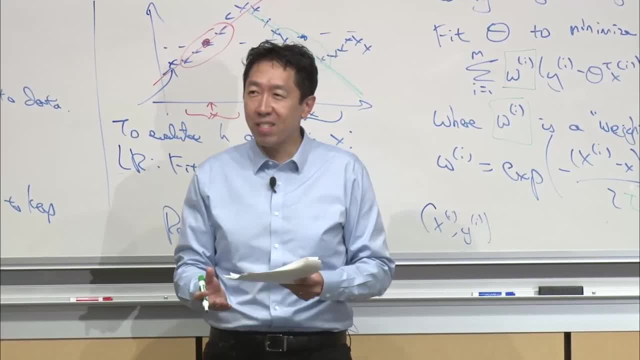 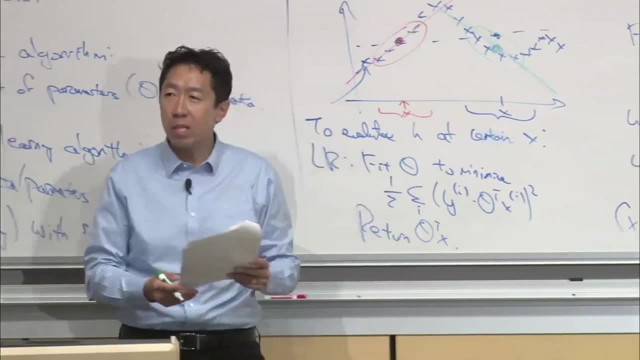 and we have a lot of data and you don't wanna think about what features to use, right, So- so that's the scenario. So if- if you actually have a dataset that looks like these up in drawing, you know, locally weighted linear regression, is- is, a- is a pretty good algorithm. 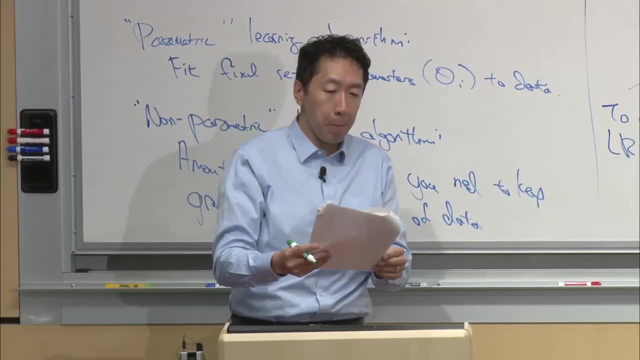 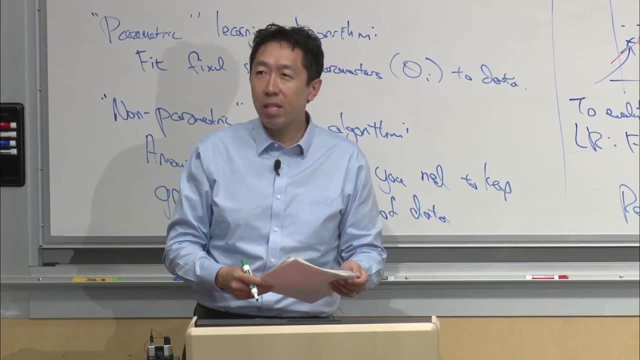 All right, just one last question, then we'll move on. Oh sure, Yes, If you have a lot of data, won't this be computationally expensive? Yes, it would be. Uh, I guess a lot of data is relative. 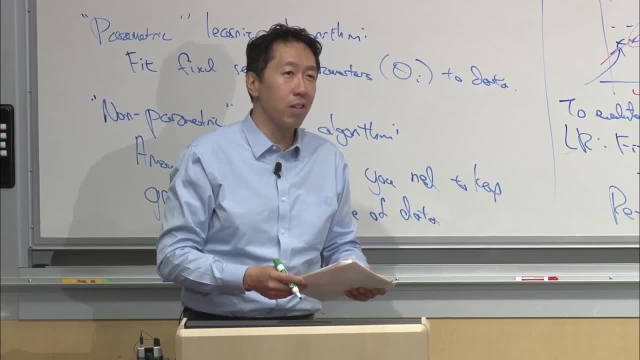 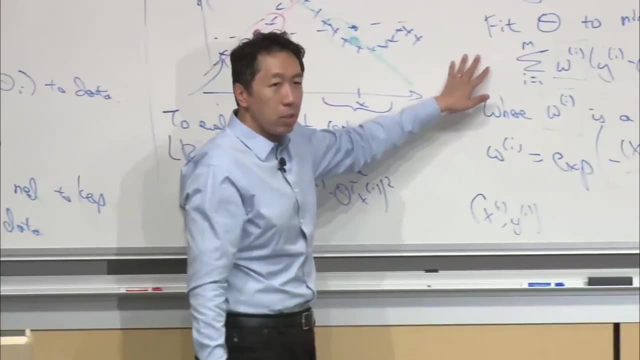 Uh, yes, We have, you know, two, three four-dimensional data and hundreds of examples. I mean thousands of examples. Uh, it turns out the computation needed to fit the minimization is, uh, similar to the normal equations. 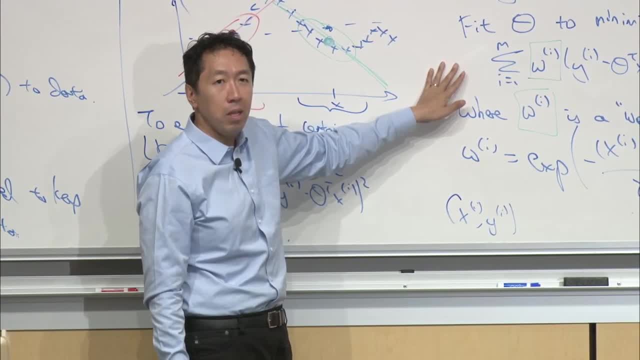 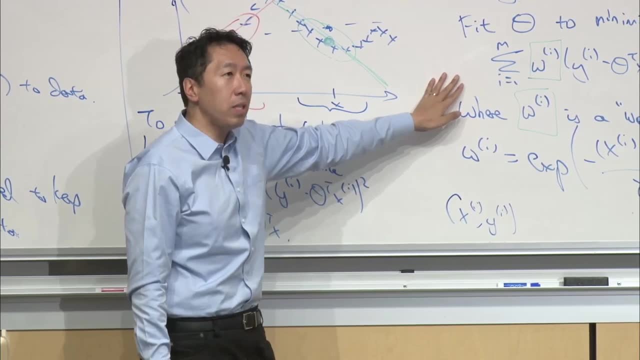 Um, and so you-. it involves solving a linear system of equations of dimension equal to the number of training examples you have. So if that's, you know, like a thousand or a few thousand, that's not too bad. Uh, if you have millions of examples, then- then, 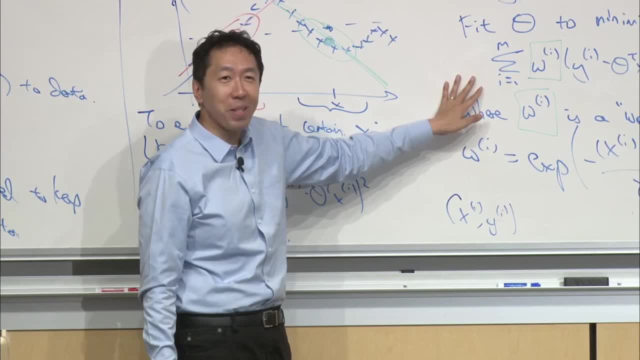 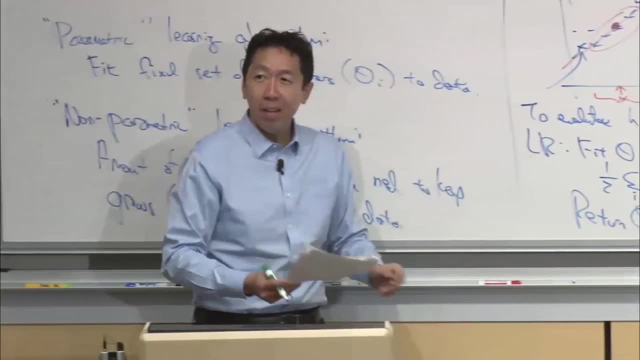 there are also more sophisticated algorithms like KD trees and much more complicated algorithms to do this when you have millions or tens of millions of examples. Yeah, Um, okay. So really you get a better sense of this algorithm when you play with it. 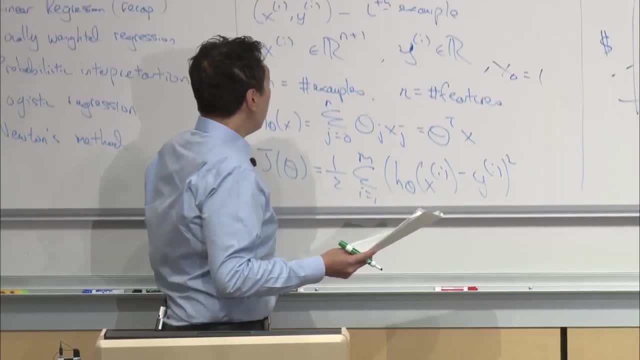 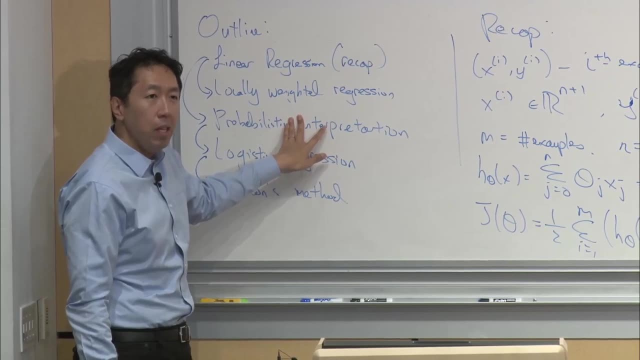 um in the problem set. Now the second topic when the- so- so I'm gonna put aside locally weighted regression. Uh, we won't talk about that set of ideas anymore. uh, today, But- but what I want to do today is um, uh, on last one. 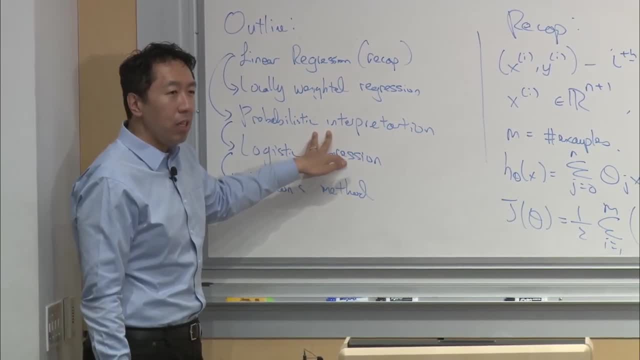 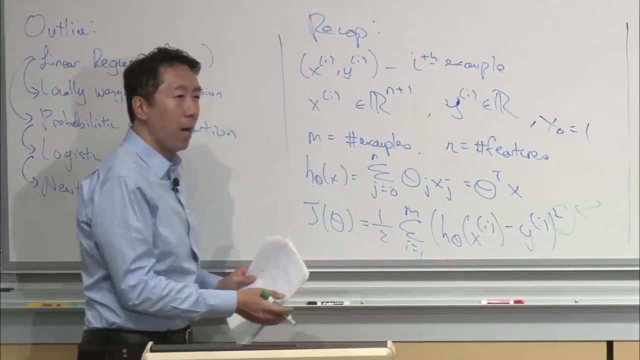 say, I had said that I had promised last Wednesday that today I'll give a justification for why we use the squared error right. Why the squared error? Why not, you know, to the full power or absolute value? um And so um. what I want to show you today, now, is: 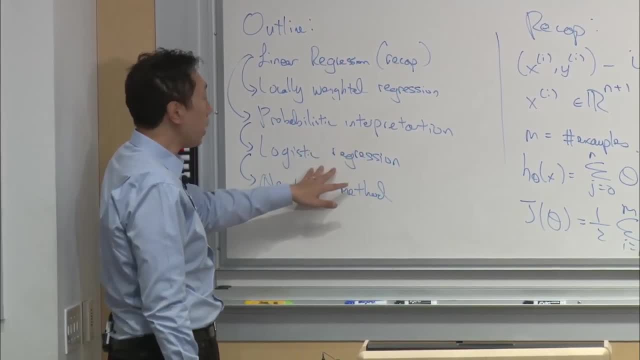 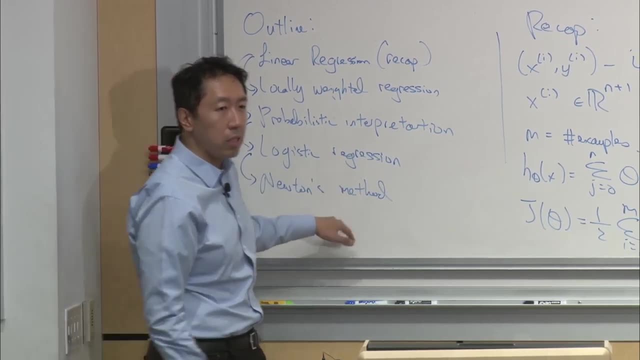 the probabilistic interpretation of linear regression. And this probabilistic interpretation will put us into good standing as we go on to logistic regression today, uh, and then generalize linear models, uh, later this week. Okay, Maybe I'll keep up the-. 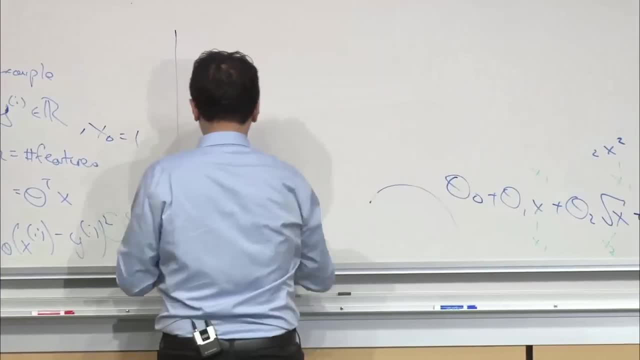 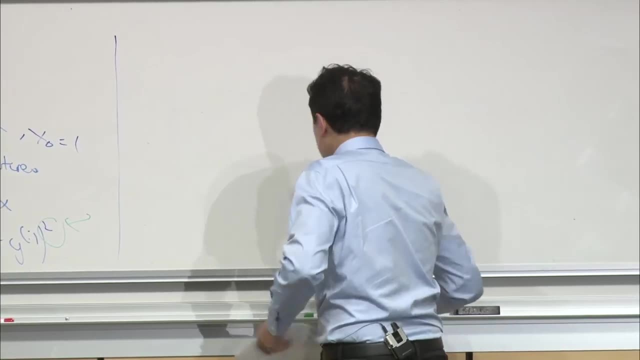 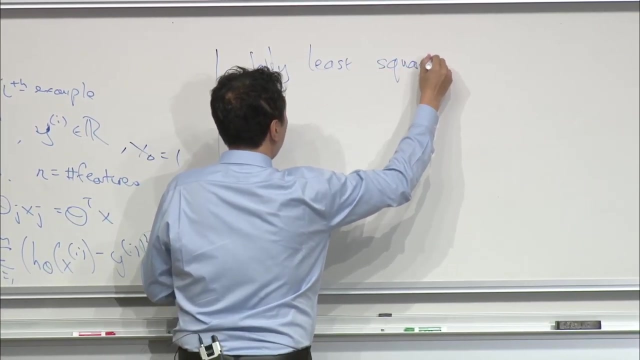 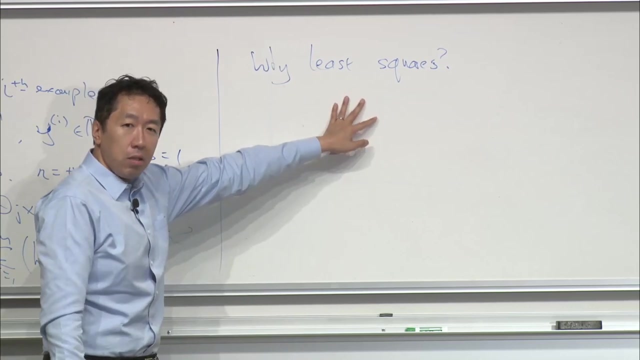 keep the notation there so you can continue to refer to it, So right. So why these squares? Why squared error? Um, I'm gonna present a set of assumptions under which these squares using squared error falls out very naturally, right, Which is? 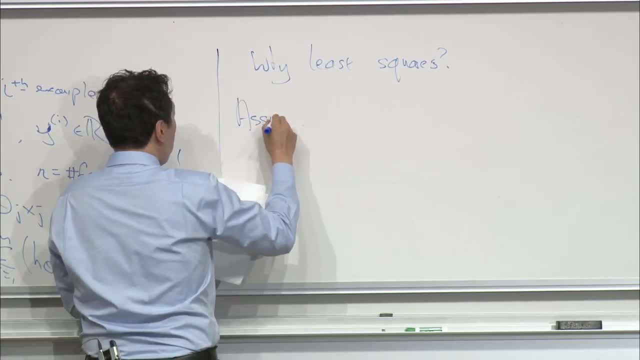 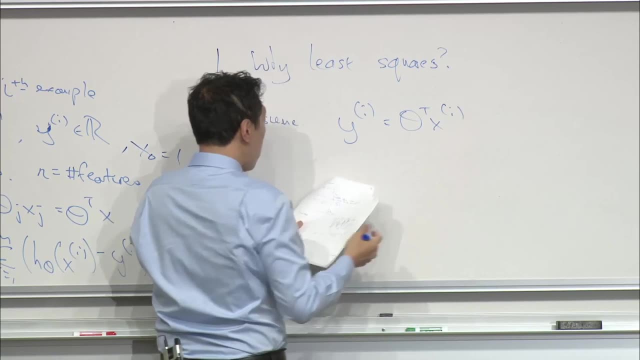 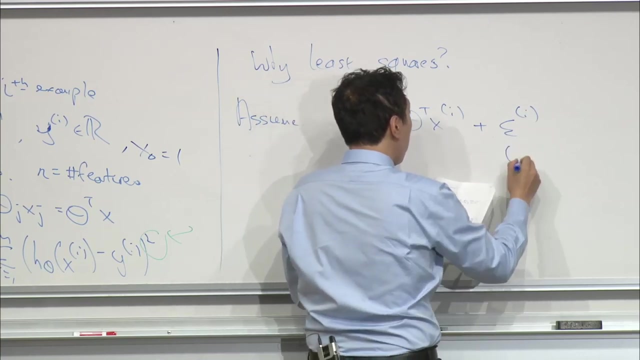 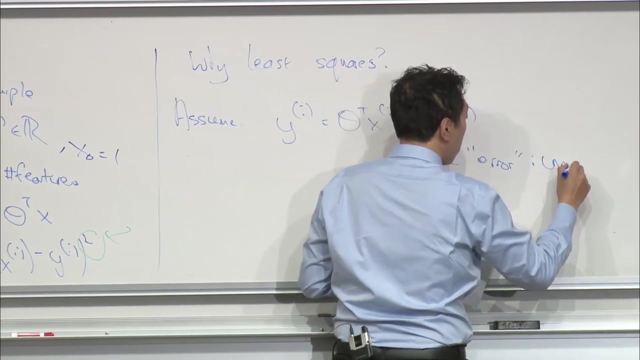 Let's say, for housing price prediction, let's assume that there's a true price of every house: y, i, which is x. transpose um theta i plus epsilon i, where epsilon i is an error term. that includes um unmodeled effects. you know. 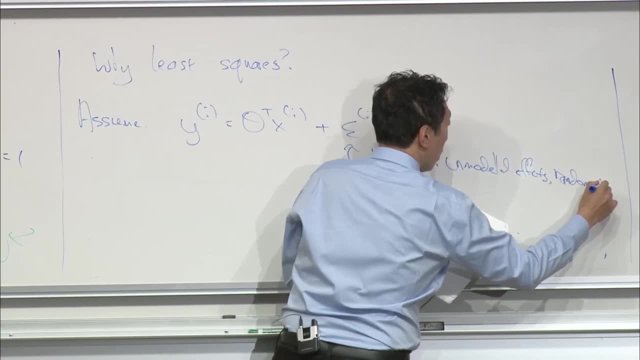 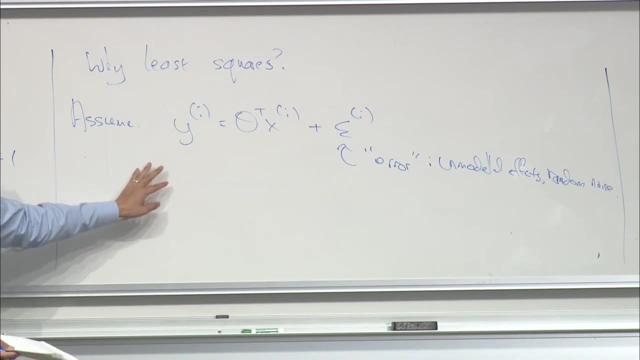 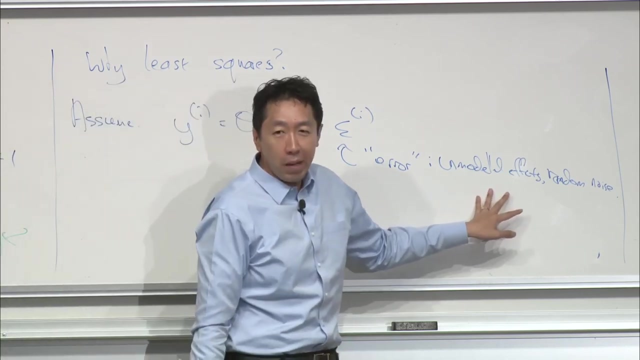 and just random noise. okay, So let's assume that the way you know housing prices truly work is that every house's price is a linear function of the size of the house and number of bedrooms, plus an error term that captures unmodeled effects. 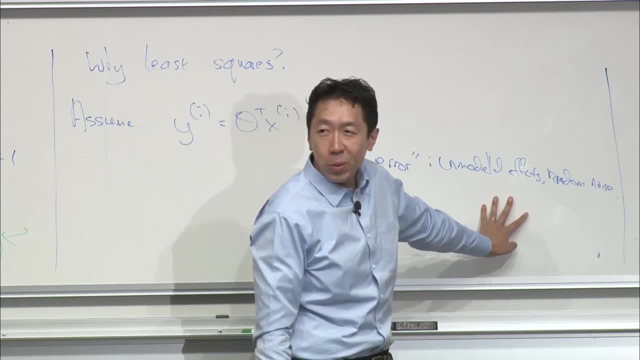 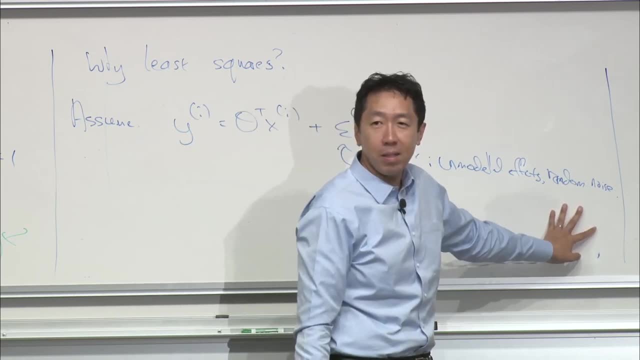 such as: maybe one day that cell is in an unusually good mood or an unusually bad mood, and so that makes the price go higher or lower, and we just don't model that um as well as random noise, right, Uh, or maybe I'm- maybe don't want to screw this straight. 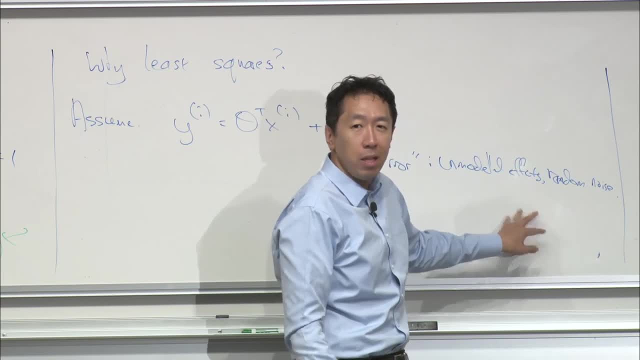 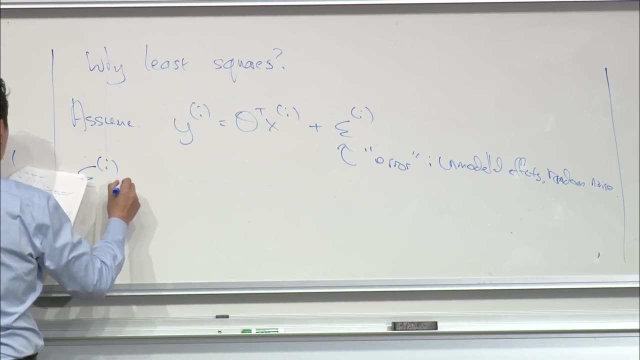 you know, just to capture that as one of the features, but other things that have an impact on housing prices, Um, and we're going to assume that, uh, epsilon i is distributed, Gaussian would mean zero and covariance sigma squared, So I'm gonna use this notation to mean 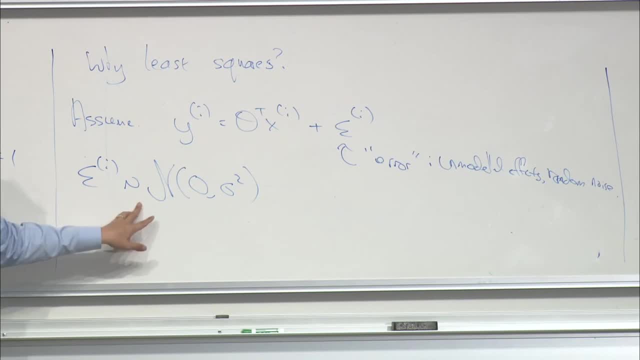 uh, so the way you read this notation is: epsilon i, this twiddle you pronounce as is distributed, and then script n, parenthesis, zero, comma, sigma squared. This is a normal distribution, also called the Gaussian distribution. same thing: Normal distribution and Gaussian distribution mean the same thing. 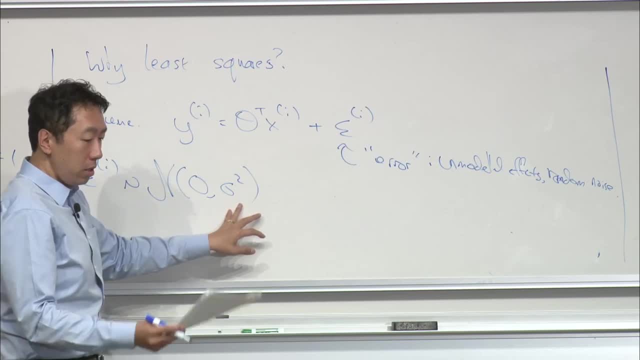 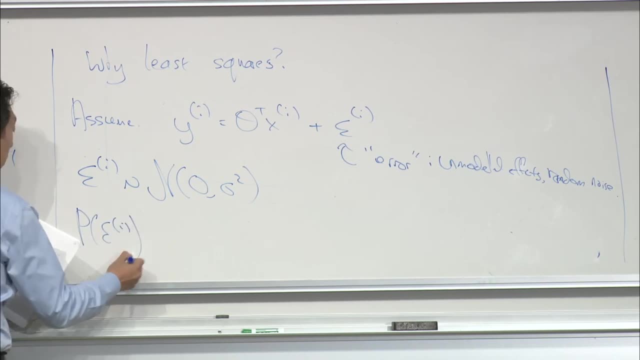 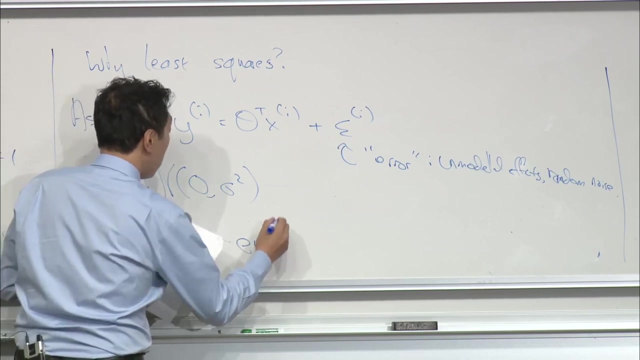 The normal distribution uh would mean zero and um variance sigma squared okay, Um, and what this means is that the probability density of epsilon i is: this is the Gaussian density, one of the root 2 pi sigma e to the negative epsilon i. 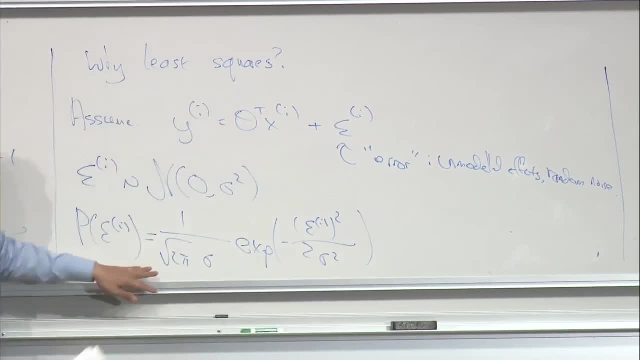 squared over 2 sigma squared, okay. Oh, and unlike the bell shape, the bell-shaped curve I used earlier for uh locally weighted linear regression, this thing does integrate to 1, right, This? this function integrates to 1, uh. 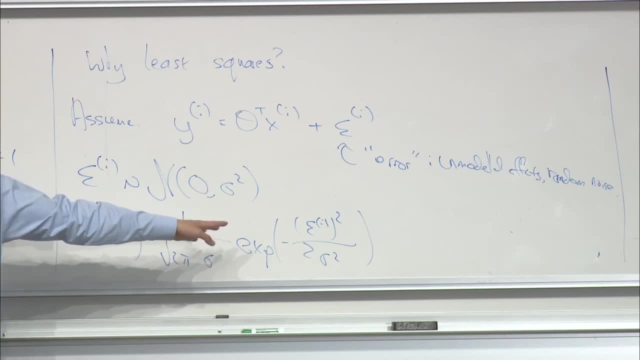 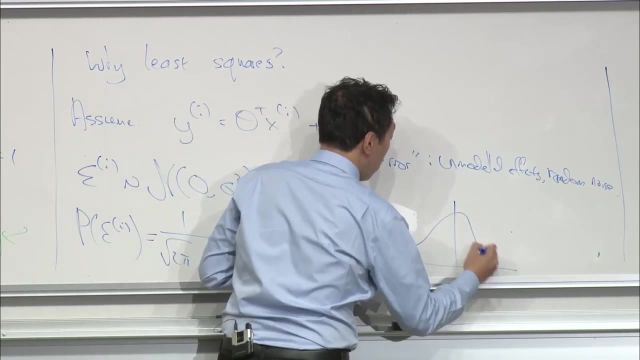 and so this is a Gaussian density, This is a prob-, prob- probability density function. okay, Um, and this is the familiar, you know, Gaussian bell-shaped curve with mean zero and uh covari- and uh variance um. 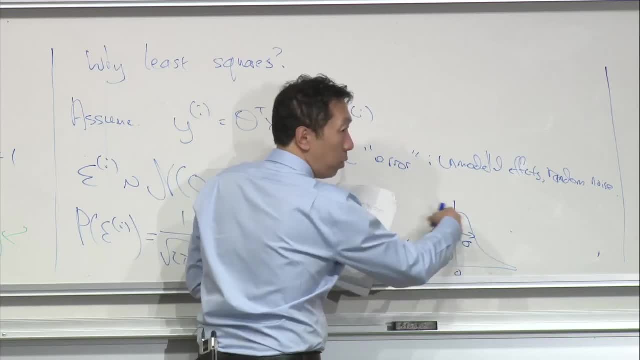 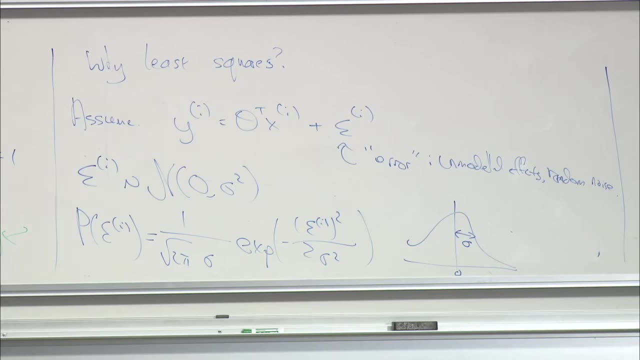 uh, sigma squared right Where sigma kind of controls the width of this Gaussian. okay, Uh, and if you haven't seen Gaussians for a while, we'll go over some of the uh probability- probability prereqs as well in the 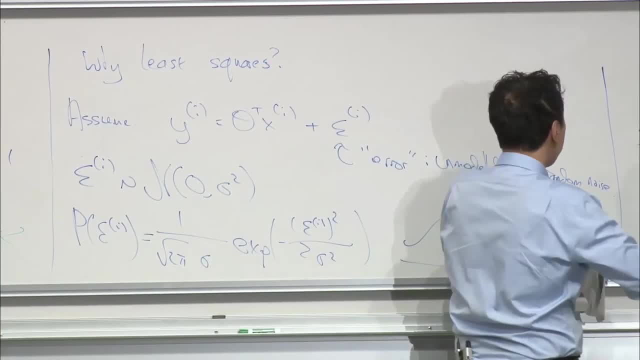 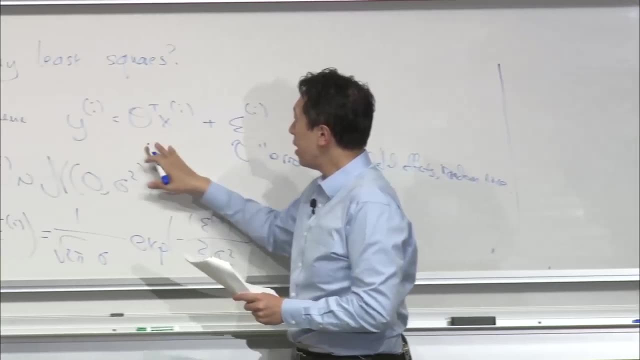 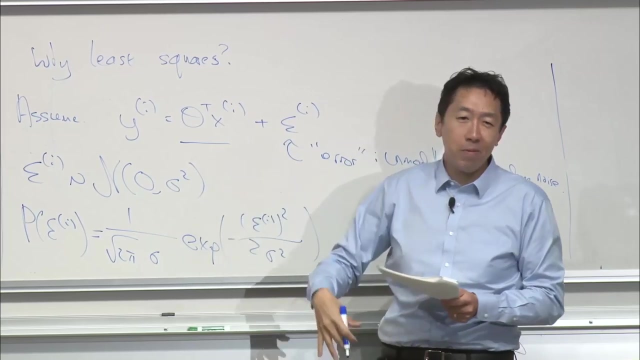 uh classes, Friday discussion sections. So, in other words, um, we assume that the way housing prices are determined is that first is a true price, theta transpose x, and then, you know some random force of nature, right the mood of the seller. 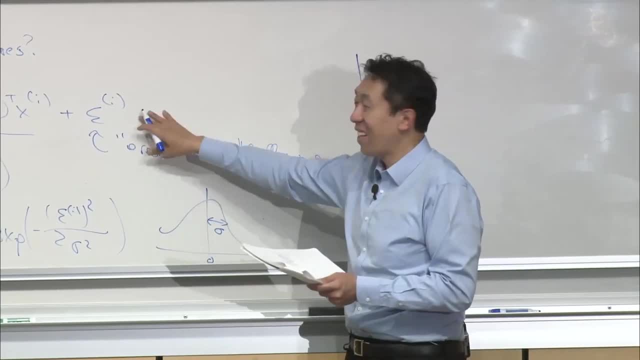 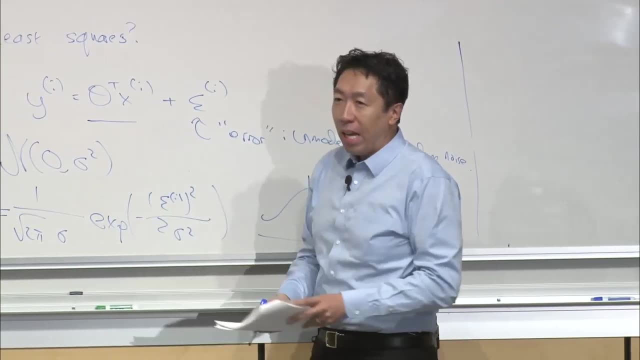 or uh, uh, uh, I don't know, I- I- I don't know other factors right, Perturbs it from this true value. theta transpose x, i, Um, and the huge assumption we're gonna make is that the epsilon i's. 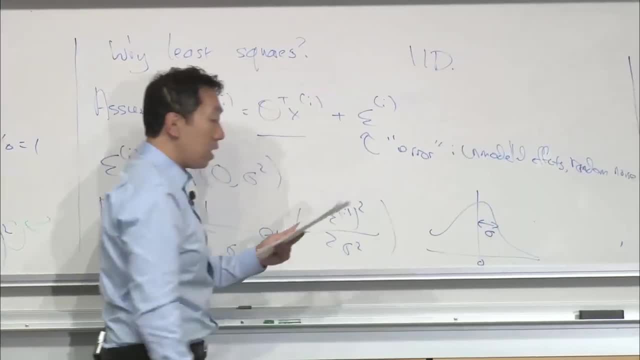 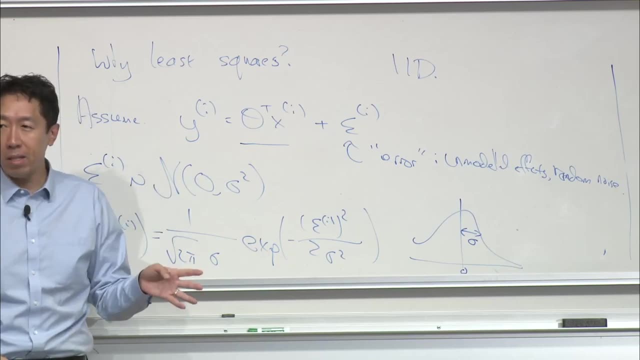 these error terms are iid, And iid from statistics stands for independently and identically distributed, And what that means is that the error term for one house is independent, uh, as the error term for a different house, which is actually not a true assumption, right. 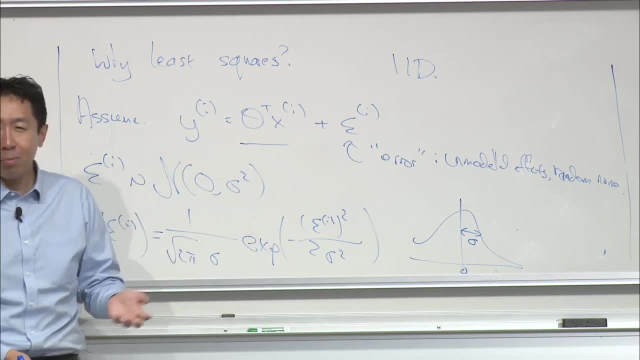 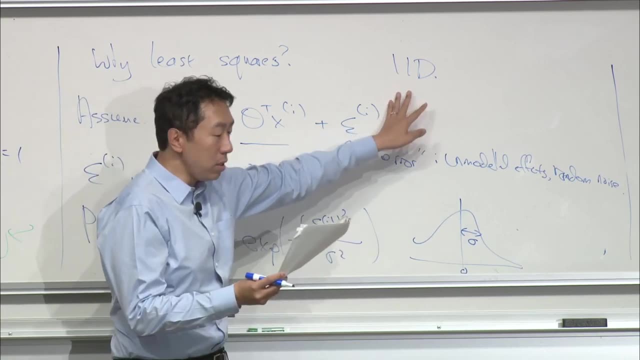 Because you know if- if one house's price on one street is unusually high, probably a price on a different house on the same street will also be unusually high, And so- but uh, this assumption that these epsilon i's are iid stands for. 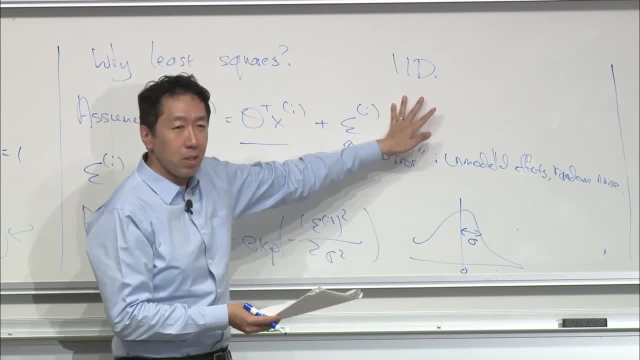 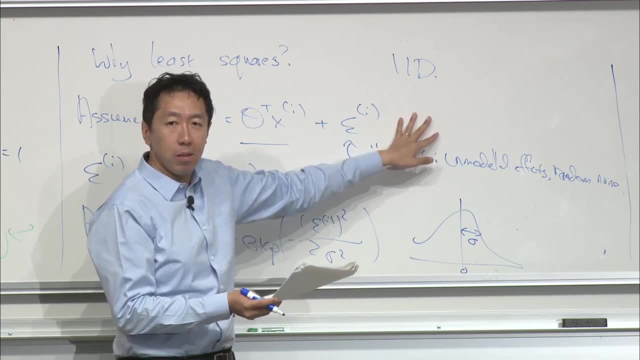 independently and identically distributed um is one of those assumptions that- that, you know, is probably not absolutely true, but may be good enough that if you make this assumption, you get a pretty good model. okay, Um, and so let's see. 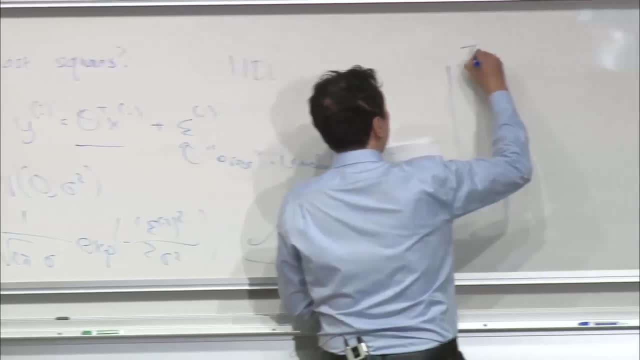 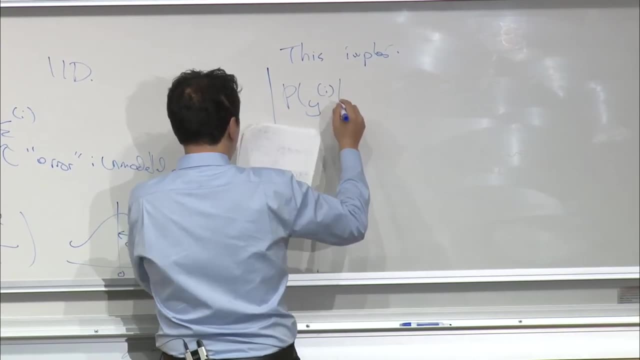 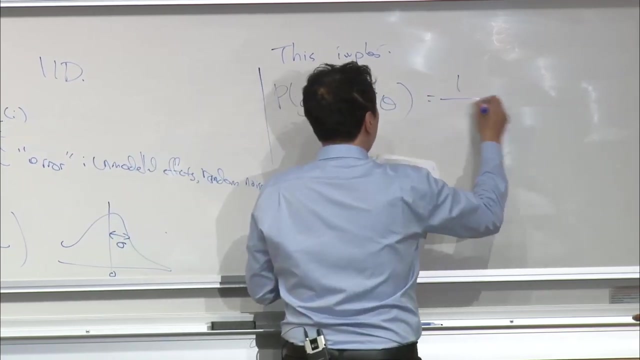 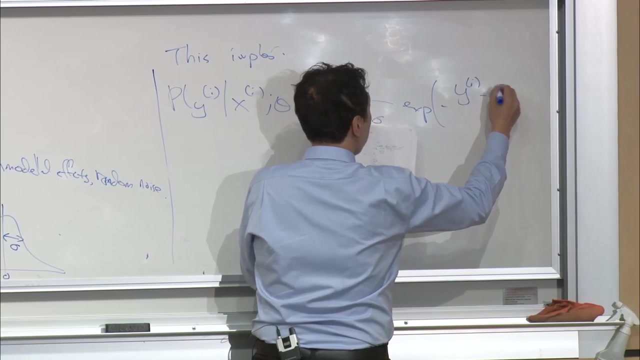 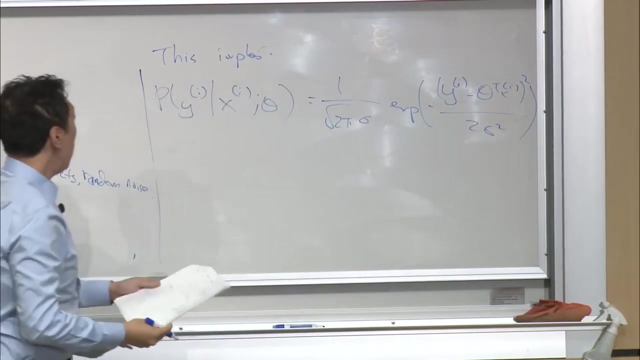 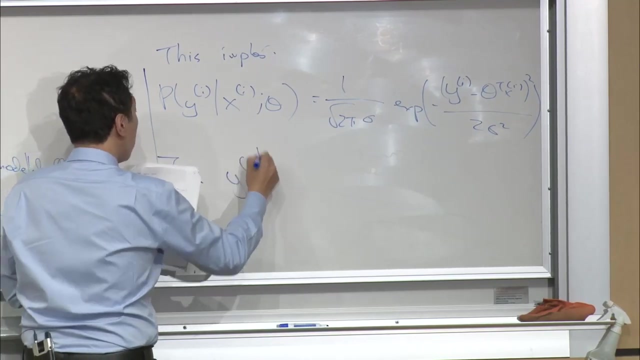 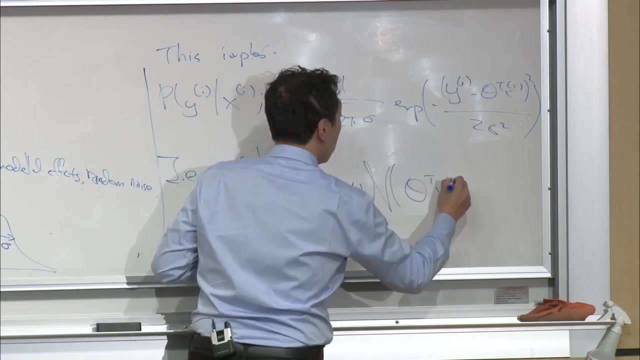 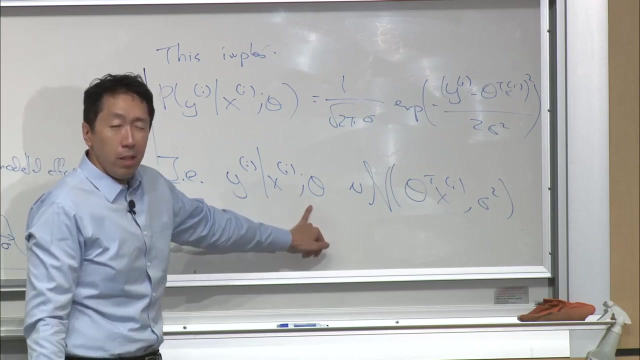 Under this set of assumptions. this implies that the density or the probability of y, i given x, i and Theta, this is going to be this: Okay, Um and I'll- I'll take this and write it in another way. In other words, um given x and Theta. 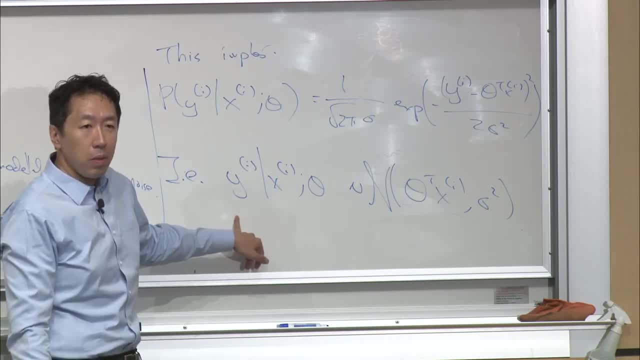 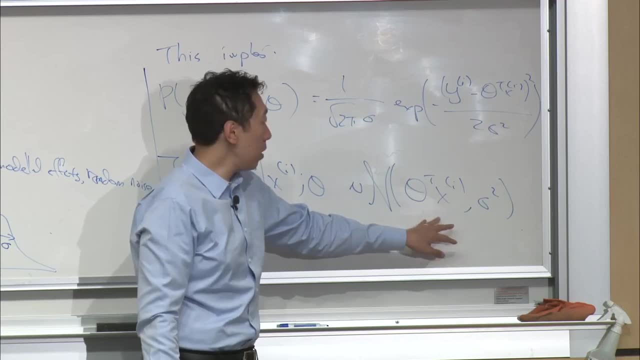 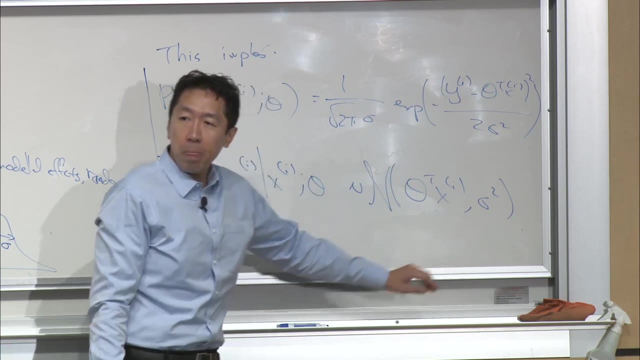 what's the density- what's the probability of a particular house's price? Well, it's going to be Gaussian, with mean given by Theta transpose x, i, or Theta transpose x, and variance um given by Sigma. squared, Okay, Um and so uh. 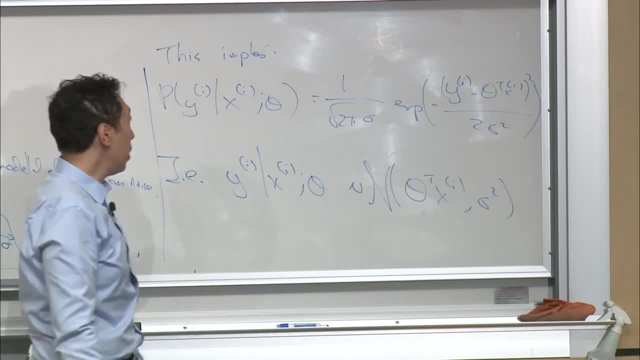 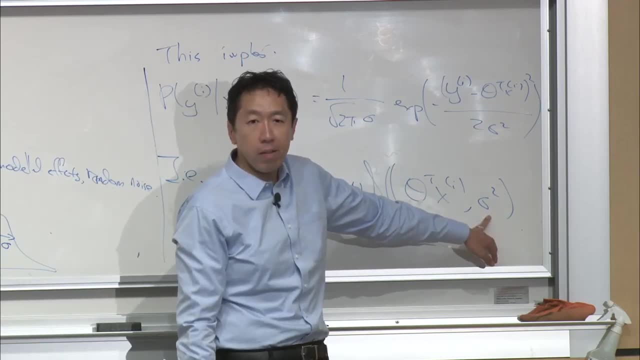 because the way that the price of a house is determined is by thinking: Theta transpose, x was the- you know the quote- true price of the house, and then adding noise or adding error of variance, Sigma squared to it, And so, um the- the assumptions on the left imply that, given x and Theta, 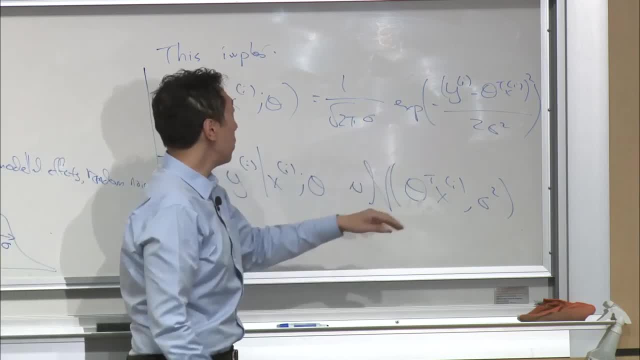 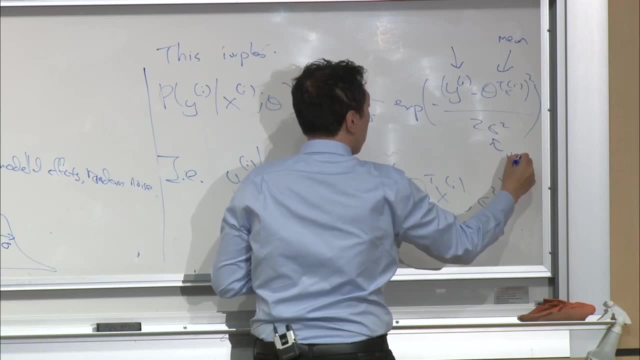 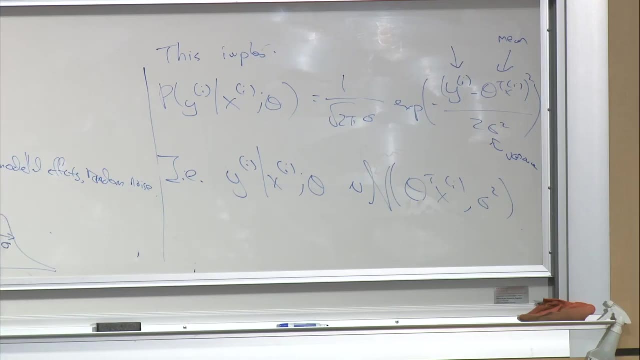 the density of y, you know, has this distribution which is really. this is the random variable, y, and that's the mean right, And that's the variance of a Gaussian density. Okay, Now um two pieces of notation. 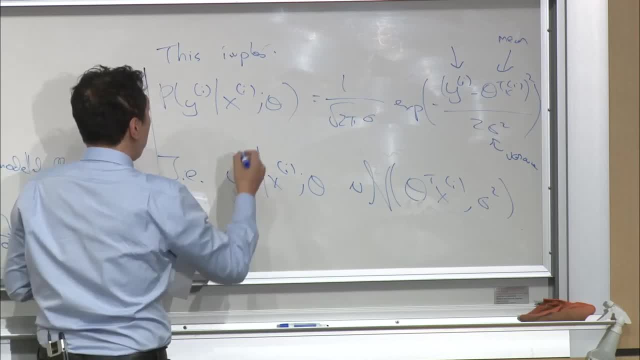 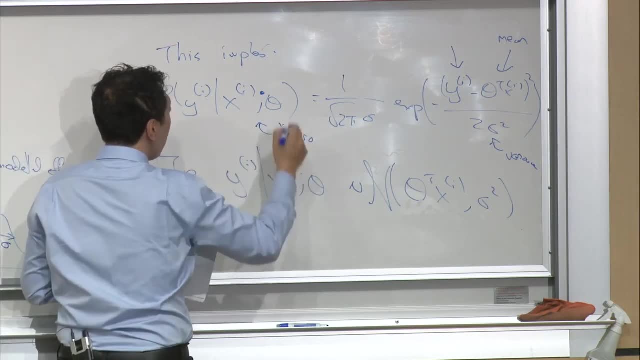 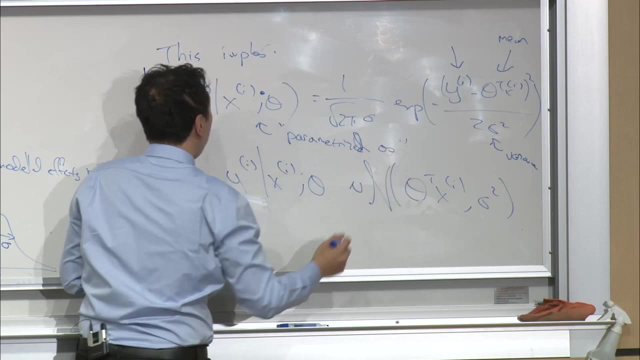 um, I wanna- one more that- that you should get familiar with. Um, the reason I wrote a semicolon here is, uh, that- the way you read this equation is. the semicolon should be read as: uh, parameterized as um. 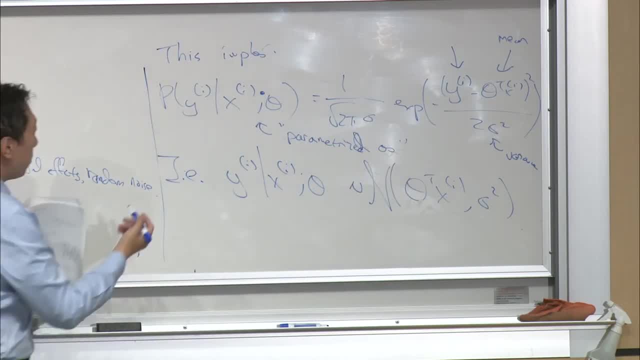 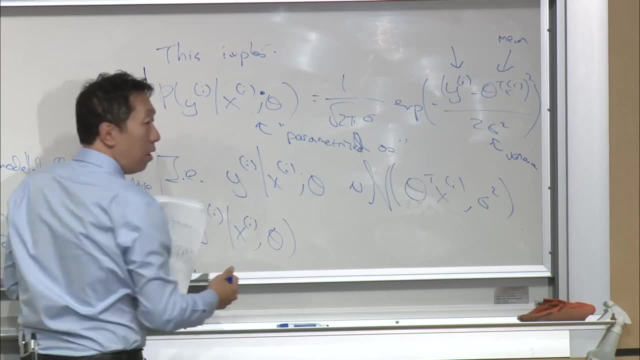 and so because, uh, uh, you know the- the alternative way to write this would be to say: p of x, i given y. i excuse me, p of y given x, i, comma Theta. But if you were to write this notation this way, 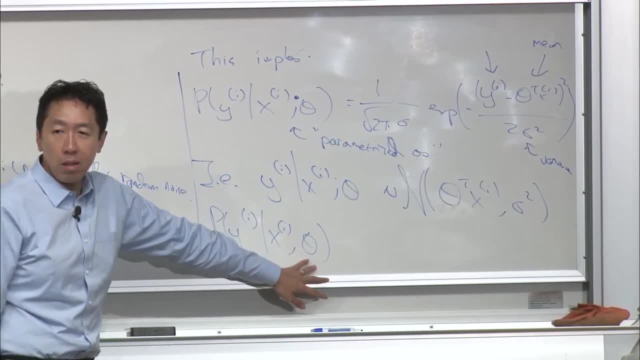 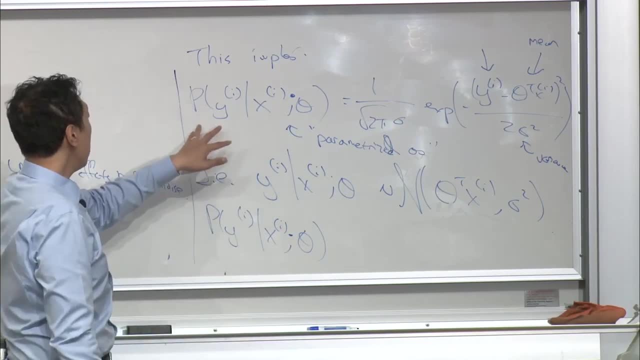 this would be conditioning on Theta, but Theta is not a random variable, So you shouldn't condition on Theta, which is why I'm gonna write a semicolon. a semicolon, And so the way you read this is the probability of y- i given x- i and parameterized. 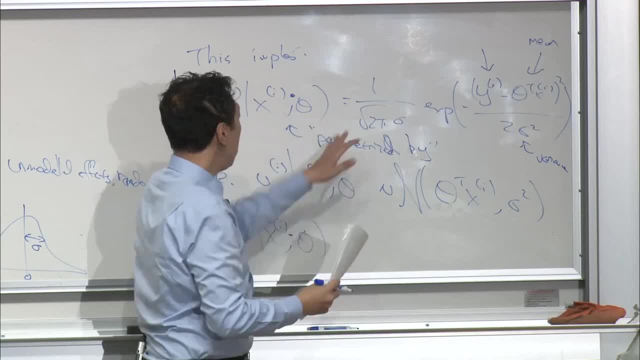 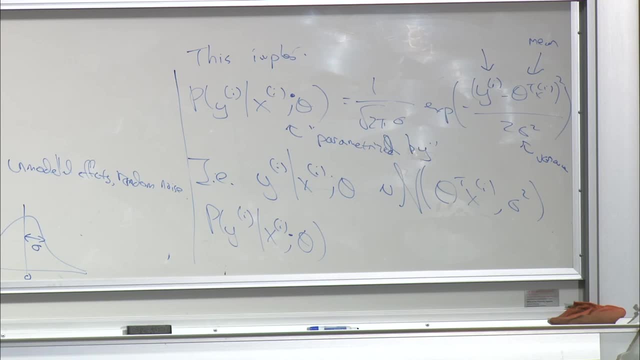 excuse me, parameterized by Theta is equal to that formula. Okay, Um, if- if-. if you don't understand this distinction again, don't worry too much about it. In- in statistics there are multiple schools of statistics called Bayesian statistics and frequency statistics. 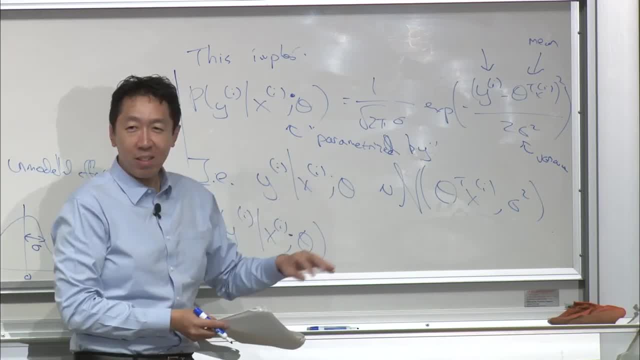 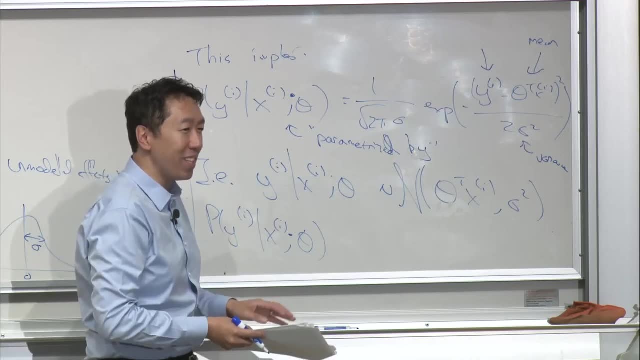 This is a frequencies interpretation. uh, for the purposes of machine learning, don't worry about it. but I find that being more consistent with terminology prevents some of our statistician's friends. I'm getting really upset, that- that- that you know. 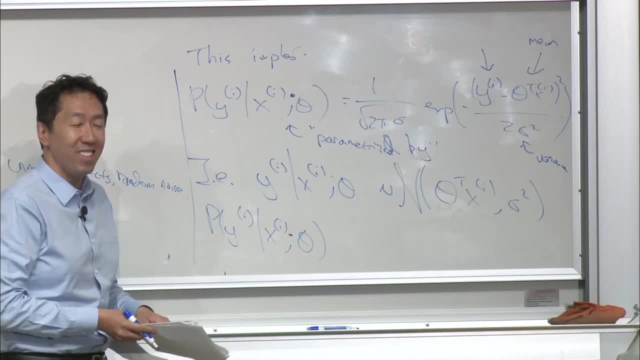 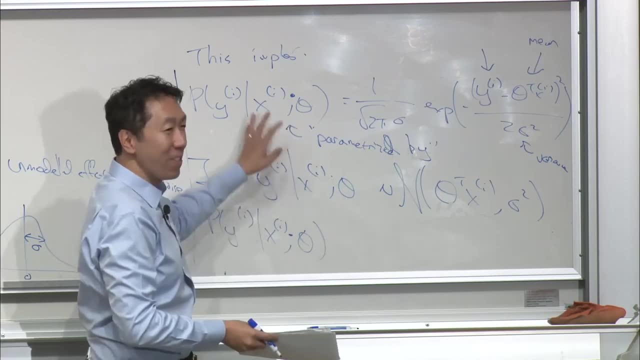 So I'm- I'll try to follow statistics convention, uh, uh. so, because just don't need unnecessary flack, I guess. Um, but for the pr- for practical purposes, it's not that important If you get this notation wrong in your homework. 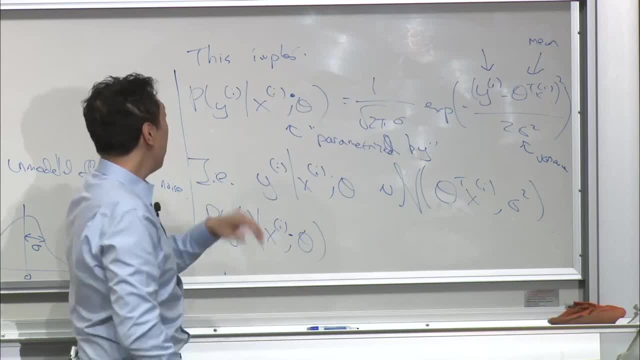 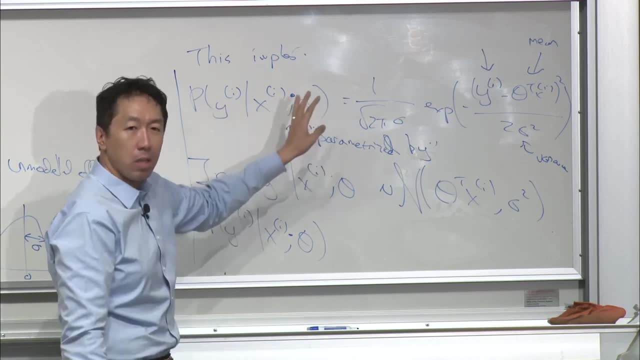 don't worry about it, we won't penalize you, but I'll try to be consistent. Um, but this just means that Theta, in this view, is not a random variable, it's just. Theta is a set of parameters that parameterizes this probability distribution. 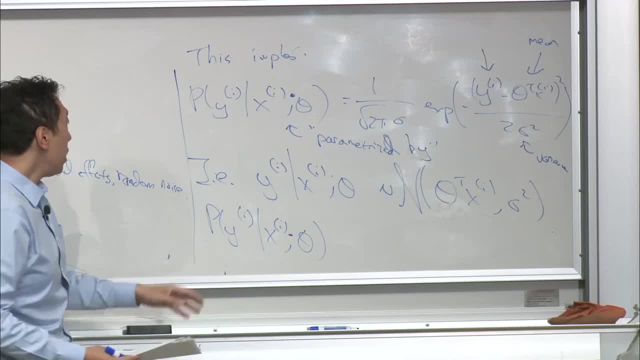 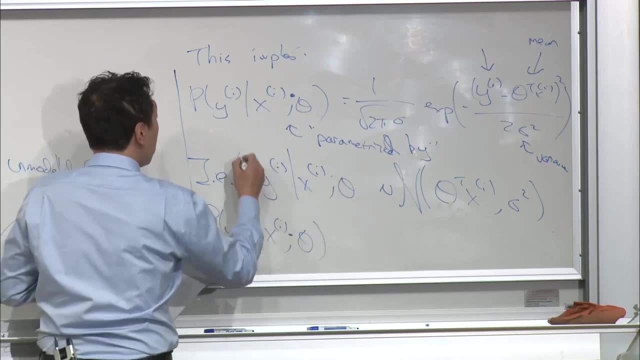 Okay, Um, and the way to read this. the second equation is: um. when you write these equations, you usually don't write them with parentheses, but the way to pause this equation is to say that this thing, as a random variable. 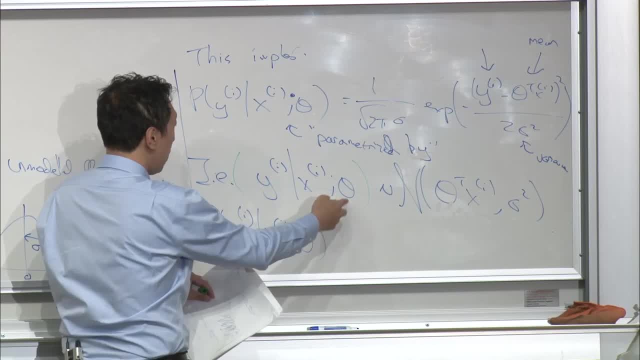 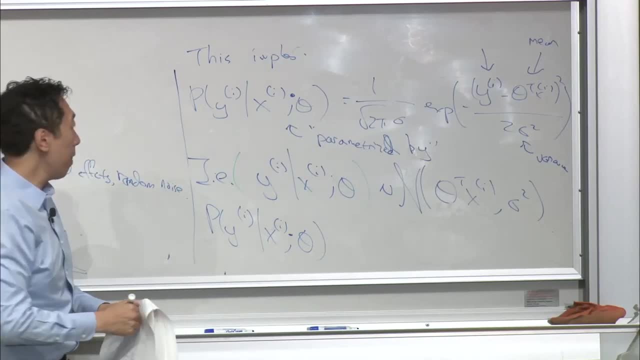 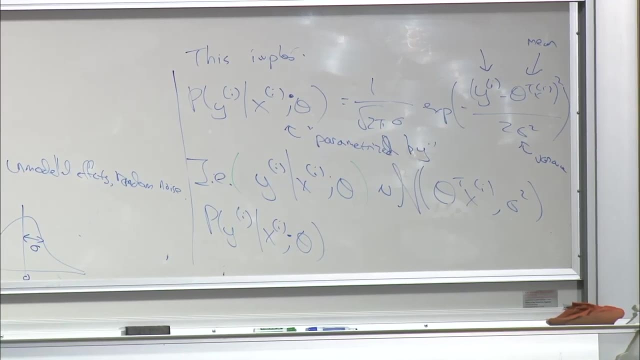 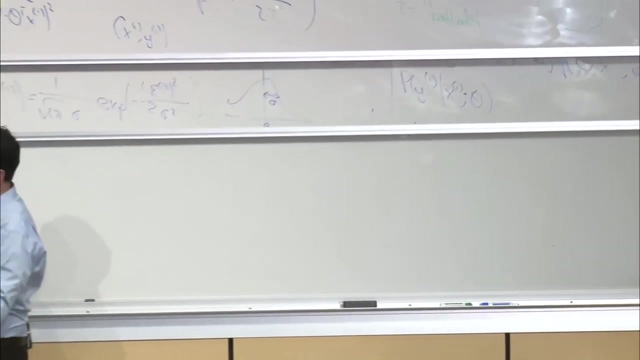 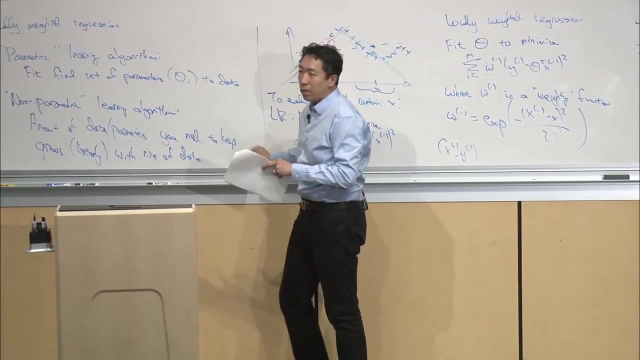 the random variable Y, given X and parameterized by Theta. this thing that I just drew in green parentheses is distributed to a Gaussian with that distribution. Okay, Okay, All right. Um, any questions about this? Okay, Cool, So it turns out that if you are willing to make those assumptions, 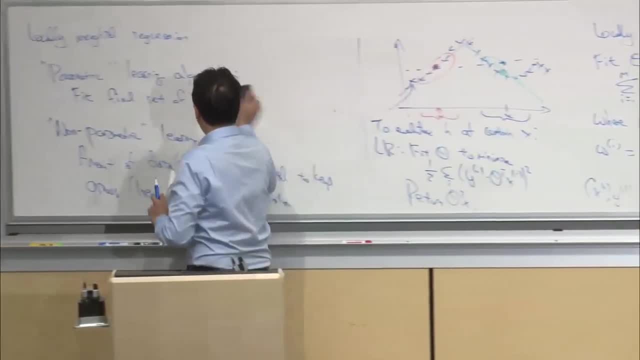 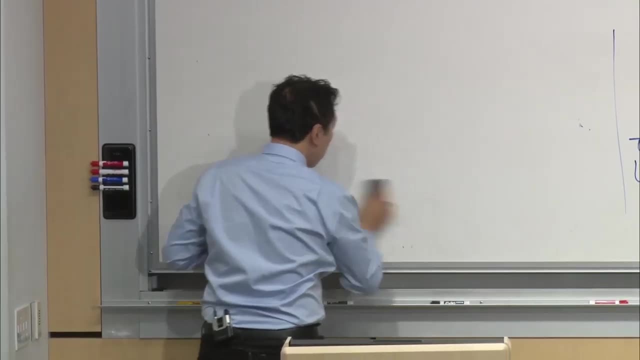 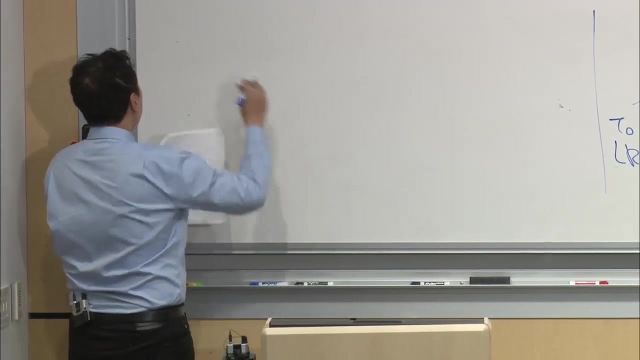 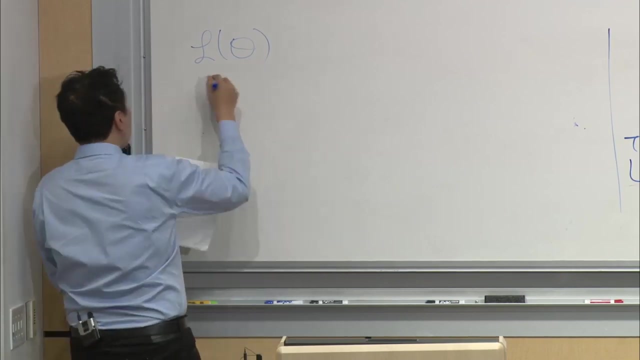 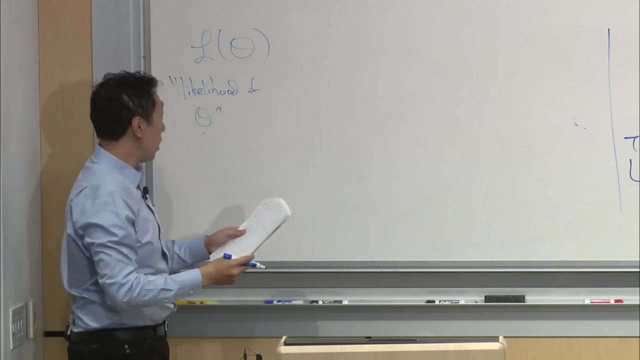 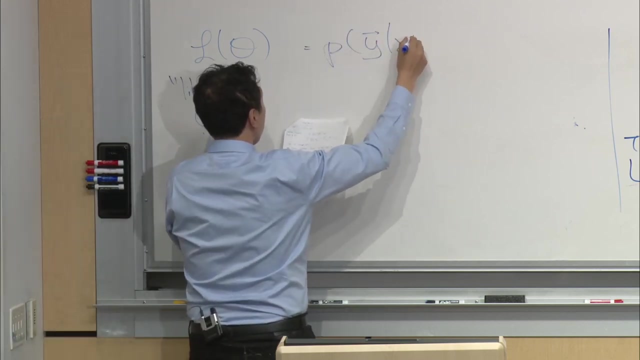 then linear regression um falls out almost naturally of the assumptions we just made And in particular, under the assumptions we just made um the likelihood of the parameters Theta- So this is pronounced: the likelihood of the parameters Theta, uh L of Theta, which is defined as the probability of the data right. 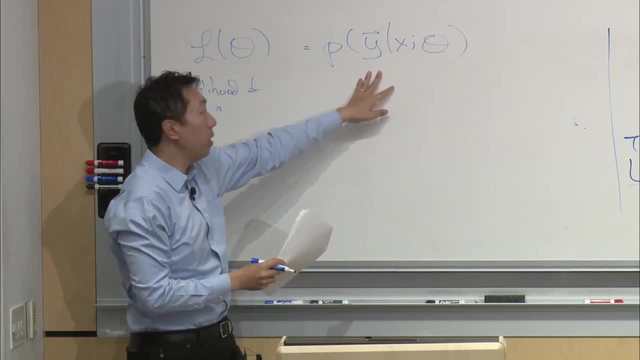 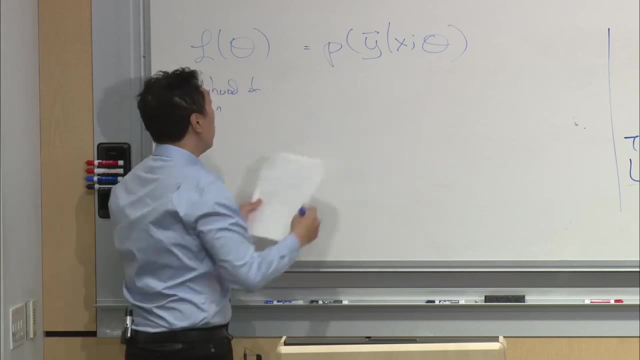 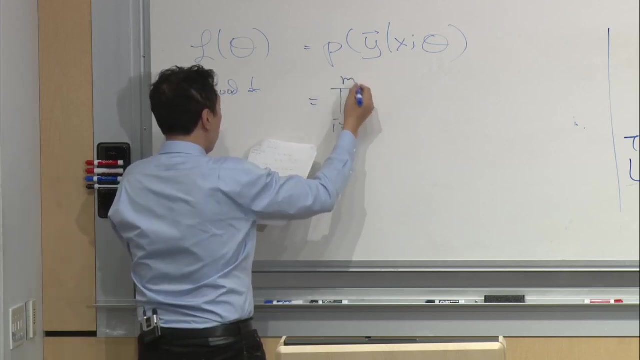 So this is probably of all the values of Y, of Y1 up to Ym, given all the Xs and given uh the parameters, Theta, parameterized by Theta Um. this is equal to the product from: i equals 1 through m of p, of yi, given xi. 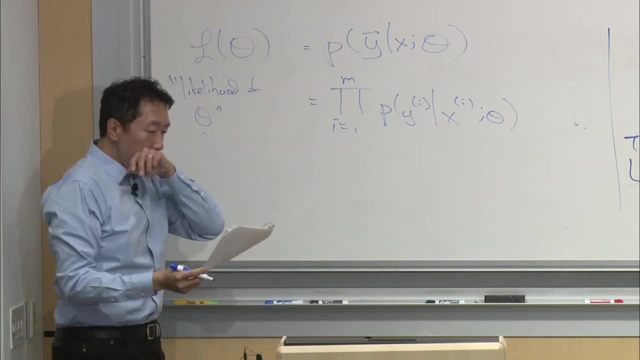 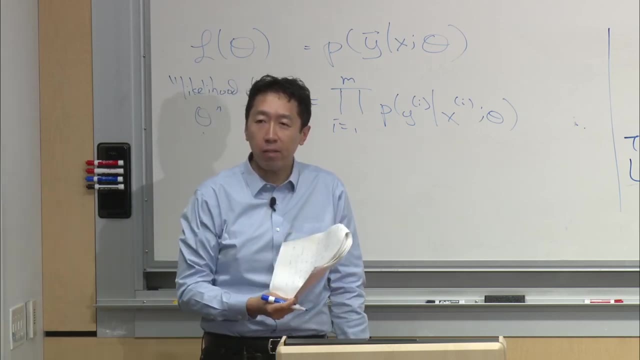 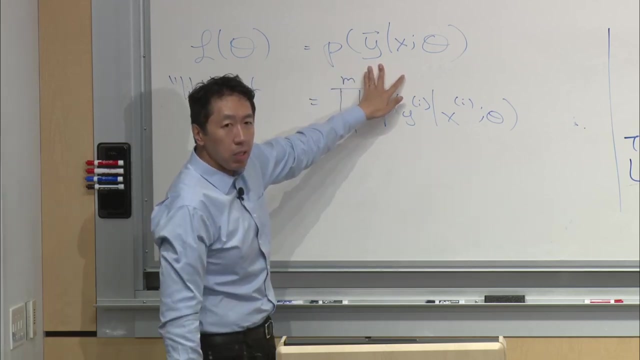 parameterized by Theta um, because we assume the examples were- because we assume the errors are iid right, That the error terms are independently and identity distributed to each other. So the probability of all of the observations, of all the values of y in 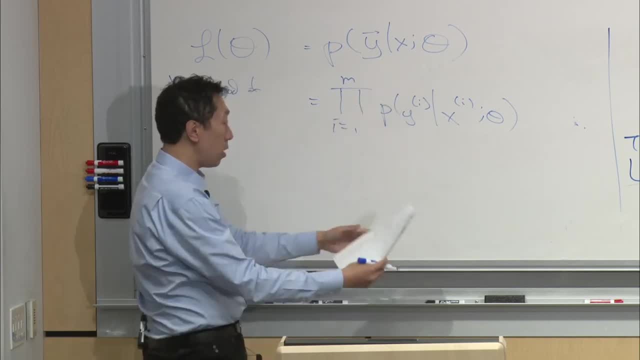 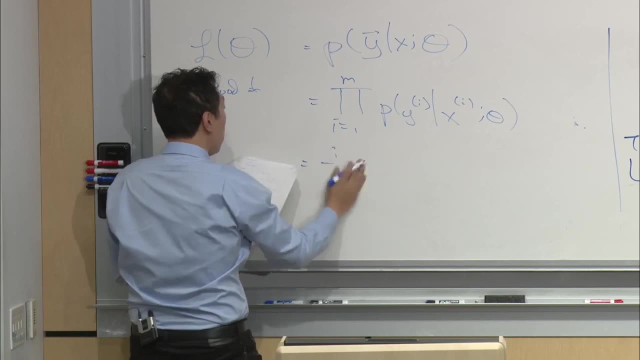 your training set is equal to the product of the probabilities, because of the independence assumption we made And so, plugging in the definition of p of y, given x parameterized by Theta that we had up there, this is equal to product of that. 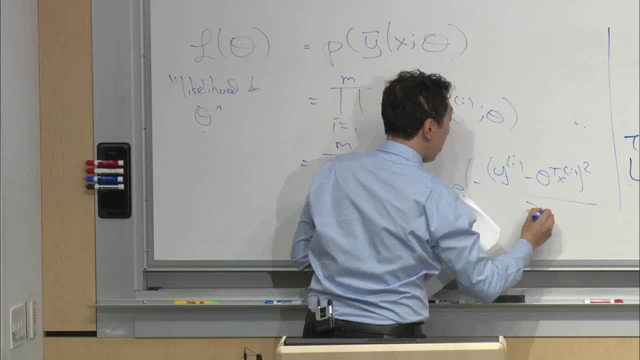 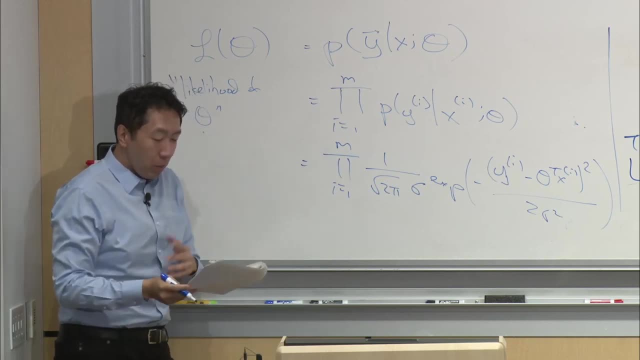 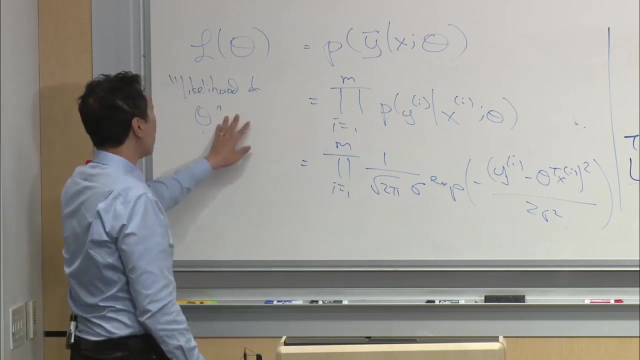 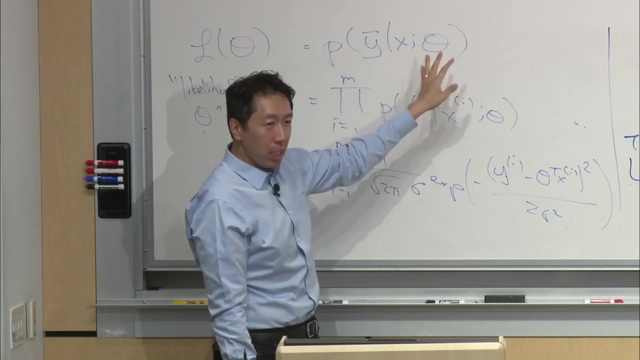 Okay, Now, um, again one more piece of terminology, Uh, you know. another question about Banal is we say: hey, Andrew, what's the difference between likelihood and probability? right, And so the likelihood of the parameters is exactly the same thing as the probability of the data. 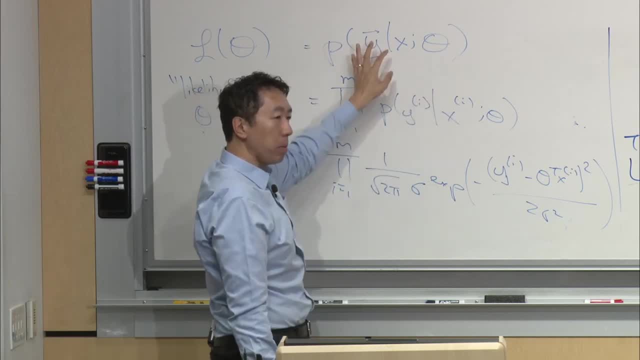 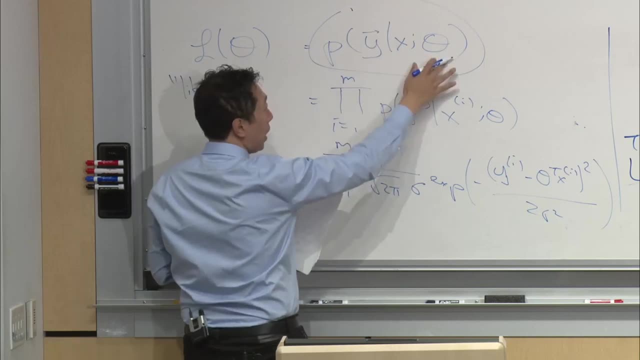 Uh, but the reason we sometimes talk about likelihood and sometimes talk about probability is, um, we think of likelihood, So this- this is some function, right? This thing is a function of the data as well as a function of the parameters. Theta. 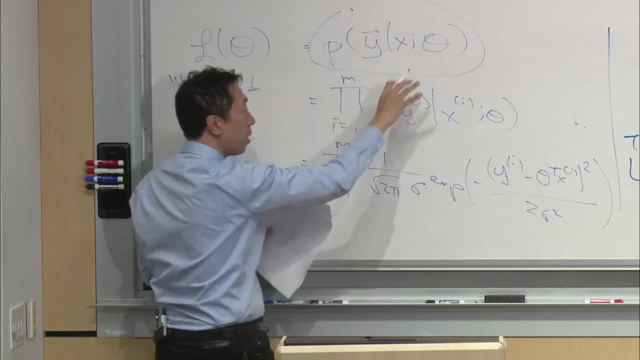 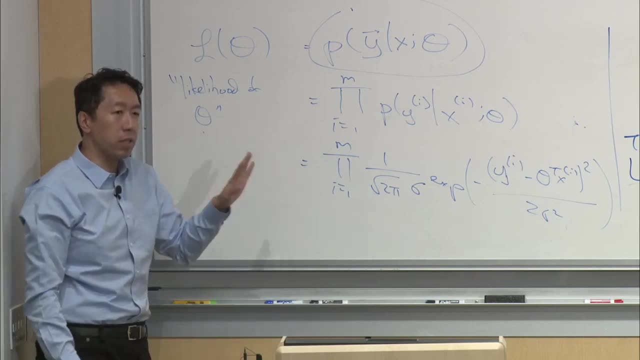 And if you view this number- whatever this number is- if you view this thing as a function of the parameters holding the data fixed, then we call that the likelihood. So if you think of the training set, the data is a fixed thing. 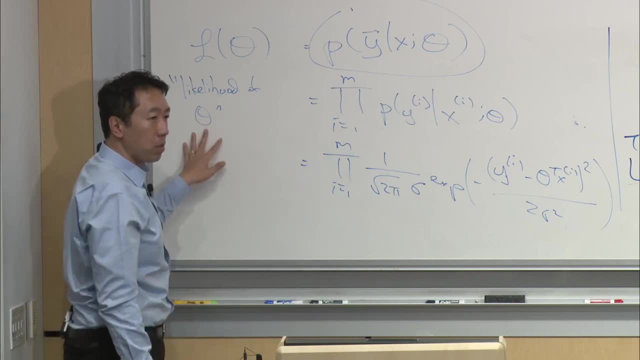 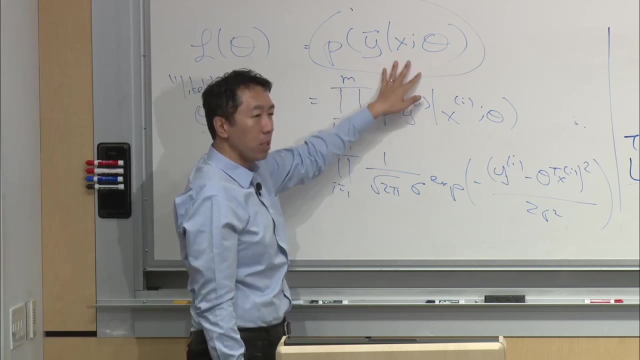 and then varying parameters Theta, then I'm gonna use the term likelihood, Whereas if you view the parameters Theta as fixed and maybe varying the data, I'm gonna say probability. Right, So- so you hear me use well, ho- I'll- I'll try to be consistent. 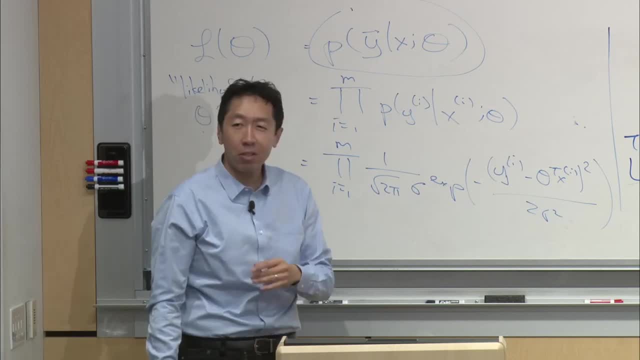 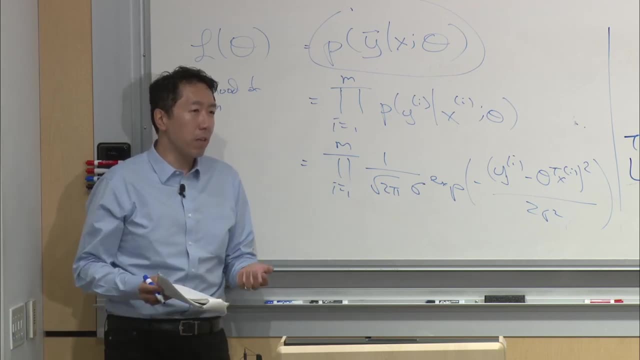 I find I'm- I'm pretty good at being consistent, but not perfect. But I'm gonna try to say likelihood of the parameters and probability of the data, even though those evaluate to the same thing. it's just, you know, for this function. 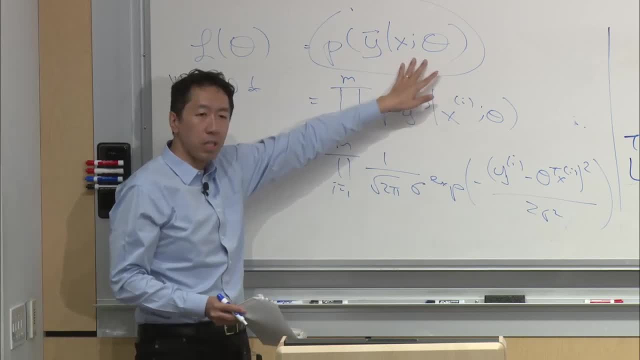 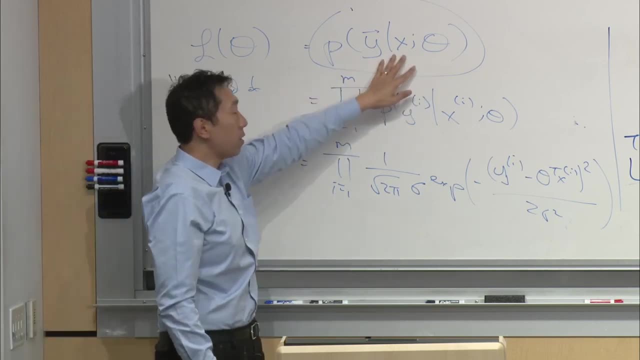 this function is a function of data and the parameters: which one are you viewing as fixed and which one are you viewing as- as variable? So when you view this as a function of Theta, I'm gonna use the term likelihood. Uh, but so- so hopefully you hear me say likelihood of. 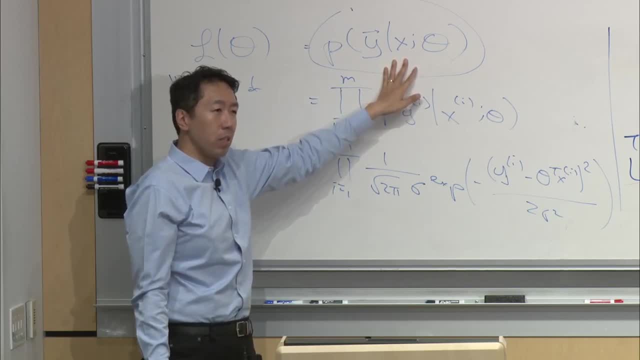 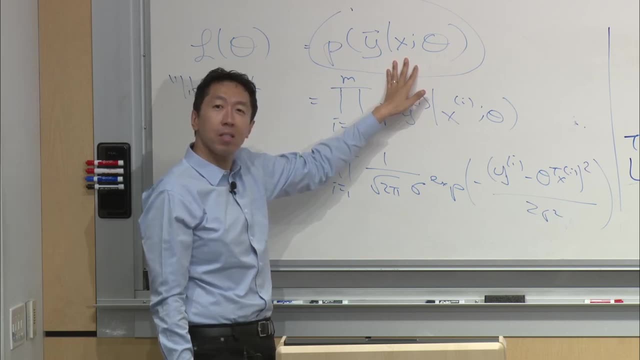 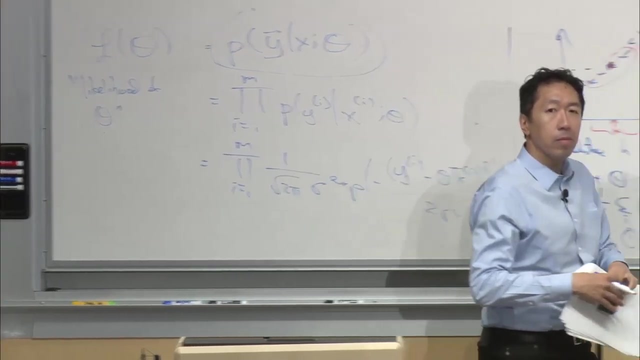 the parameters. hopefully you won't hear me say likelihood of the data- Right And- and similarly, hopefully you hear me say probability of the data and not the probability of the parameters. Okay, Okay, Yeah, Likely of the parameters. 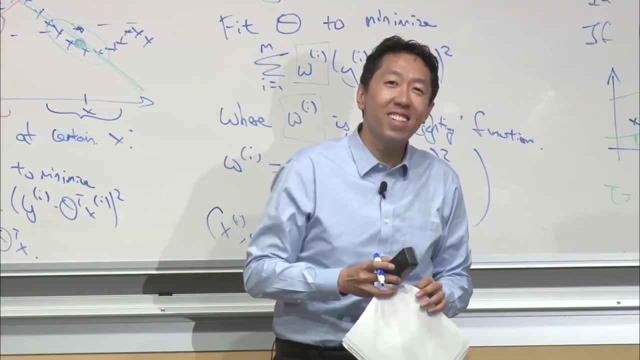 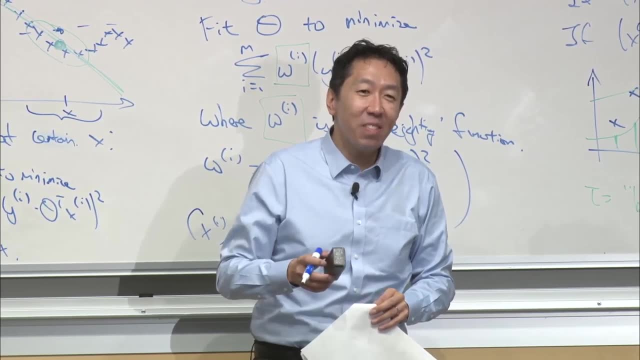 Uh, okay. So probability of the data: No, Uh, uh, Oh, Theta Got it. Sorry, Yes, likelihood of Theta Got it. Yes, Sorry, Yes, likelihood of Theta. That's correct. 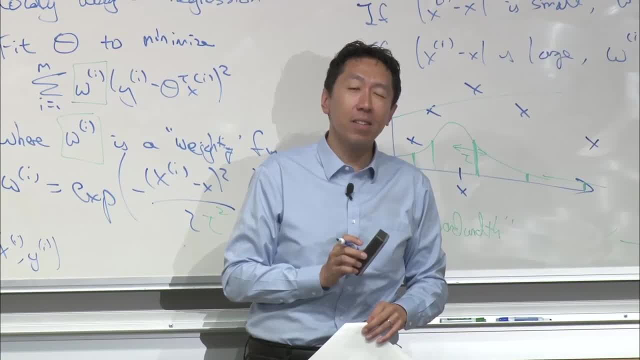 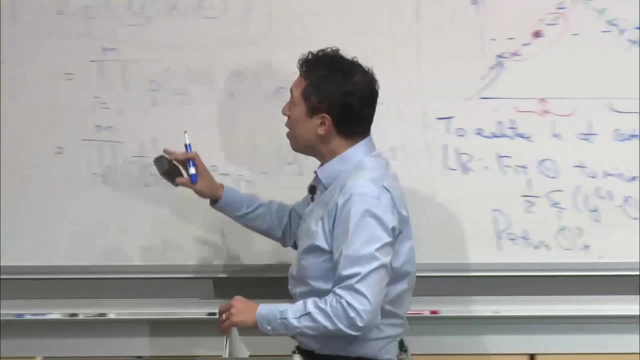 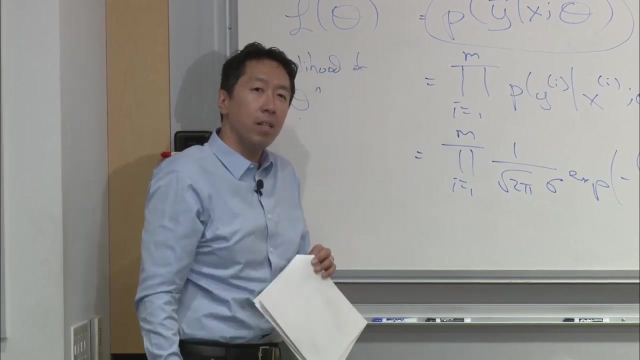 Oh, uh, no, So, no, uh, uh. so Theta is a set of parameters, It's- it's not a random variable. So likelihood of Theta doesn't mean Theta is a random variable, Right, Cool, Yeah, Thank you. 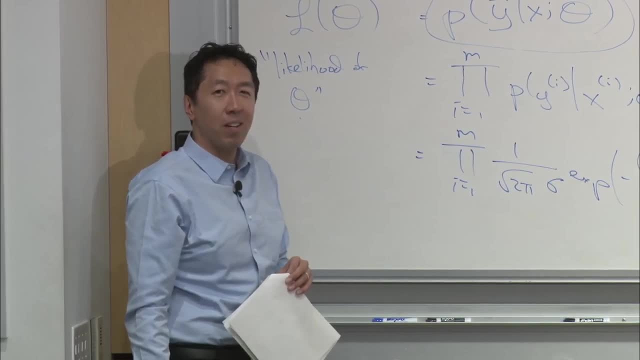 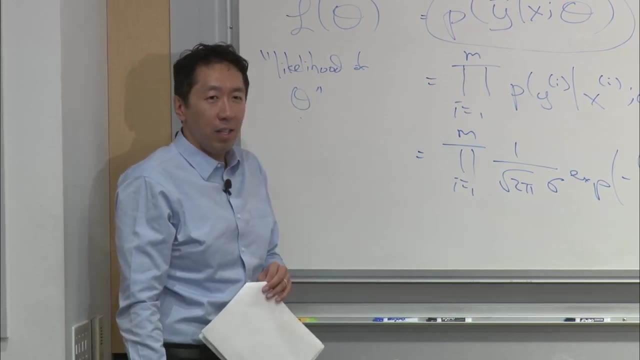 Um, by the way, the- the stuff about what's a random variable and what's not, to semicolon versus comma thing. We explained this in more detail in the lecture notes. To me, this is part of um uh. 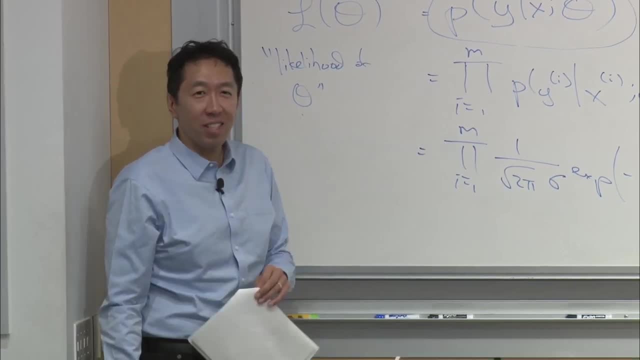 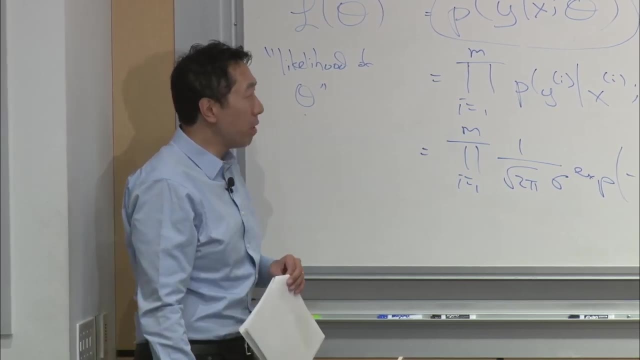 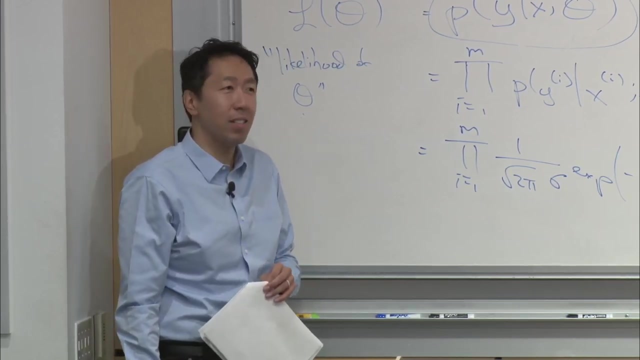 you know a little bit, paying homage to the, to the religion of Bayesian frequencies versus Bayesian uh frequencies versus Bayesian statistics From a, from a machine, from applied machine learning, operational. what you write, code point of view, it doesn't matter that much. uh, yeah. 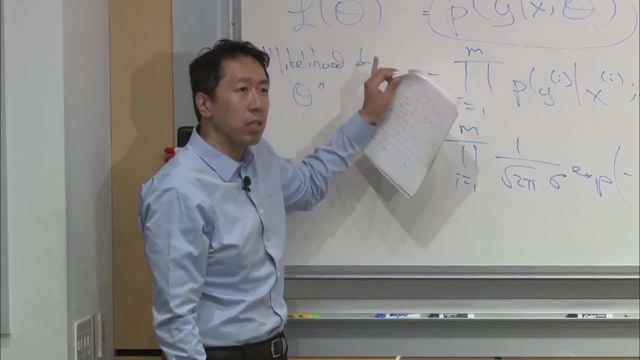 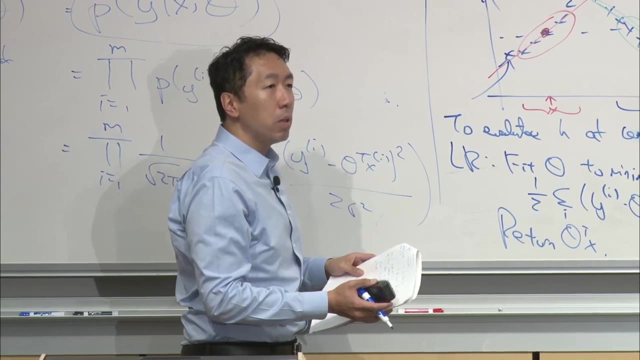 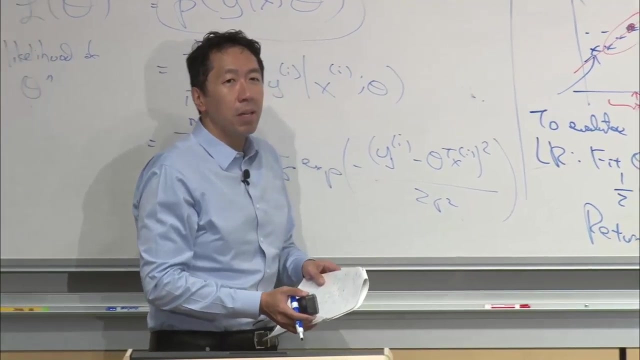 But Theta is not a random variable. We have likelihood of parameters which are not a random variable. Yeah, Oh, what's the rationale for choosing? uh- Oh sure, Why is epsilon i Gaussian? Uh, so, uh, uh, it turns out because the central limit theorem. 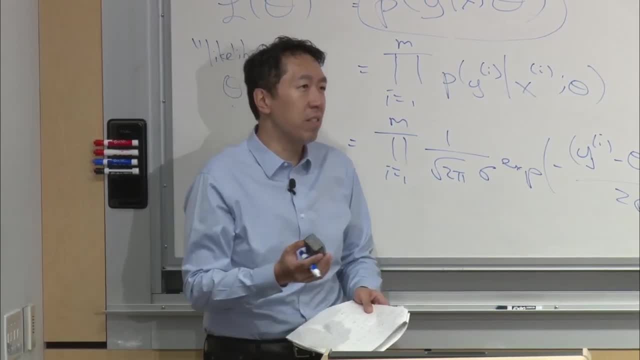 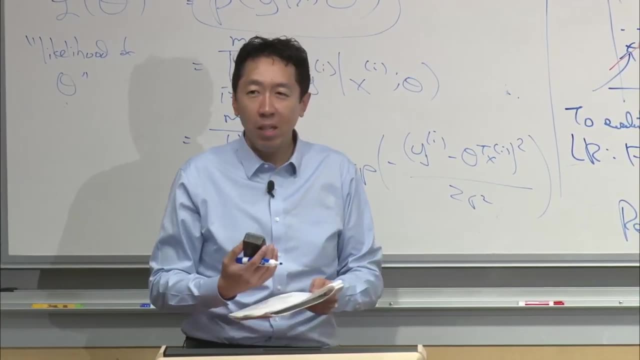 uh, from statistics, uh, most error distributions are Gaussian, right? If something is- if there's an error that's made up of lots of low noise sources which are not too correlated, then by the central limit theorem, it will be Gaussian. 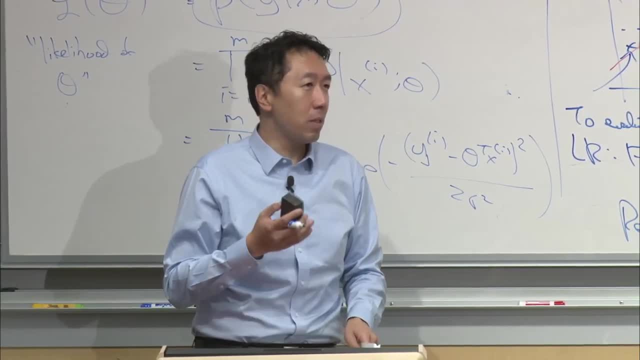 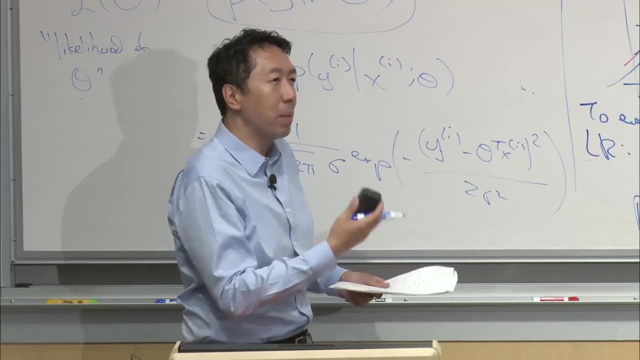 So if you think that how the- the noise perturbations are the mood of the cellar, what's the school district, you know what's the weather, like access to transportation and all of these sources are not too correlated and you add them up. 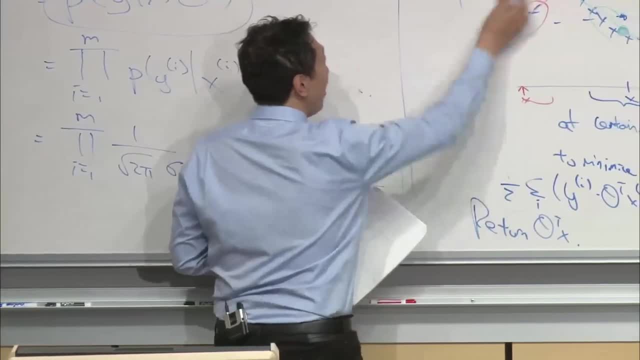 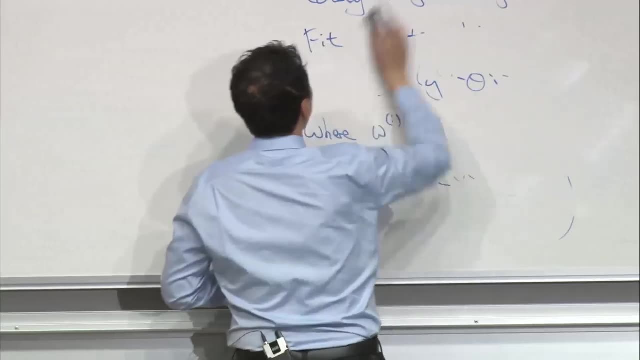 then the distribution will be Gaussian, Um, and, and I think, well, yeah, So really, because the central limit theorem, I think the Gaussian- has become a default noise distribution. But for things where the true noise distribution is very far from Gaussian, 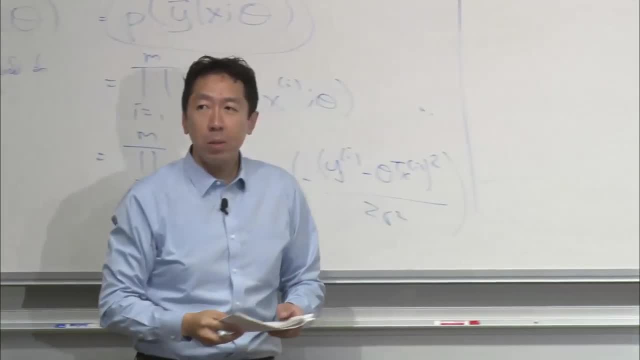 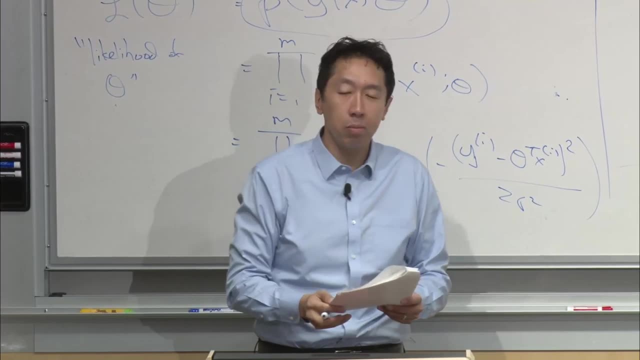 uh, this model does do that as well And, in fact, for when you see generalized linear models on Wednesday, you see when- how to generalize all of these algorithms to very different distributions like Poisson and so on. All right, So um. 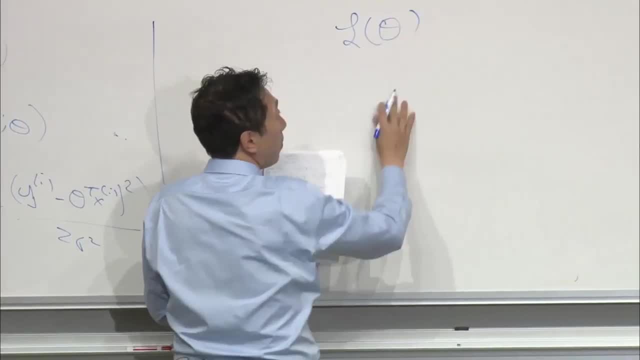 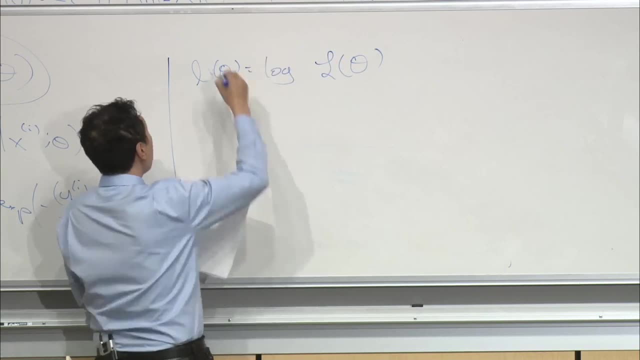 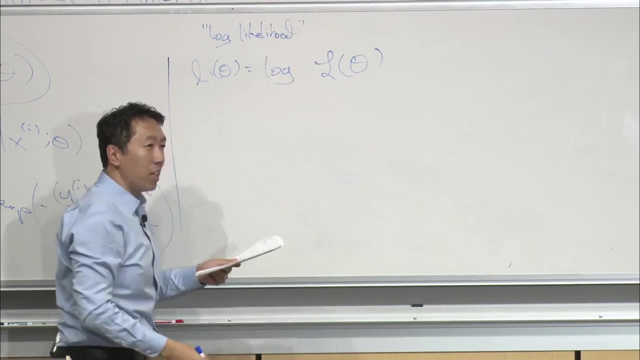 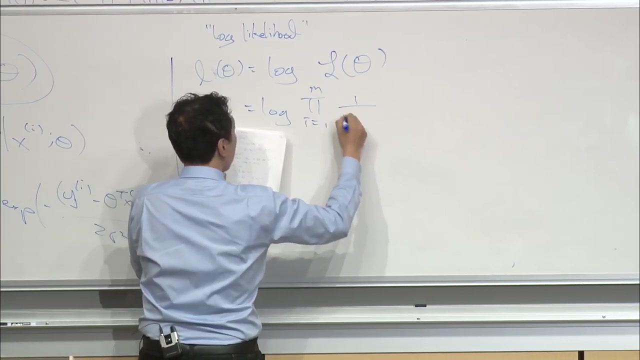 so we've seen the likelihood of the parameters theta, Um. so I'm gonna use lowercase l to denote the log likelihood. And the log likelihood is just a log of the likelihood, Um, and so well, let me just right. 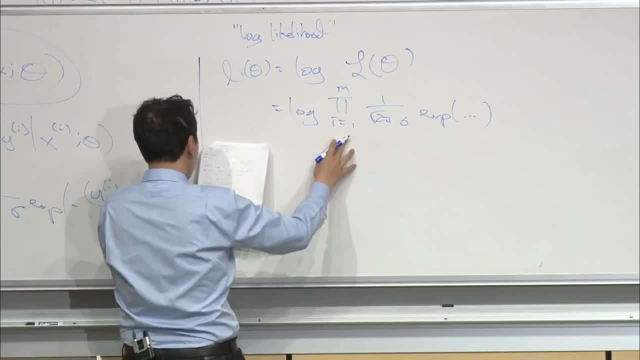 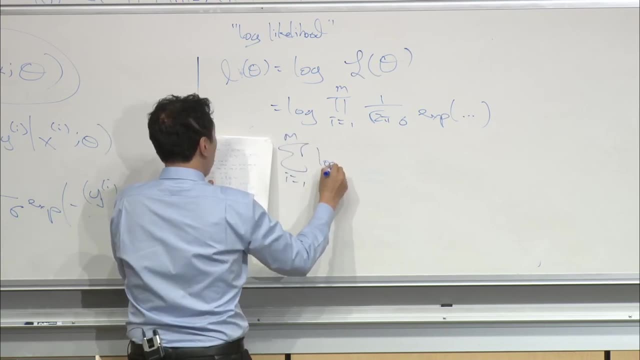 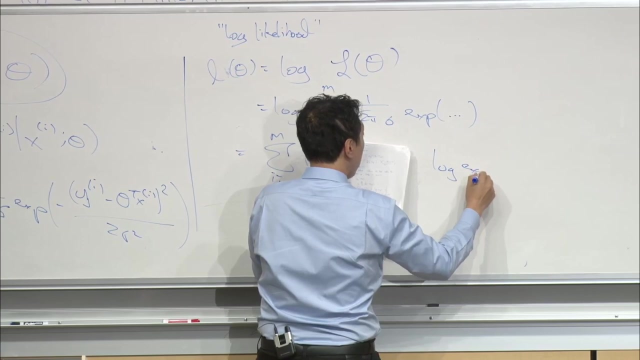 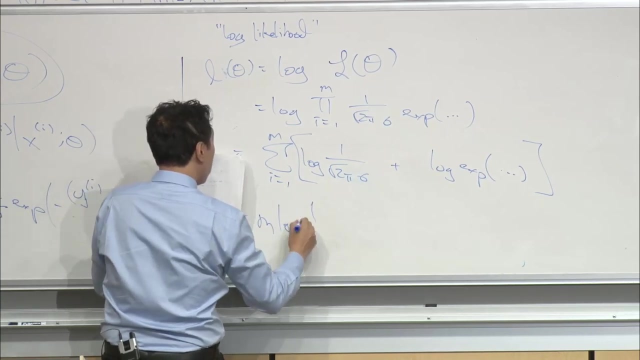 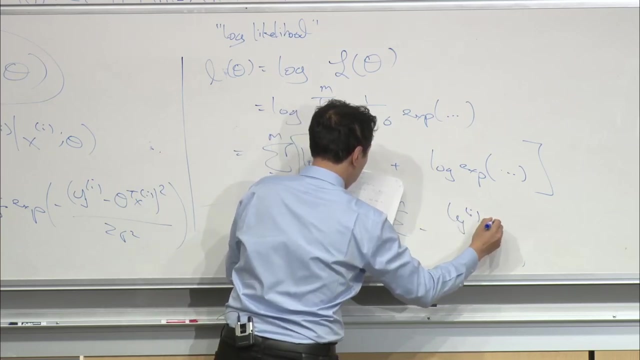 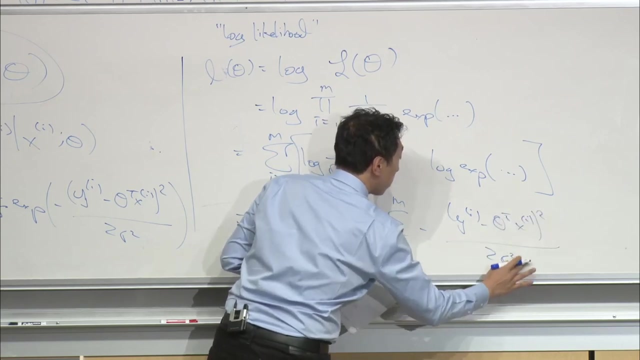 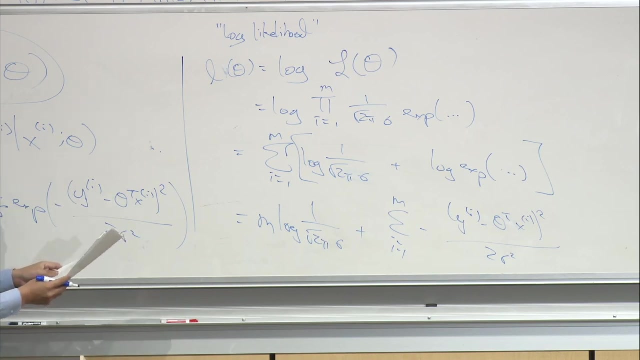 And so, um log of a product is equal to the sum of the logs, right, Uh, and so this is equal to, and so this is L log, one over root, Okay, Um and so, um, one of the, uh, you know, well-tested. 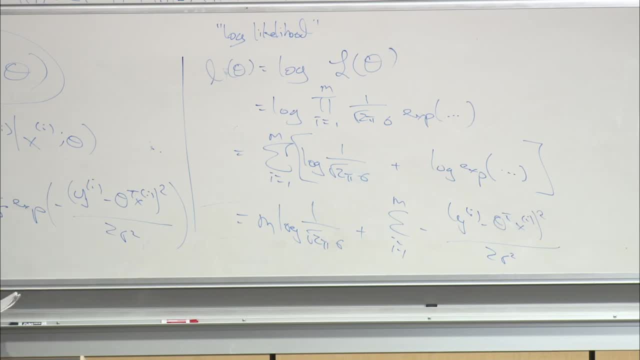 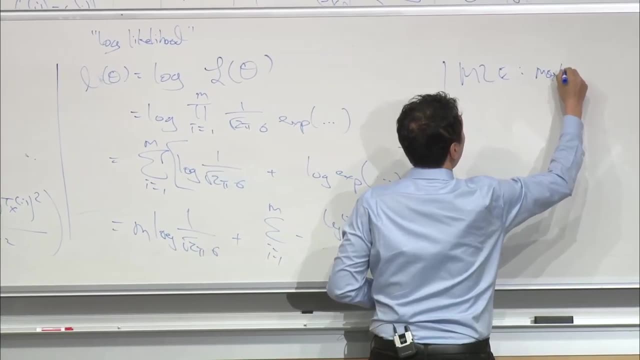 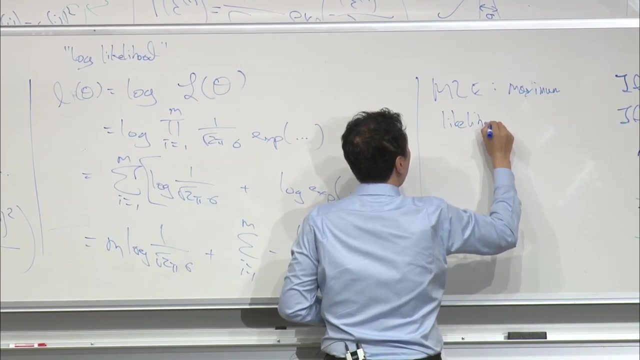 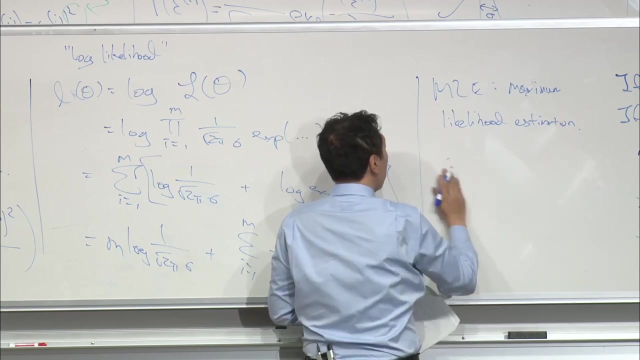 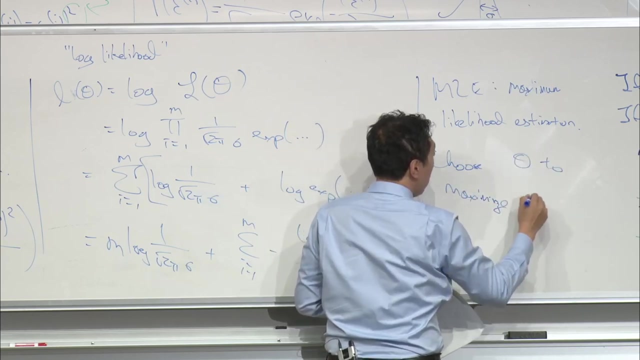 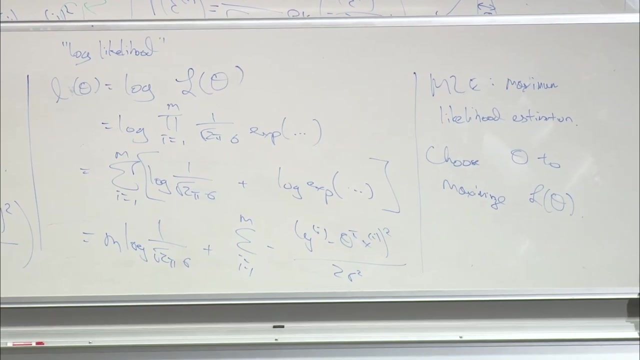 methods and statistics for estimating parameters is to use maximum likelihood estimation, or MLE, which means to choose Theta to maximize the likelihood right. So, given a dataset, how would you like to estimate Theta? Well, one natural way to choose Theta is to choose. 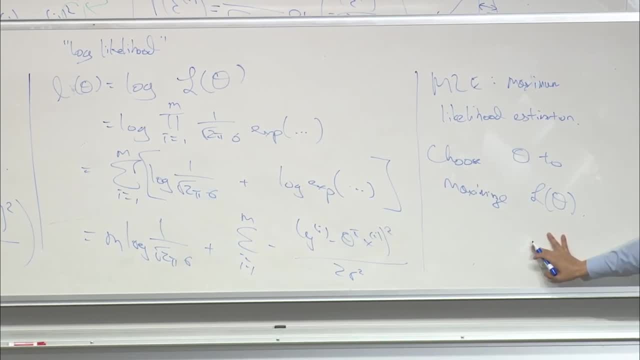 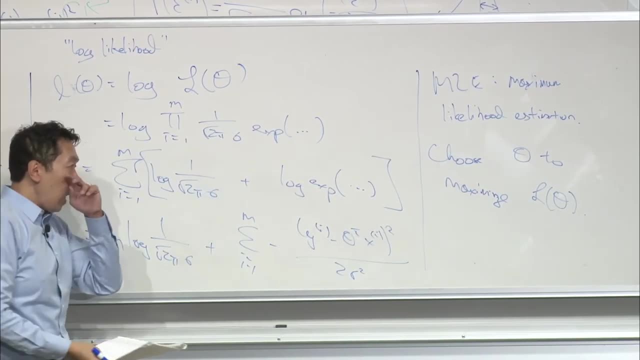 whatever value of Theta has the highest likelihood. Or in other words, choose the value of Theta so that that value of Theta maximizes the probability of the data right. And so, um for- uh, to simplify the algebra rather than maximizing. 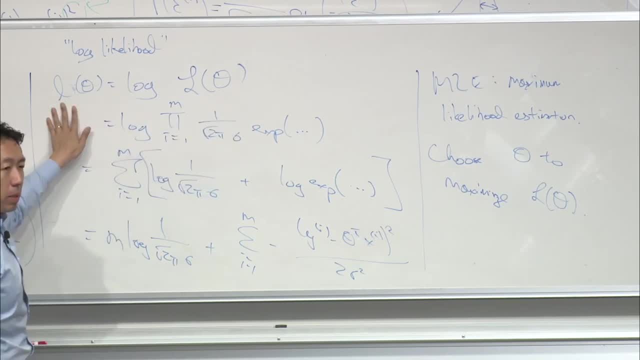 the likelihood. capital L is actually easier to maximize the log likelihood, But the log is a strictly monotonically increasing function. So the value of Theta that maximizes the log likelihood should be the same as the value of Theta that maximizes the likelihood. 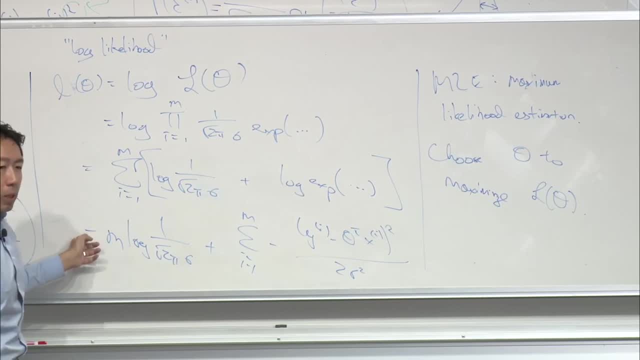 And if you derive the log likelihood, um, we conclude that if you're using maximum likelihood estimation, what you'd like to do is choose the value of Theta that maximizes this thing, right, But uh, this first term is just a constant. 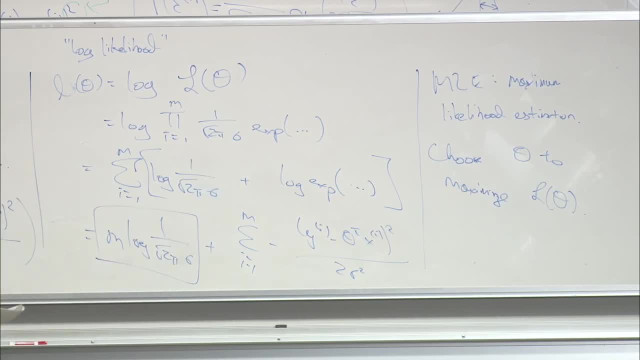 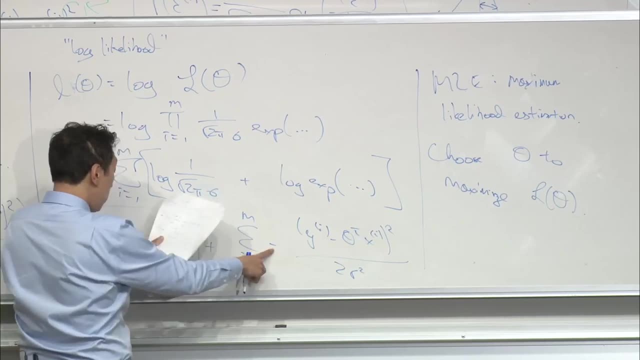 Theta doesn't even appear. It doesn't appear in this first term, And so what you'd like to do is choose the value of Theta that maximizes the second term. Uh, notice, there's a minus sign there, And so what you'd like to do is: 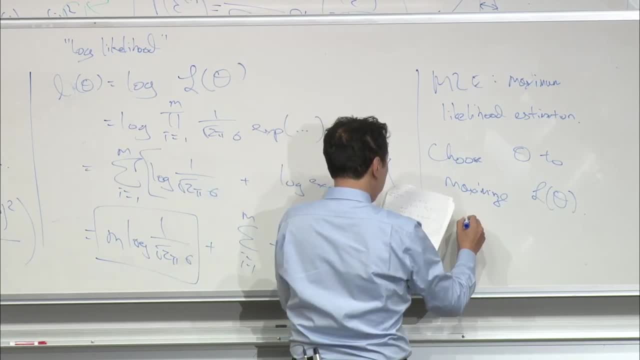 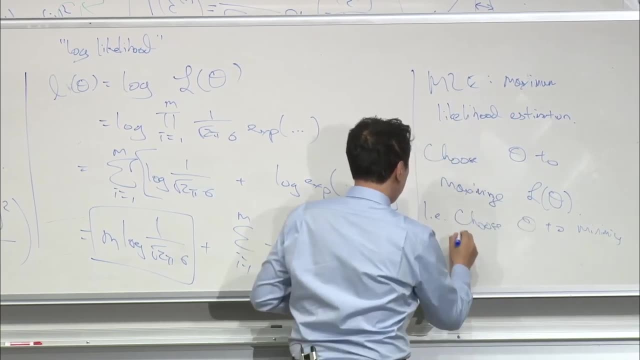 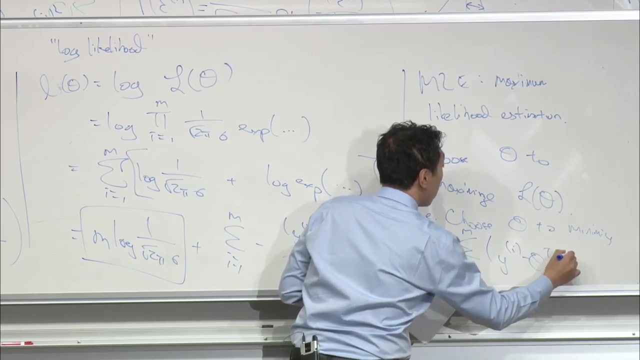 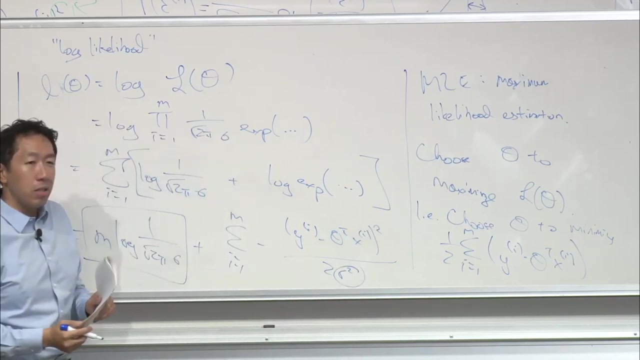 um, uh, ie, you know, choose Theta to minimize this term, Right? Oh, so sigma squared is just a constant right, No matter what sigma squared is, you know so, so, uh, so, if you want to minimize this term, excuse me, 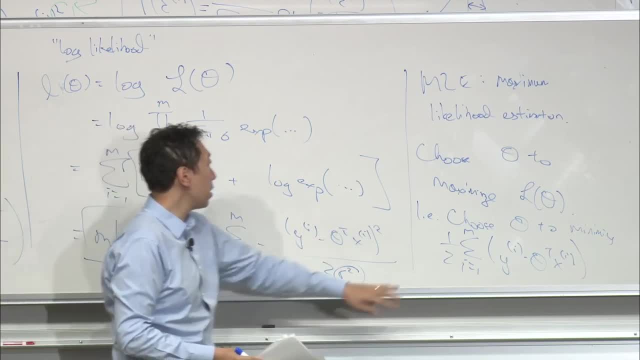 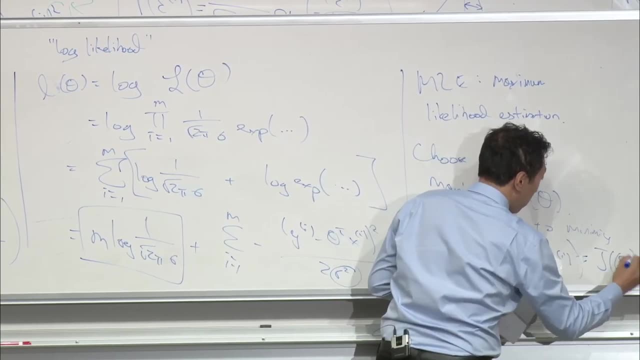 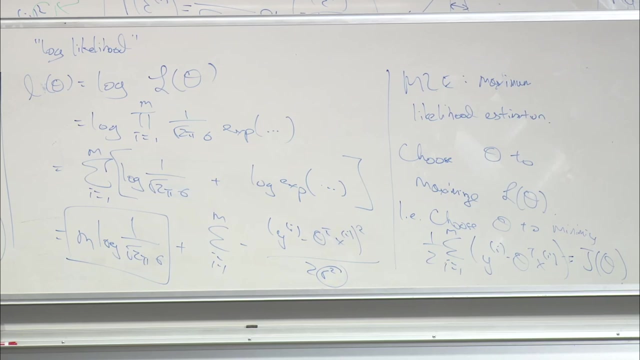 if you want to maximize this term negative of this thing, that's the same as minimizing this term. Uh, but this is just J of Theta, the cost function you saw earlier for linear regression. okay, So this little proof shows that um. 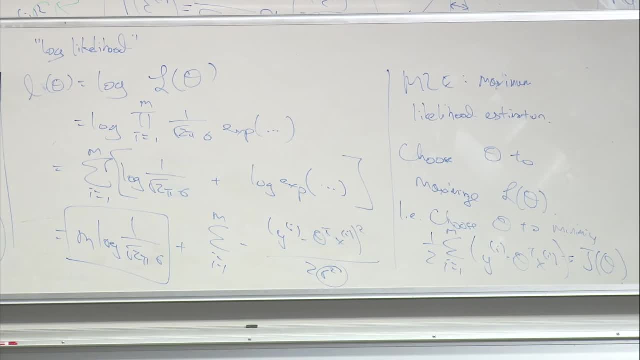 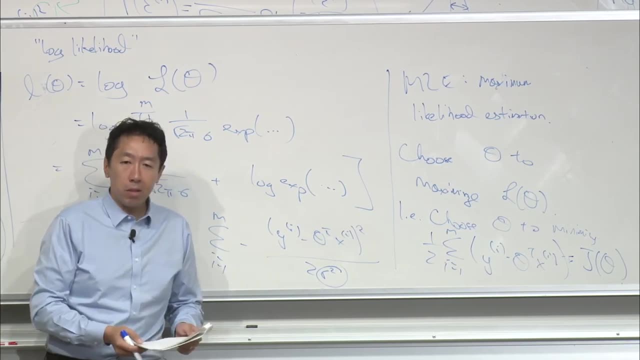 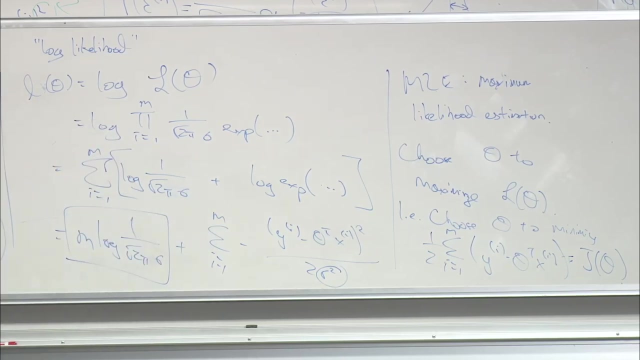 choosing the value of Theta to minimize the least squares errors, like you saw last Wednesday. that's just finding the maximum likelihood estimate for the parameters Theta under the set of assumptions we made that the error terms are Gaussian and iid. Okay, Um, go ahead. 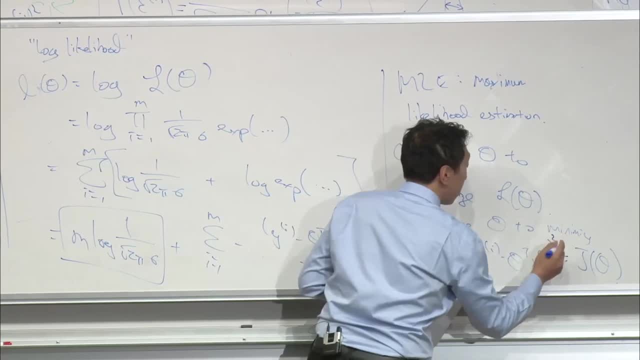 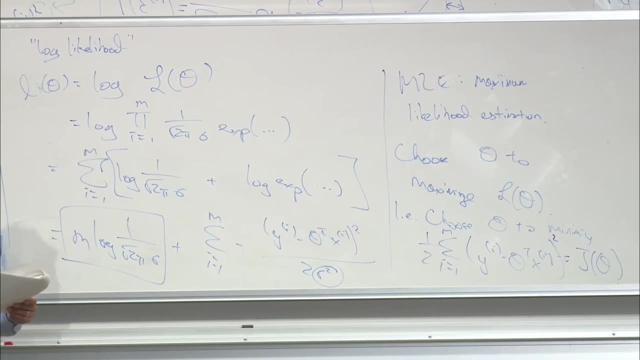 Oh, thank you. Yes, Great, Yeah, Thanks, Yeah, go ahead. Oh, is there a situation of using this formula to set the least squares cost? function with better idea? No, So this. I think this derivation shows that this. 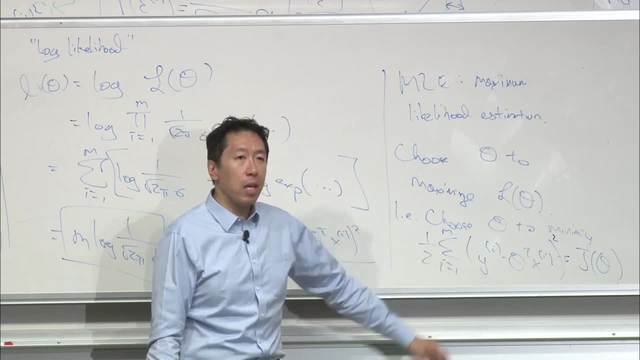 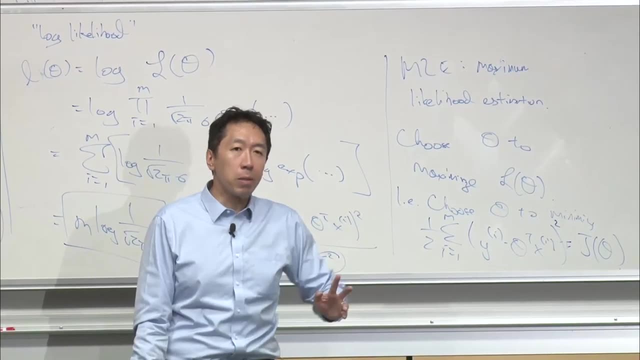 this is completely equivalent to least squares right. That if, if you want, if you're willing to assume that the error terms are Gaussian and iid, and if you want to use maximum likelihood estimation, which is a very natural procedure in statistics. 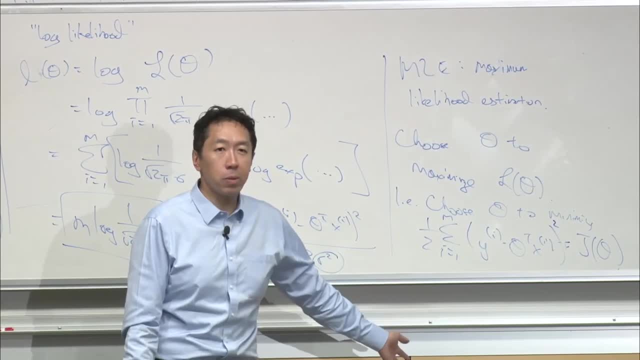 right. So if you want, if you're willing to assume that the error terms are Gaussian and iid, and if you want to use maximum likelihood estimation, which is a very natural procedure in statistics, then you know, then you should use. 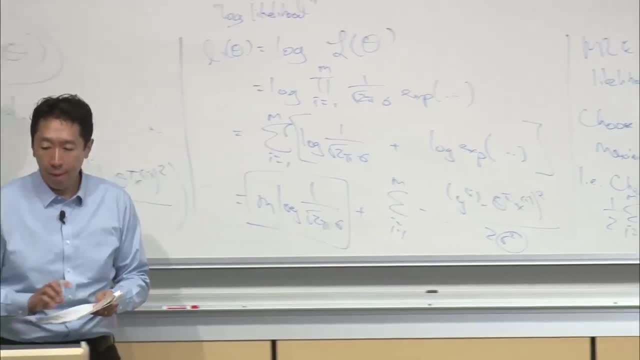 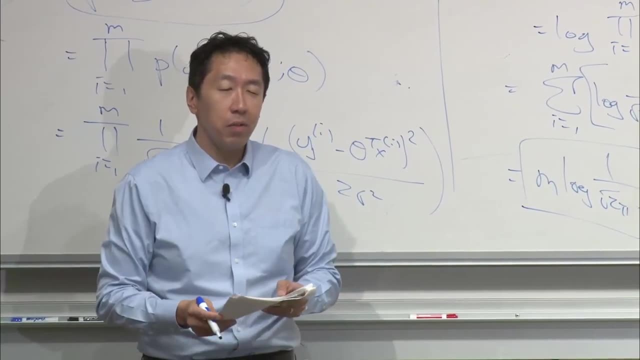 uh, uh, least squares right. So yeah, Did you know, for some reason, errors are not iid? Like, is there a better way? like, did you figure out a better cost function? Uh, if you knew, for some reason, errors are not iid. 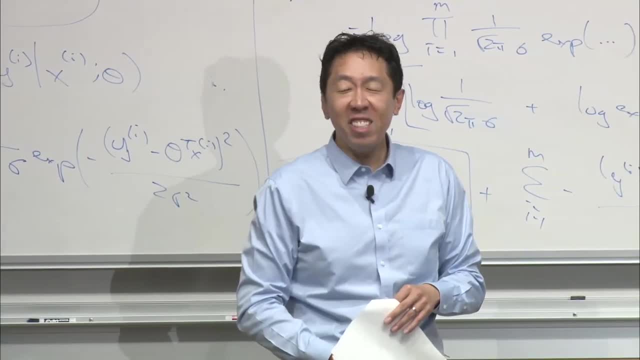 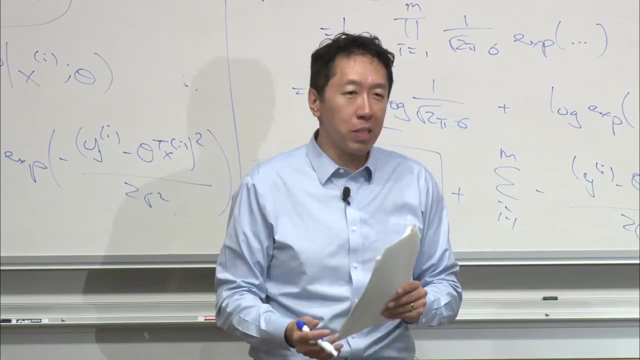 would you figure out a better cost function? Uh, yes and no. I think that, um, you know, when building learning algorithms? uh, often we make model, we make assumptions about the world that we just know are not 100 percent true, because it leads to algorithms. 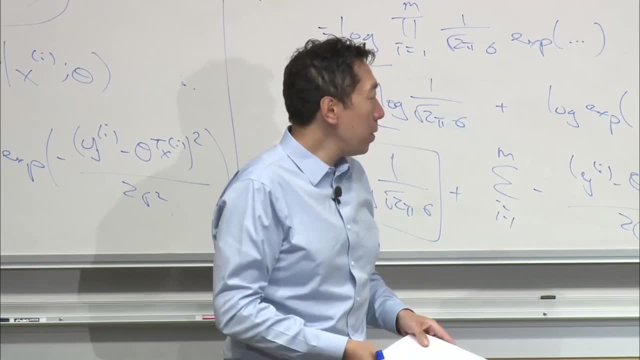 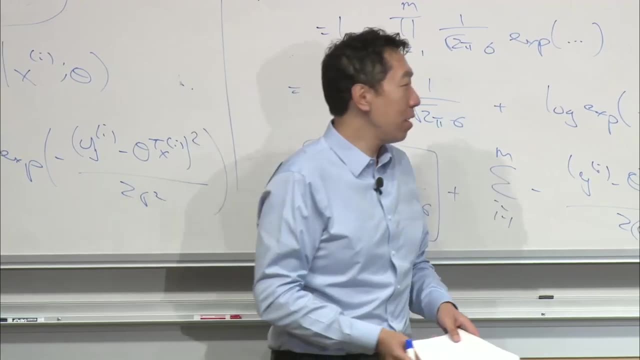 that are computation efficient. um, and so, if you knew that your, if you knew that your training set was very, very non-iid, there are, there are more sophisticated models you could build, But um, uh, uh, yeah. 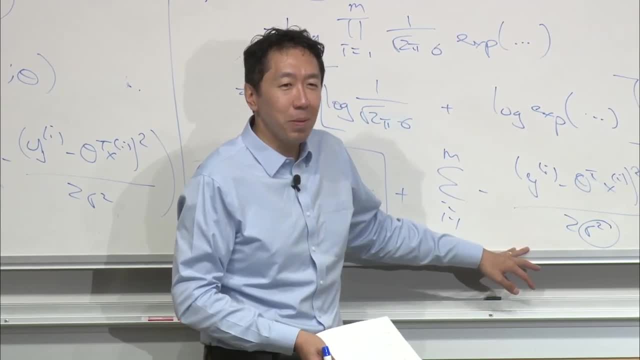 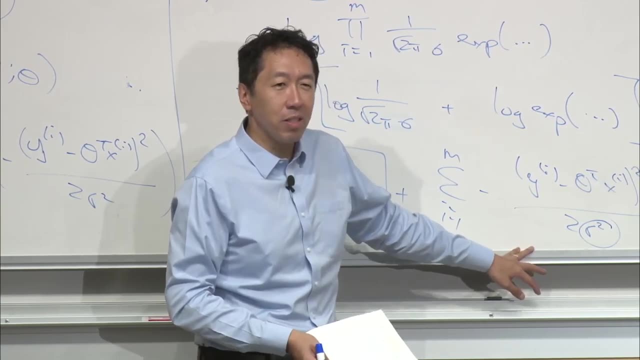 But but very often we wouldn't bother. I think, Yeah, More often than not we might not bother. Uh, I can think of a few special cases where you would bother, but only if you think the assumptions are really really bad, uh, if you don't have enough data, and so on, and so on. 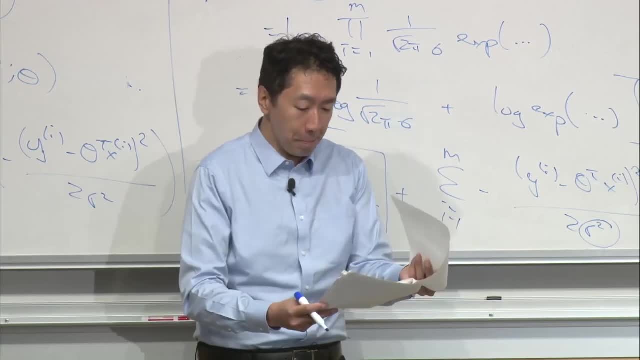 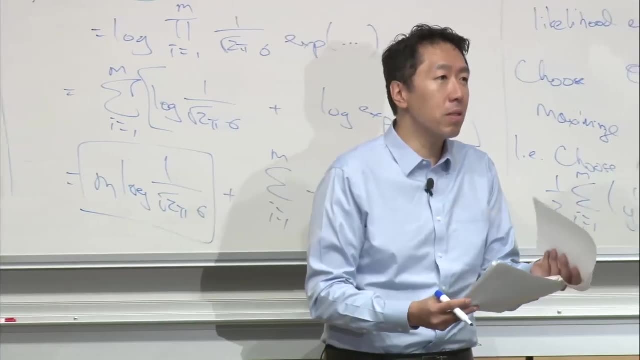 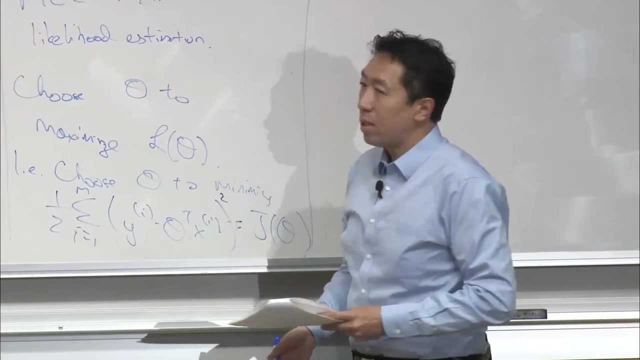 Quite, quite rare. All right, Um, let me think. All right, I want to move on to make sure we get through the rest of things. Any burning questions? Yeah, Okay, cool, All right, Um, so on to this machinery, right? 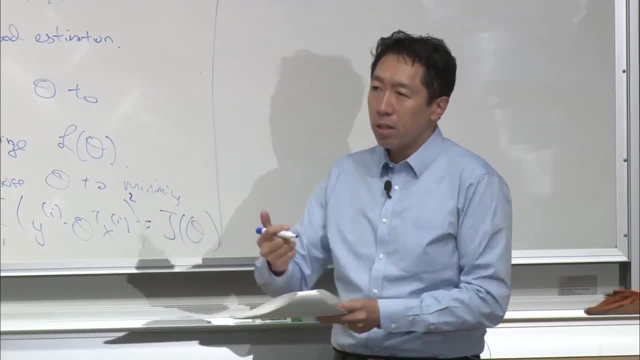 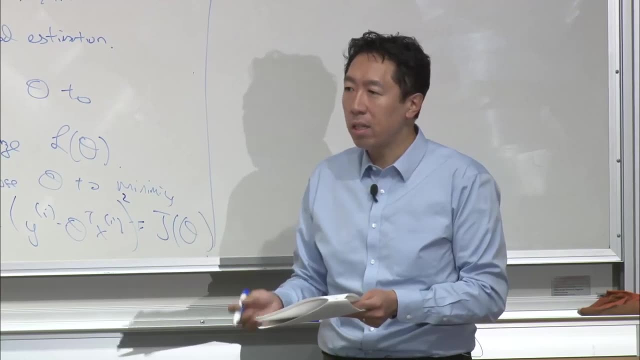 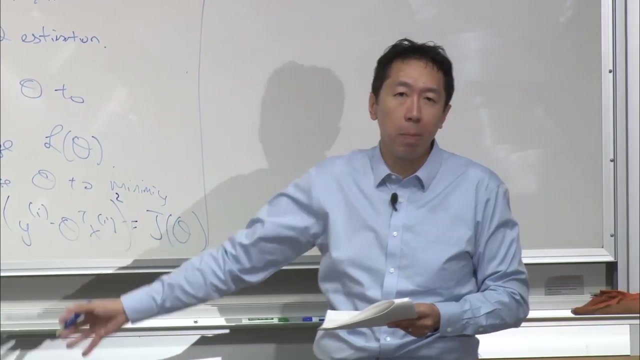 So so. so what did we do here was we set up a set of probabilistic assumptions. We made certain assumptions about p of y, given x right. The key assumption was Gaussian errors in iid, And then, through maximum likelihood estimation, we derived an algorithm which turns out to be exactly the least squares algorithm, right. 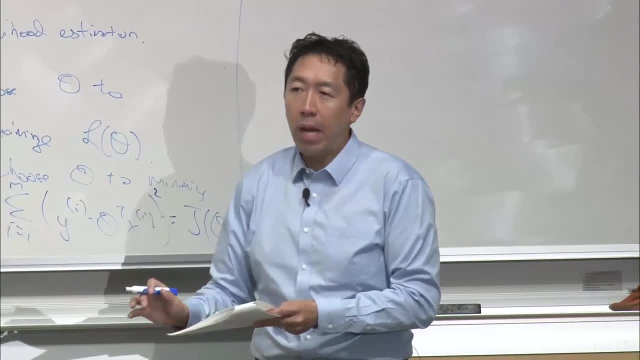 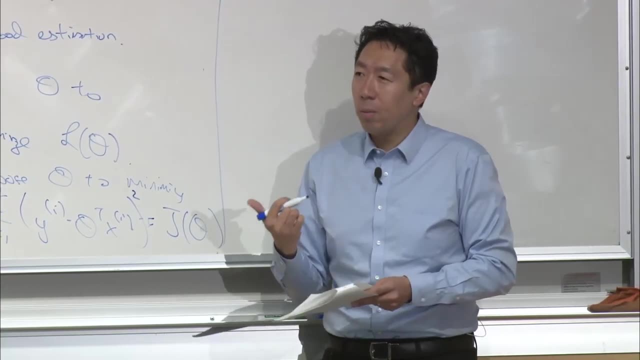 Um, what I'd like to do is take this framework, uh, and apply it to our first classification problem. right, And so the the the key steps are, you know? one make an assumption about p of y given x. 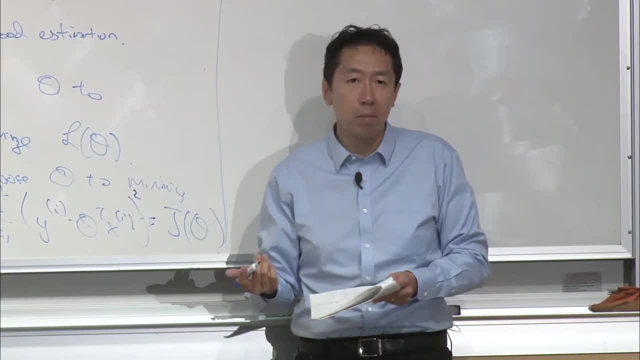 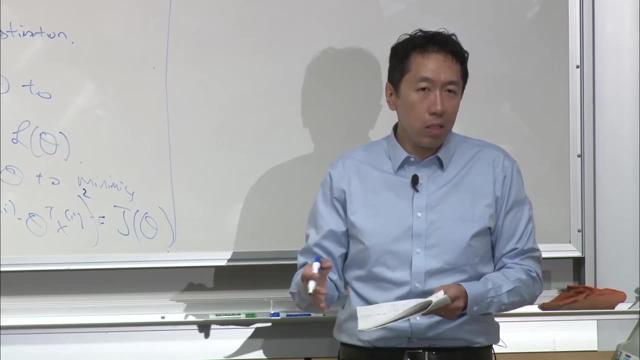 uh p of y given x parameter on this data, And then second is figure out maximum likelihood estimation. So I'd like to take this framework and apply it to a different type of problem where uh, the value of y is now either 0 or 1.. 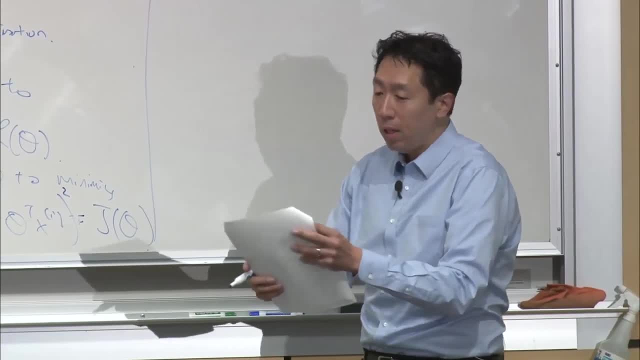 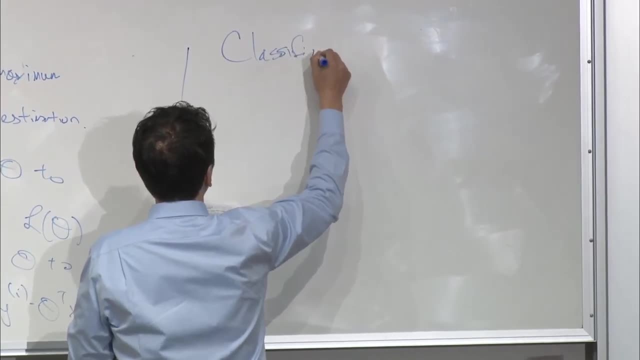 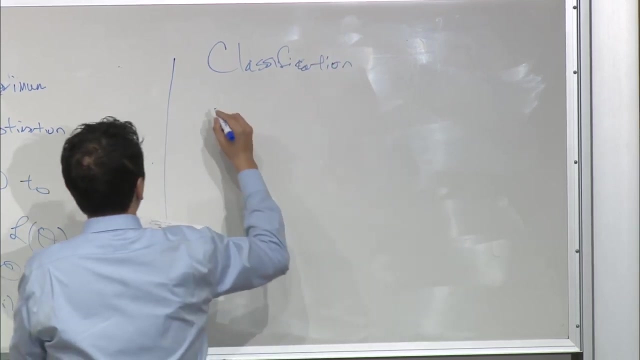 So this is your classification problem, okay, So, um, let's see. So in the classification problem, in our first classification problem, we're going to start with binary classification. So the value of y is either 0 or 1.. 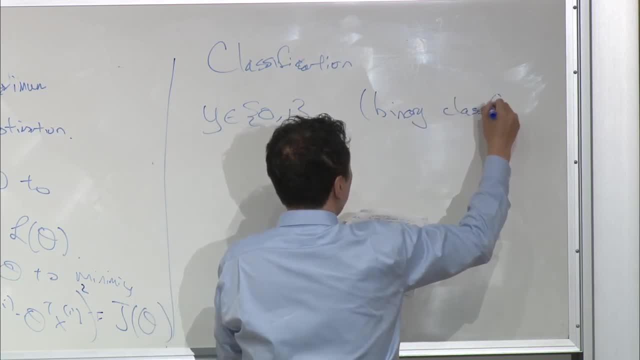 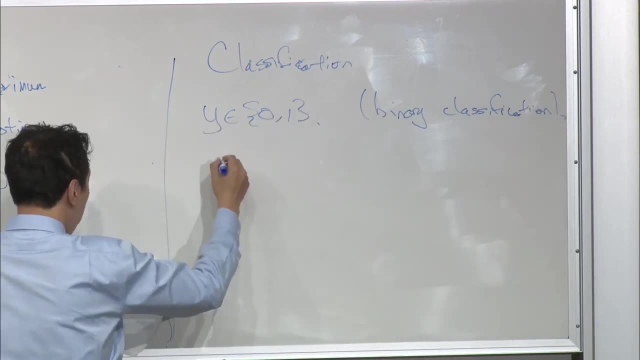 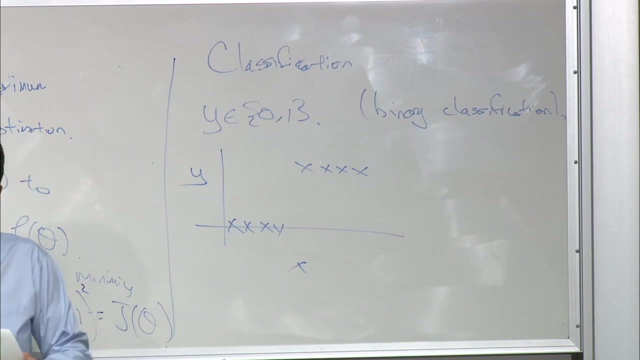 And sometimes we call this binary classification because there are two classes Classification: Right, Um and so right. So that's a dataset where I guess this is x and this is y, Um. so something that's not a good idea is apply linear regression to this dataset. 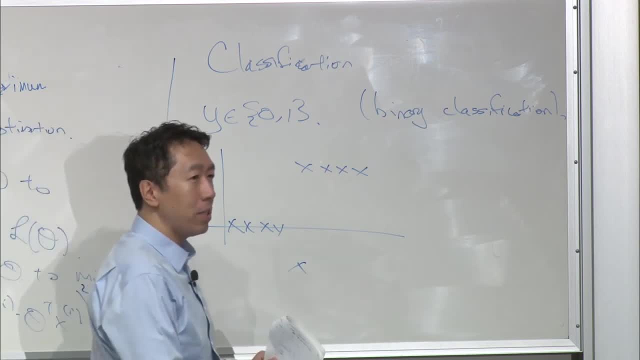 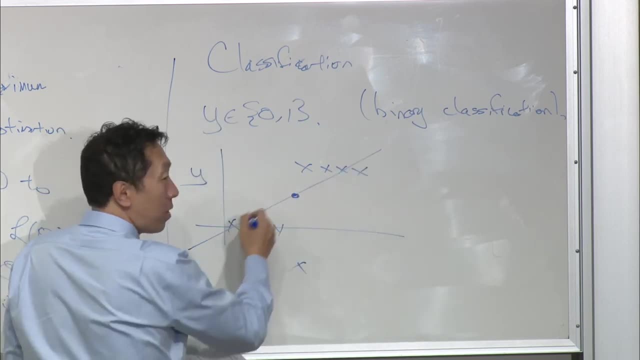 Sometimes. sometimes you will do it and maybe you'll get away with it, but I wouldn't do it. And here's y, which is um. it is tempting to just fill a straight line to this data and then take the straight line and threshold it at 0.5,. 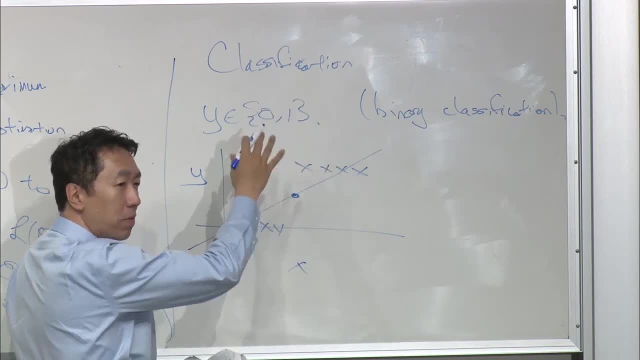 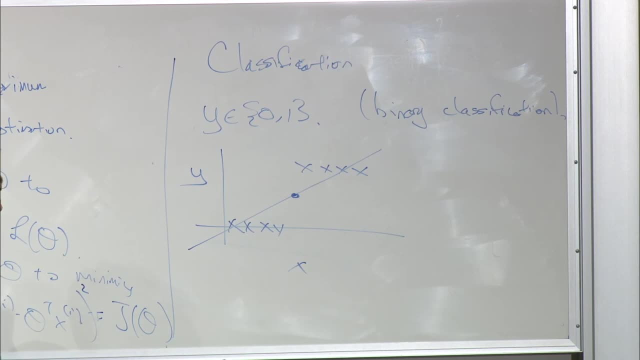 and then say: oh, if it's above 0.5, round off to 1,, if it's below 0.5, round it off to 0.. But it turns out that this um is not a good idea. 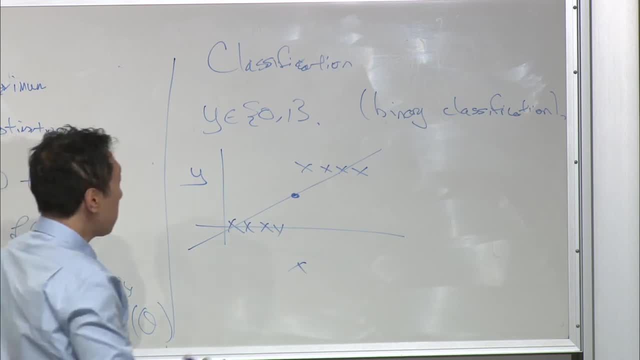 uh, for classification problems. And and here's y, which is for this dataset. it's really obvious what the what, the pattern is right. Everything to the left of this point predict 0, I think, to the right of that point, predict 1.. 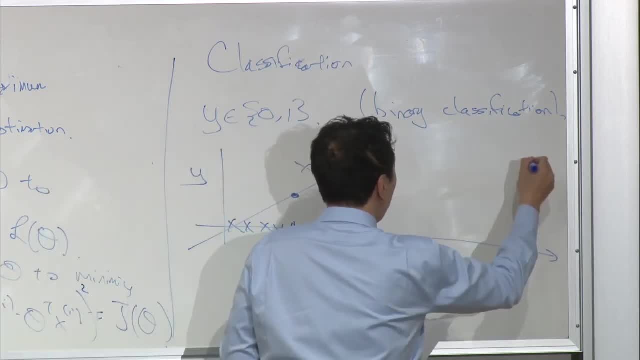 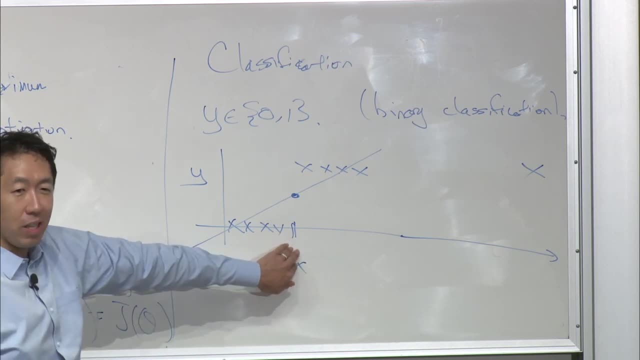 But let's say we now change the dataset to just add one more example there right, And the pattern is still really obvious. It's: everything to the left of this, predict 0, I think, to the right of that, predict 1.. 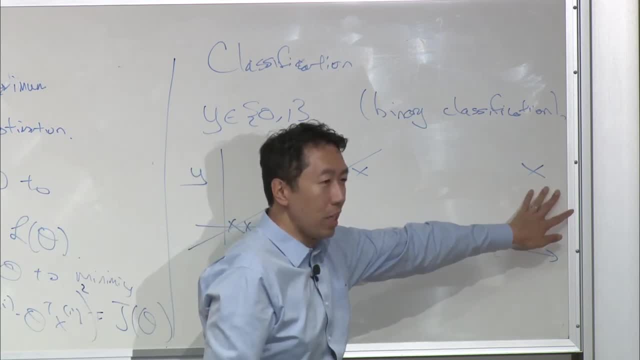 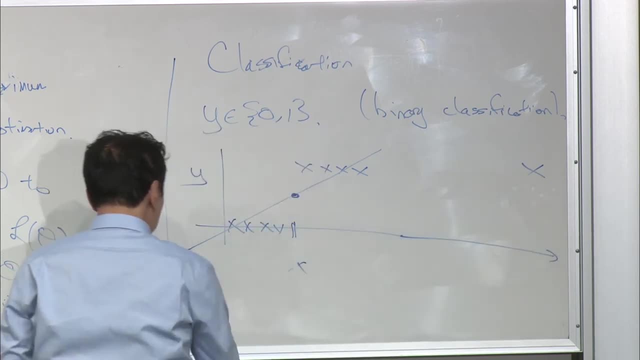 But if you fill a straight line to this dataset with this extra one point there- and this is not even the outlier- it's really obvious that this point way out there should be labeled 1.. But with this extra example, um, if you fit a straight line to the data, 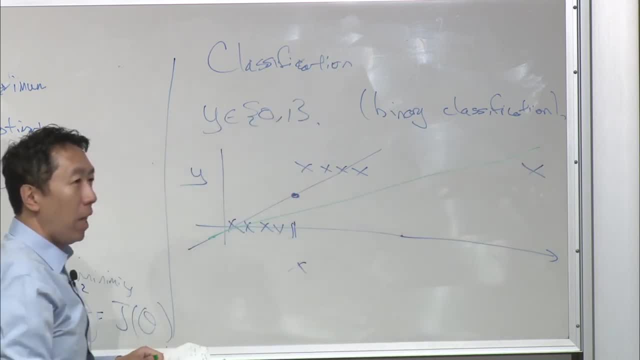 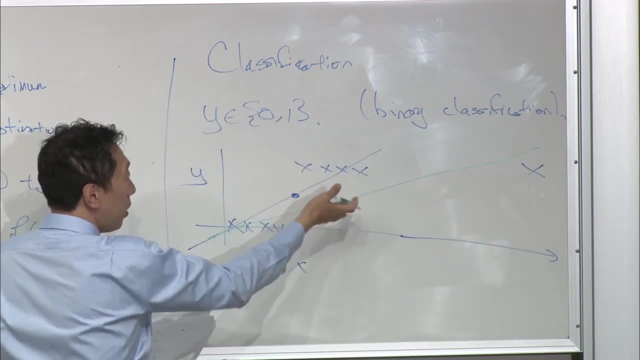 you end up with maybe something like that: Um, and somehow adding this one example. it really didn't change anything, right, But somehow the straight line fit. move from the green line to the uh, move from the blue line to the green line. 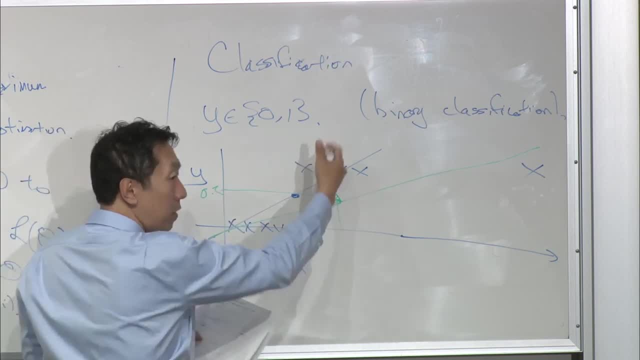 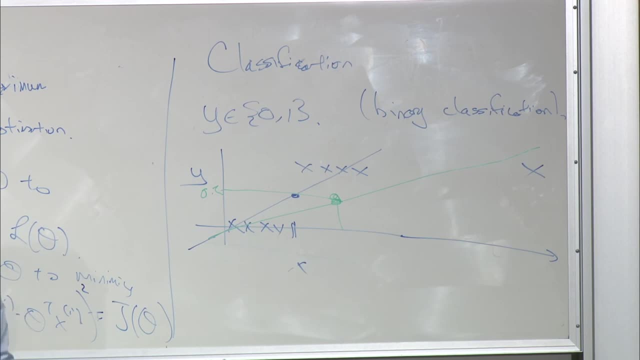 and if you now threshold it at 0.5, you end up with a very different decision, boundary right, And so linear regression is just not a good algorithm for classification. Some people use it and sometimes they get lucky, and it's not too bad. 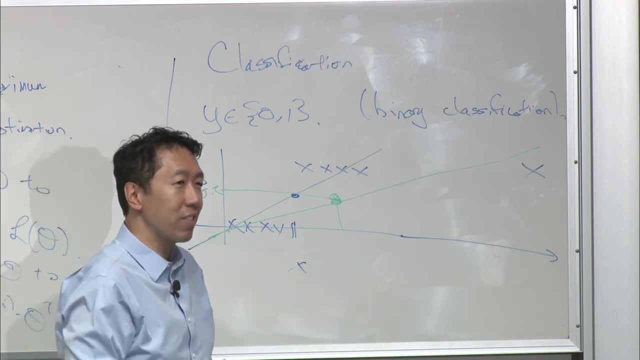 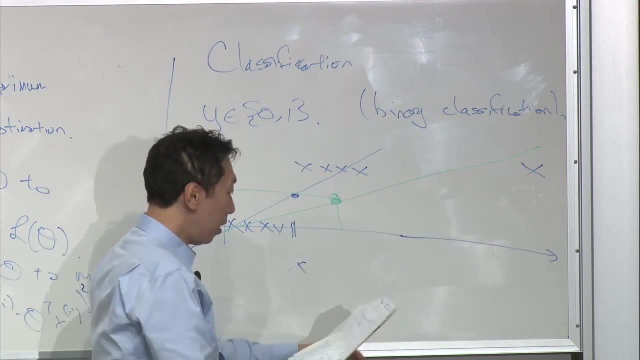 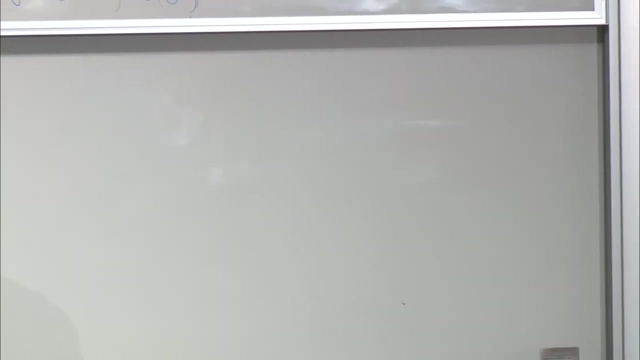 but I, I, I personally never use linear regression for classification algorithms, right? Because you just don't know if you end up with a really bad fit to the data, like this: okay, Um, so, oh, and, and and the other unnatural thing about using linear regression for: 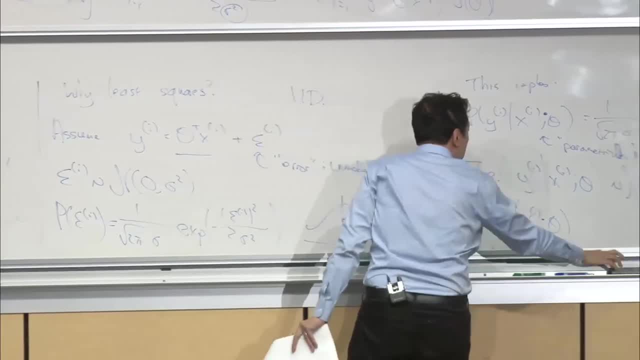 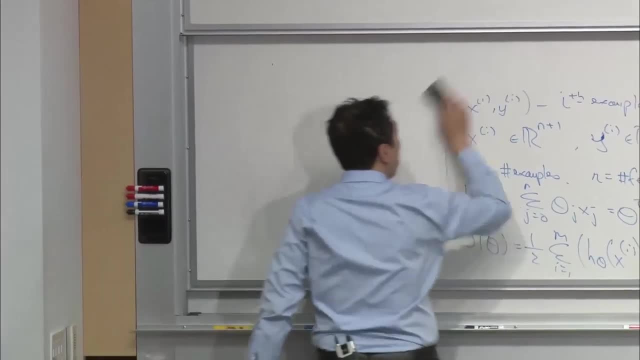 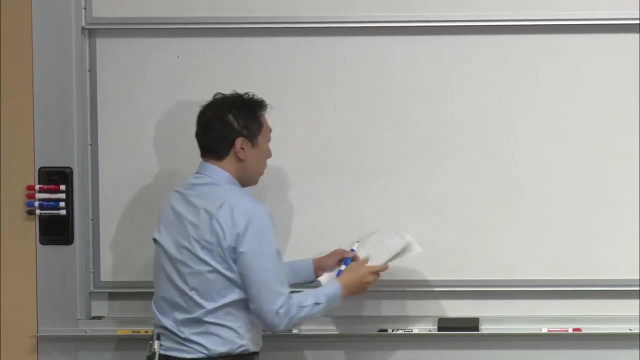 a classification problem is that, um, you know for a classification problem that the values are, you know, 0 or 1, right, And so its output- negative values or values even greater than 1, seems, seems strange. Um, so what I'd like to share with you now is really: 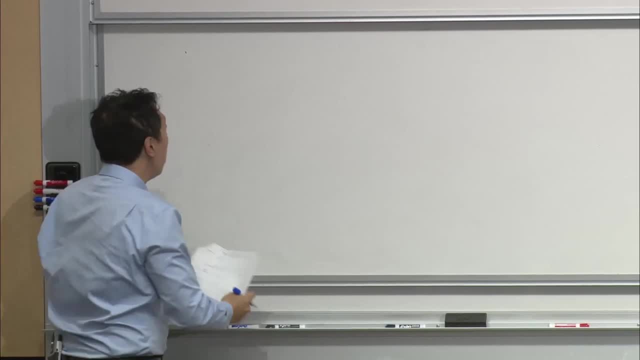 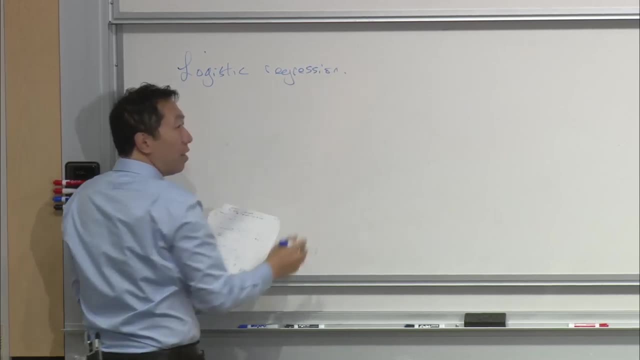 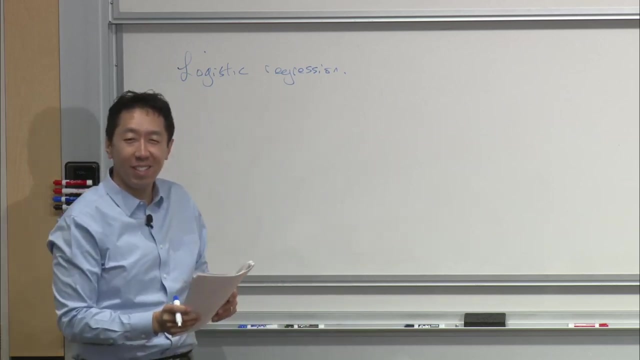 probably by far the most commonly used classification algorithm, uh called logistic regression. I wanna say, the two learning algorithms I probably use the most often are linear regression and logistic regression. Yeah, probably, probably, that's true. yeah, right, Um and uh, this is the algorithm. 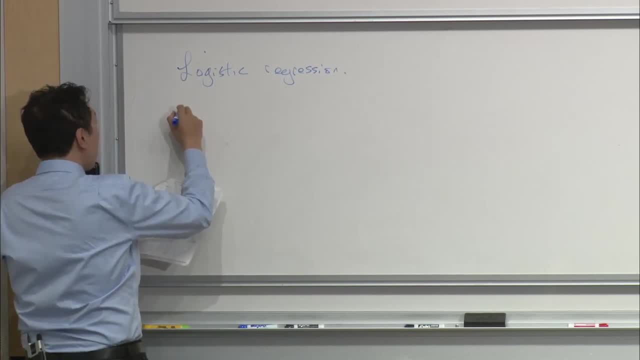 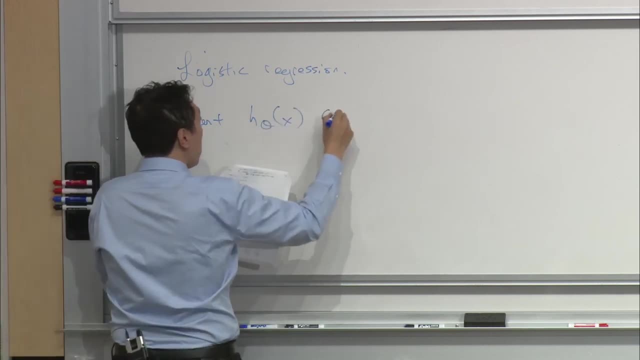 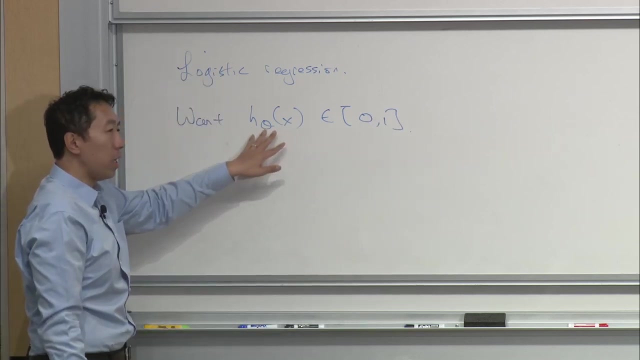 So, um, as, as we designed the logistic regression algorithm, one of the things we might naturally want is for the hypothesis to uh output values between 0 and 1, right, And this is mathematical notation for the values for h of x or h prime. 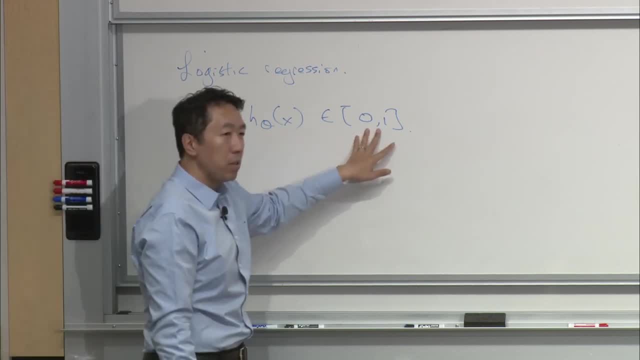 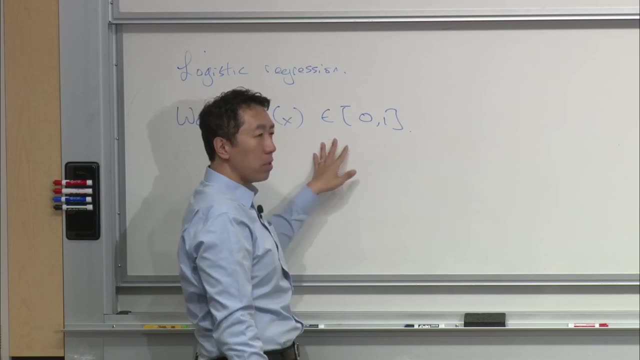 you know, h subscript. Theta of x, uh lies in the set from 0 to 1, right The 0 to 1 square bracket is a set of all real numbers from 0 to 1.. So this says we want the hypothesis output values in. 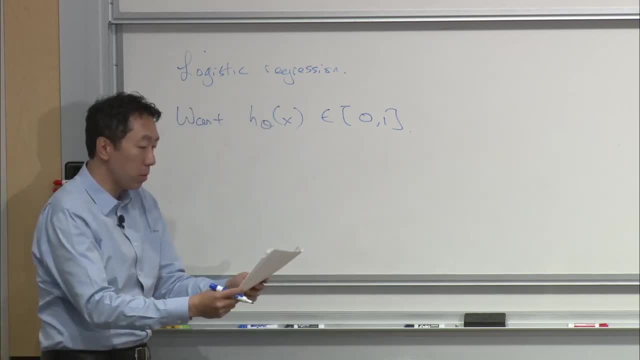 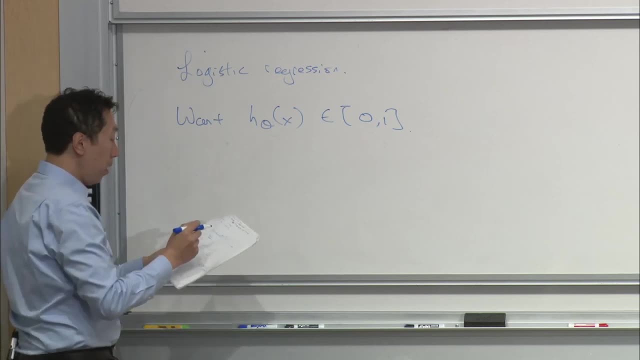 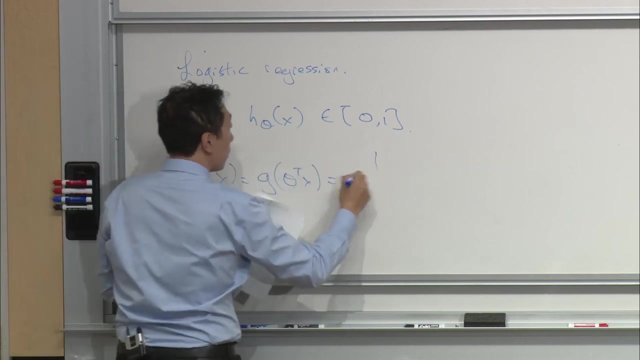 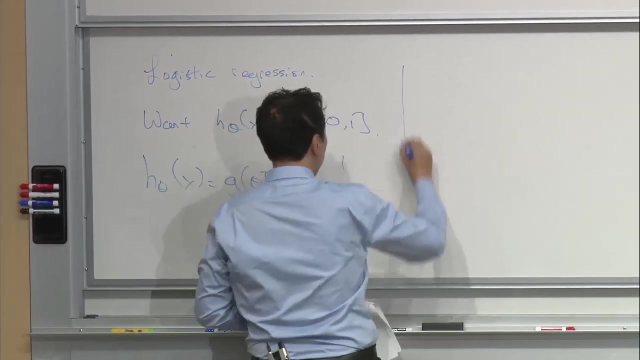 you know, between 0 and 1, so in, in the set of all numbers, which is from 0 to 1.. Um, and so we're going to choose the following form of the hypothesis: Um. so so I'm going to define a function g of z that looks like this: 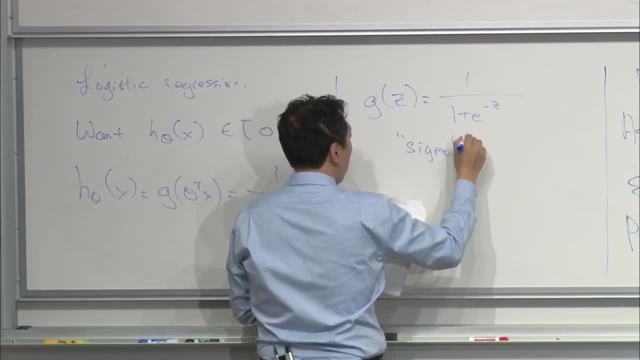 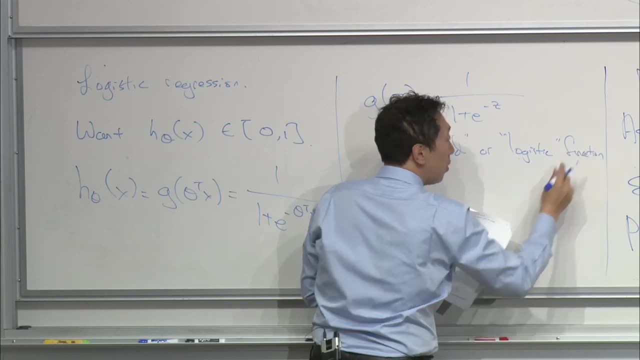 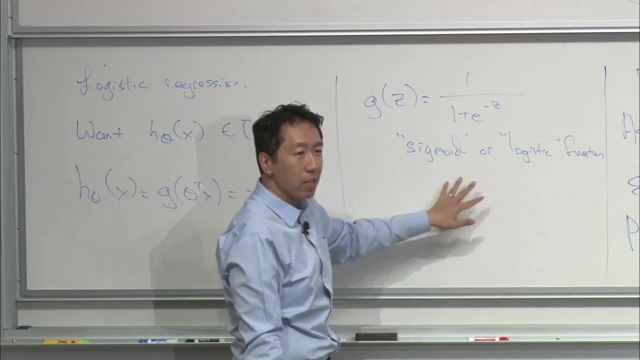 And this is called the sigmoid, uh or the logistic Function, Uh, these are synonyms, they mean exactly the same thing. So, uh, it can be called the sigmoid function or the logistic function. it means exactly the same thing. 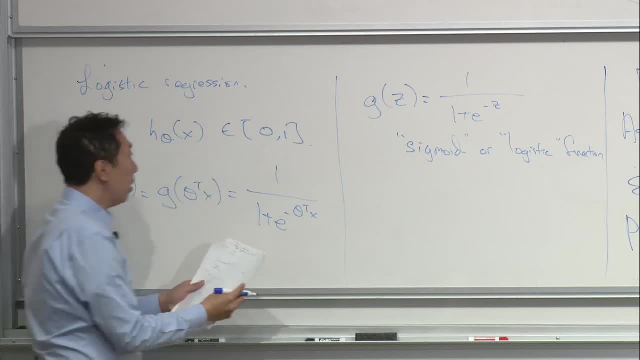 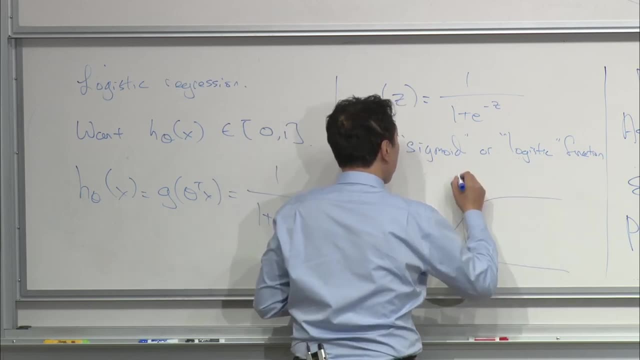 But I'm gonna choose a function g of z, um, and this function is shaped as follows: If you plot this function, you find that it looks like this: um, where if the horizontal axis is z, then this is g of z. 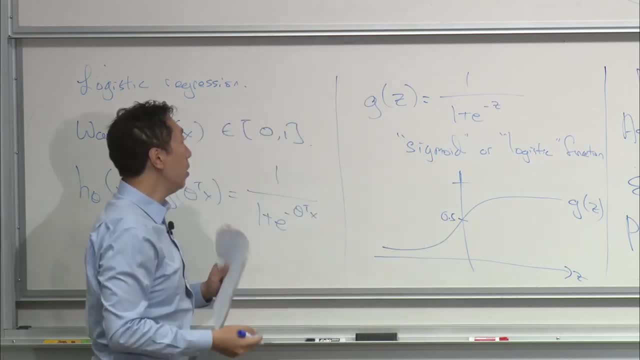 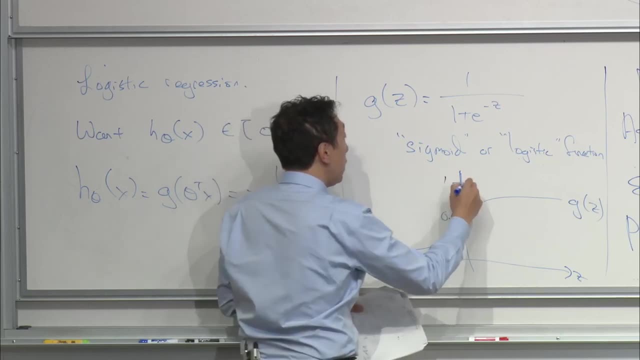 and so it crosses x intercept at 0.. Um, and it, you know, starts off well, really really close to 0, rises, and then asymptotes towards 1, okay, And so g of z outputs values. uh. 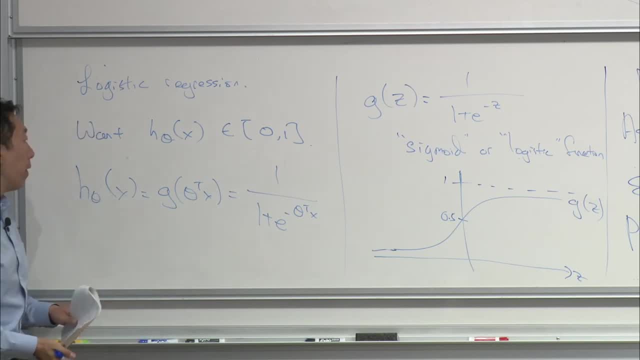 between 0 and 1.. And um, what logistic regression does is instead of- let's see So previously for linear regression, we had chosen this form for the hypothesis right. We just made a choice that we'll say that housing prices are. 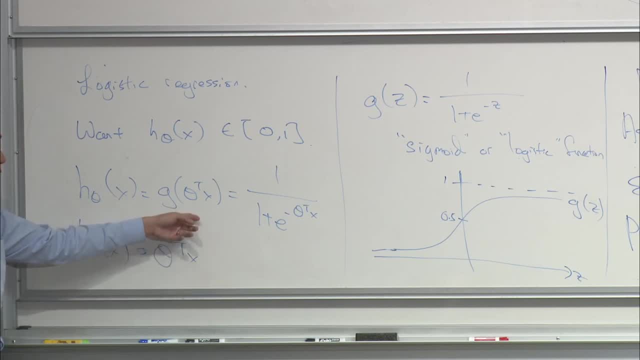 a linear function of the features x. And what logistic regression does is theta transpose x could be bigger than 1, it could be less than 0, which is not very natural, but instead it's gonna take theta transpose x and pass it through this sigmoid function g. 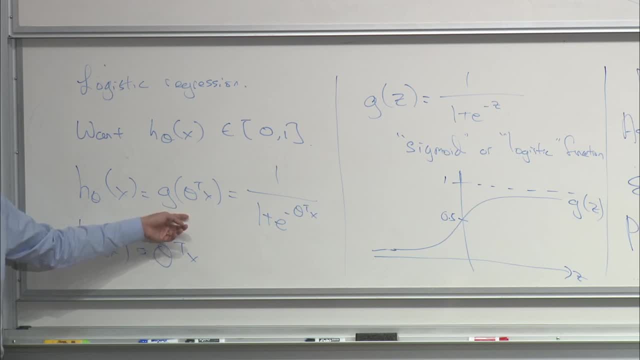 so that it's forced to output values only between 0 and 1, okay, Um, so you know, when designing a learning algorithm, uh, sometimes you just have to choose the form of the hypothesis. How are you gonna represent the function h or h of h? subscript theta. 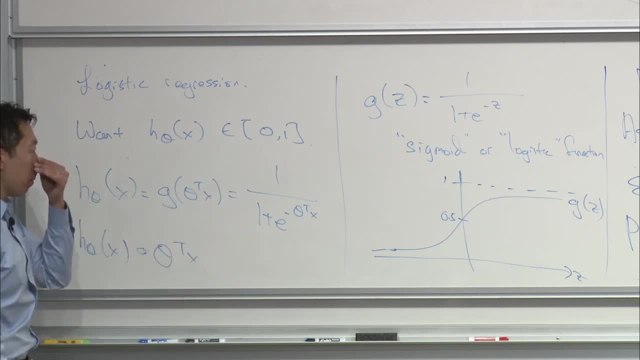 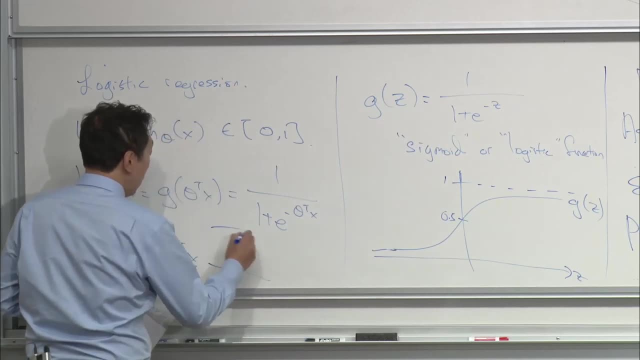 And so we're making that choice here today. And if you're wondering, you know there are lots of functions that we could have chosen right. There are lots of- why- why not, uh, uh, why not this function, or why not, you know? 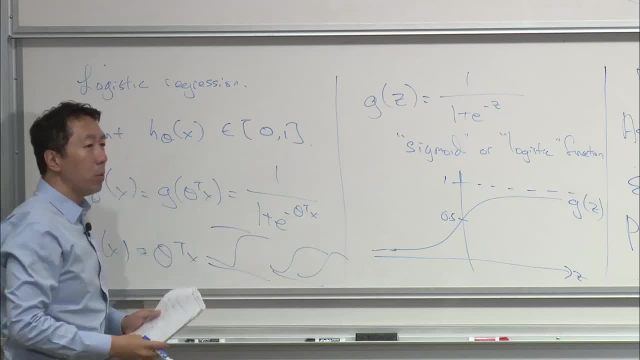 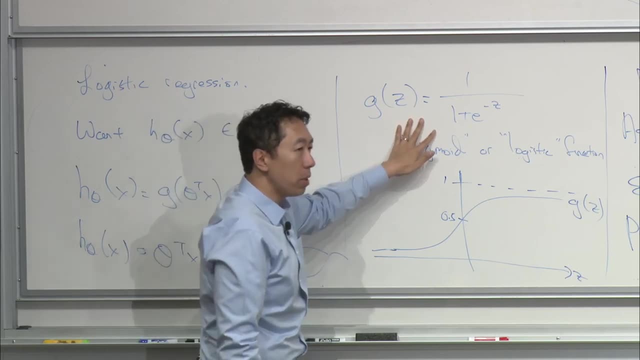 there are lots of functions with vaguely this shape that go between 0 and 1.. So why are we choosing this specifically? It turns out that there's a broader class of algorithms called generalized linear models- You hear about them Wednesday, uh- of which this is a special. 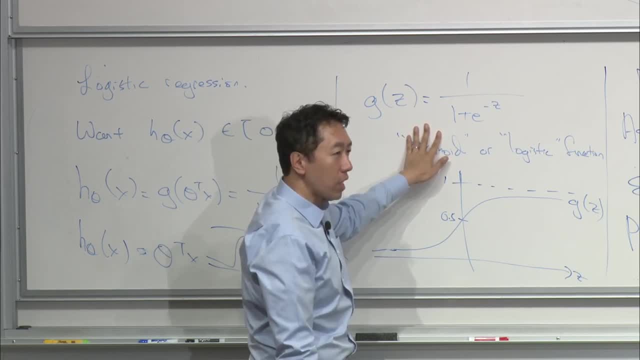 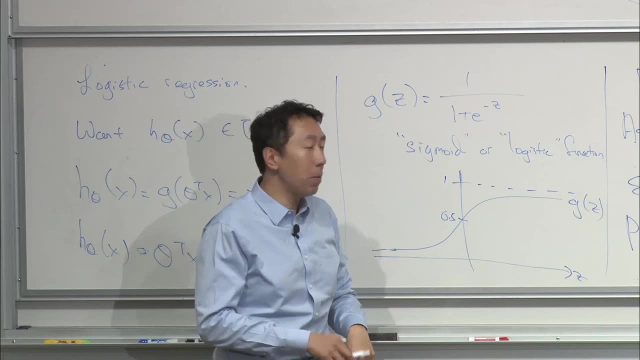 So we've seen linear regression, you see logistic regression in a second, And on Wednesday you see that both of these examples of a much bigger set of algorithms derive using a broader set of principles. So- so for now, just you know. 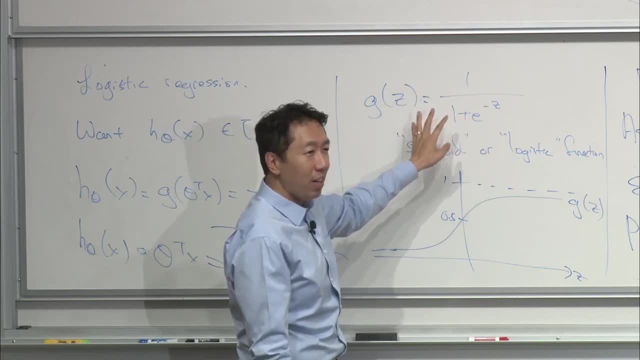 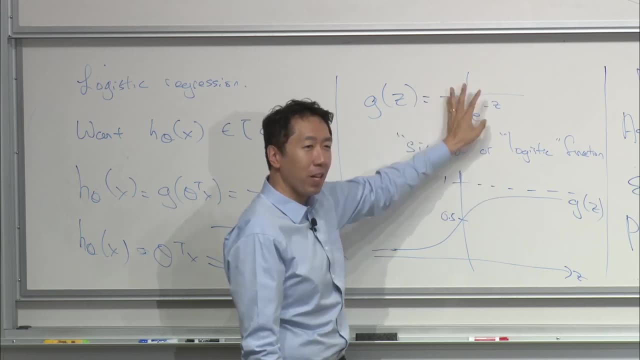 take my word for it that- that we want to use the logistic function. Uh, uh, it'll turn out, you see, on Wednesday, that there's a way to derive even this function from, um, uh, from more basic principles, rather than just putting on this- this hat. 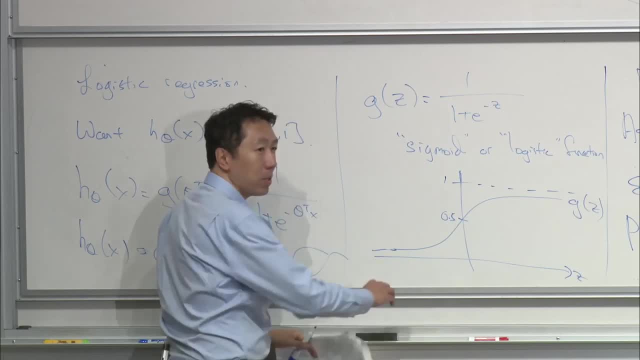 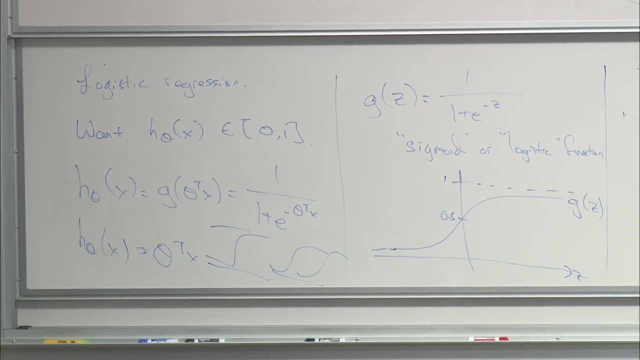 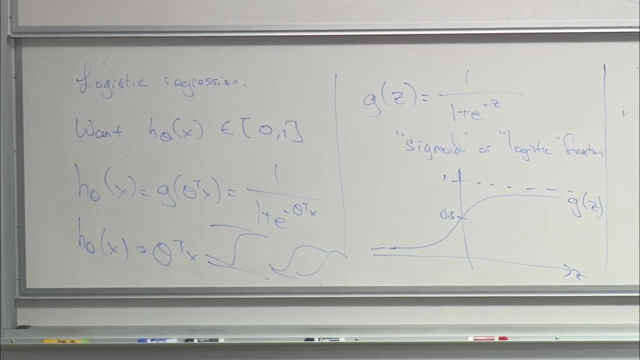 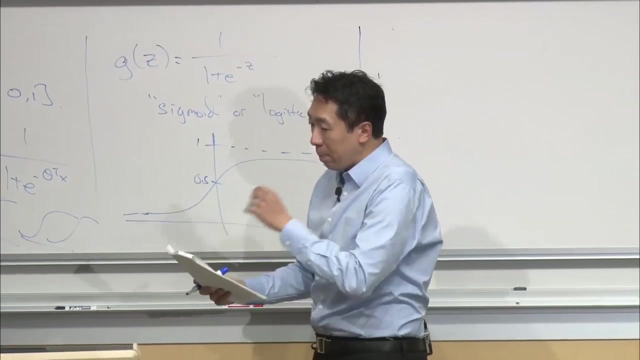 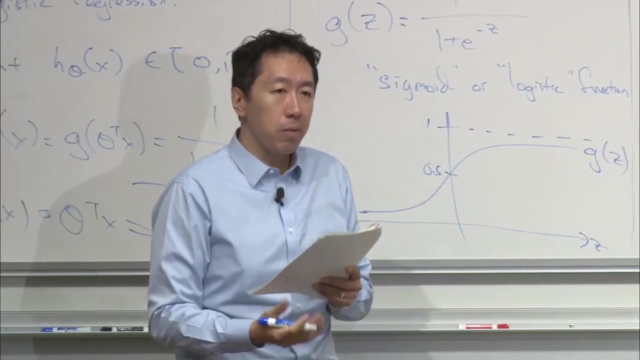 But for now, let- let me just pull this out of the hat and say that's the one we want to use. Okay, So, um, let's make some assumptions about the distribution of y given x parameterized by Theta. So I'm going to assume: 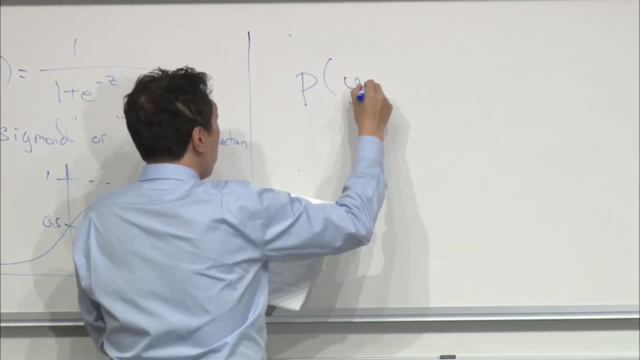 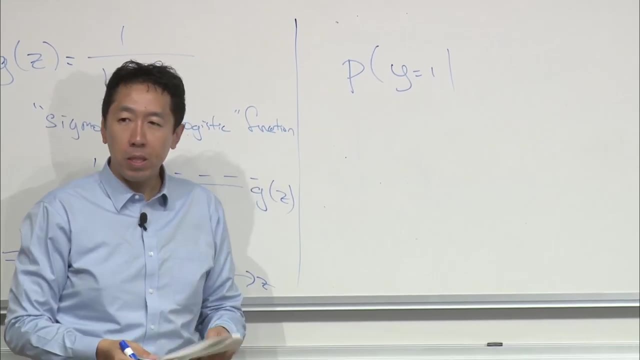 um that the data has the following distribution, The probability of y being 1,. uh, again, from the breast cancer prediction that we had from uh, the first lecture, right, It would be the chance of a tumor being cancerous or being. 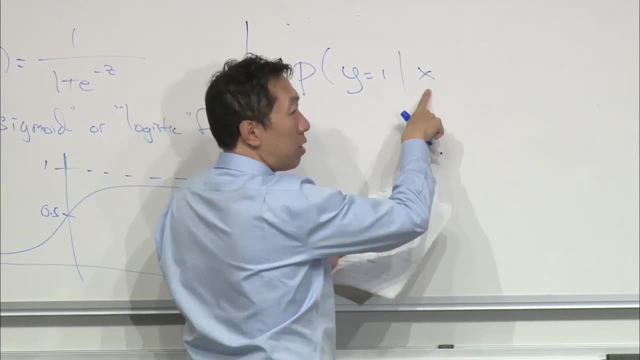 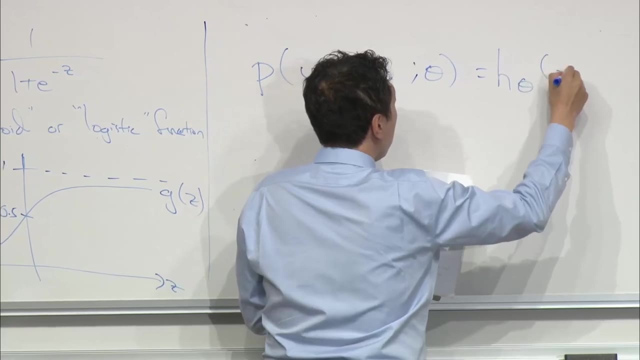 um uh, malignant chance of y being: 1. Given the size of a tumor- that's a feature x parameterized by Theta, that this is equal to the output of your hypothesis. Okay, So in other words, we're gonna assume that. 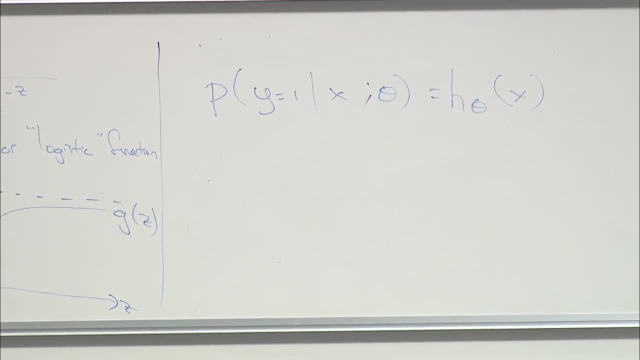 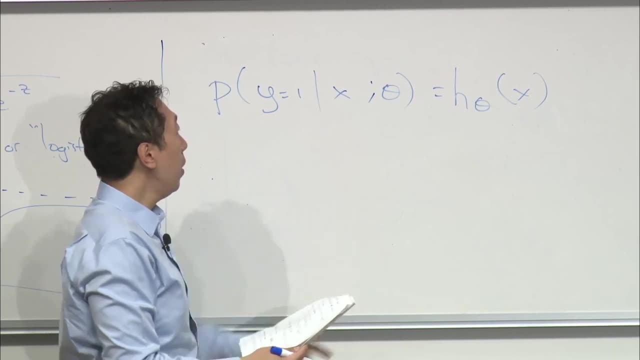 um, what you want your learning algorithm to do is input the features and tell me what's the chance that this tumor is malignant, right? What's the chance that y is equal to 1?? Um, and by logic, I guess, because y can be only 1 or 0,. 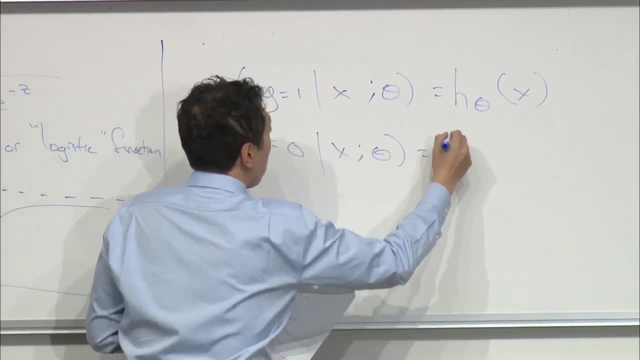 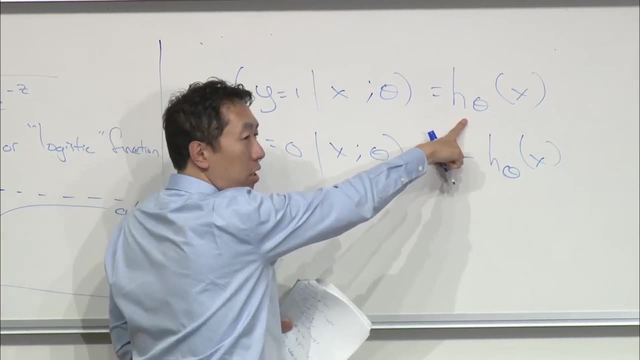 the chance of y being equal to 0, this has got to be 1 minus that, right, Because if a tumor has a 10 percent chance of uh being malignant, that means it has a 1 minus that. It means it must have a 90 percent chance of being benign, right. 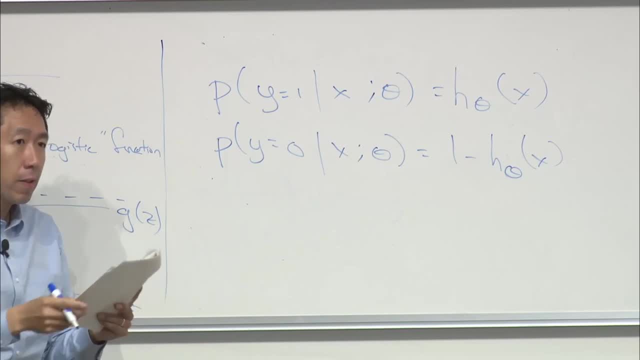 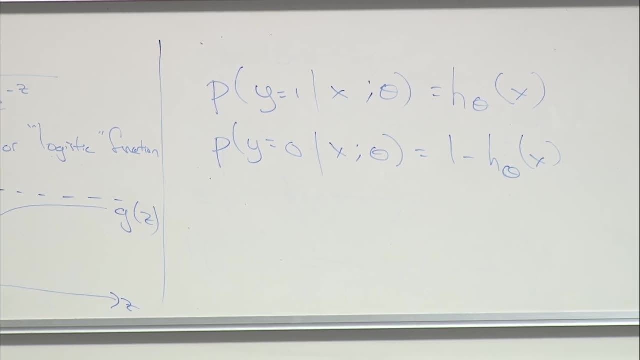 Since these two probabilities must add up to 1.. Okay, Yeah, Say that again. Oh, can we change the probability? Yes, you can, but I'm not. yeah, But I think just to stick with convention in the other direction. 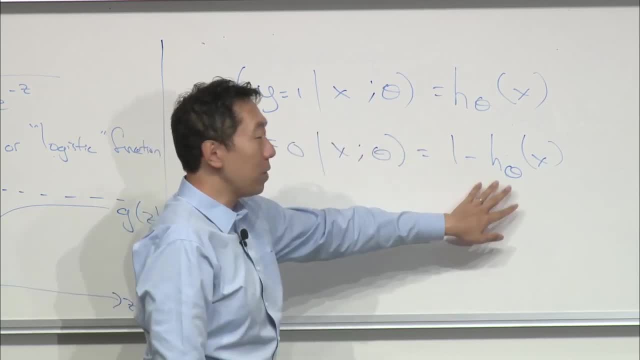 you, you, yeah sure, We could assume that P of y equals 1 was this and P of y equals 1 was that, but I think, either way, it's just what you call a positive example, what you call a negative example, right. 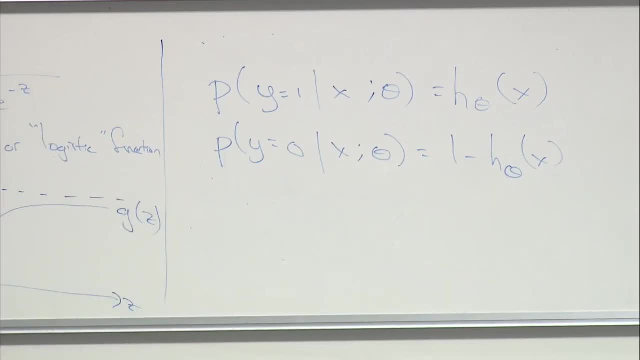 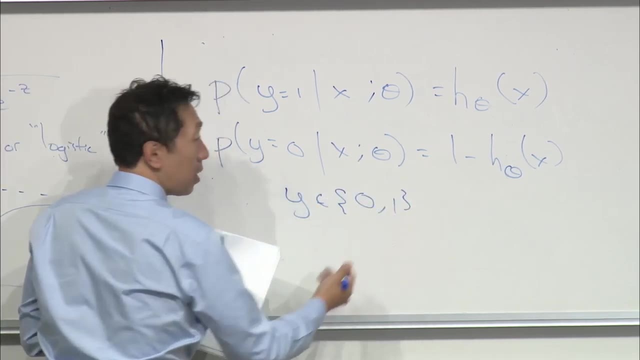 So, so I wanna use this convention, okay, Um, and now, bearing in mind that y right by definition, because it's a binary classification problem, but bearing in mind that y can only take on two values: 0 or 1,. 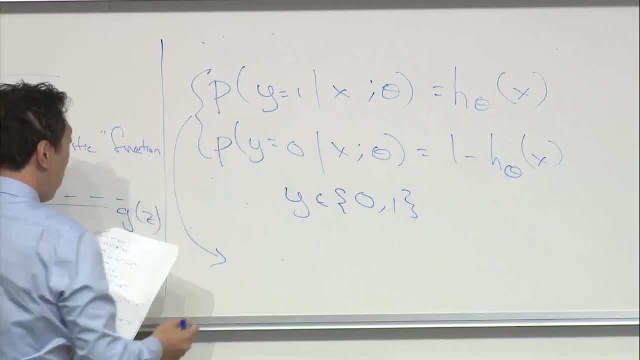 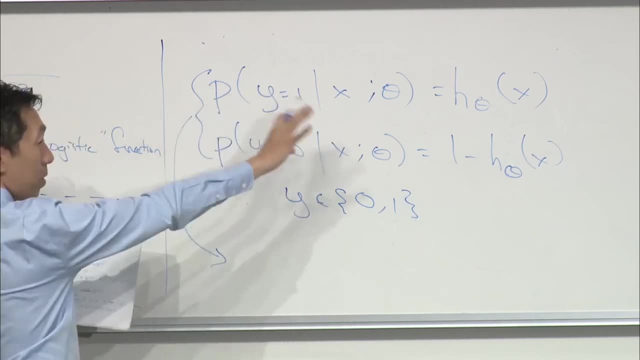 um, there's a nifty sort of a little algebra way to take these two equations and write them in one equation, And this will make some of the math a little bit easier. We're gonna take these two equations, take these two assumptions. 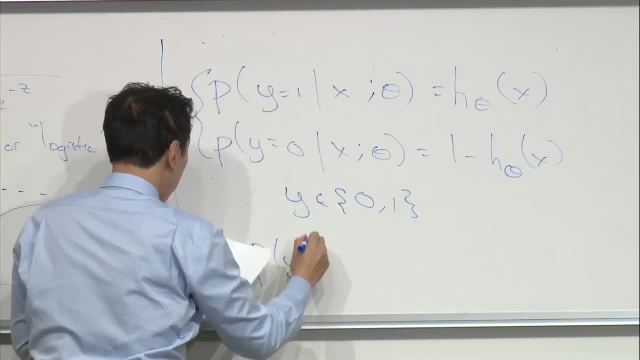 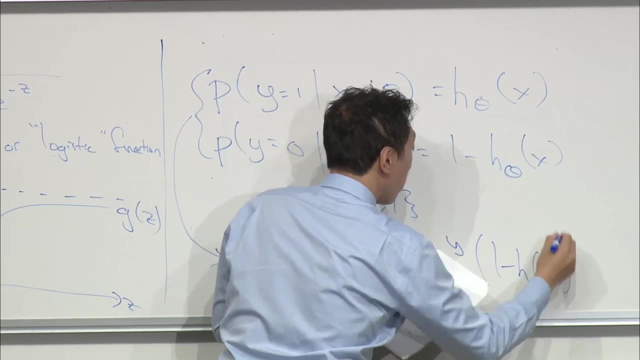 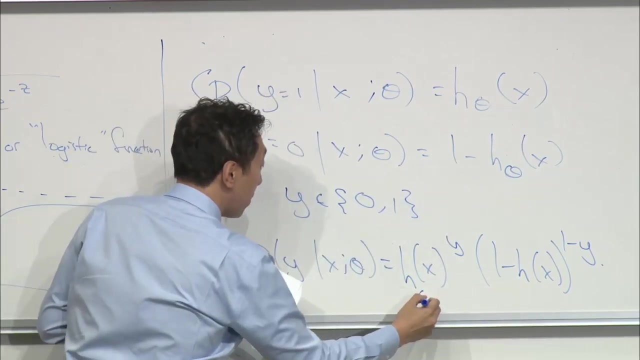 or take these two facts and compress it into one equation, which is this: okay, Oh, and I dropped the Theta subscript just to simplify the notation a bit. right, I'm, I'm gonna be a little bit sloppy sometimes. Well, a little less formal, whether I write the Theta there or not. 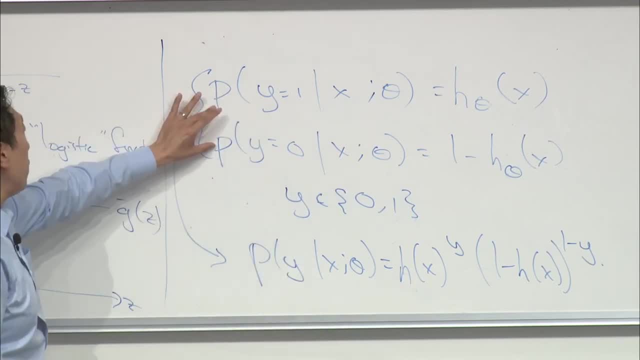 Okay, Um, but these two definitions of p, of y, given x parameterized by Theta- bearing in mind that y is either 0 or 1, can be compressed into one equation like this: Uh, and, and let me just say y, right. 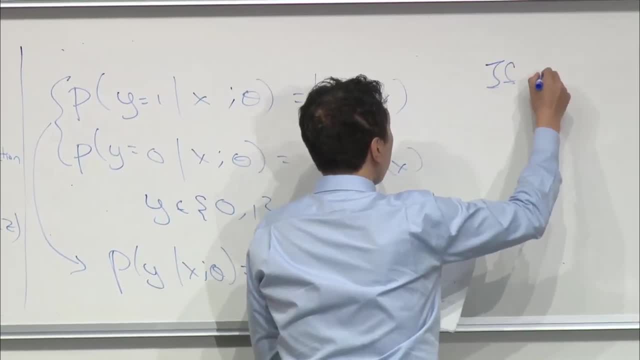 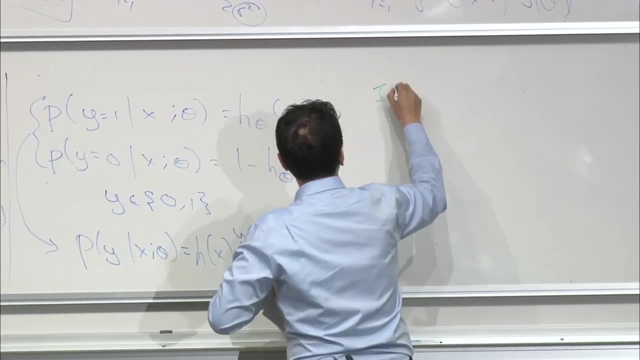 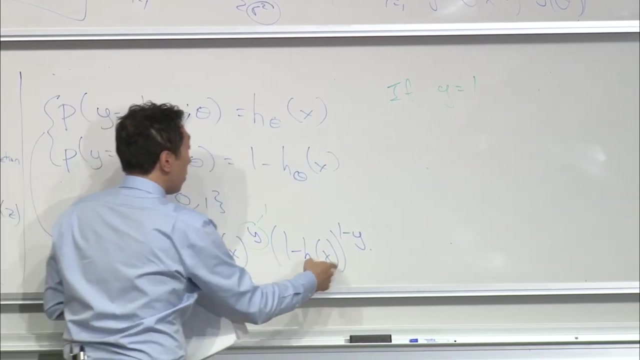 It's because if y it's a different color, all right. If y is equal to 1, then this becomes h of x to the power of 1, times this thing to the power of 0, right, If y is equal to 1,. 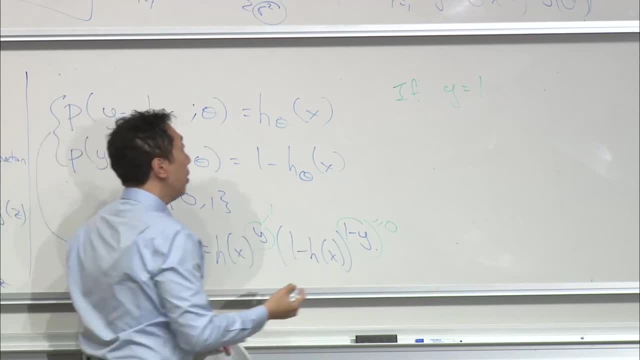 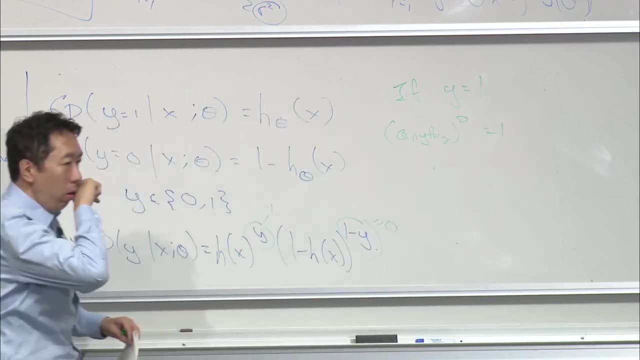 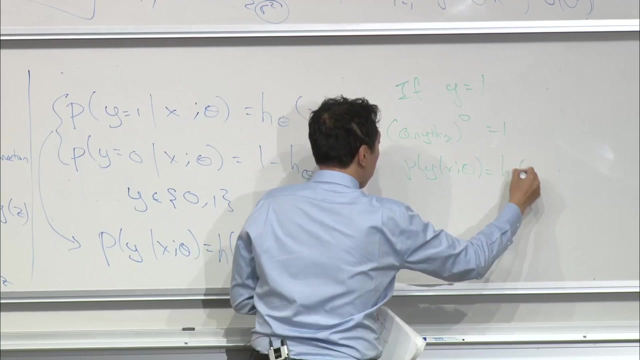 then um 1 minus y is 0. And you know, anything to the power of 0 is just equal to 1.. And so if y is equal to 1, you end up with p of y, given x parameterized by Theta equals h of x, right. 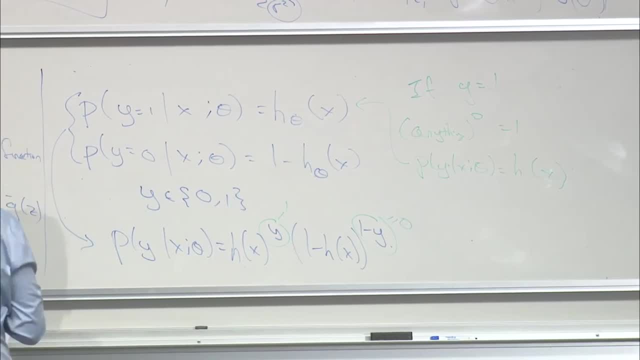 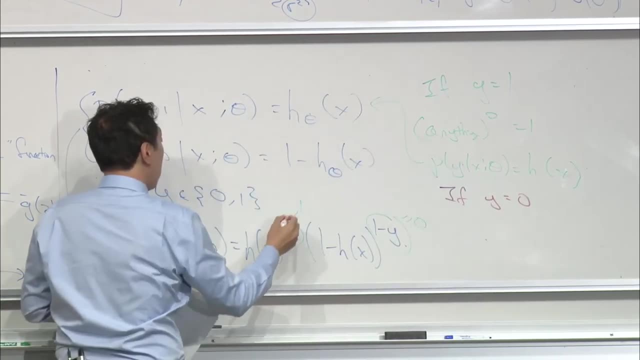 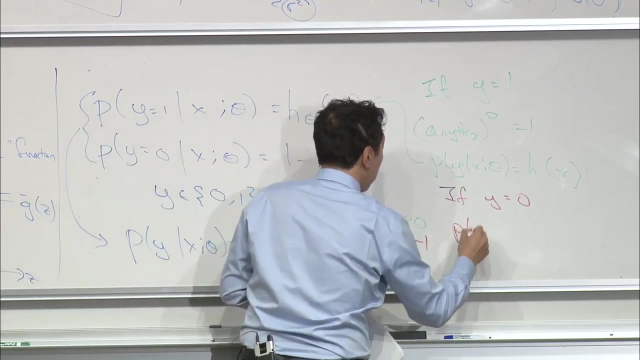 Which is just what we had there. And conversely, if y is equal to 0, then um, this thing would be 0, and this thing would be 1.. And so you end up with p of y, given x, parameterized Theta is equal to 1 minus h of x. 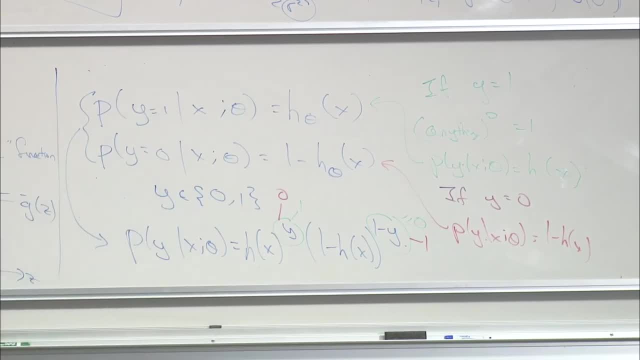 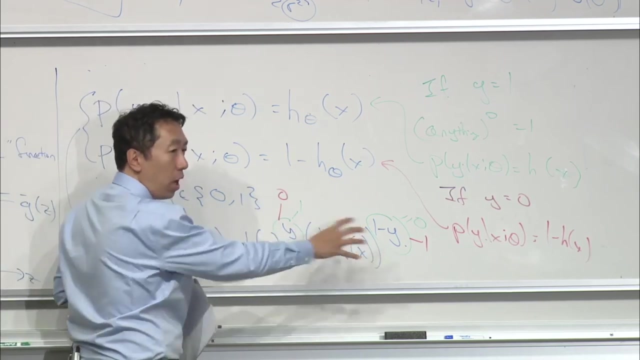 which is just equal to that second equation. Okay, Right, Um, and so this is a nifty way to take these two equations and compress them into one line, Because, depending on whether y is 0 or 1, one of these two terms switches off because it's. 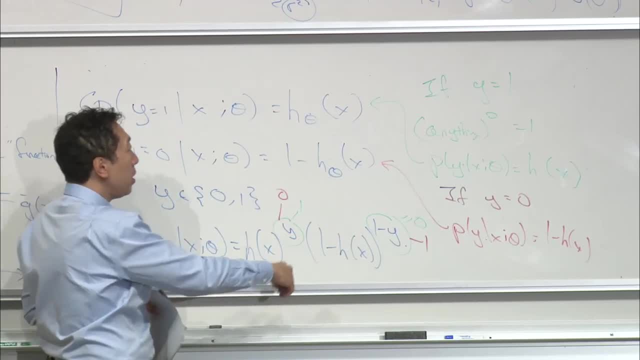 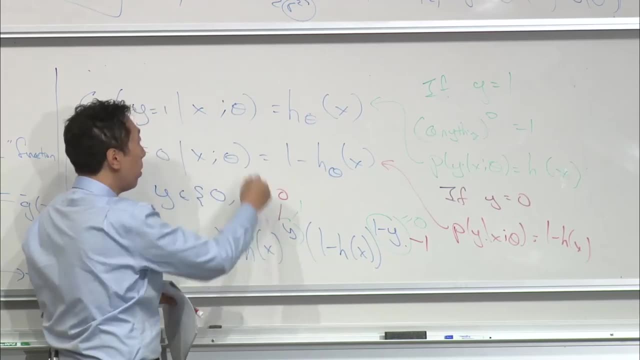 exponentiated to the power of 0, um, and anything to the power of 0 is just equal to 1, right? So one of these terms is just, you know, 1.. Uh, thus leaving the other term, and thus: 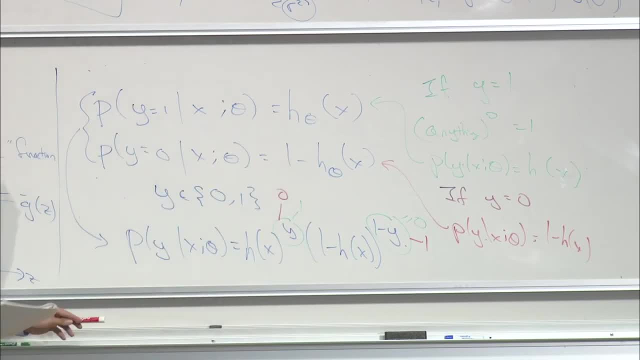 selecting the- the appropriate equation, depending on whether y is 0 or 1, okay, So with that, um, uh, so with this little- uh, I don't know- notational trick, I'll make the Theta derivation. It's simpler, Okay. 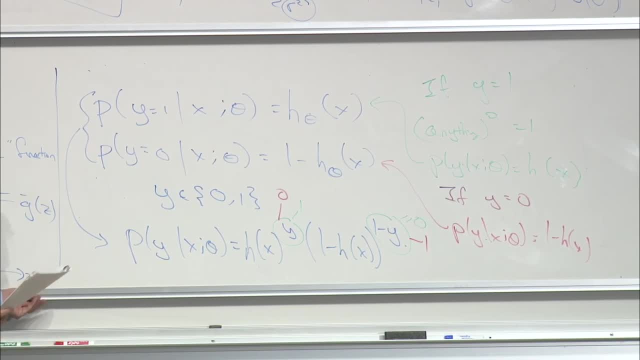 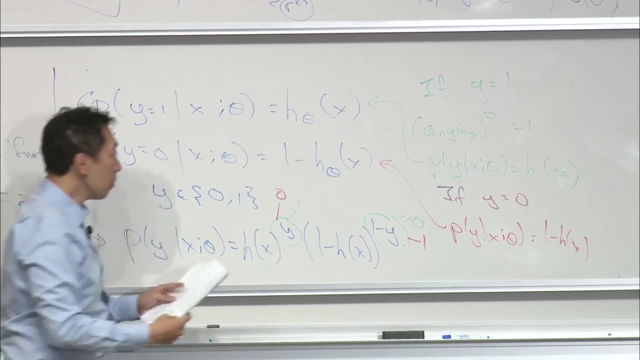 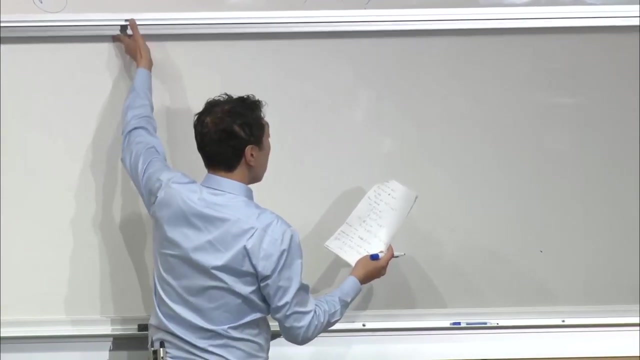 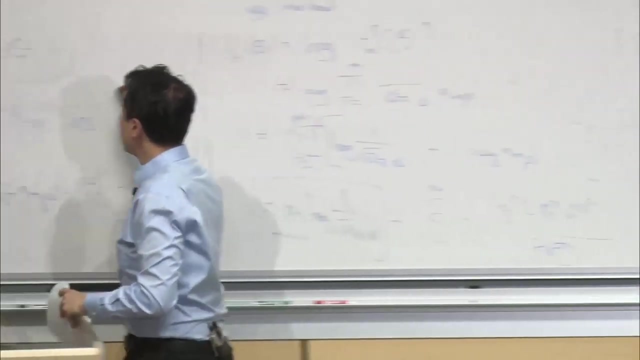 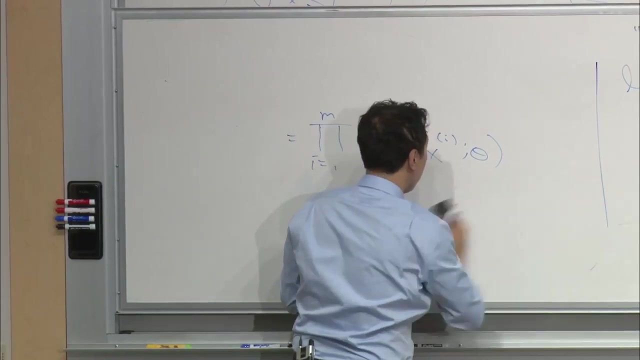 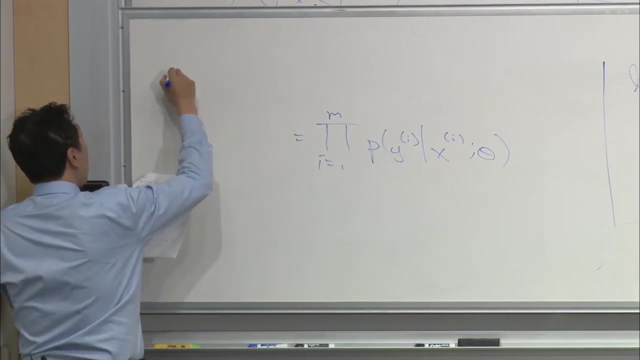 Um, yeah, So Let me use the new board. I want that. Oh, All right. Actually, I can reuse a lot of this, All right. So, uh, we're gonna use maximum likelihood estimation again, So let's write down the likelihood of the parameters. 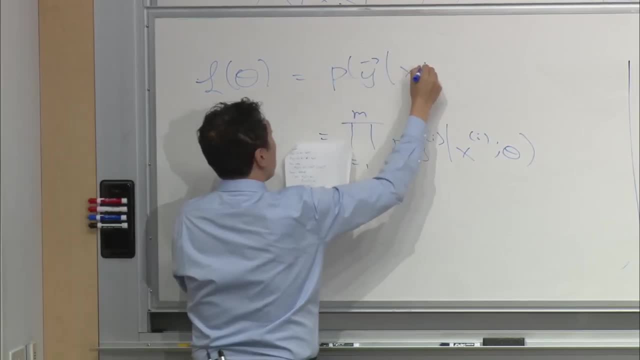 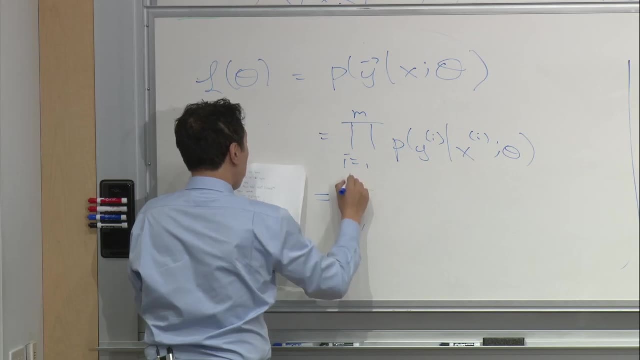 Um, so, oh well, it's actually p of all the y's, given all the x's parameterized by Theta, which is equal to this uh, which is now equal to product from. i equals 1 through m, h of x, i. 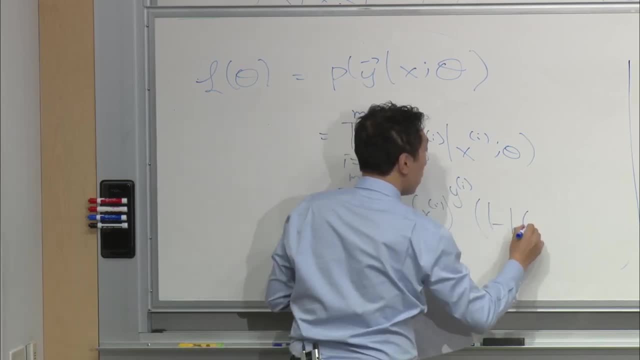 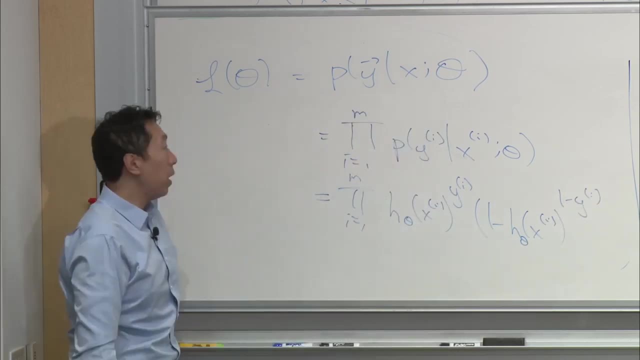 to the power of y i times 1 minus h of x i to the power of 1 minus y i. okay, Where, uh, all I did was take this definition of p of y given x parameterized by Theta. uh, you know from that. 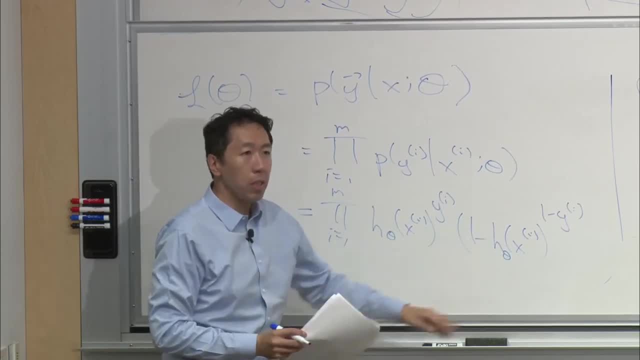 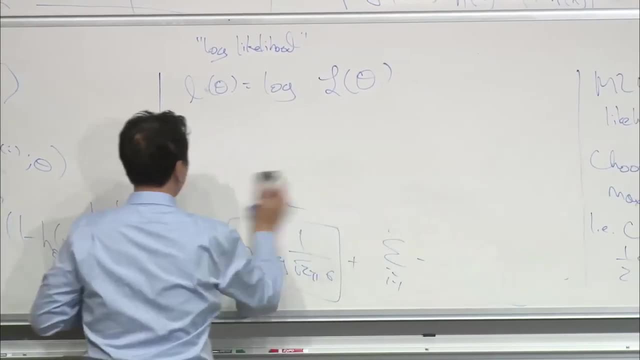 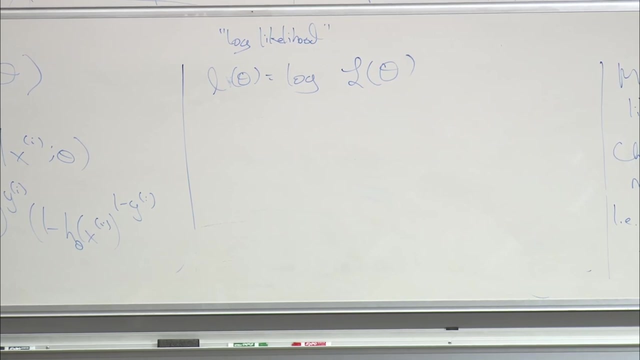 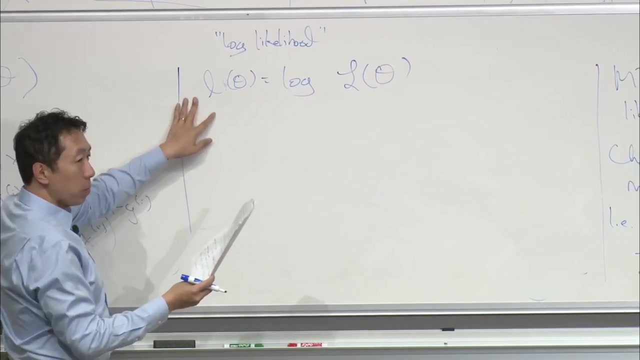 after we did that little exponentiation trick and wrote it in here, right, Um, and then, uh, with maximum likelihood estimation, we'll want to find the value of Theta that maximizes the likelihood, maximize the likelihood of the parameters, And so um, same as what we did for linear regression. 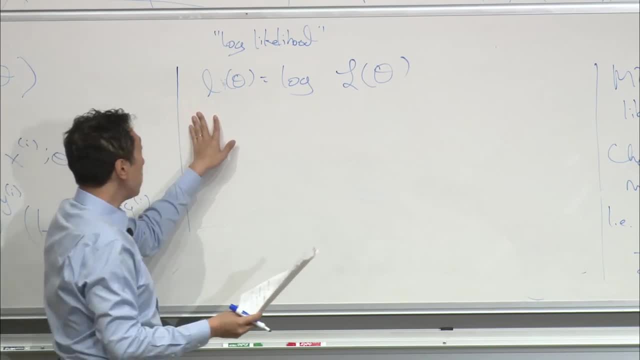 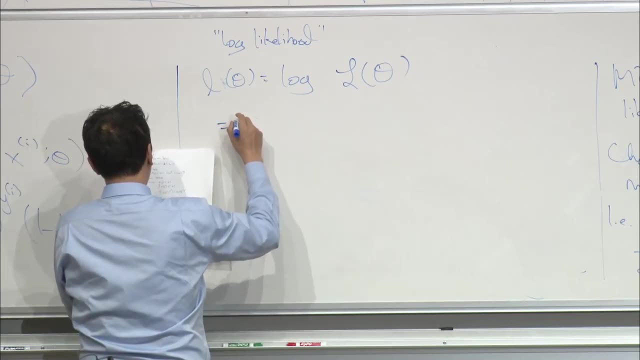 to make the algebra you know to. to make the algebra a bit more simple, we're going to take the log of the likelihood and so compute the log likelihood, And so that's equal to um. let's see, right. 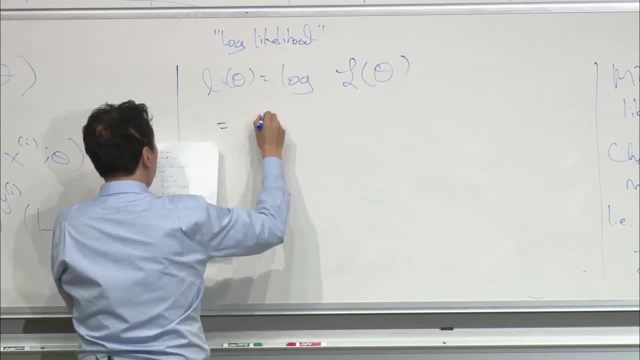 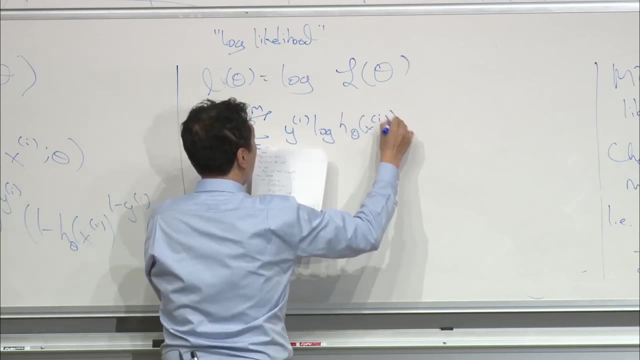 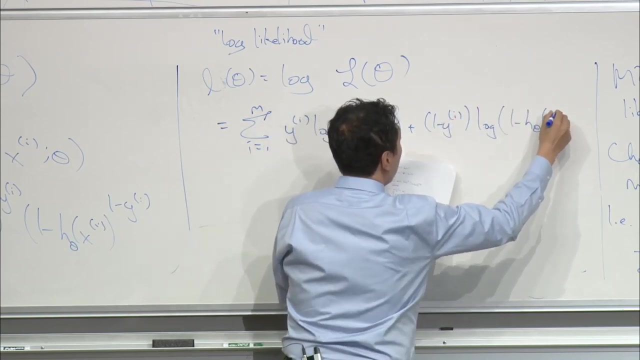 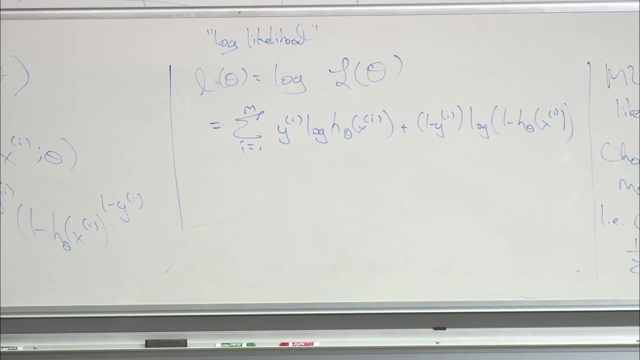 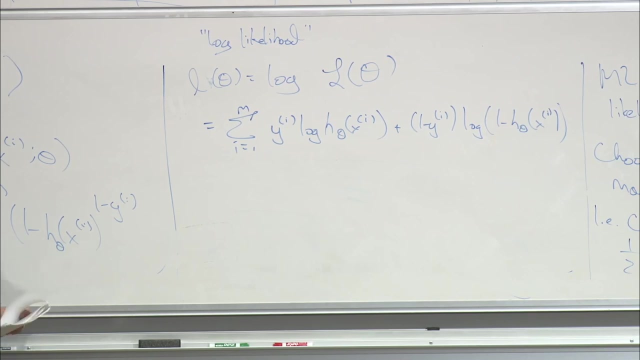 And so if you take the log of that, uh, you end up with. you end up with that, Okay, And um it- so. so, in other words, uh, the last thing you want to do is try to choose the value of Theta. 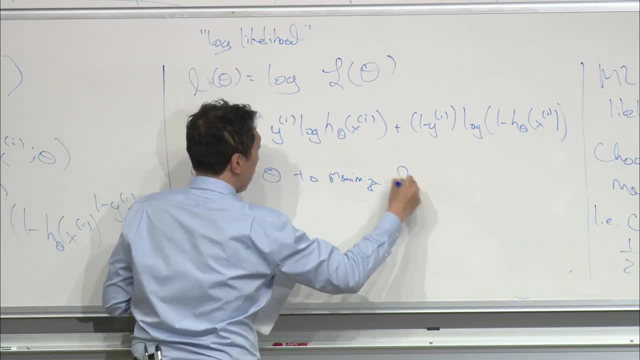 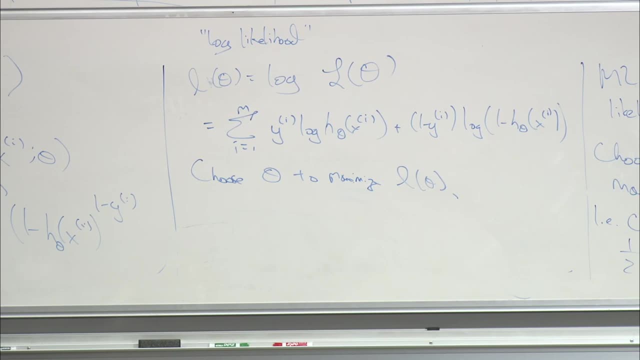 to try to maximize L of Theta. Okay Now, so so just just to summarize where we are right: Uh, if you're trying to predict, you know, malignancy and benignness of uh tumors, you'd have a training set with x, i, y, i. 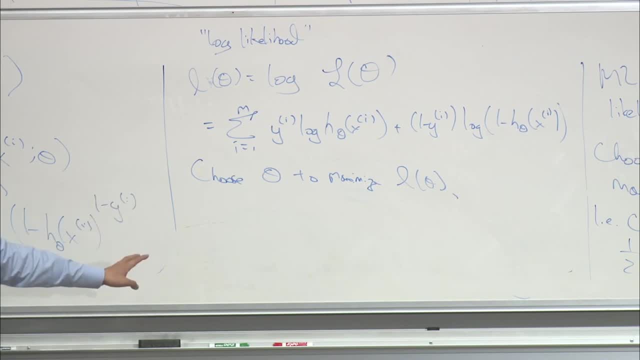 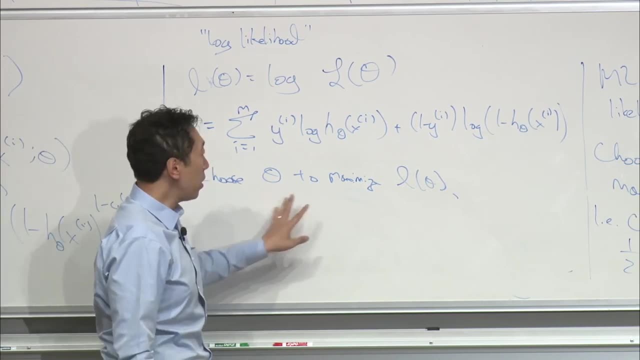 you define the likelihood, define the log likelihood and then what you need to do is have an algorithm, such as gradient descent or gradient descent- talk about that in a sec- to try to find the value of Theta that maximizes the log likelihood. 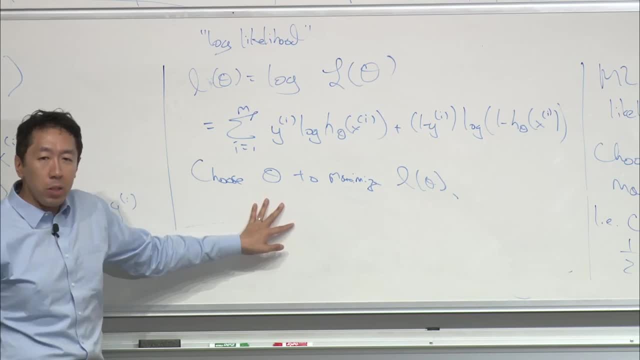 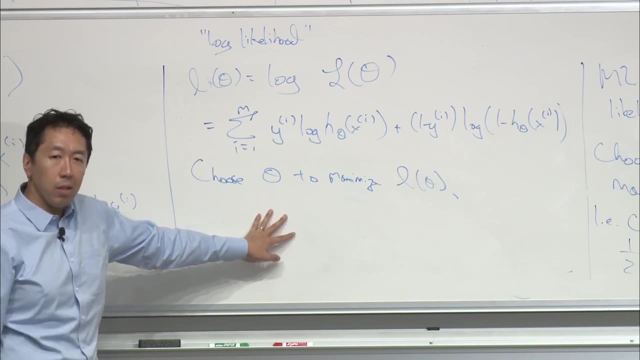 And then, having chosen the value of Theta, when a new patient walks into the doctor's office, you would, you know, take the features of the new tumor and then use H of Theta to estimate the chance that this new tumor and the new patient that walks in tomorrow, to estimate the chance that this 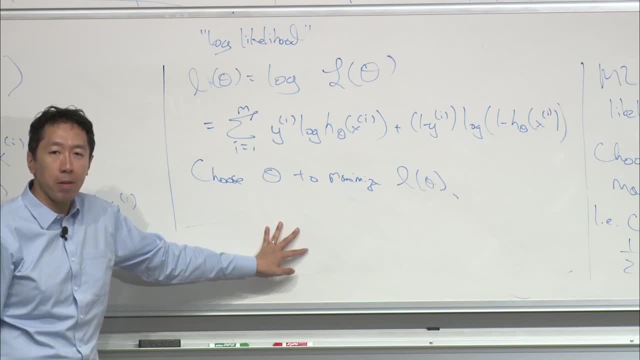 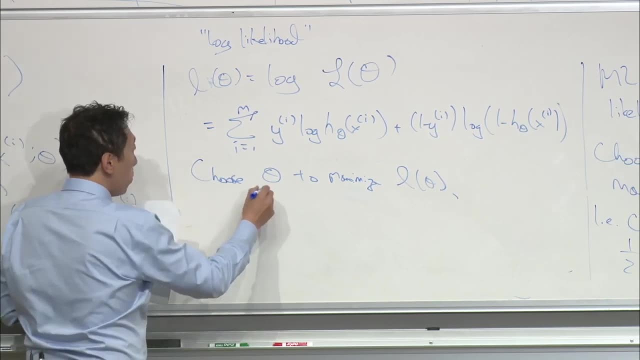 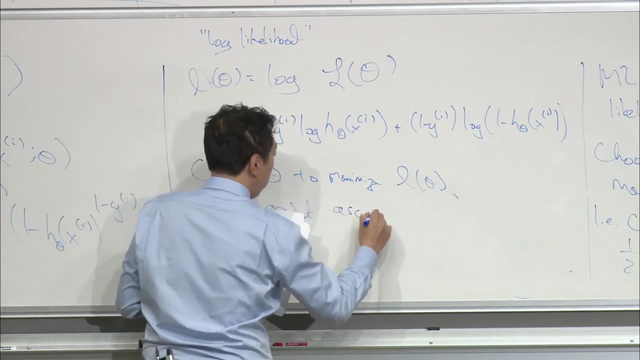 you think is, uh, is is molecular or benign. Okay, So, um, the algorithm we're going to use to choose Theta to try to maximize the log likelihood is, uh, gradient ascent or batch gradient ascent, And what that means is um, 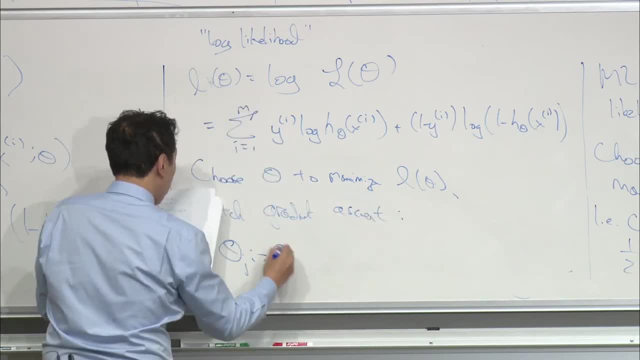 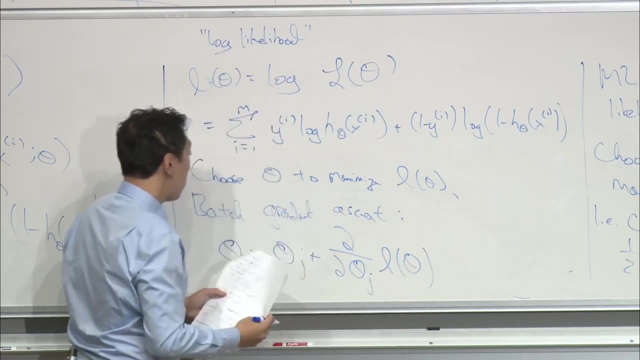 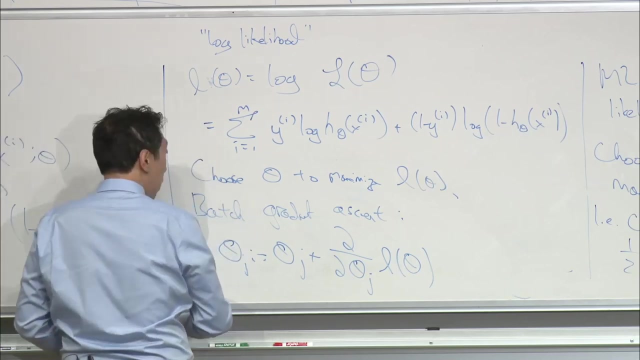 we will update the parameters Theta j according to Theta j plus uh, the partial derivative with respect to the log likelihood. Okay, Um, and the differences from what you saw for uh linear regression from last time is the following: Uh, just two differences, I guess. 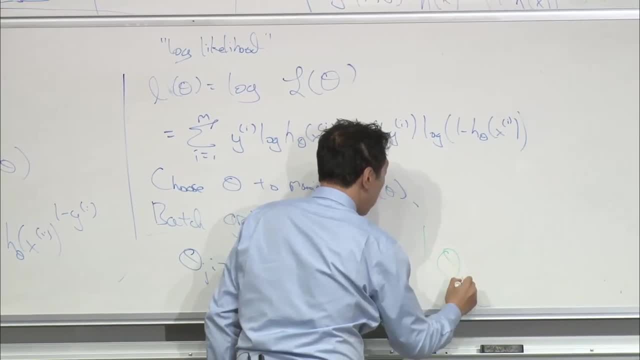 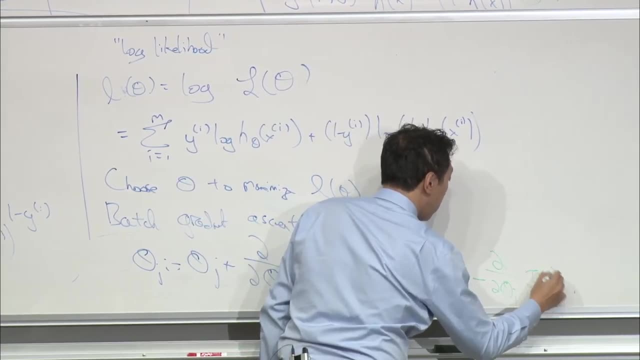 For linear regression. last week I had written this down: Theta j gets updated as Theta j minus partial with respect to Theta j of j of Theta right. So you saw this on Wednesday. So the two differences between that is uh. 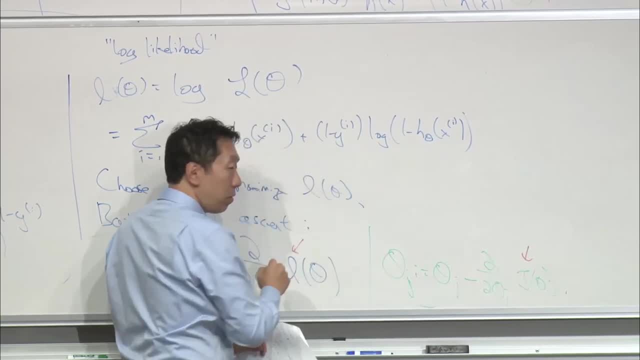 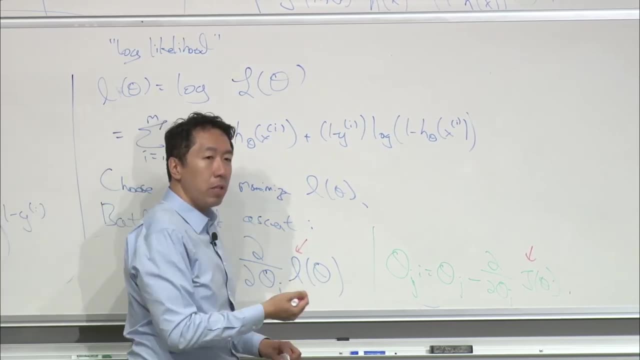 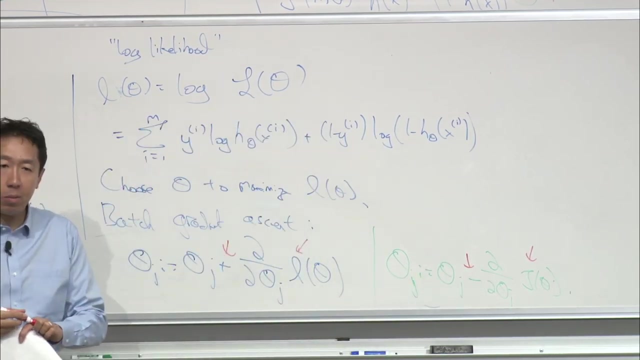 well, first, instead of j of Theta, you're now trying to optimize the log likelihood instead of the squared cost function. And the second change is: previously you were trying to minimize the squared error, That's why we had the minus, And today you're trying to maximize the log likelihood. 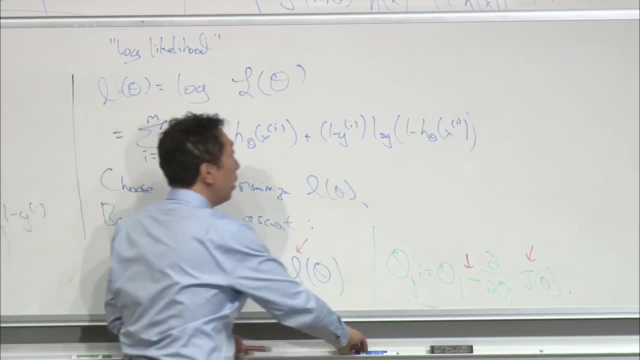 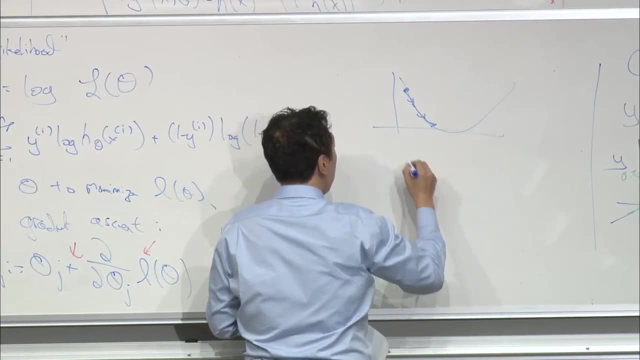 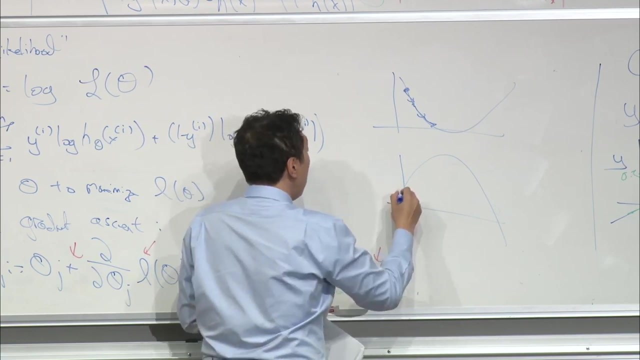 which is why there's a plus sign: Okay And so, um. so gradient descent, you know, is trying to climb down this hill, whereas gradient ascent has a- um, uh, has a- has a concave function like this: 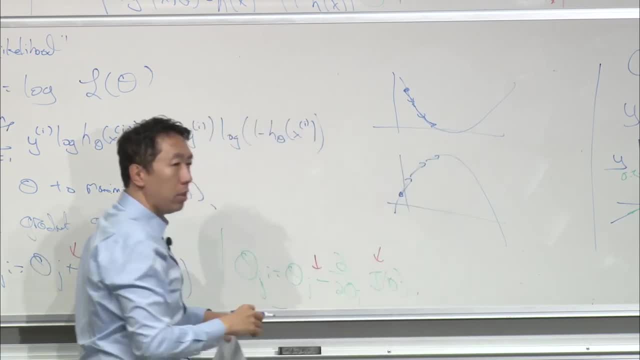 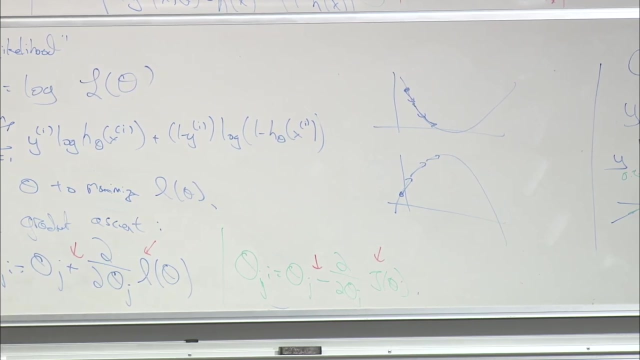 And it's trying to right climb up the hill rather than climb down the hill. So that's why there's a plus symbol here instead of a minus symbol, because you're trying to maximize the function rather than minimize the function, Mm-hmm. So, um, the last thing to- to really flesh out this algorithm. 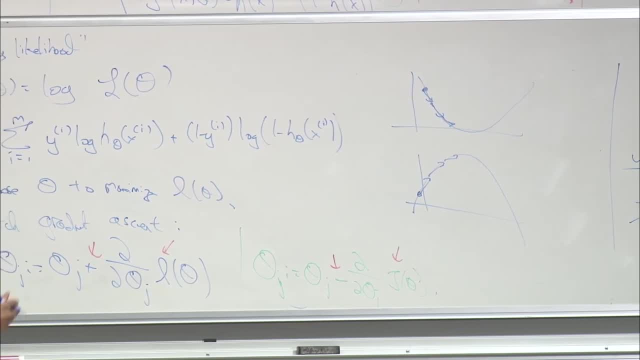 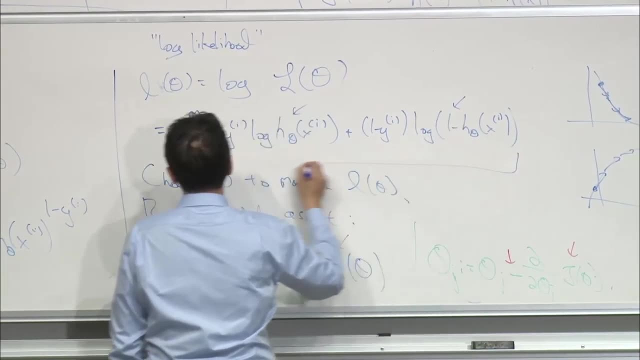 which, uh, is done in the lecture notes by- I don't want to do it here today- is to um plug in the definition of h of Theta into this equation and then take this thing, So that's the log likelihood of Theta. 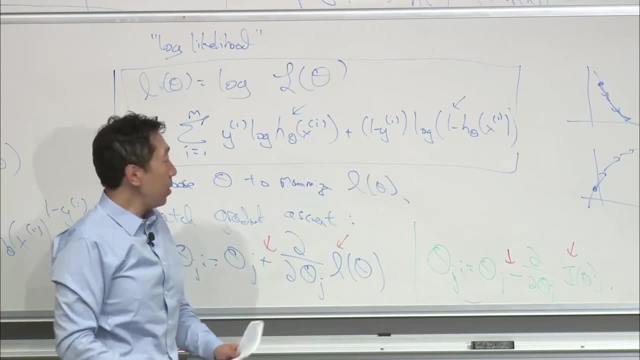 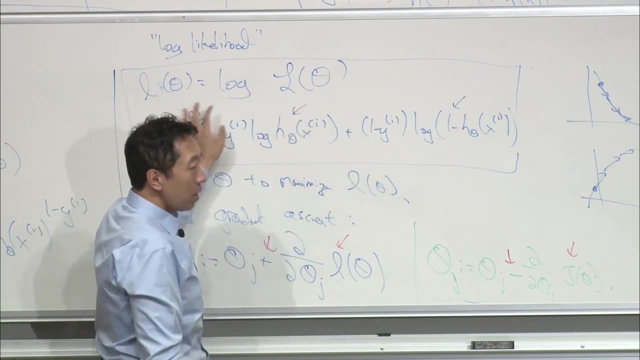 And then through you know calculus and algebra. uh, you could take derivatives of this whole thing. with respect to Theta, This is done in detail in the lecture notes, so I don't want to do this in class, But go ahead and take derivatives of this big formula with respect to. 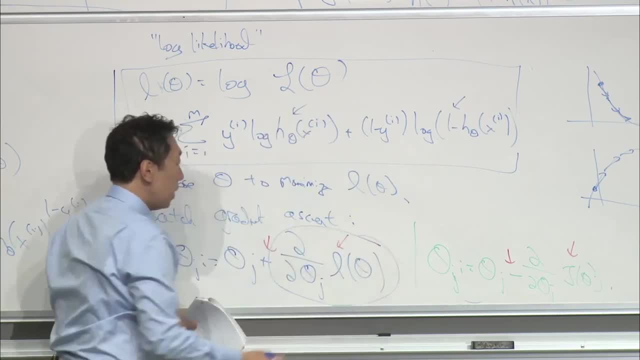 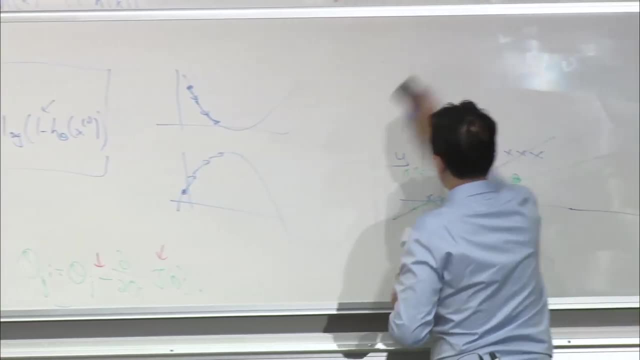 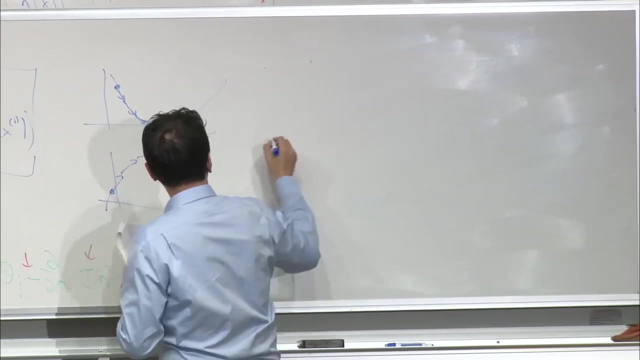 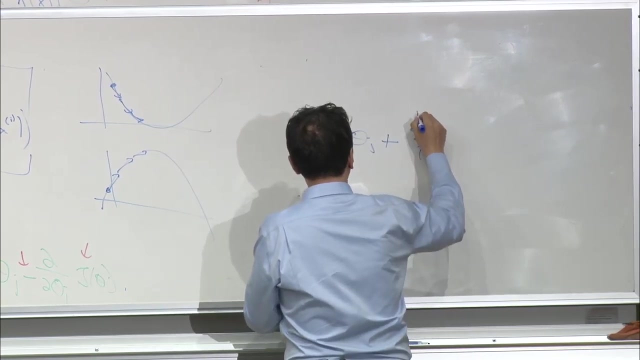 um the parameters Theta, in order to figure out what is that thing right, What is this thing that I just circled? And it turns out that if you do so, you will find that batch gradient ascent is the following: You update Theta j according to- oh. 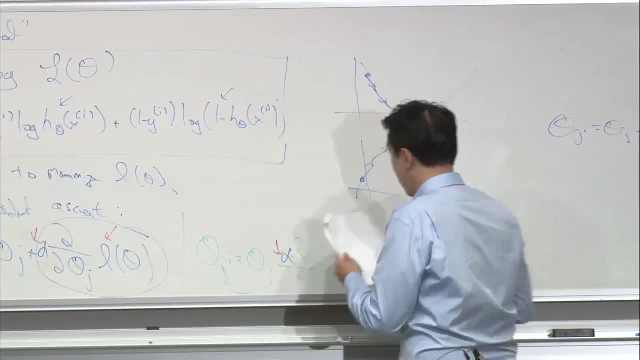 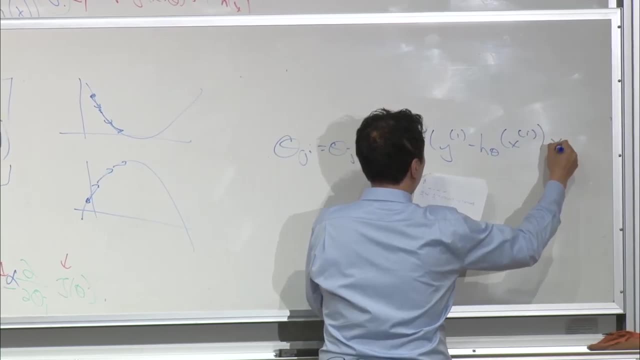 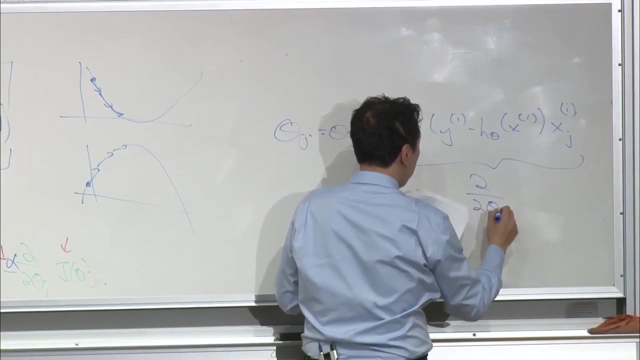 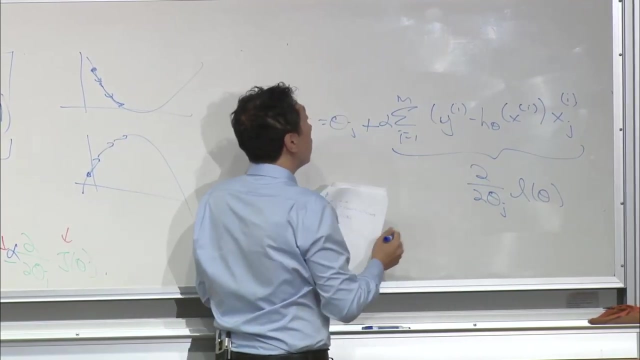 actually, I'm sorry, I forgot the learning rate. Yeah, it's your learning rate alpha, Okay. Learning rate alpha times. this okay, Uh, because this term here is the partial derivative, with respect to Theta j, of the log likelihood, okay. 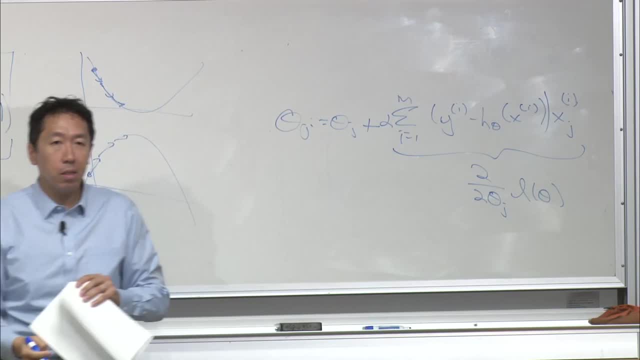 And the full calculus and so on. derivation is given in the lecture notes. Okay, Um, yeah, Is there a chance of local maximum in this case? Uh, no, there isn't. It turns out that this function, that the log likelihood function, 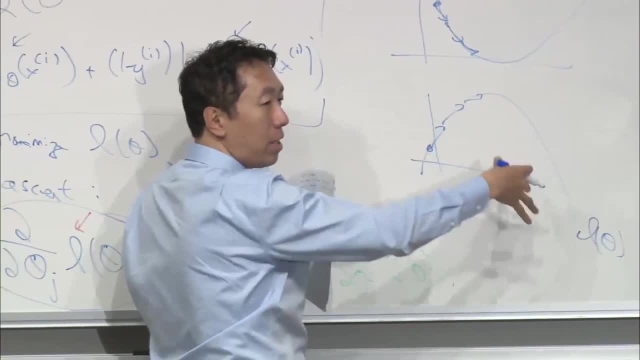 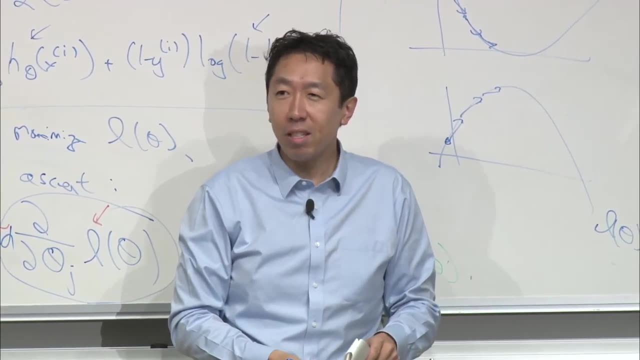 L of Theta, full logistic regression. it always looks like that. So this is a uh concave function. So there are no local op-, the- the- the only maximum is the global maximum. There's actually another reason why we chose the logistic function. 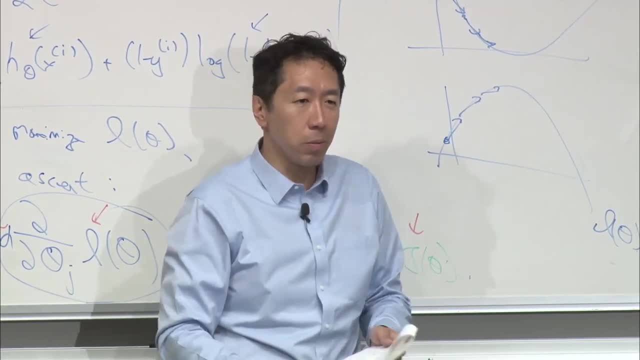 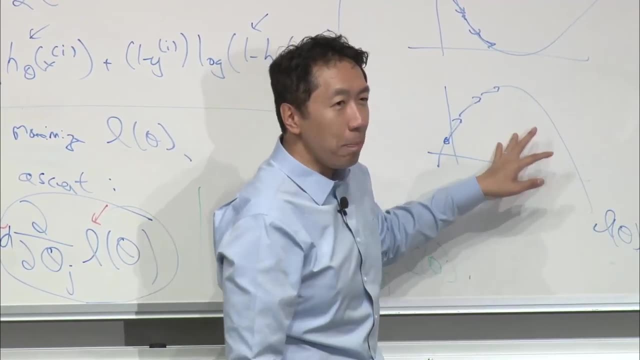 because if you choose the logistic function rather than some other function greater than 0 to 1, you're guaranteed that the likelihood function has only one global maximum. uh, and this- there's actually a big class of algorithms, Actually, what you'll see on Wednesday. 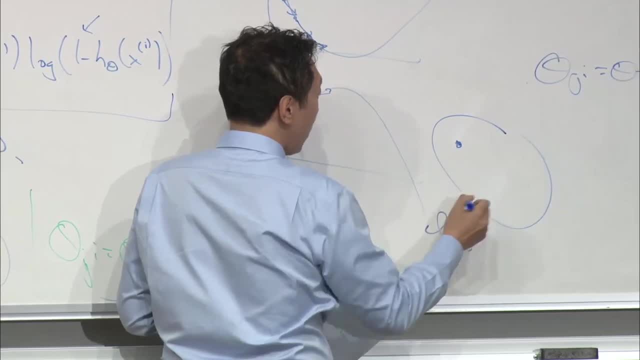 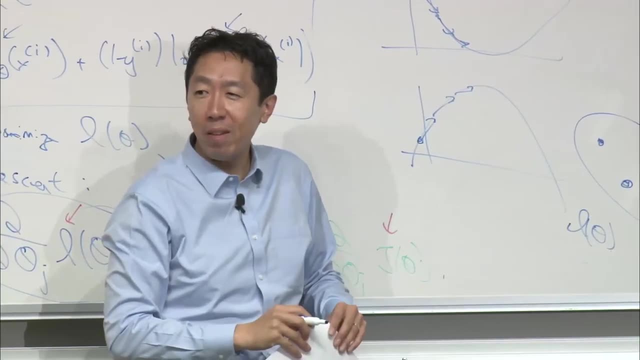 this is a big class of algorithms, of which linear regression is one example, logistic regression is another example, and for all of the algorithms in this class, there are no local optimal problems when you- when you- derive them this way. So you see that on Wednesday, when we talk about generalizing the models, 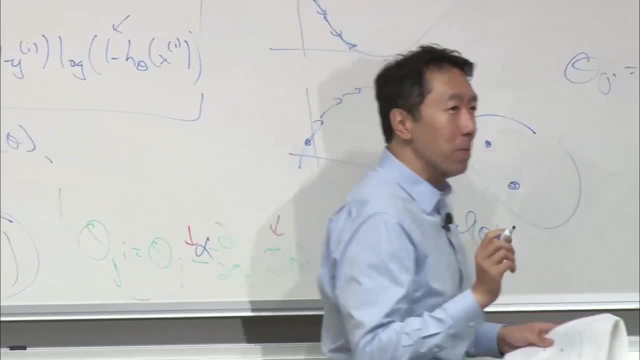 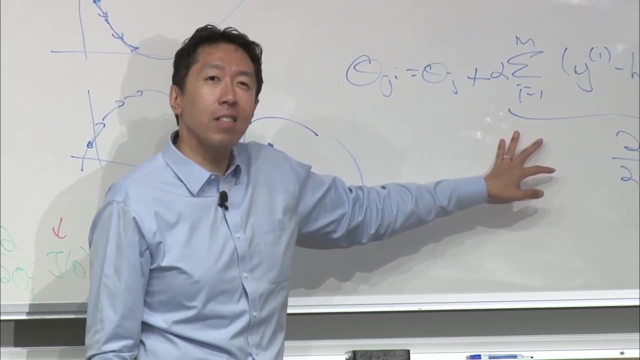 Okay, Um. so actually, before I take your questions, just one- one question for you to think about. This looks exactly the same as what we've figured out for linear regression, right, Like when- when- actually the difference for linear regression was I had 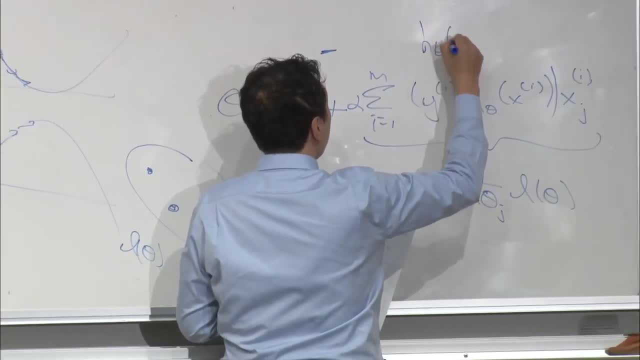 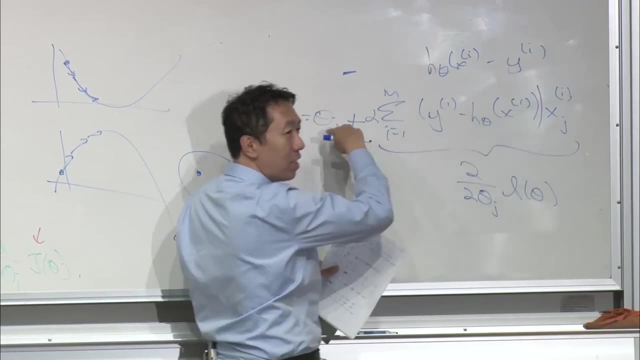 the minus sign here and I reversed these two terms. I think I have h theta big sine minus yi If you put the minus sign there and reverse these two terms. so take the minus minus. this is actually exactly the same as what we had come up with for linear regression. 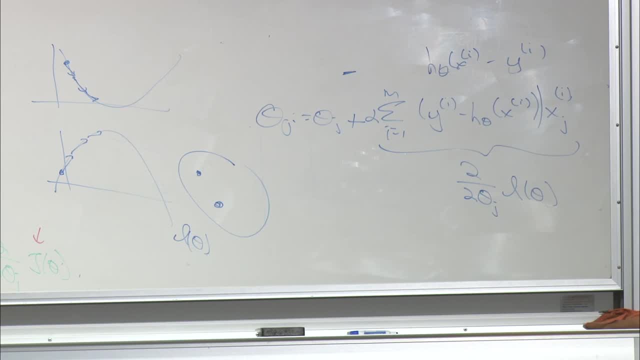 So why- why- why is this different? right? I started off saying: don't use linear regression for classification problems because of, uh, because of that problem- that a single example could really you know. so I- I started off with an example, saying that linear regression is really bad for. 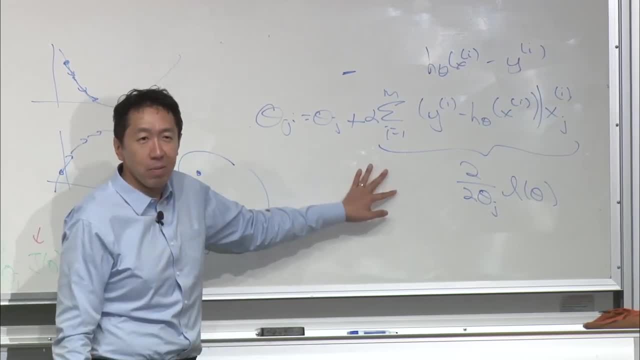 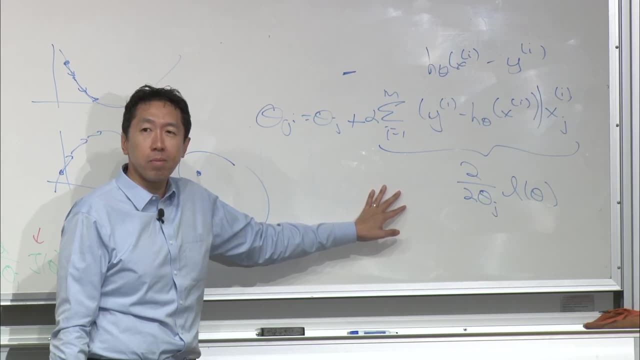 classification, and then we did all this work and came back to the same algorithm. So what happened? Just-? yeah, go ahead. Um, your h of theta is normally here now. Yeah, All right, Cool, Awesome Right. So what happened is the definition of h of theta is now different than before. 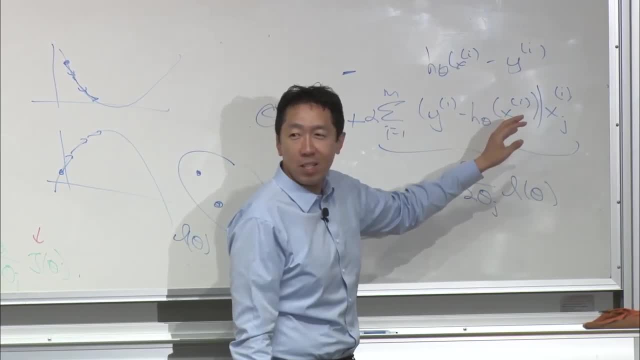 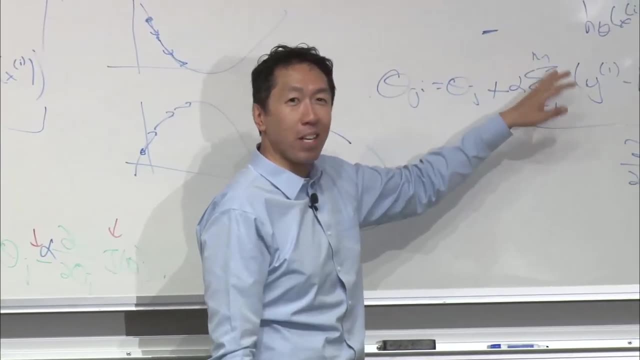 but the surface level, the equation turns out to be the same. Okay, Um and again, it turns out that for every algorithm in this class of algorithms you see on Wednesday, you- you end up with the same thing. Actually, this is a general property of a much bigger class of algorithms called generalized linear models. 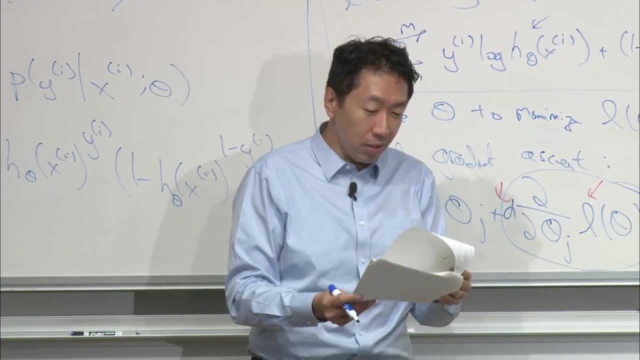 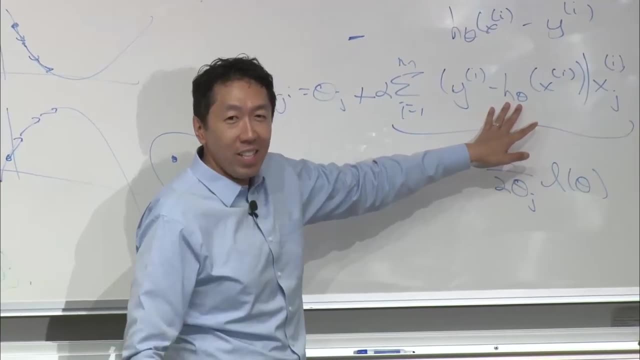 Um, although, yeah, interesting historical divergence, uh, uh uh, because of the confusion between these two algorithms in the early history of machine learning, there was some debate about, you know, between academics saying, no, I invented that. 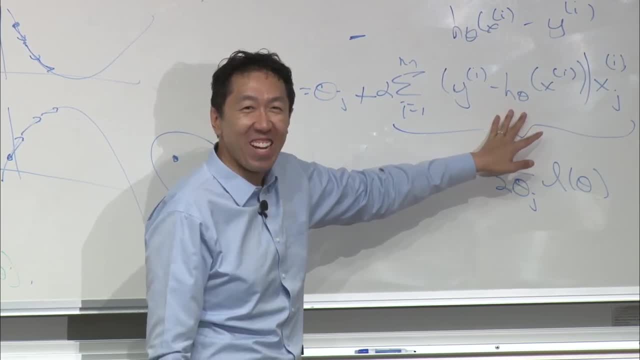 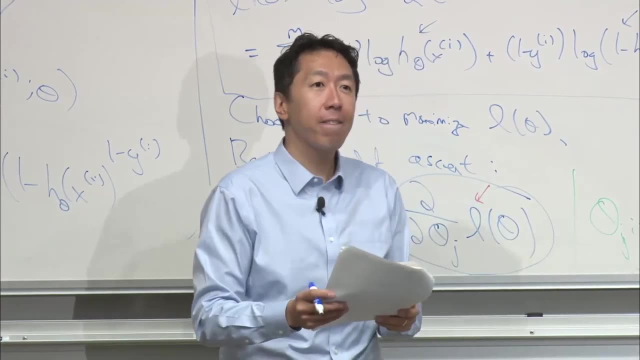 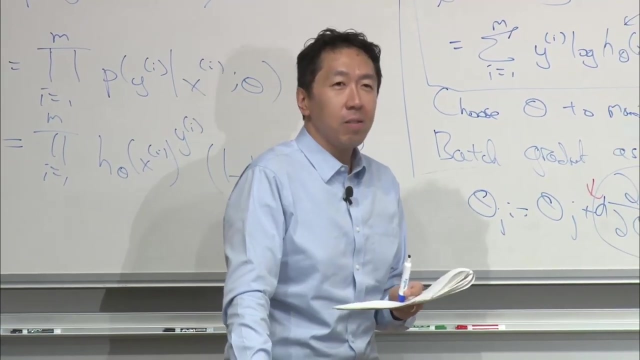 No, I invented that But- and then- and then- and then it goes. no, it's actually different algorithms, right, Um All right, Any questions? Oh, go ahead. Oh, great question: Is there equivalence of? 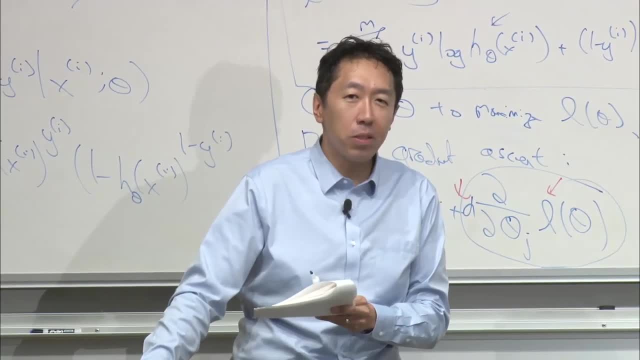 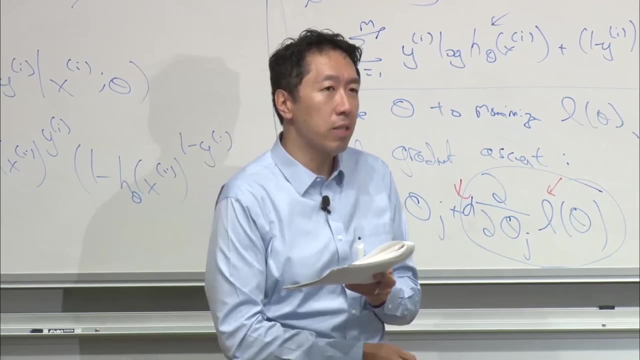 um normal equations to logistic regression? Um, short answer is no. Uh, so for linear regression, the normal equations gives you like a one-shot way to just find the best value of theta. Uh, there is no known way to just have a closed form equation that lets you find the best value of theta. 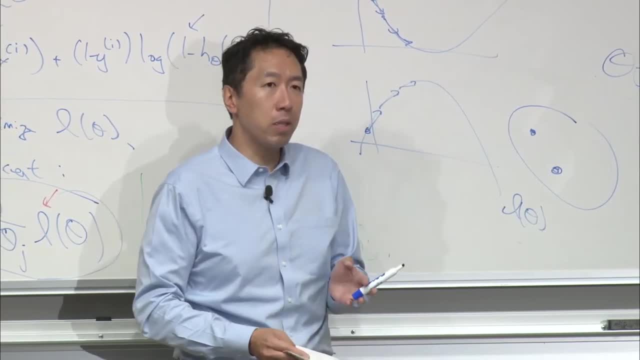 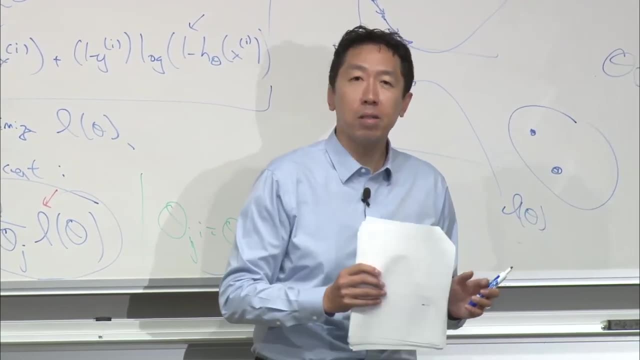 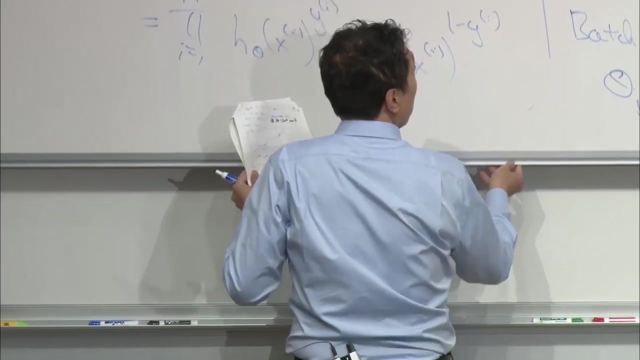 which is why you always have to use an algorithm, An iterative optimization algorithm, such as gradient ascent or- uh in- we'll see in a second Newton's method. All right, Cool, So um, there's a great lead-in to. 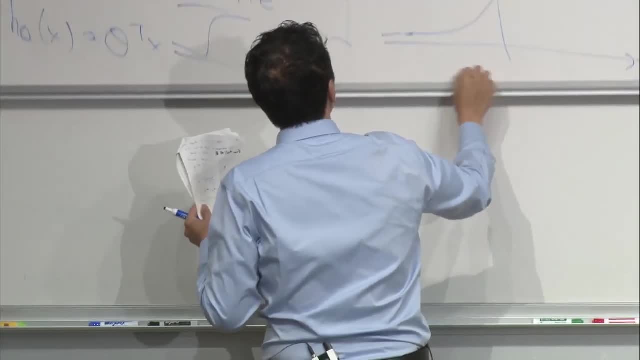 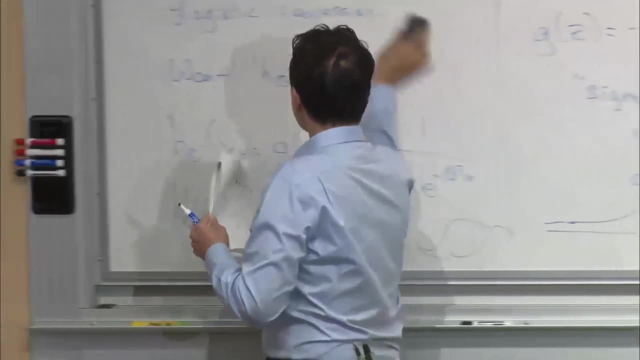 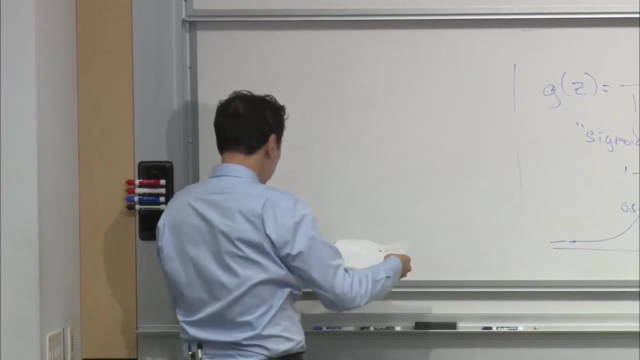 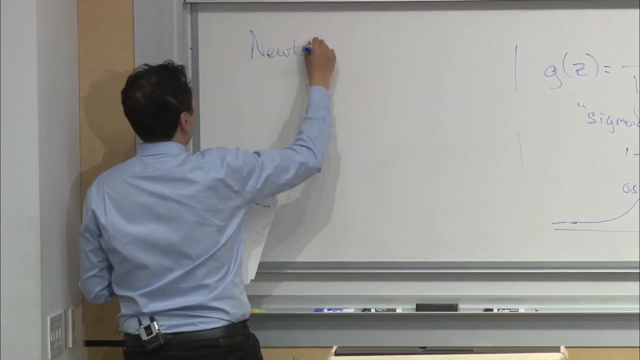 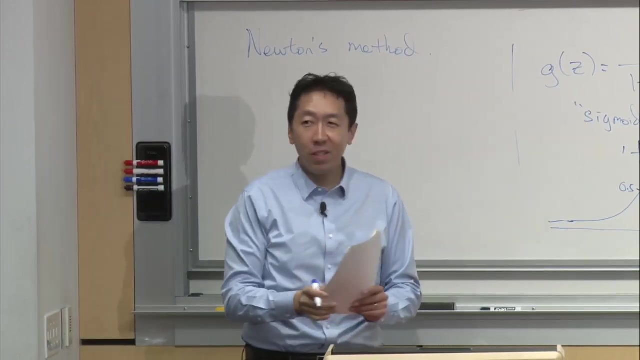 um, the last topic for today, which is Newton's method. Um, you know, gradient ascent. right, It is a good algorithm. I use gradient ascent all the time, but it takes a baby step, takes a baby step, takes a baby step. 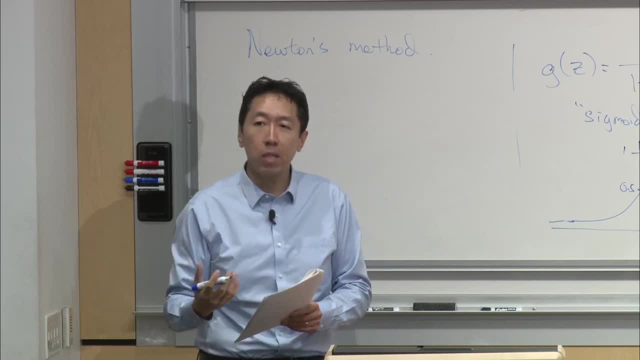 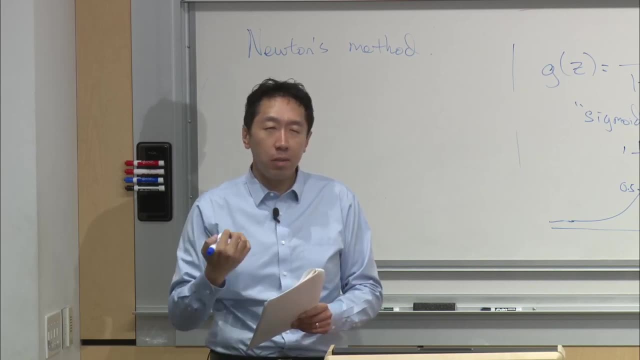 takes a lot of iterations for gradient ascent to converge. Um, there's another algorithm called Newton's method, which allows you to take much bigger jumps. So let's theta you know. so. so, uh, there are problems where you might need. 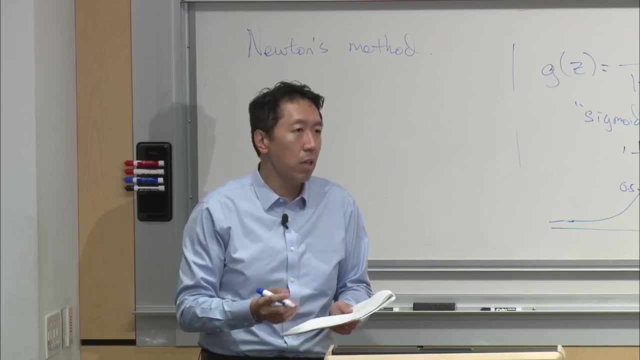 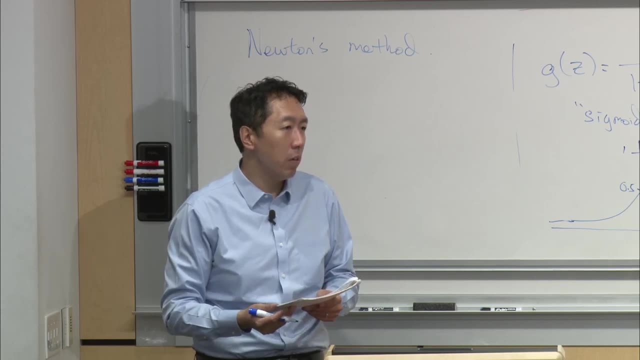 you know, say, a 100 iterations or 1,000 iterations of gradient ascent, that if you run this algorithm called Newton's method, you might need only 10 iterations to get to a very good value of theta Um, but each iteration will be more expensive. 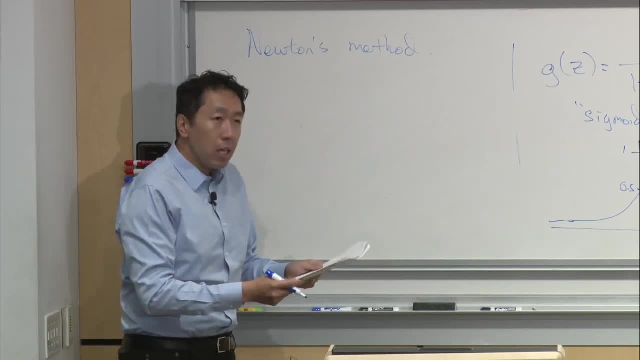 We'll talk about pros and cons in a second, But um, let's see how-. let's. let's describe this algorithm, which is sometimes much faster for gradient than gradient ascent, for optimizing the value of um theta. 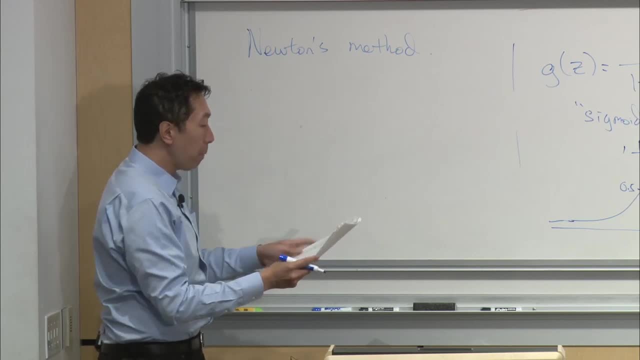 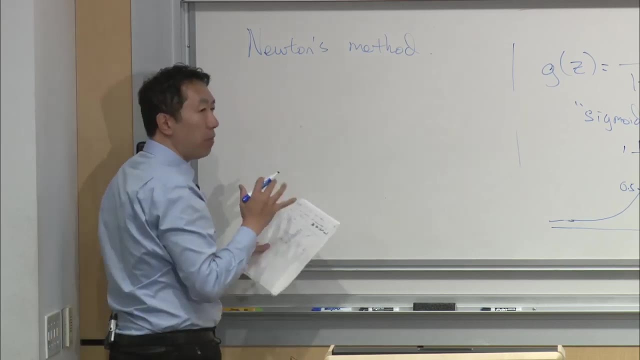 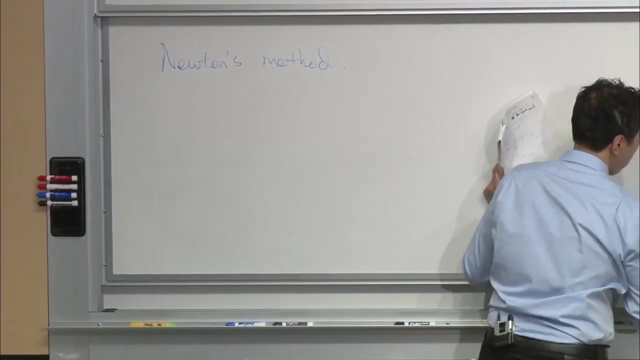 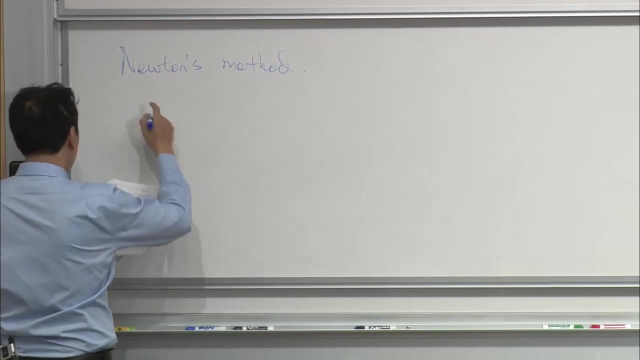 The value of theta. okay, So, um, what we'd like to do is, uh, all right, so let me, let me use a simplified one-dimensional problem to describe Newton's method. Um, so I'm gonna solve a slightly different problem with Newton's method. 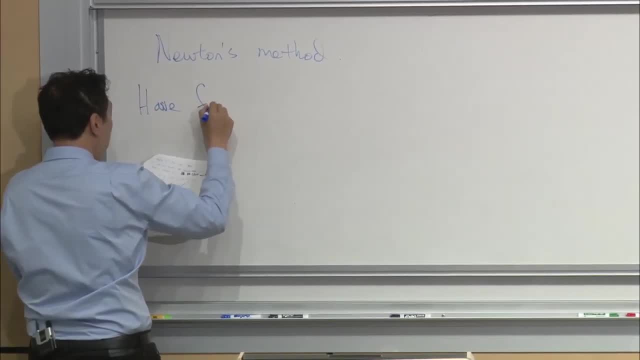 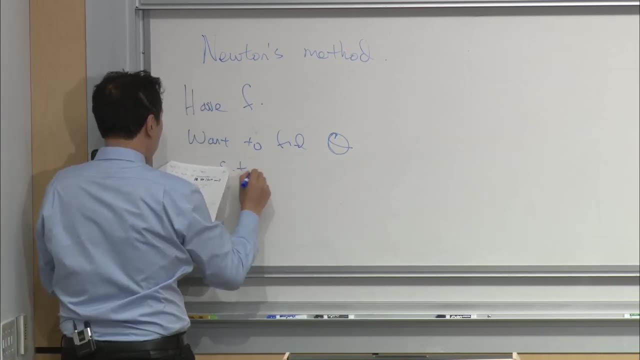 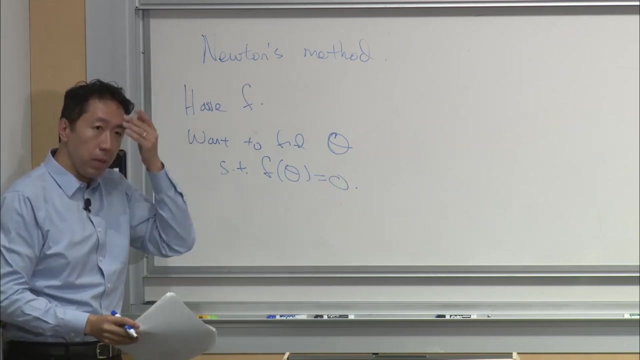 which is say, you have some function f right And you want to find, uh theta, such that f of theta is equal to 0, okay, So this is a problem that Newton's method solves And the way we're gonna uh. 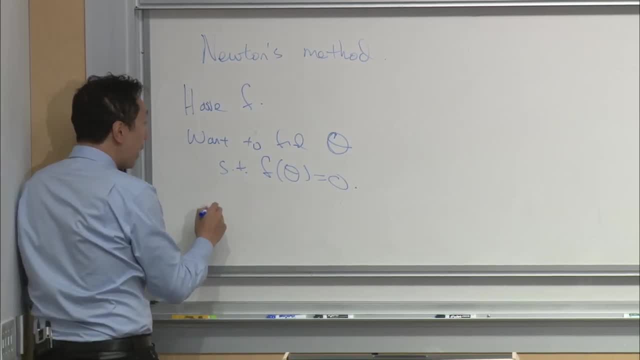 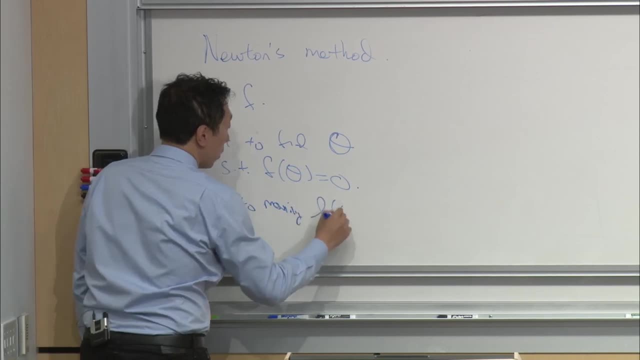 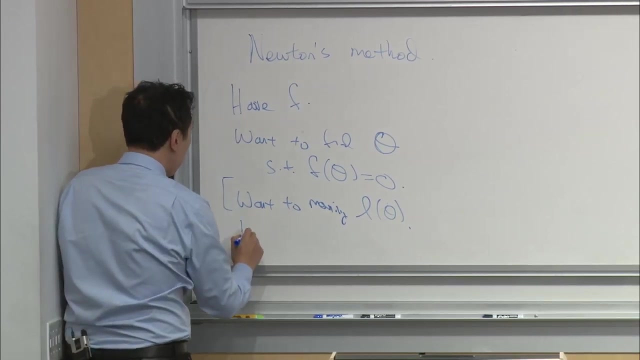 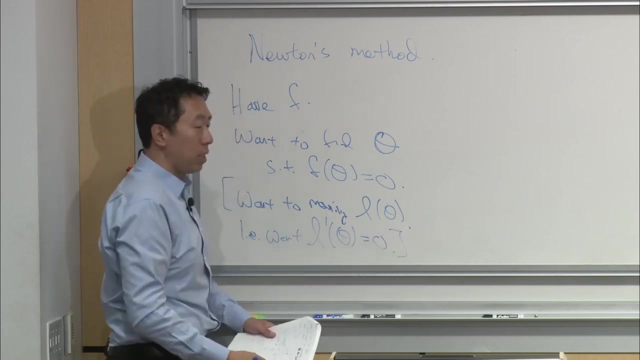 use this later is what you really want is to maximize L of theta right And well. at the maximum, the first derivative must be 0. So ie you want a value where the derivative L prime of theta is equal to 0, right. 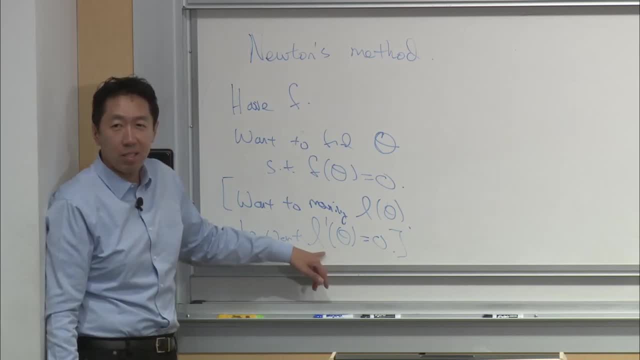 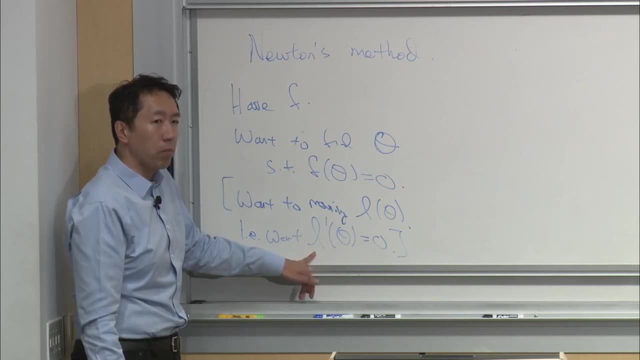 And L prime is the derivative of theta. uh, because this is right, L prime is, uh, another notation for the first derivative of theta. So you want to maximize the function or minimize the function. What that really means is you want to find a point where the derivative is equal to 0. 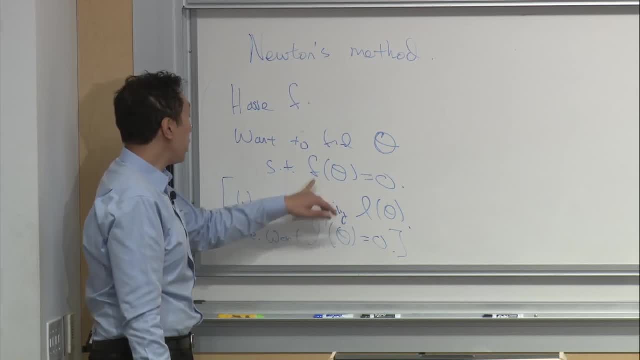 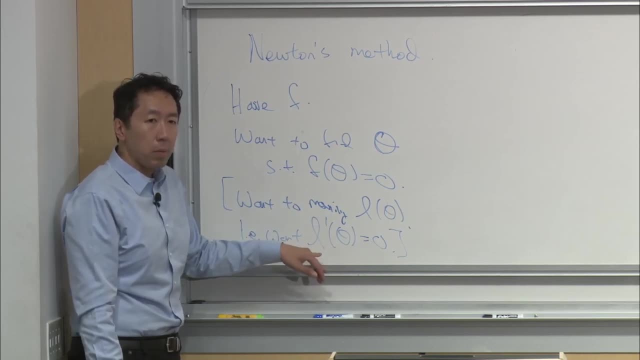 So the way we're going to use Newton's method is we're gonna set f of theta equal to the derivative and then try to find a point where the derivative is equal to 0, okay, But uh, to explain Newton's method. 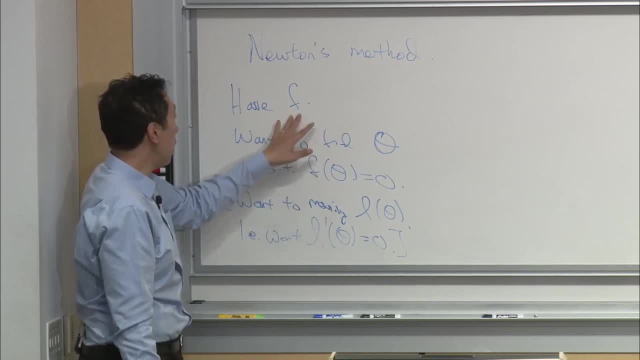 I'm gonna, you know, work on this other problem, where you have a function f and you just want to find the value of theta, where f of theta is equal to 0. And then- and then we'll set f equal to L, prime theta. 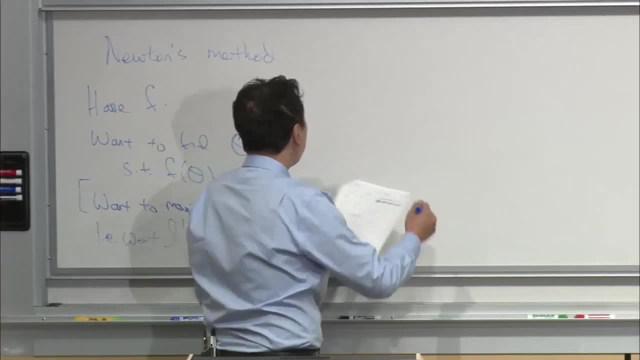 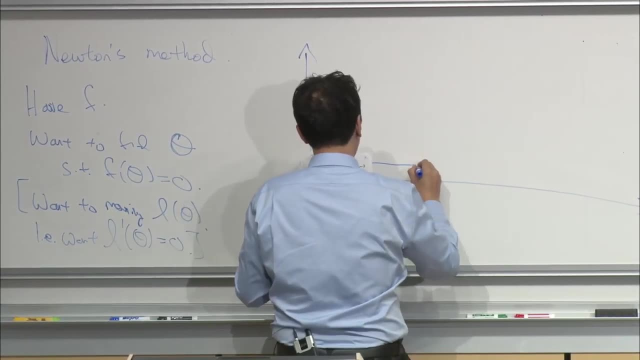 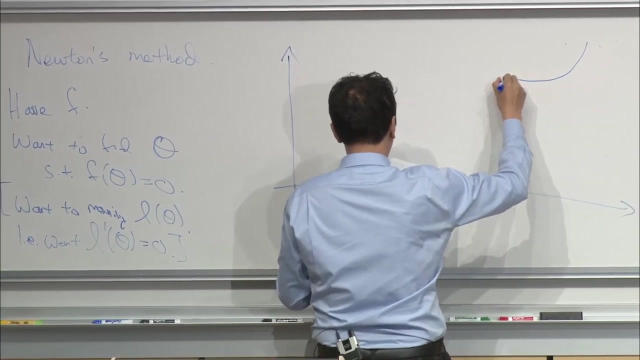 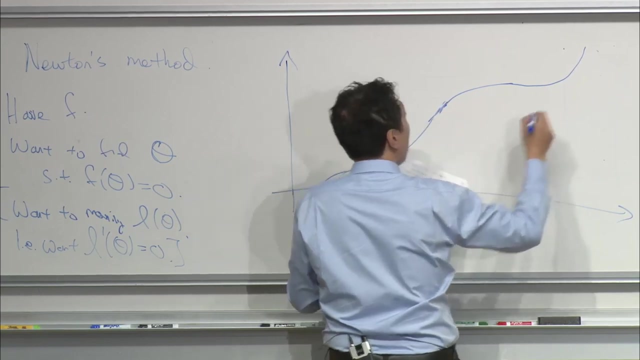 and that's how we'll- we'll apply this to um logistic regression. So let me draw in pictures how this algorithm works. All right, So let's say that's the function f? um, and you know to make this drawable on a whiteboard. 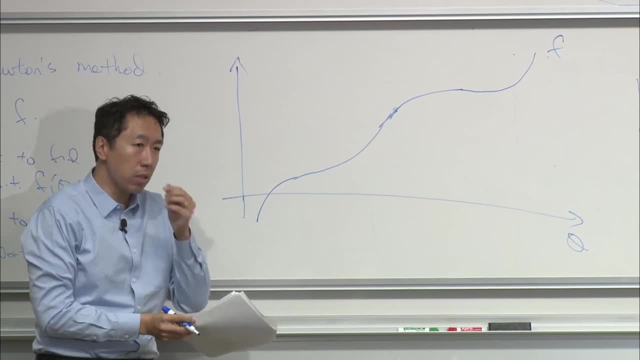 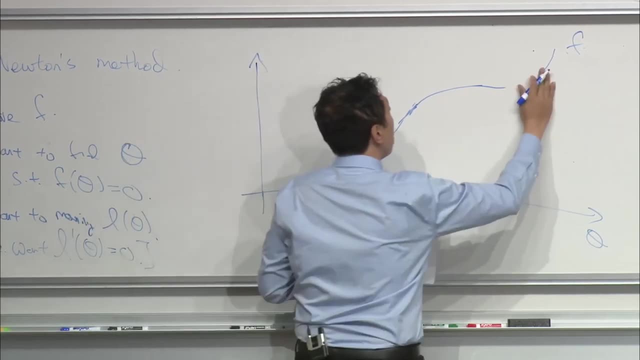 I'm gonna assume theta is just a row number for now. So theta is just a single, you know, like a scalar, a row number. Um, so this is how Newton's method works. Um, oh, and the goal is to find this point right. 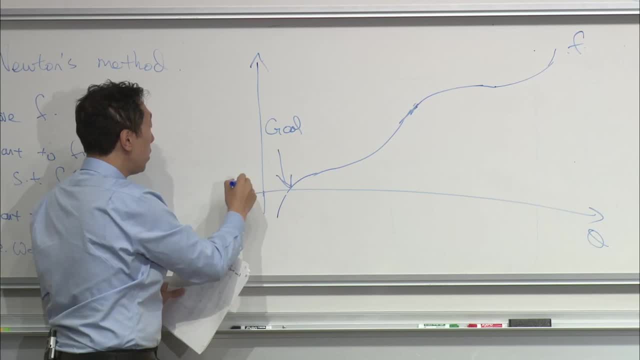 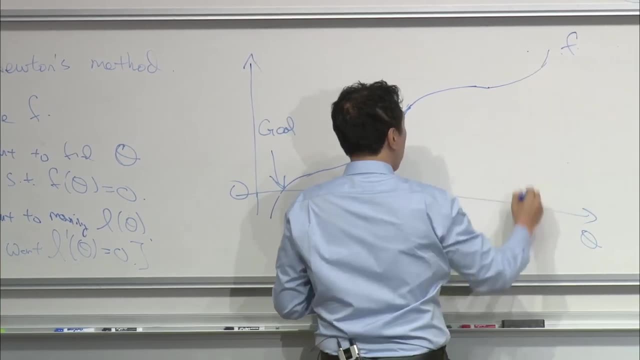 The goal is to find the value of theta where f of theta is equal to 0,. okay, So let's say you start off um right, Let's say you start off at this point, right, At the first iteration, you know. 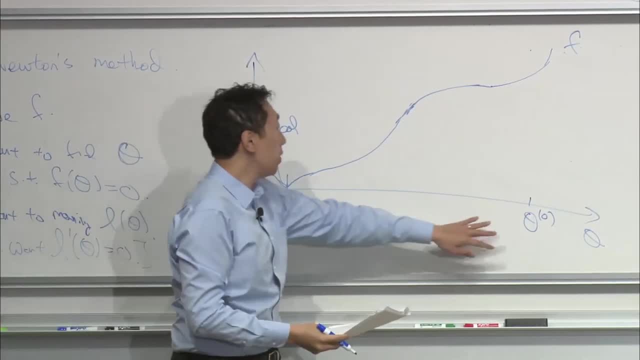 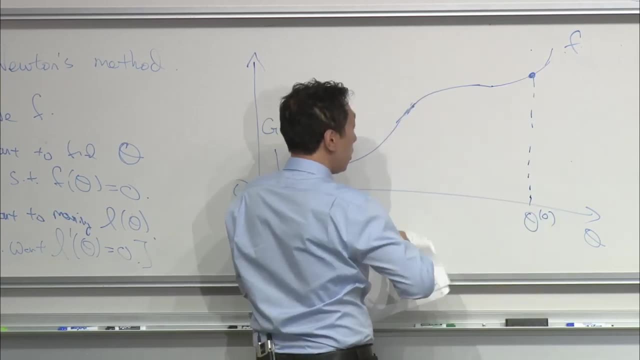 random initialized theta or initialized theta 0 or something. But let's say you start off at that point. This is how one iteration of Newton's method will work, which is actually- I'm gonna use a different color right- Start off with theta 0,. 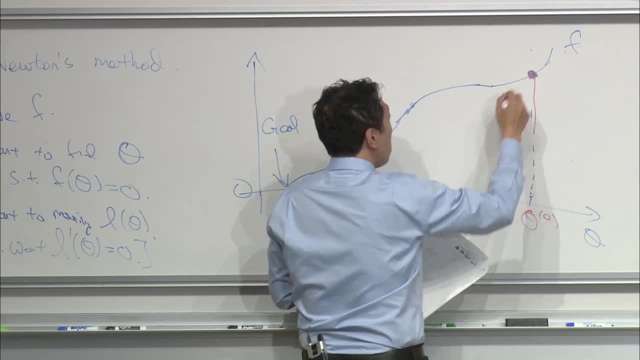 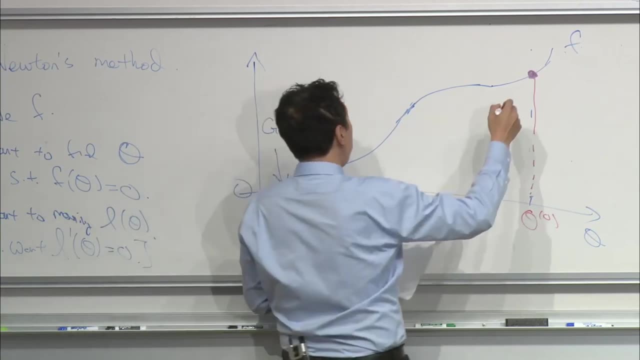 that's just the first value, first iteration. What we're going to do is look at the function f and then find a line that's just tangent to f. So take the derivative of f and find a line that's just tangent to f. 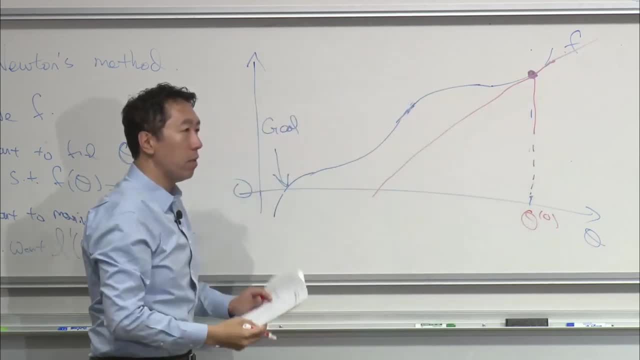 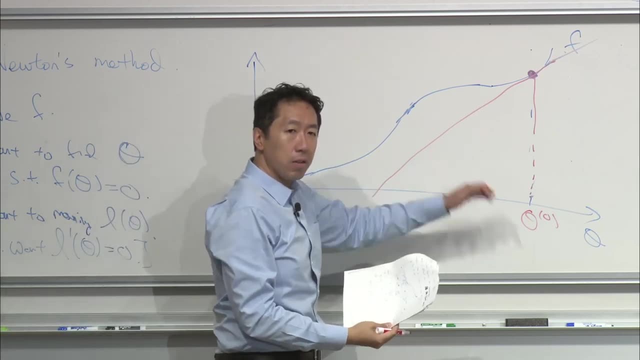 So take that red line that just touches the function f And we're gonna use, if you will use, a straight line approximation to f and solve for where f touches the horizontal. So we're gonna solve for the point where this straight line touches the horizontal axis, okay, 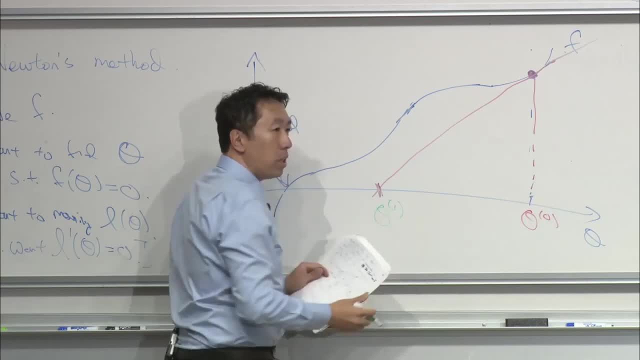 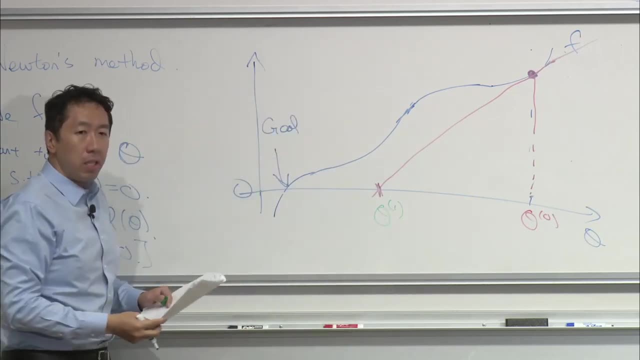 And then we're going to set this, and that's one iteration of Newton's method. So we're gonna move from this value to this value, okay, Um, and then, in the second iteration of Newton's method, we're gonna look at this point. 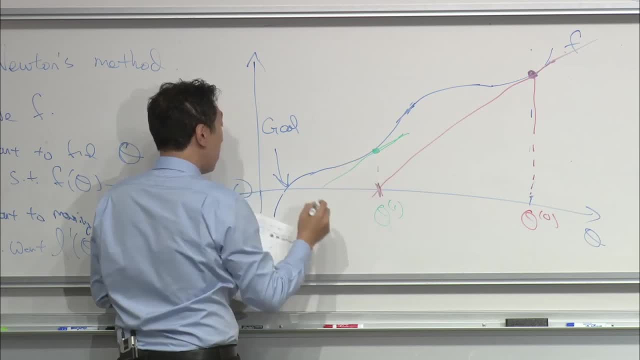 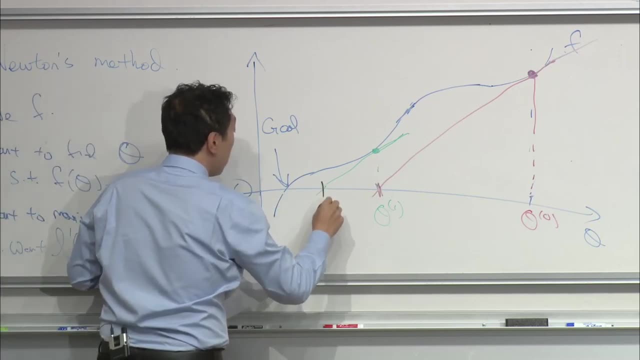 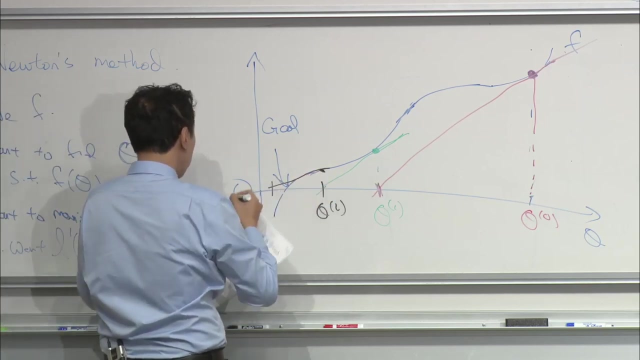 and again, you know, take a line that's just tangent to it and then solve for where this touches the horizontal axis, And then that's after two iterations of Newton's method, right. And then you repeat: Take this. Sometimes you can overshoot a little bit, but that's okay, right? 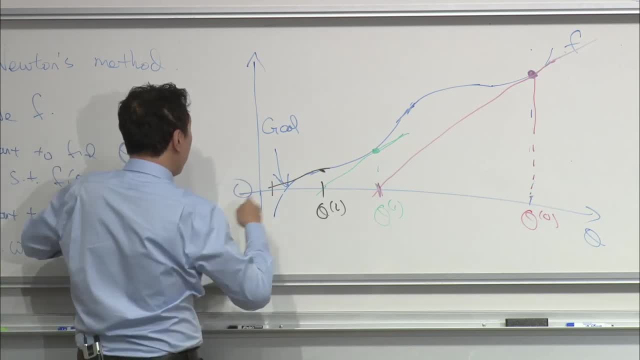 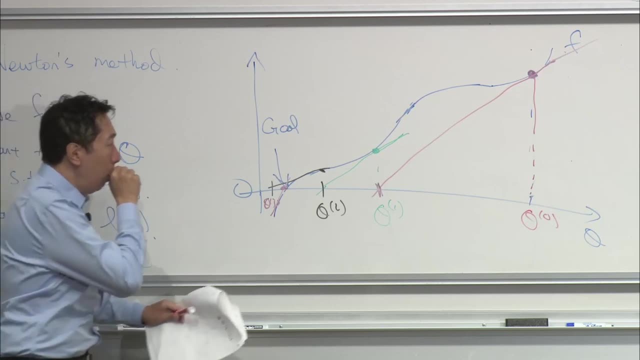 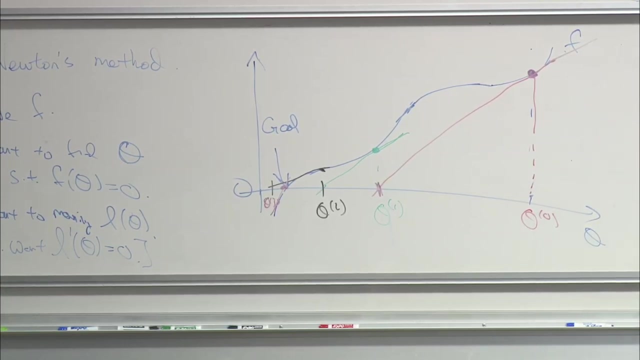 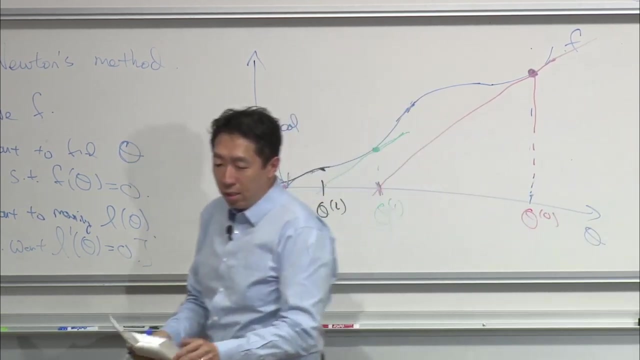 And then that's um, because I'll cycle back to red. That's theta 3.. Then you take this: That's theta 4.. Excuse me, So you can tell that, um, Newton's method is actually a pretty fast algorithm, right? 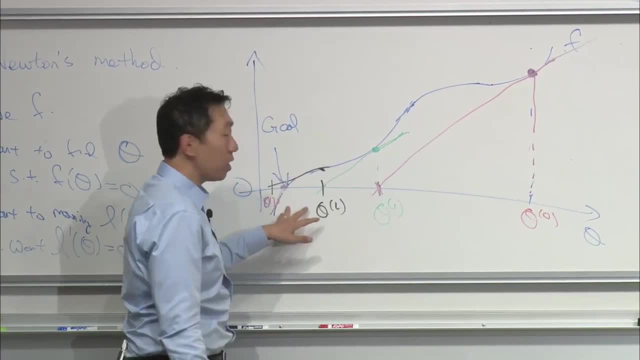 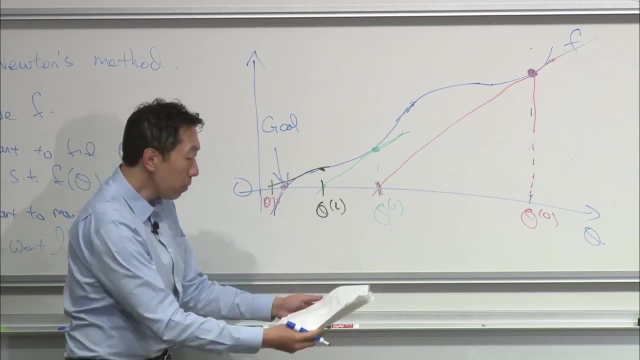 When- in just what 1,, 2,, 3, 4 iterations. we've gotten really really close, uh, to the point where f- if theta is equal to 0.. Um, so let's write out the math for how you do this. 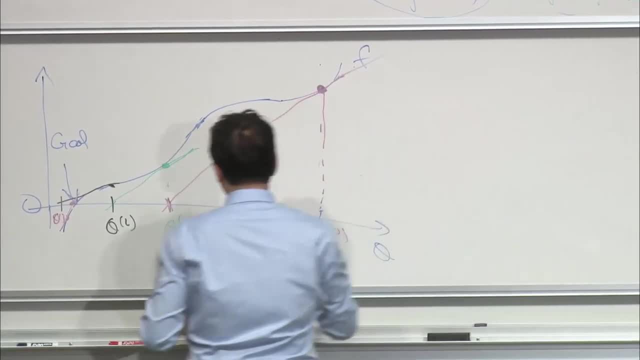 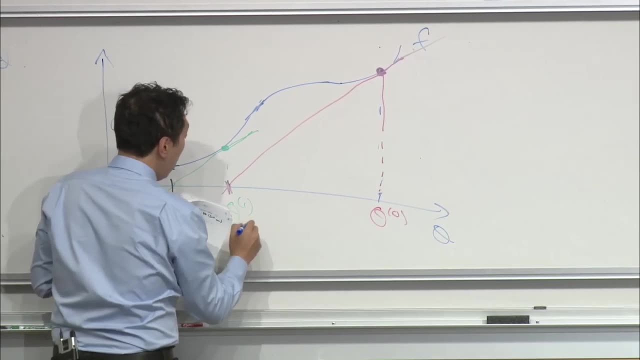 So, um, let's see I'm going to- so let me just write out the- derive. um, you know how you go from theta 0 to theta 1.. So I'm going to use this horizontal distance. I'm gonna denote this as uh, delta. 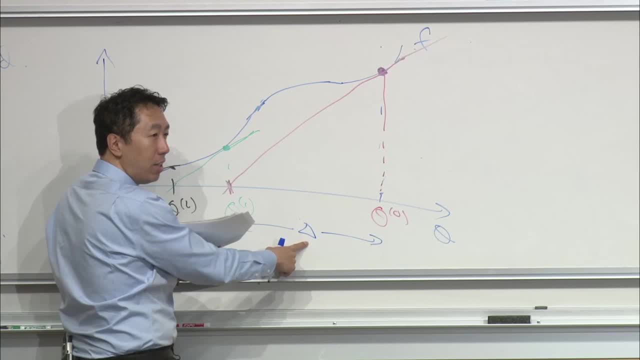 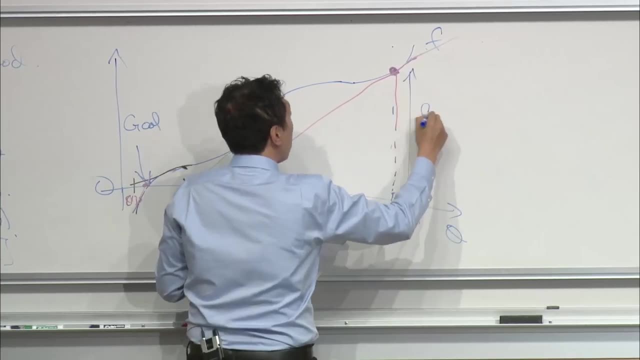 This triangle is uppercase Greek alphabet delta. right, This is lowercase delta. That's uppercase delta right. Um. and then the height here. well, that's just f of theta 0, right, Since the height is just f of theta 0.. 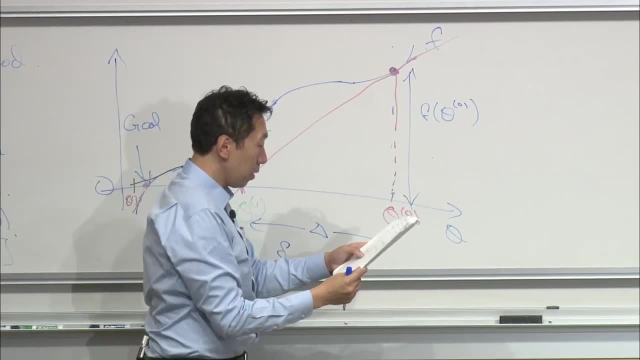 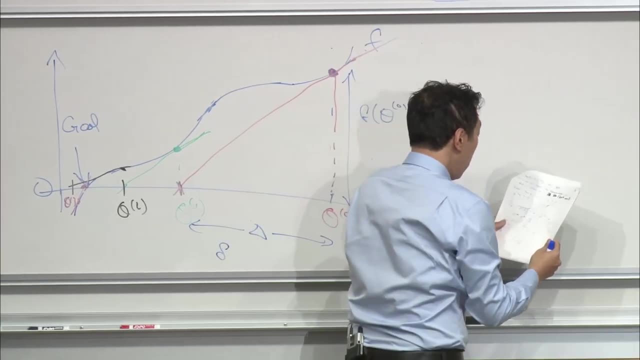 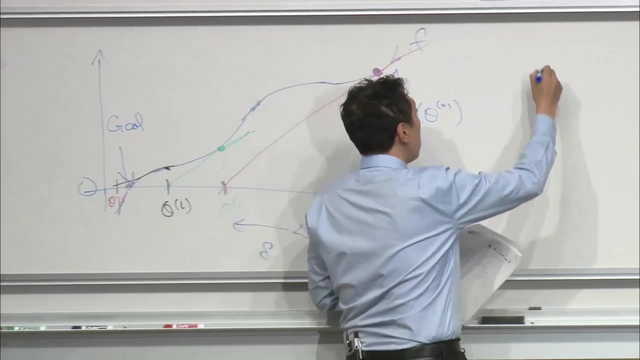 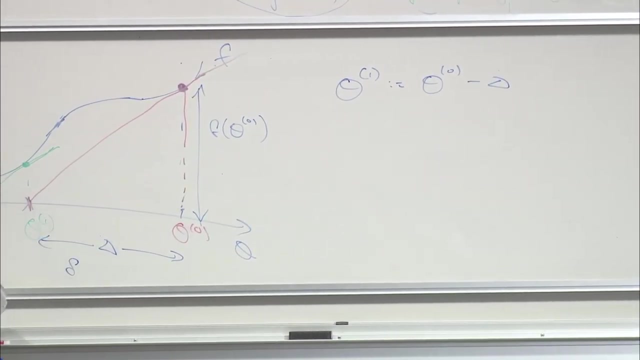 And so, um, let's see right. So, uh, what we'd like to do is solve for the value of delta, because one iteration of Newton's method is to set. you know, theta 1 is set to theta 0 minus delta, right? 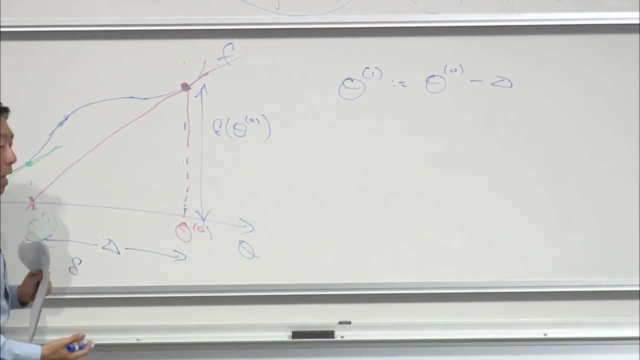 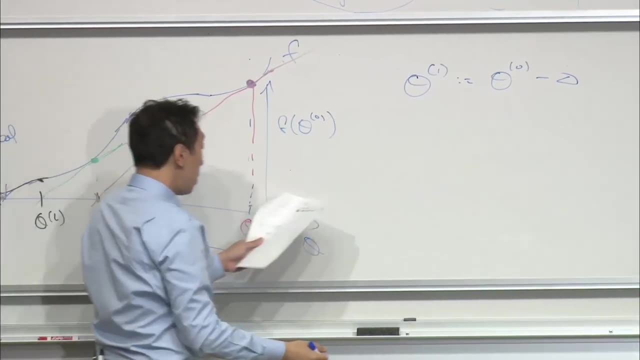 So how do you solve for delta? Well, from uh calculus we know that the slope of the function f is the height over the run right, Height over the width, And so we know that the derivative of delta f prime. 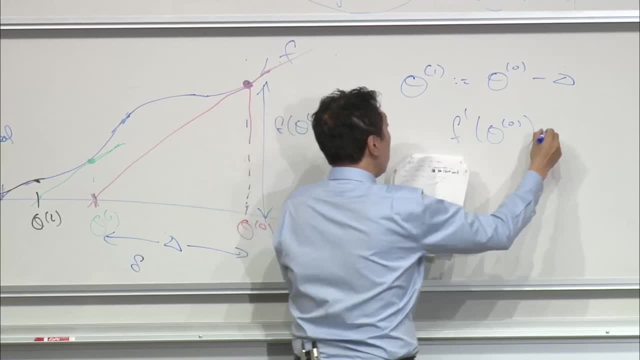 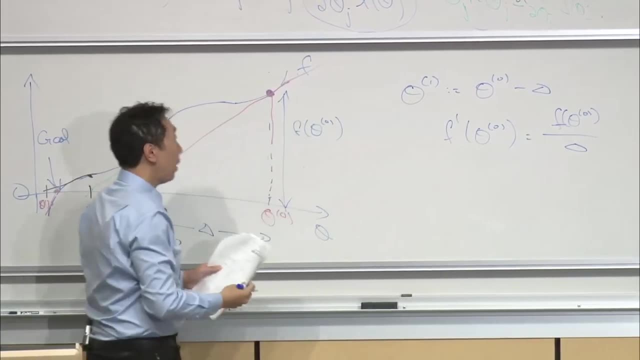 that's the derivative of f at the point theta 0, that's equal to the height, that's f- of theta divided by the horizontal right. So the derivative meaning the slope of the red line, this is by definition of derivatives. 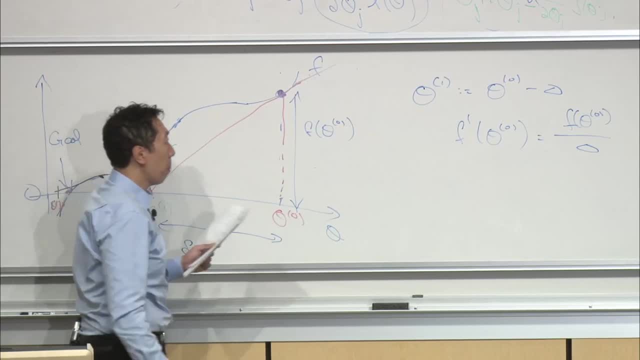 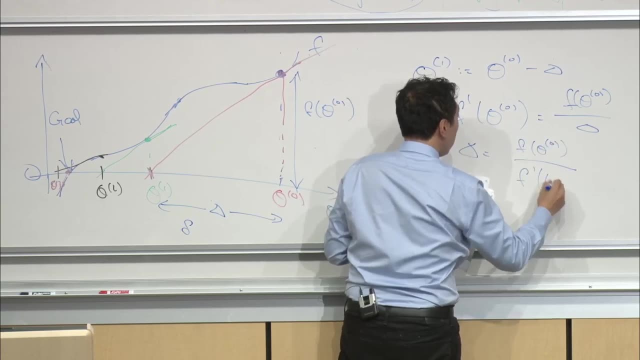 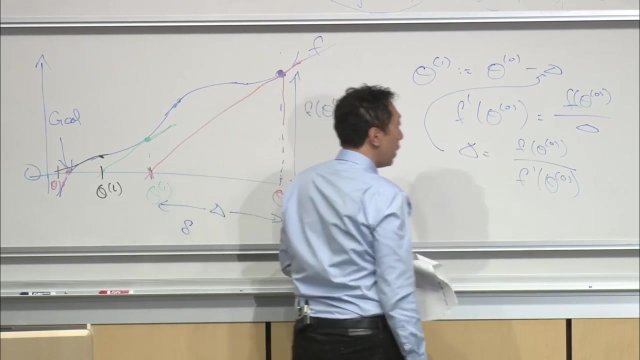 it's this ratio between this height over this width, Um, and so delta is equal to f of theta 0 over f, prime of Theta 0, and if you plug that in, then you find that a single iteration of Newton's method is the following rule of Theta: 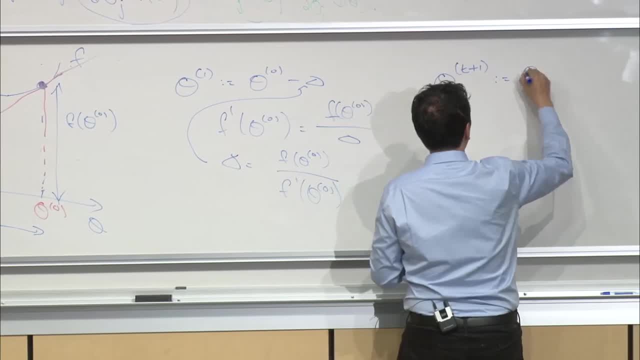 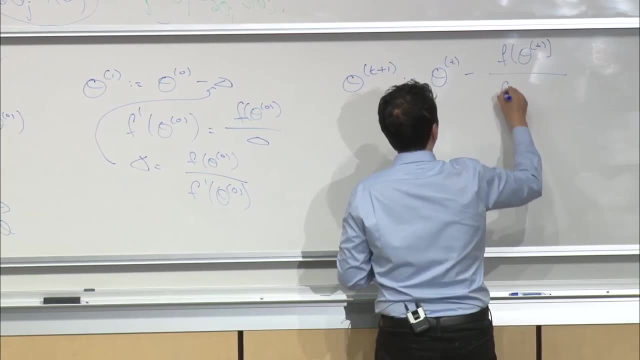 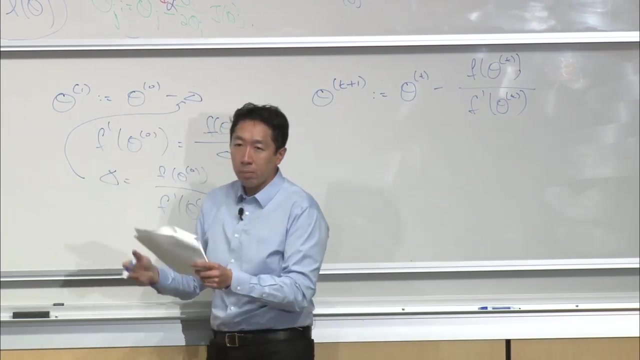 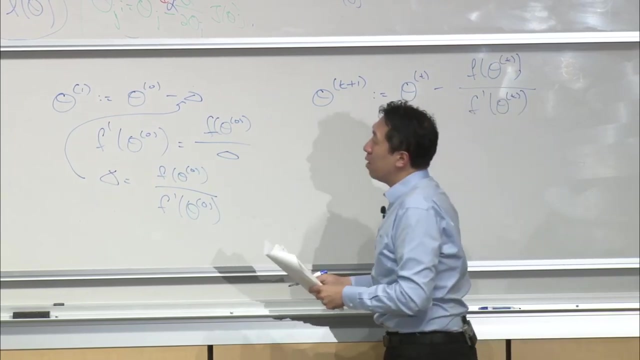 T plus 1 gets updated as Theta t minus f of Theta t over f. prime of Theta t. okay, Uh, where instead of 0 and 1, I replaced it with T and T plus 1, right, Um, and finally to- to you know. 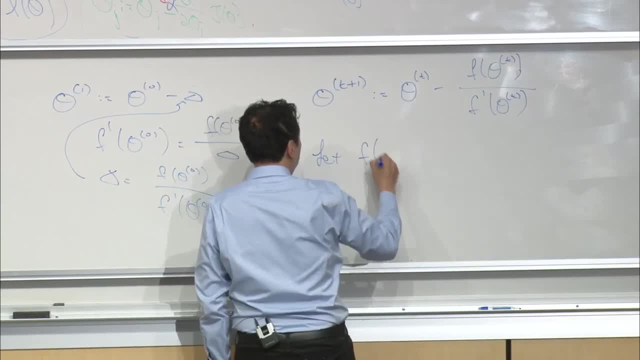 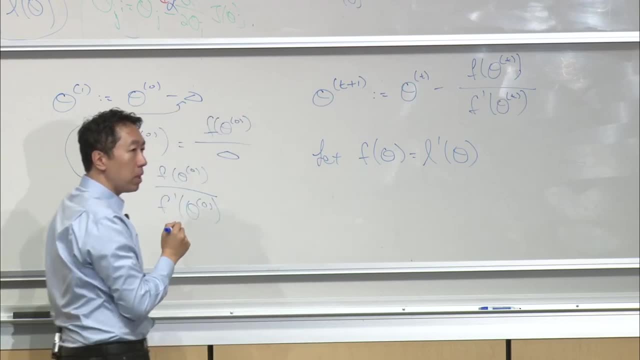 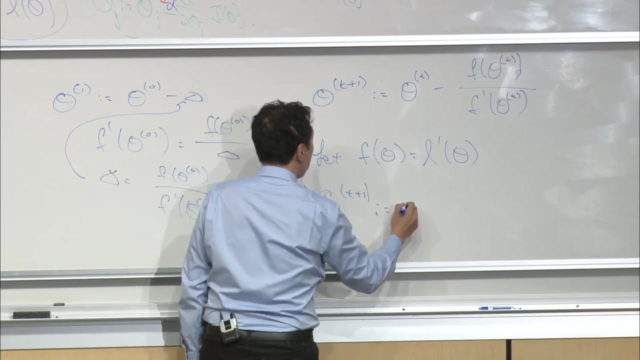 the very first thing we did was: uh, let's let f of Theta be equal, to say L prime of Theta, right, Because we wanna find the place where the first derivative of L is 0, then this becomes Theta t plus 1 gets updated as Theta t. 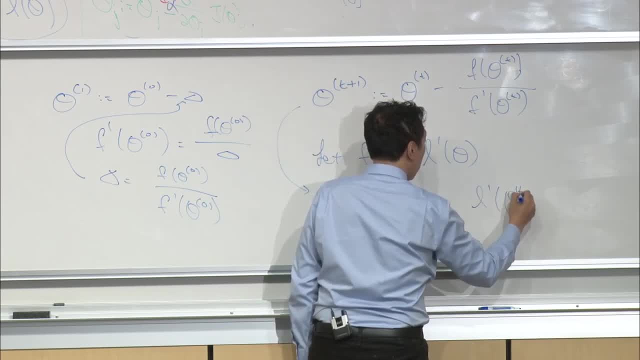 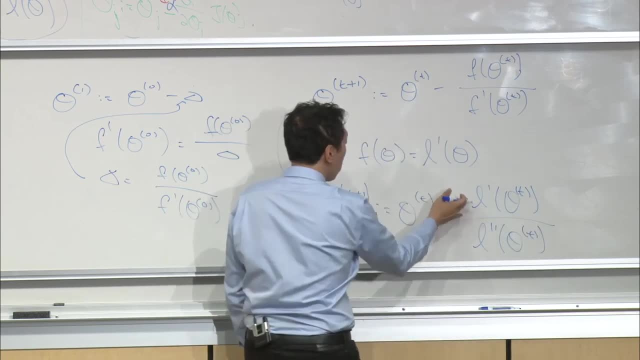 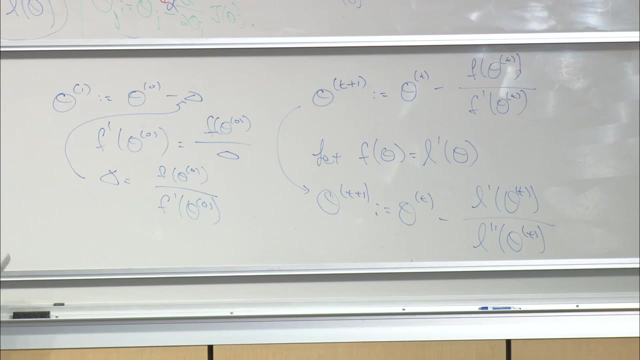 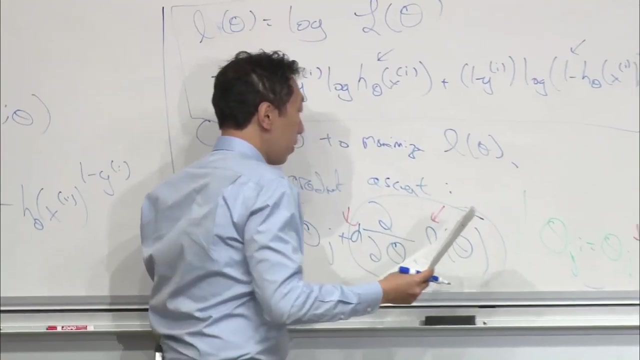 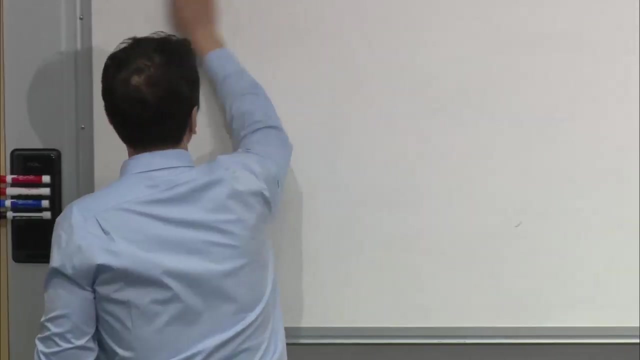 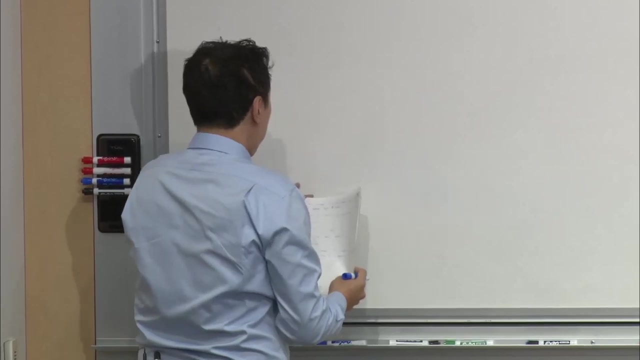 minus L prime of Theta t over L double prime of Theta t. So it's really, uh, the first derivative divided by the second derivative. okay, Um, so- Newton's method is a very fast algorithm And, uh, it has um. 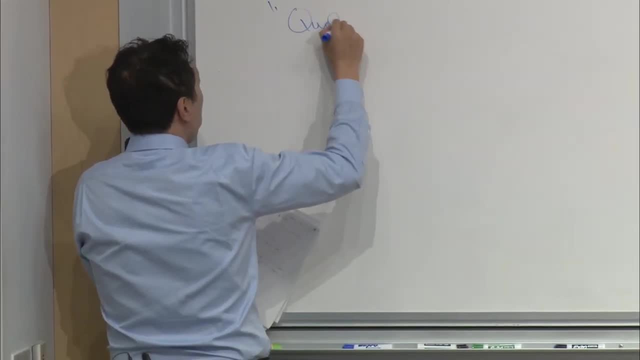 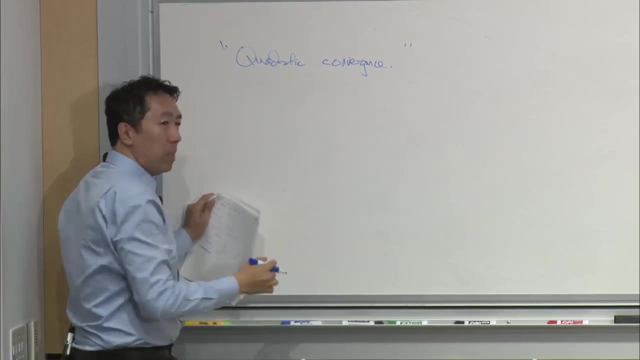 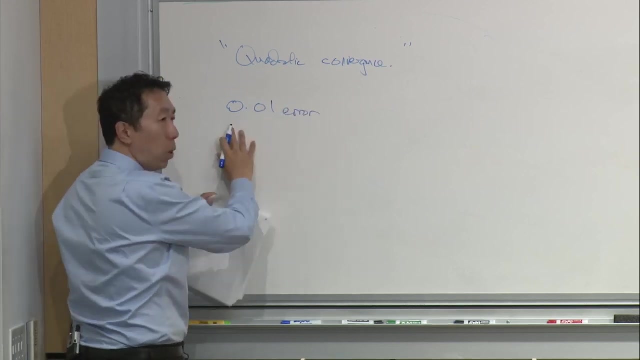 Newton's method enjoys a property called quadratic convergence. Not a great name, Don't worry. don't worry too much about what it means, But-, but informally, what it means is that, um, if on one iteration Newton's method has 0.01 error, 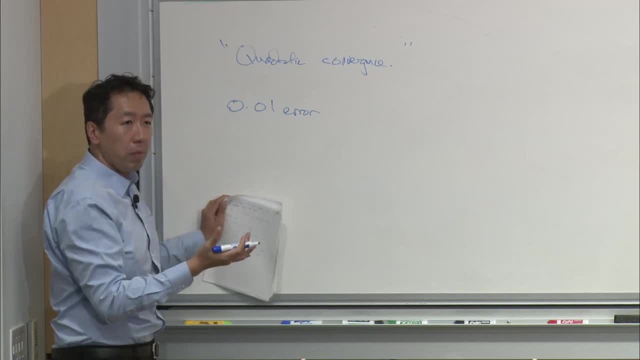 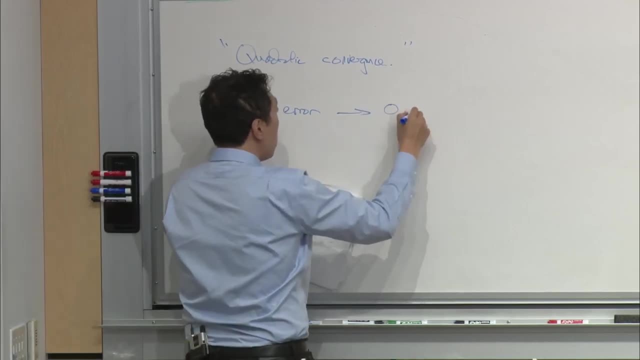 so on the x-axis, you're 0.01 away from the- from the value from- from the true minimum of the true value of f is equal to 0.. Um, after one iteration the error could go to 0.0001 error. 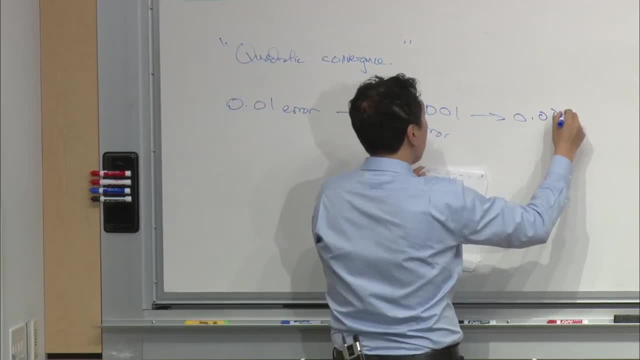 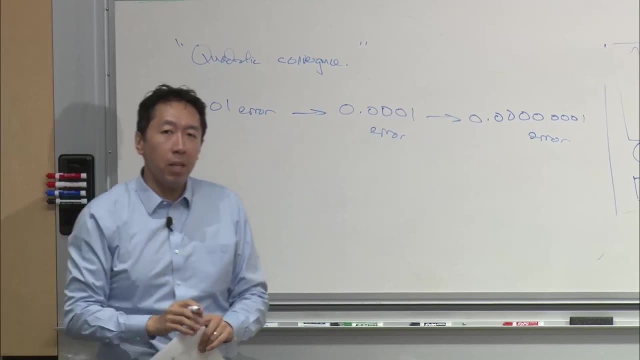 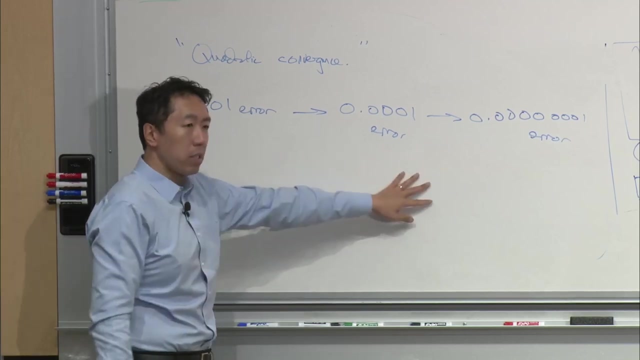 And after two iterations it goes 0, 0,. it goes 0, 0. But roughly Newton's method. um, under certain assumptions, uh uh, that function is smooth, not too far from quadratic, the number of significant digits that you have converged to the minimum. 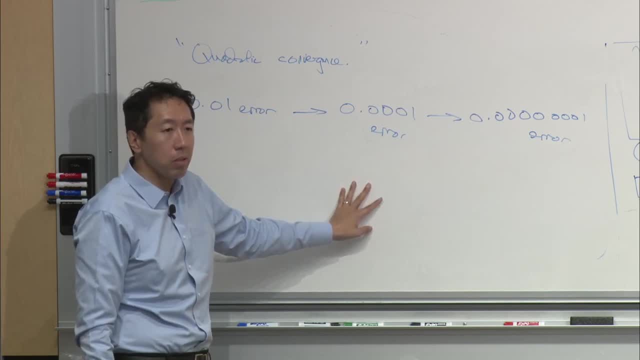 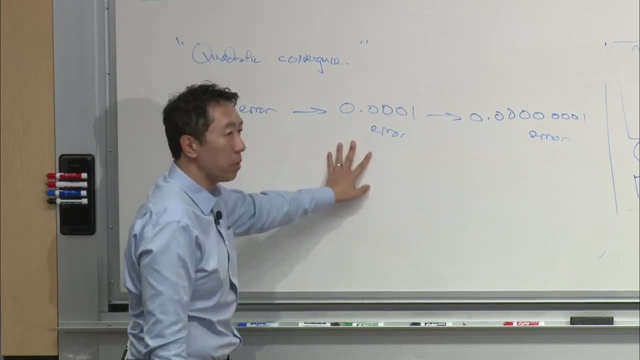 doubles on a single iteration, So this is called quadratic conversions. Um and so, when you get near the minimum, Newton's method converges extremely rapidly, right, So- so after a single iteration it becomes much more accurate, After another iteration it becomes way. 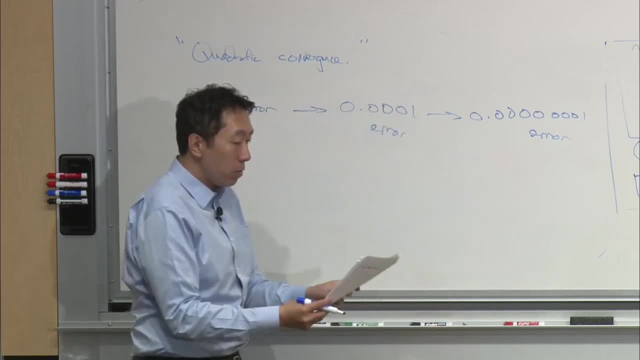 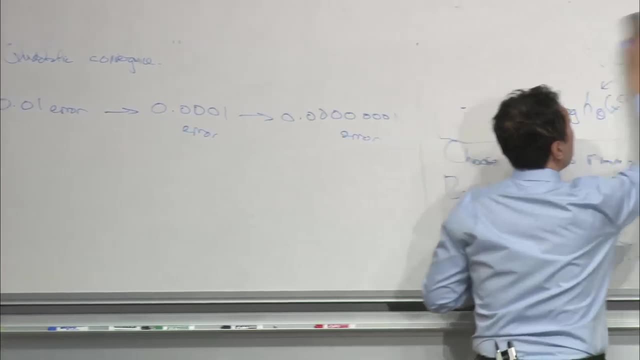 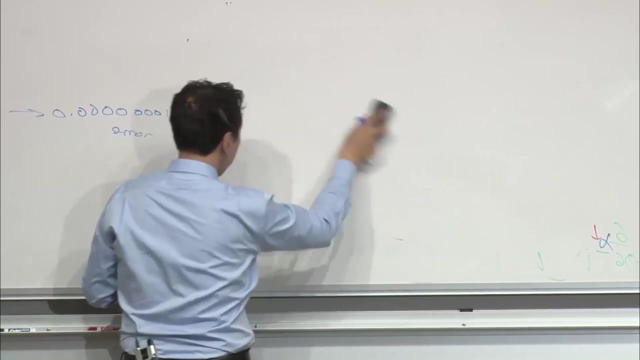 way, way more accurate, which is why Newton's method requires relatively few iterations. Um and uh. let's see, I have written out Newton's method. for when Theta is a real number, Um, when Theta is, uh, a vector, right. 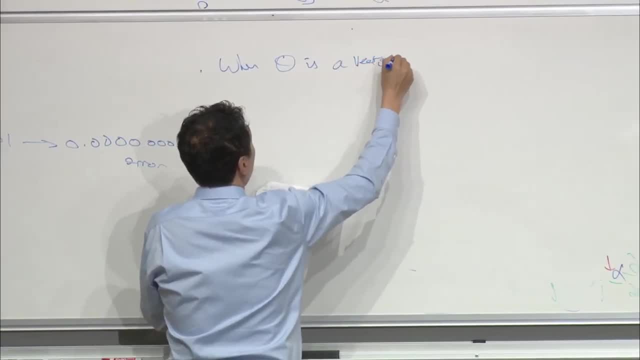 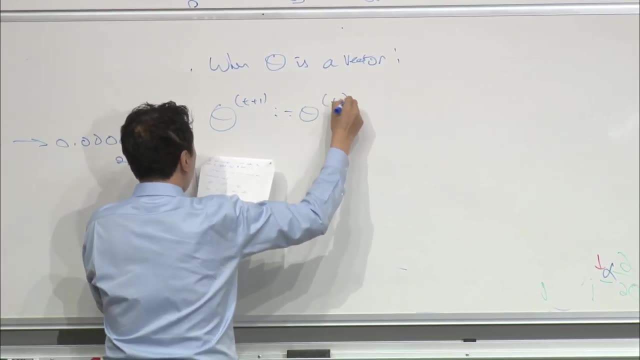 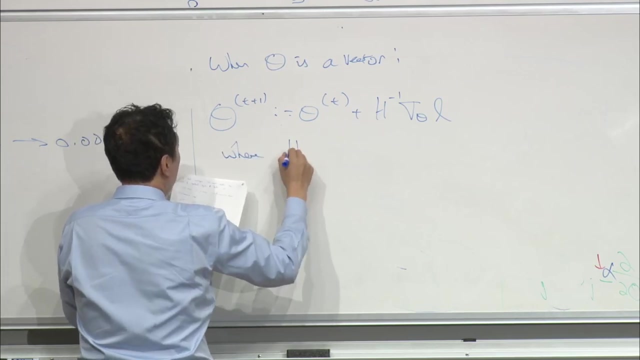 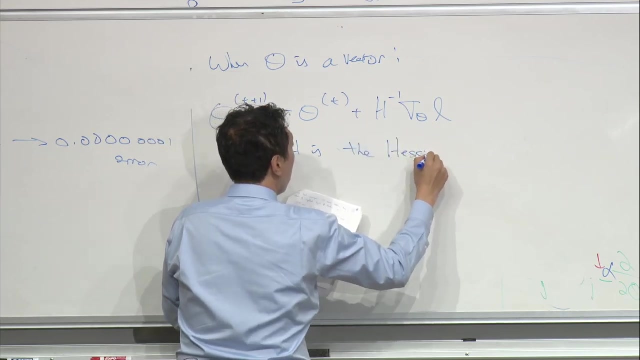 Then the generalization of the rule I wrote above is the following: Theta t plus 1 gets updated as Theta t plus h, That where h is the Hessian matrix. So these details are written in lecture notes. Um, but to give you a sense, 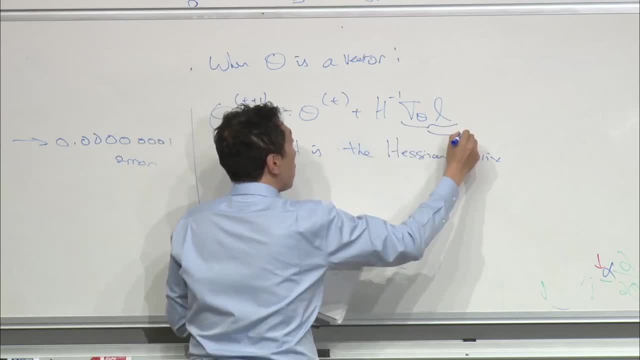 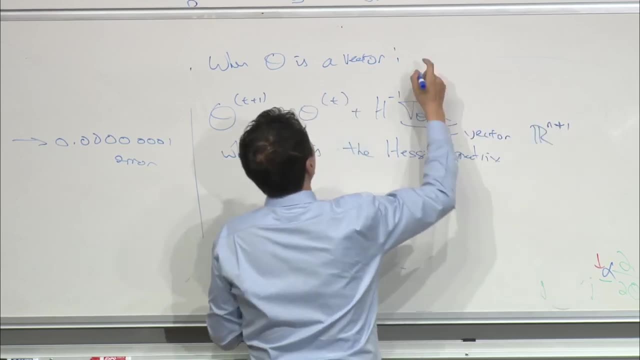 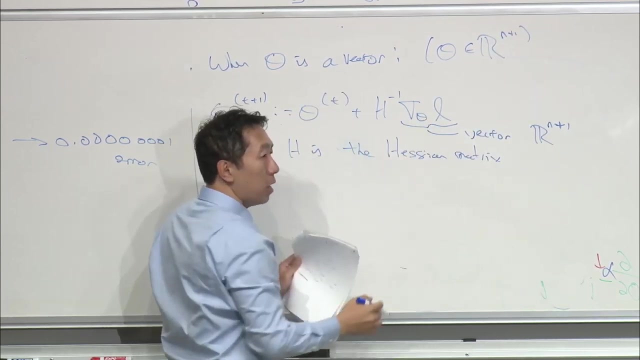 it- when Theta is a vector, this is a vector of derivatives, right? So it's- I guess, this Rn plus 1 dimensional? If, uh, Theta is an Rn plus 1, then, uh, this derivative respect to Theta of the log likelihood becomes a vector of derivatives. 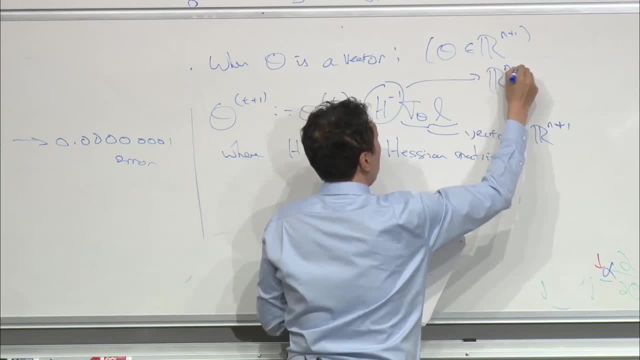 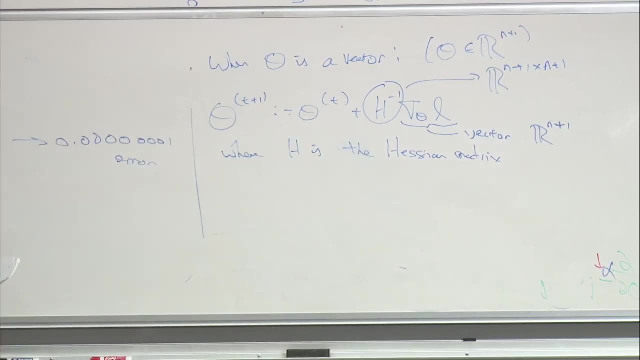 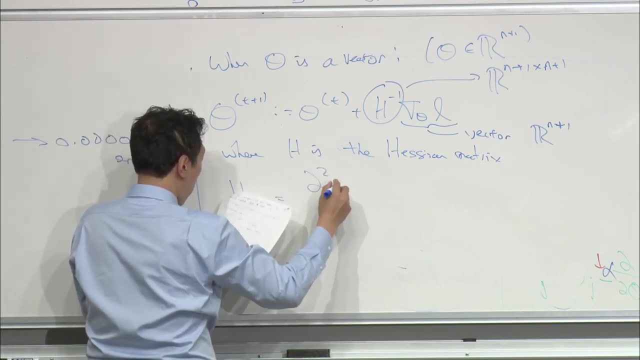 And the Hessian matrix. this becomes a matrix as Rn plus 1, by n plus 1.. So it becomes a squared matrix with the dimension equal to the parameter vector Theta. And the Hessian matrix is defined as the matrix of partial derivatives. um right, 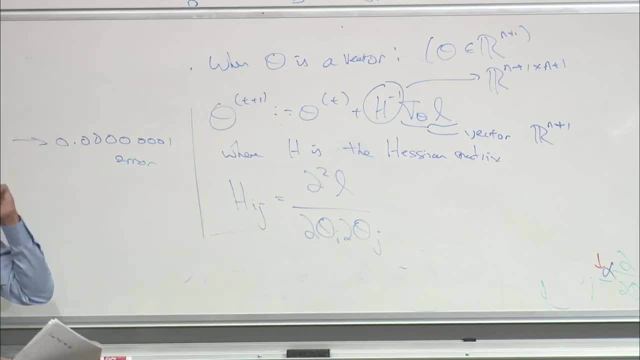 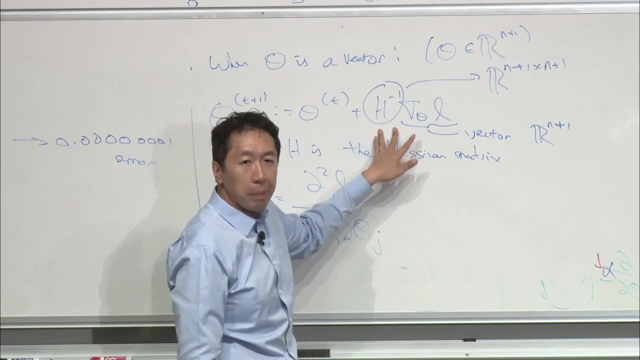 So, um and so, the disadvantage of Newton's method is that in high-dimensional problems, if Theta is a vector, that each step of Newton's method is much, much more expensive because, um, you're- you're either solving linear system equations or having to invert a pretty big matrix. 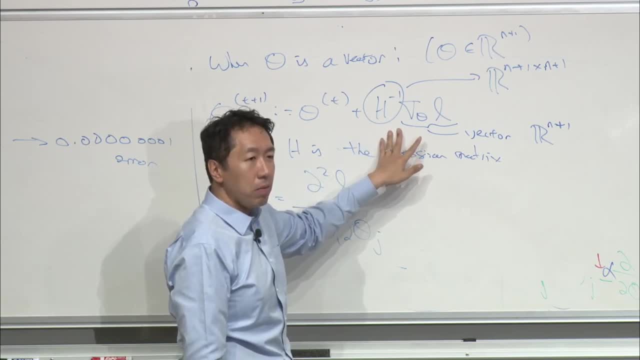 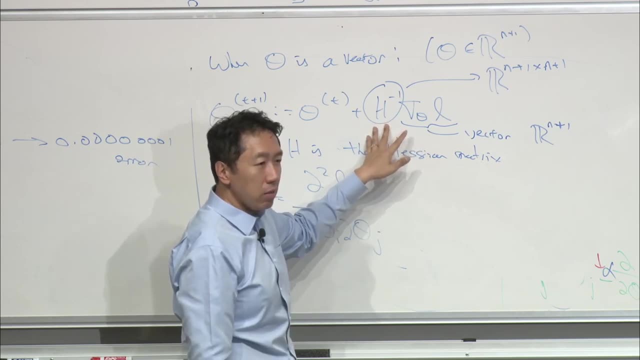 So if Theta is 10-dimensional, you know this involves inverting a 10 by 10 matrix, which is fine. But if Theta was 10,000 or 100,000, then each iteration requires computing like 100,000 by 100,000 matrix and inverting that. 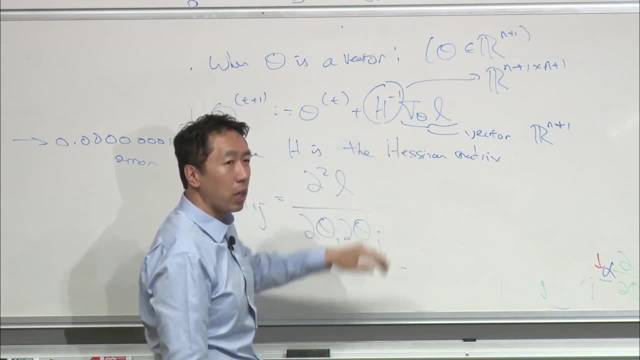 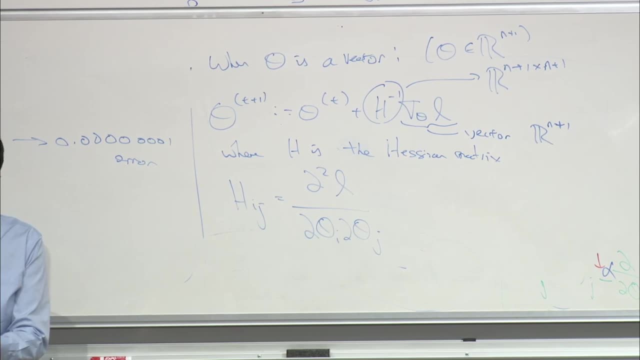 which is very hard right. It's actually very difficult to do that in very high-dimensional problems. Um, so you know some rules, some rules of thumb. um, if the number of parameters you have for the, if the number of parameters in the linear regression is not too big,